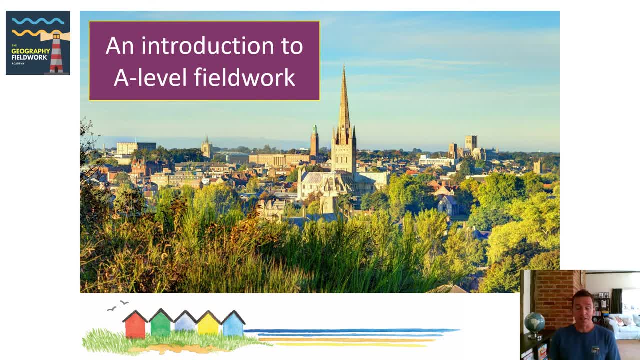 This first video here is a fairly hefty chunk of work as, unfortunately, it's quite a bit of talking, but you can skip through bits that are going to be more or less relevant to you, but the idea was to just put in a few different places the key things that you would need to know before you come. 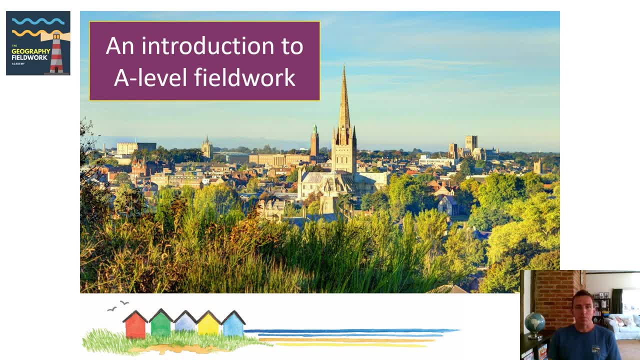 to Southwold. The purpose of this video is mainly to give you first of all a bit more of an indication about what the geography NEA is and what the geography NEA is, and what the geography NEA is, NEA is all about, because I've already kind of covered that in enough detail. that's fine, you. 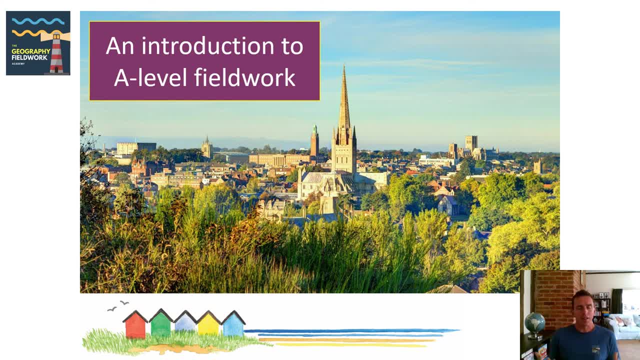 can kind of skip those sections. there's bits where I talk to you about how you could design an NEA field study, and then probably the bit that's going to be most important is going to be the bit where I'm going to give you more information about Southwold's geography itself. 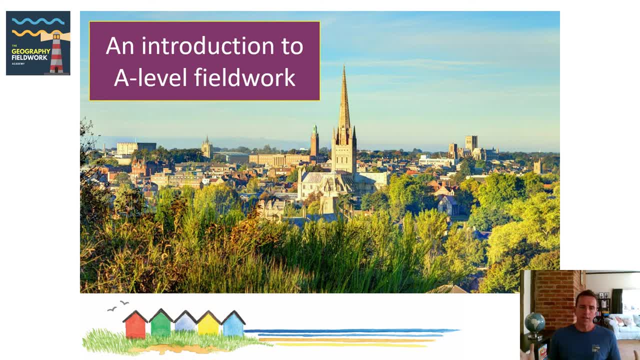 talking about the human geography in Southwold and the physical- mainly coastal- geography in Southwold, so you've got a much better idea on which issue to focus your study on. I'm also going to include within the presentation quite a bit of about different methods of data collection. you. 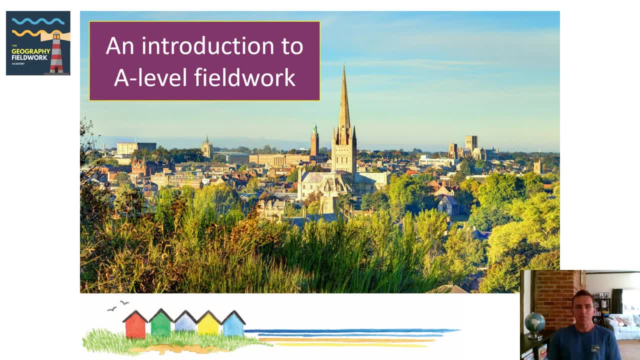 can do and use, and ultimately it should give you a pretty good introduction to A-level fieldwork and what is required of you and what you then can complete when you come to Southwold. In addition to this video, you'll have a virtual tour that I've put together on Google Earth, just showing you. 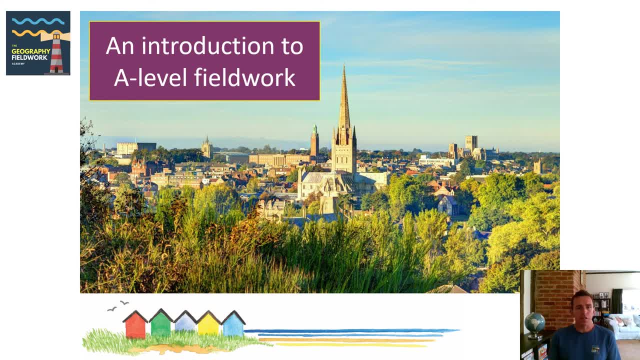 essentially the main streets, and you know the physical geography of Southwold and the key types. and in addition to those two videos, your teachers should be able to provide you with one of these as well. a booklet doesn't have to be an A5 one like this, but a booklet which is titled geographical. 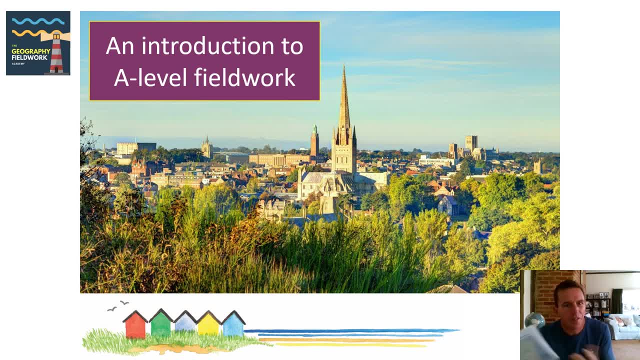 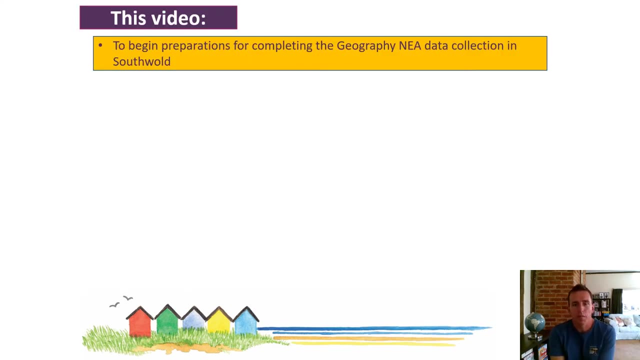 issues and fieldwork methods, and that covers quite a lot of the stuff that I'm about to cover in this presentation. so make use of all of these things if they're going to be helpful to you. so to start off with, then, just to give you a bit of an overview about this video, which I've 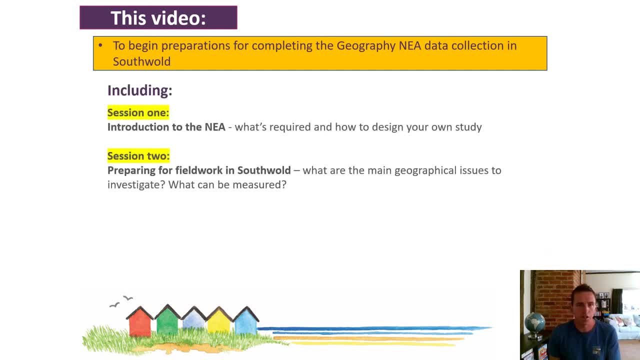 already done is that it's going to be including two real sections. the first one is going to be where I talk to you about what the NEA is and what is required of you, how perhaps you might want to structure it and design it, and the different sections that, logistically, you'll 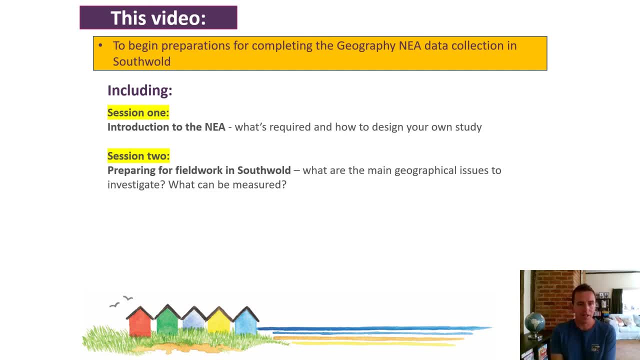 probably need to include within your study. the second section, as I say you might just want to skip straight away to section two- is where we're thinking more about fieldwork, specifically within Southwold. what issues can you study here and what can be measured? so obviously everyone around the country this year is having to slightly adjust. 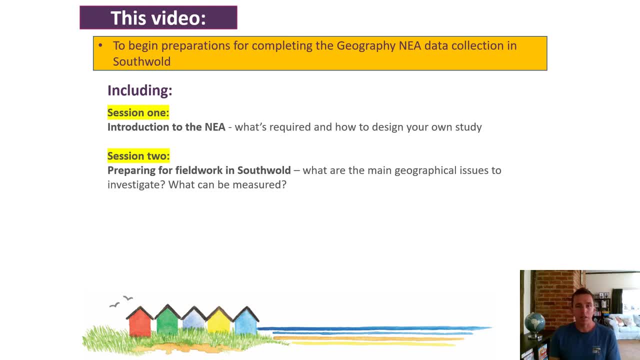 their plans and slightly tailor what they're going to be doing, depending on the information that they collect. they can collect, but also, obviously, the places that they can get to. so you've got a real advantage. you're not just collecting fieldwork data in your local area. 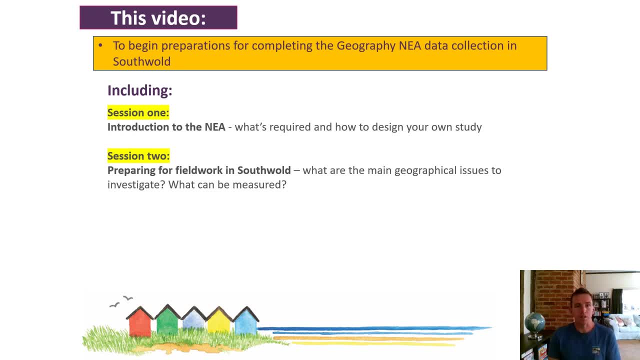 which you know, the vast majority of people this year, in year 13, will be doing. so you're actually being taken to somewhere which is- but I might be a bit biased, but it is- an absolute geographical gem. there's a huge amount of variety of geographical issues, particularly coastal geography, obviously. 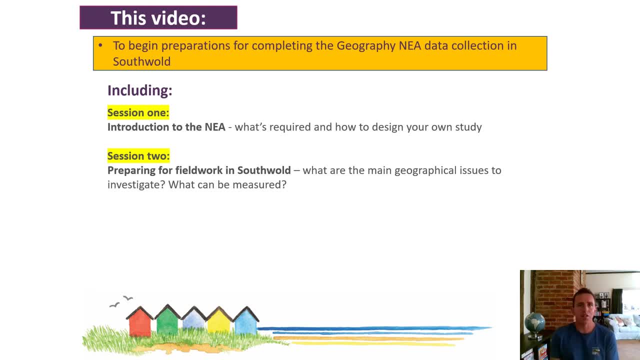 it's a coastal town, so you'd expect that, but it's called coastal management methods. it's a place where there is evidence of a sediment cell. there's a real kind of strong coastal identity in the town. they're all main coastal processes that are evident in the town. 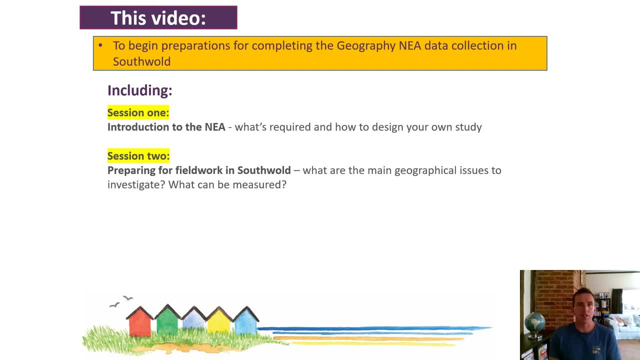 it's also a place that's been affected by storm surges in the past and rising sea levels in the future, so from a coastal perspective, Southwold is fantastic. another logistically good thing about Southwold is that the shoreline is very compact, so within 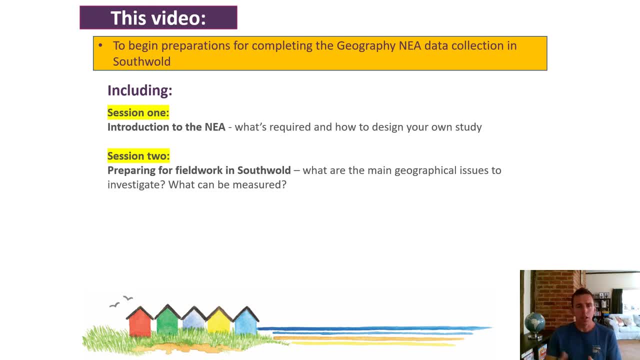 the space of about a mile, or perhaps just over a mile and a half or so, you have got the Southwold seafront and you're not having to trek a huge distance in one direction or the other to get to different sampling sites. you've got a huge amount of variety within a nice compact area. 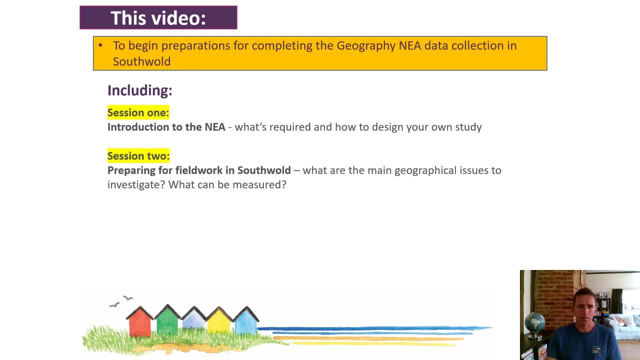 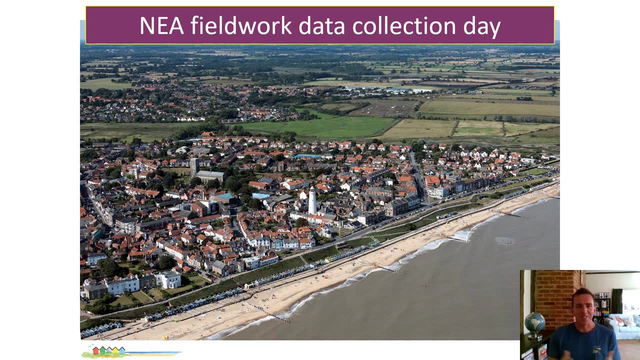 and then from the human perspective as well, we've got a huge amount of issues we can cover and I probably should have skipped onto this a little bit earlier so you can see the town as I'm talking about it. but obviously Southwold sits on the coast there- the North Sea. it is challenged and 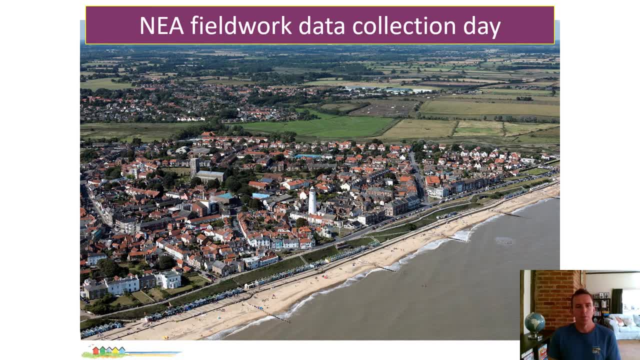 threatened by the sea, but also there's change and challenge in the town as well, and over this presentation I'll give you a bit more information about the challenges that Southwold as a community and kind of generally the town faces, and linking those all in into the geographical views that you 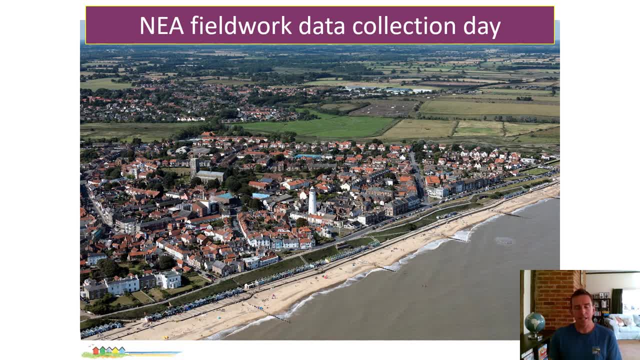 can cover. so we're kind of building up to this the NEA fieldwork data collection day should think of for that day, but that's that's what we've got there. so you have got these data. well, this data collection day where you will be coming to this town and when you get here, essentially, apart from 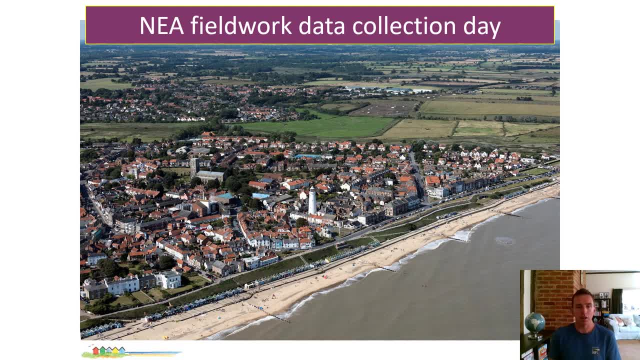 asking me a few questions and perhaps me demonstrating a few of the methods that you might not be familiar with. essentially, we're asking you to be as prepared as possible before you come so that when you get here, you can waste as little time as possible and you can get out and 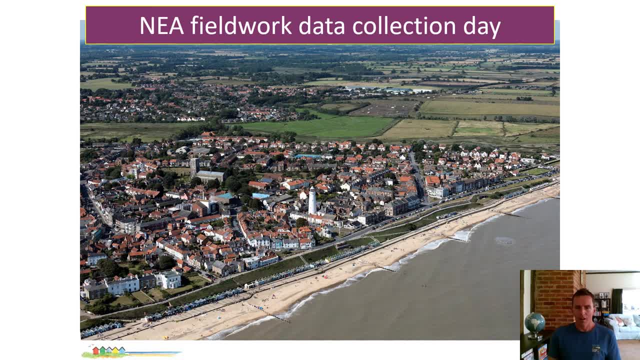 about collecting the data that you need- your study. I will obviously be on hand to help you as much as you need for that and to point you in the right direction, to demonstrate things that you're unsure about, but ultimately, what you need to do in the weeks before you come now is to try and get 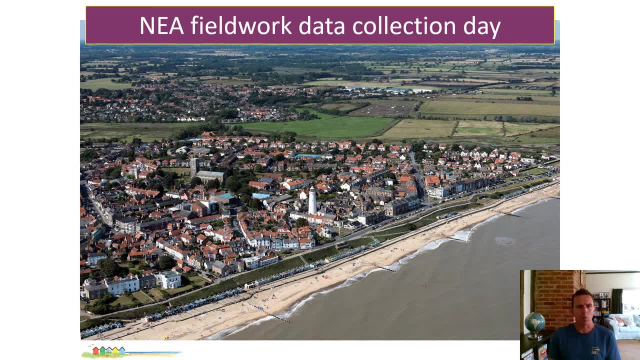 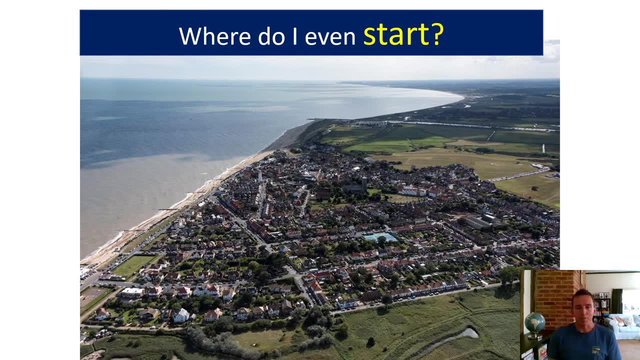 yourself prepared as possible so that you really make the most of your time when you're actually in Southwold. so this may all be a bit overwhelming. you might think, oh blimey, this is a bit of a shock to the system. I'm being told I'm going to have to do some field work. I don't even. 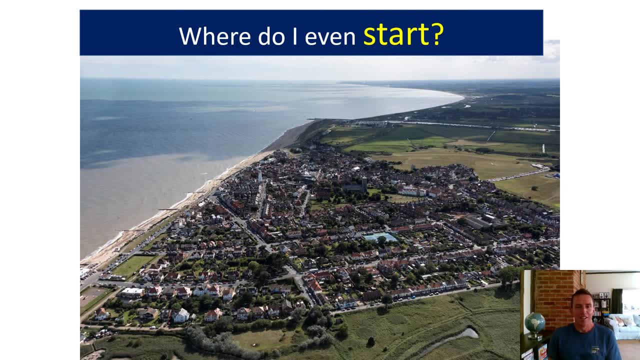 know this place. I've never been here before. I've got no idea what it's like, so I'm just going to have to dig into some of the resources that you've you'll be given so initially, at any starting point of any geography fieldwork investigation, there is perhaps a little 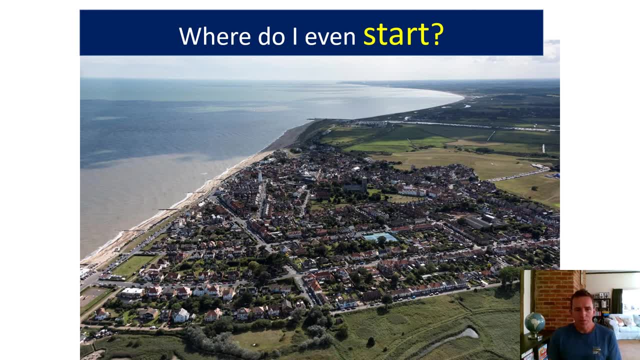 bit of a feeling of apprehension. you're told that this is a significant piece of work and it's got to be as good as can be, and you're probably going to be very keen to make this as good as possible. but you then might be feeling a little bit skeptical about making it as good as possible. 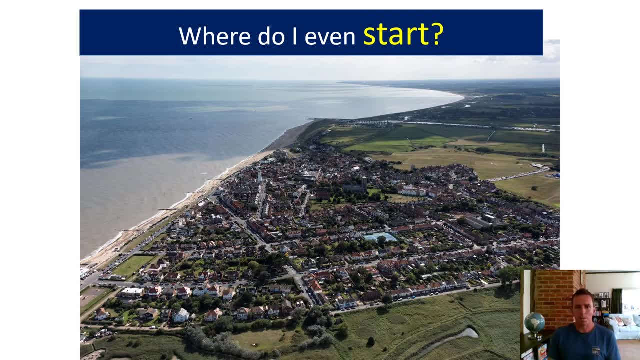 in a place that you're perhaps quite unfamiliar with. so a few things that i should say about south pole to start off with. firstly, hopefully- as you can see from this image here on your screen- is it's pretty small. actually, it's a very small, compact place. lots of people might go and do. 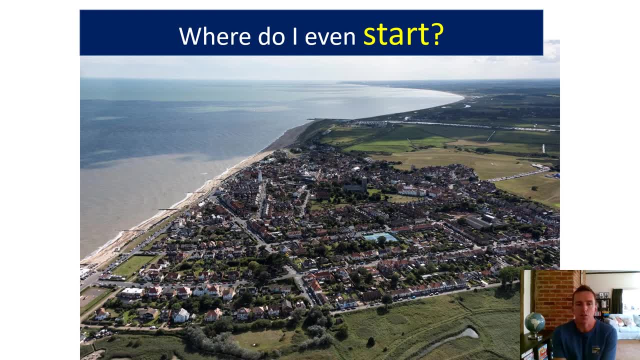 their field work in cities or in larger coastal towns or communities, which is fine. but south bold's advantage is that it is compact and even though it's compact it's got a real huge variety of geographical issues you can use and focus on, so it's not an over overwhelming place to get to. 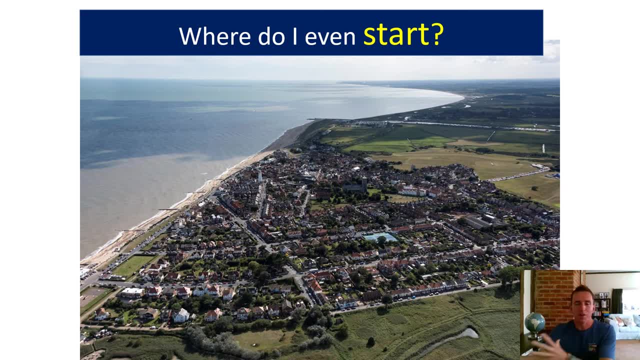 know it's not like we're taking you to brighton or you know somewhere like liverpool or manchester, these big, you know urban areas where you're actually struggling to kind of comprehend where everything is and how you get from a to b. southfold's got a high street and it's got a. 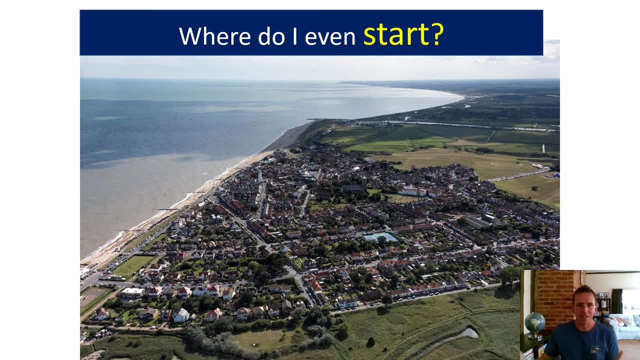 sea front and pretty much between the high street and the sea front you've got several kind of smaller residential streets and very quickly you can get in bearings. and you know, as you can see from this image here, it is not a huge place at all. our base away is: 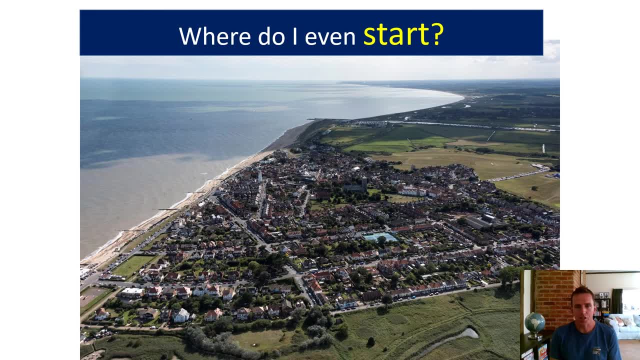 right in the center of that um image you can see a church, hopefully right in the center of the image, just to the left of the church or to the east, which is to the um seaward side of the church. there is a building right behind it which kind of looks as if it's set in kind of um parkland. well, 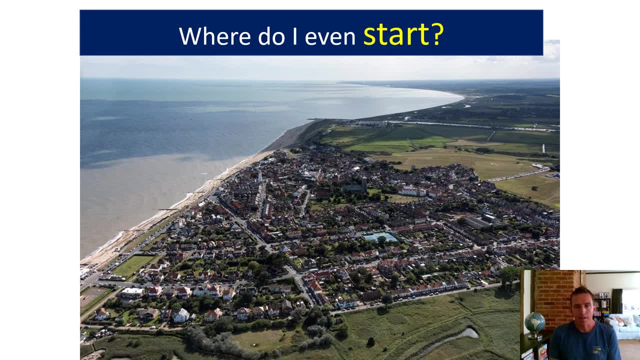 that is our building, that is the south pole art center, and, um, we have use of a classroom in there, which is the south pole art center, which is where you're going to be using when you guys come, or um, depending on the size of your group, we'll be using the actual buildings theater, so it's. 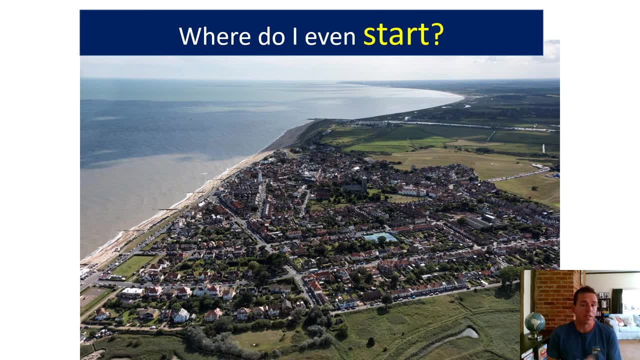 essentially south wold's theater and the south pole arts and um. it doesn't look like a significant building at all from outside, but you go into the front door and the whole building kind of opens up around you. we'll be upstairs, probably in the classroom, when you guys arrive, so this is where. 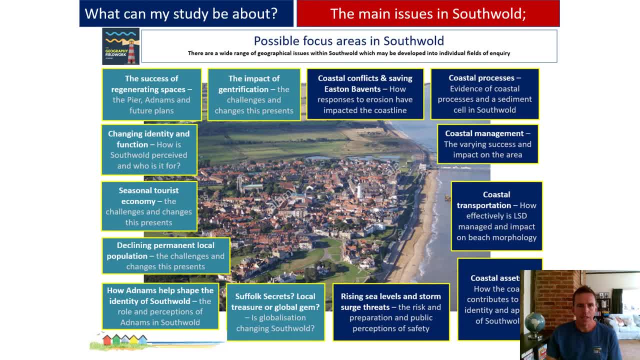 you're going to start and the starting point is getting to know south wold a bit better. you have to be a little bit more such a you know you can have an issue that merges a couple of things. so you can see, here i've selected a surface like this, that's a flat surface like this, and you can see in your booklets that. 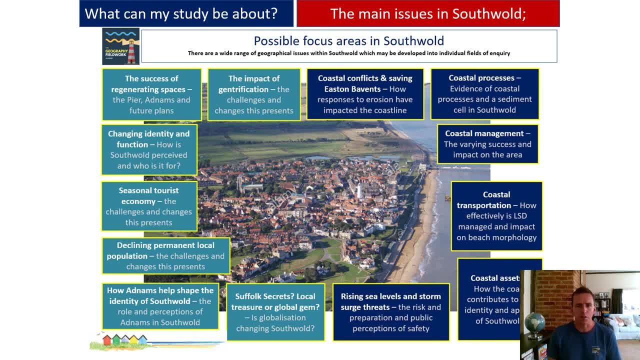 You know you can have an issue that merges and crosses the boundaries between the two. But on the right hand side you've got those themes that are linked to coastal geography, physical geography, And the ones on the left that are probably more obviously linked to human geography. 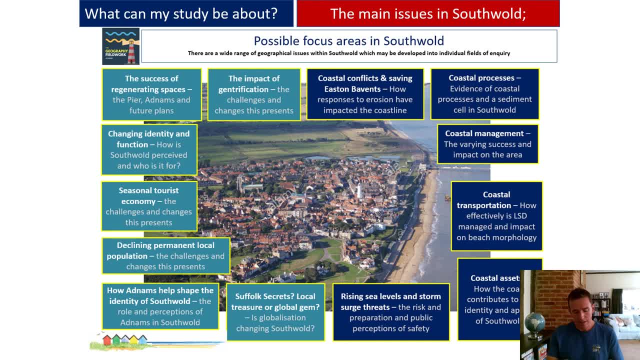 So when you've got more time or if you want to press pause on me and just kind of look through these issues, then do that. But you'll see that there is a significant variety. Some people are kind of naturally more inclined to do coastal studies. 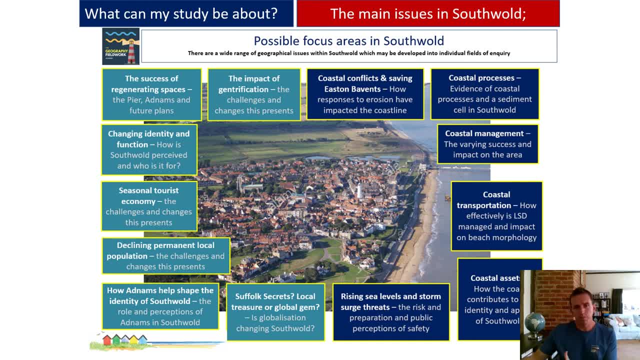 Very often some people- perhaps more science based people- choose to do coastal studies because there are generally more opportunities for kind of fairly quantitative studies where you're measuring, collecting data. You're perhaps getting more definitive black and white answers. You've also got kind of more obvious theories perhaps that you might be able to tie your studies in with, like the idea of sediment cells or longshore drift. 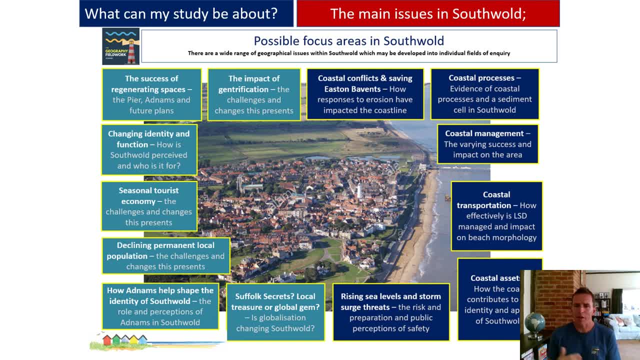 And And then the- you know- coastal morphology and how that perhaps varies along in code time. However, the joy of Southwold is that you've got a real variety of issues And, from a human perspective, we're definitely not undersold. 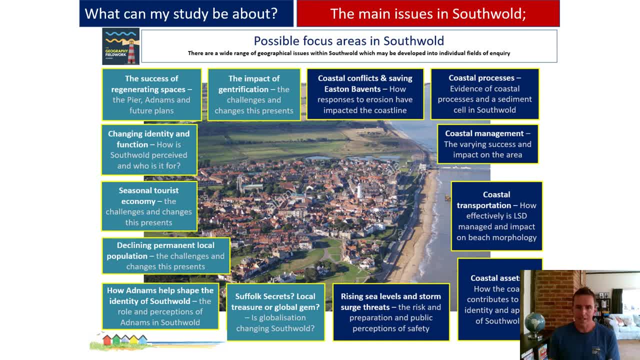 And there's plenty that you can investigate here. The whole identity of Southwold is an issue that could well be investigated further. Southwold's identity, I suppose, is probably this fairly traditional, quintessential British coastal town And physically you might look at it and think, well, this is a place that hasn't changed all that much over the time, over years, because you know, still got these kind of traditional things like here and the lighthouse and these kind of quirky independent pubs and shops and sweet shops and ice cream tellers and stuff like that. 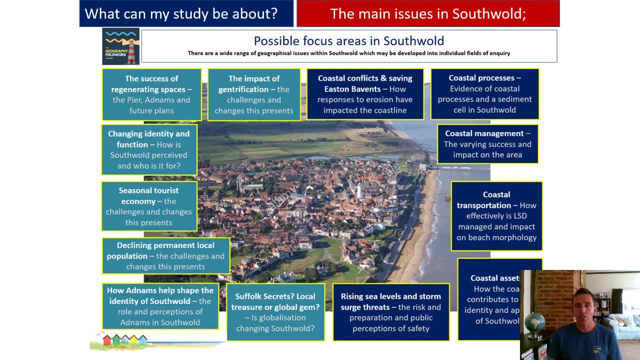 So the identity of Southwold is one of the key attractions of it. But scratch away at the surface a little bit and you'll find that there are lots of other issues that are perhaps less obvious, but just as obvious And just as important. Southwold's community here in the last 10 to 15 years has been under attack, which sounds dramatic. under attack from a kind of what seems to be a one-way process of a movement towards increased second home ownership. 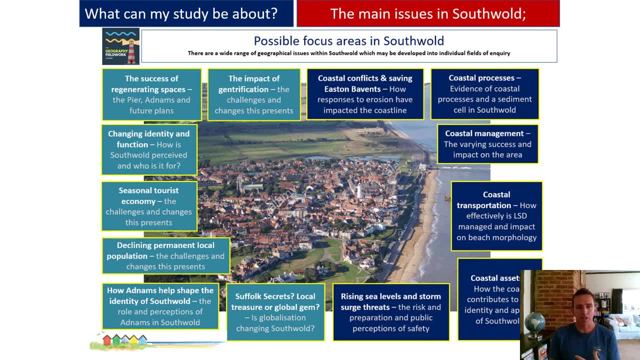 And again I'll talk to you a little bit more about that as we go through the presentation. So Southwold is, as far as I'm aware, probably the town in the country that has been most significantly impacted by the increased amount of second homes in the last 10 years. 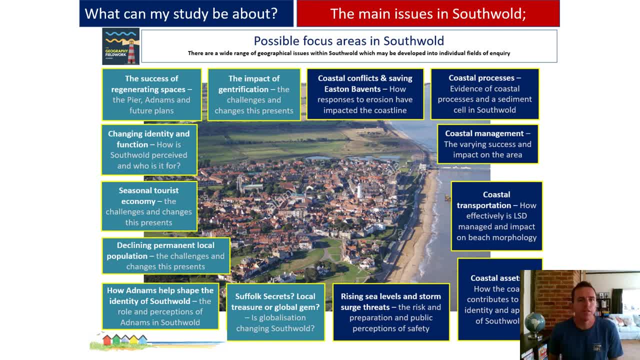 In the last 10 to 15 years it used to be the case generally in this country that if you could afford to buy a second home, that you'd go and invest your money in places like France or Spain or Portugal. But actually since we left, since the euro was introduced in 1999, it's actually been less viable to do that. 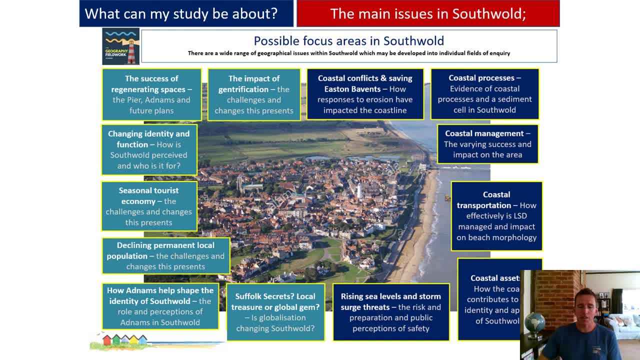 And it's actually coincided with a period where this kind of staycation and Airbnb culture has existed And more and more so people are. People are actually willing to invest in property- second home property- in the UK- And they're seeing actually returns on investing in second home property are quite good as well, because there's now more demand for people to go away for weekend breaks. 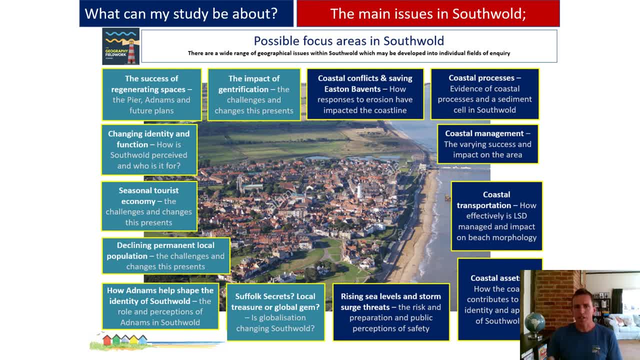 And if you buy a house by the sea, you might only physically go and visit it for four or five weeks a year, But actually in the rest of the time you can potentially use that property as a sort of income by letting it out. 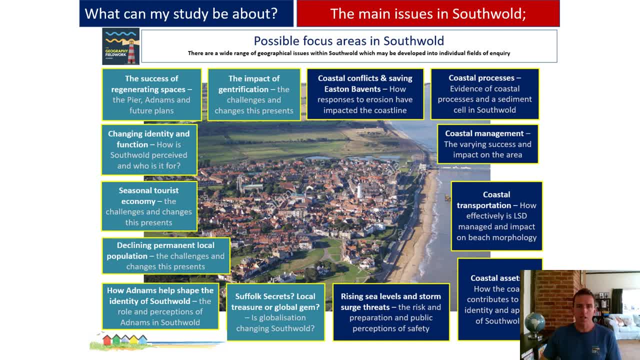 And that's what Southwold has. It has a number of these second home properties that are used. sometimes Some of them are owned by their second home owners, but are also, for a considerable amount of time, are actually just let out to holidaymakers. 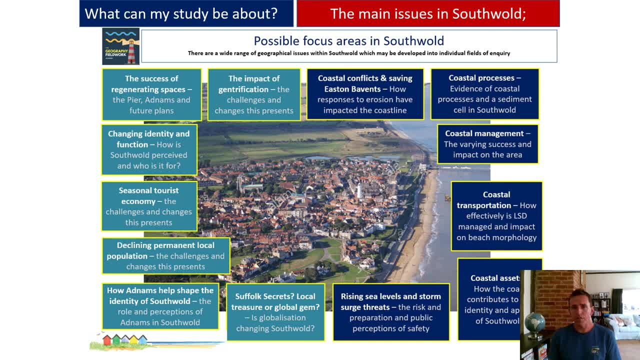 And there are several companies in the town who have a business based around that whole process, where they essentially take on these properties from the owners And they then recruit people to stay in them by advertising them on their websites. So this has had a significance. 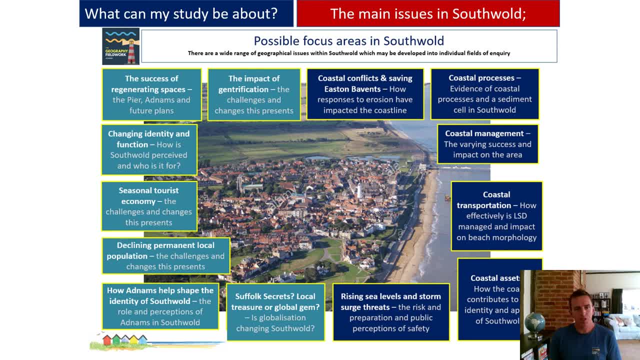 This has had a significant impact on the town. We'll also introduce Adnams. You may or may not have heard of Adnams. Adnams are a significant brewery and they've been brewing in Southwold for over 100 years. 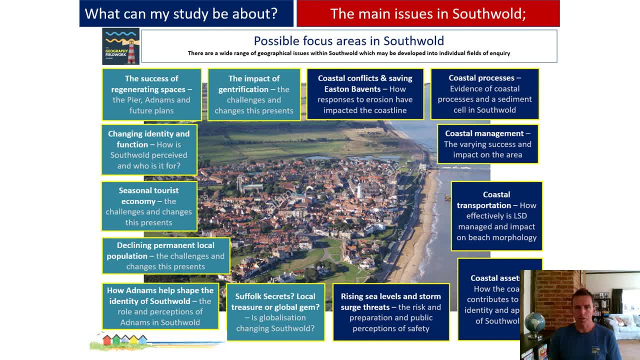 But actually in the last 10 years they've also gone through a significant business change and diversified what they're doing to now include a distillery So they can make things like whiskey and gin and vodka, And they actually make award-winning drinks that have been given internationally. 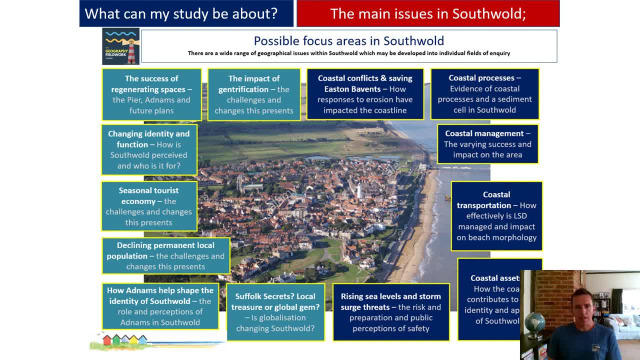 And they've won national kind of crowns and statuses by, you know, winning significant events and classes across the world. So Adnams is a significant player in Southwold, probably the biggest influencer, probably the biggest social media influencer. 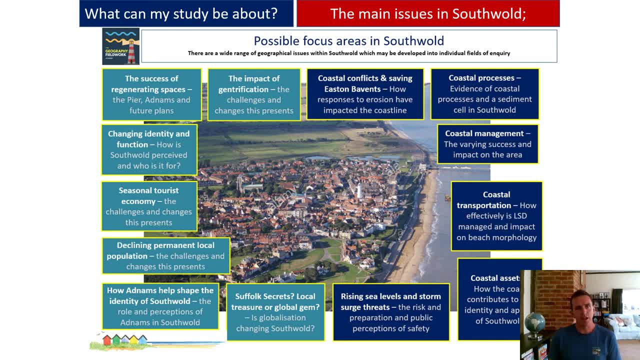 They have a huge following on Instagram and Twitter and also Southwold's biggest employer. They also own a huge amount of Southwold. They own probably Southwold's biggest- I think that definitely Southwold's biggest shop- and several of the main hotels and some second home. 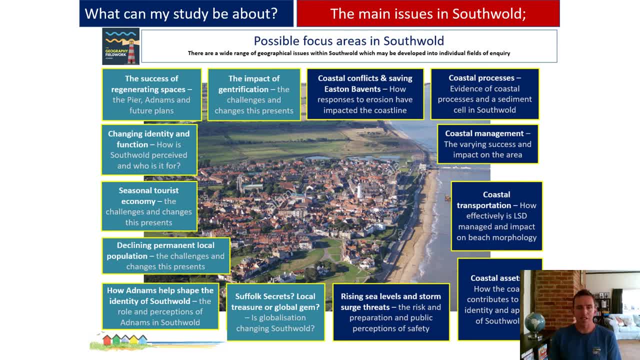 Well, they've also overseen a large redevelopment project in the town and are, you know, a huge influence on the identity of Southwold. We'll look at that too. A couple of the other issues are to do with changing demographics in the town. 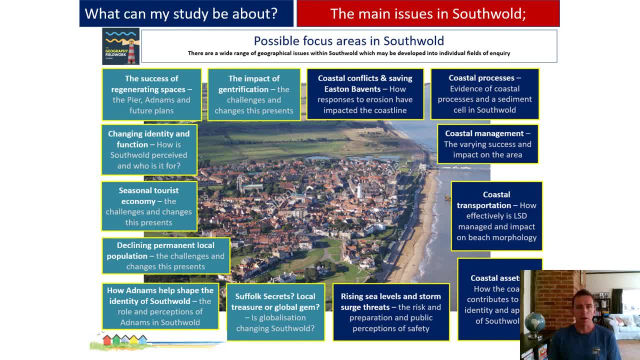 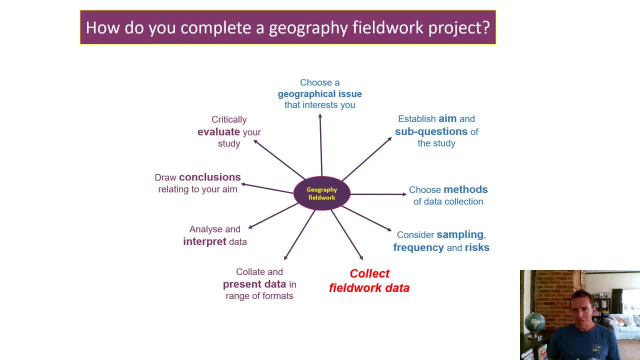 But a lot of these are then linked into the process of second home ownership. So I'll explain that in more detail as we go. OK, on the second page of your booklet here you have this kind of fairly slimmed down diagram to represent the process that a geography study naturally goes through. 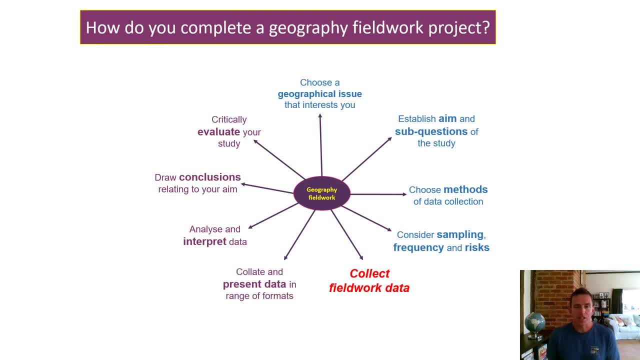 So I think it's useful just to draw this to your attention because actually you know many of you will have completed investigations in science and perhaps in other subjects as well. You guys are one of the first year groups where you haven't done your own independent field study at GCSE. 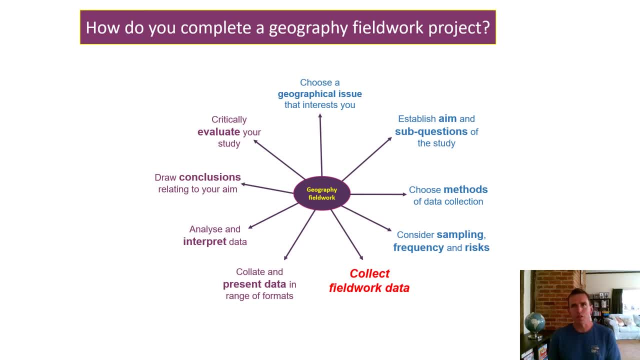 It used to be that up until three years ago- three or four years ago- that GCSE geographers had to do their own fieldwork project- A little bit like what you're being asked to do now, but slightly less detailed and less complex. 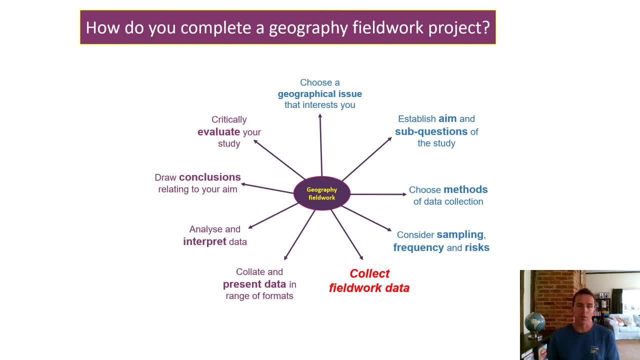 And so for those students, if they were then being asked to do it at a level they had this kind of foundation where they'd actually already gone on before. So doing it- It's called fieldwork project- would be perhaps a little bit more straightforward. 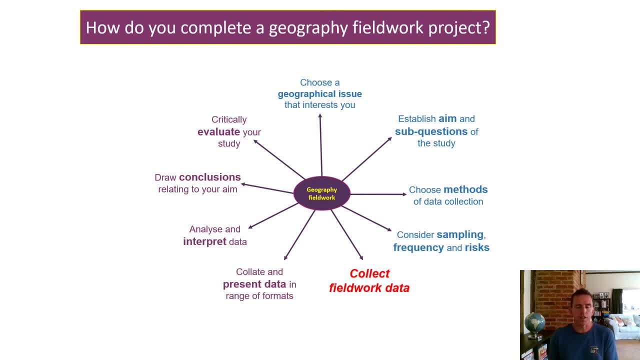 But you guys have not been asked to do this before your geography careers, unless you've been asked to do it in stage three. But at GCSE you would have been taken away somewhere to do your fieldwork- a human and a physical study. 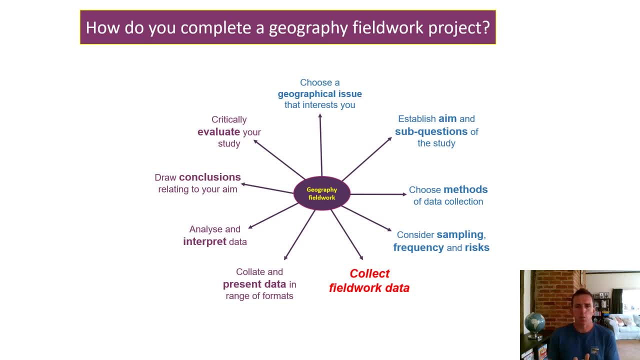 But probably more often than not, those studies will have been organised and logistically planned by your teachers, and your teachers will have taken you to a site that have told you probably what to measure, How often to measure it, for how long, what equipment to use, how to record it, and then, probably back in the school classroom, how then you would present that data. 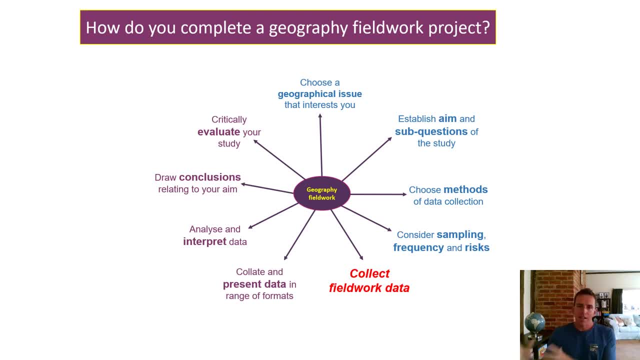 And then you draw conclusions from it and then you'd use that data in that section of the exam to help you answer the fieldwork questions. So that's different now. Now you're being asked to create your own unique fieldwork project, and you're being asked not only to do that, but to plan every single stage of it. 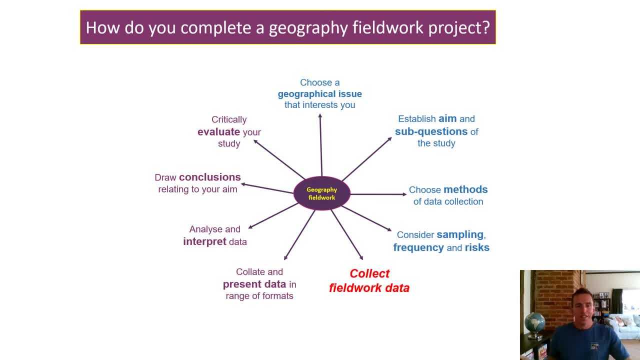 So you might think, Well, I don't know how to do that. I've never done this before. Okay, so this is just a clear, logical sequence of the stages that you then will be expected to kind of move through. The first bit here, then, is what we're going to focus on, for the next little step is the key thing that you have to do. to start off with, then, a project is to pick the issue that your study is going to be on. 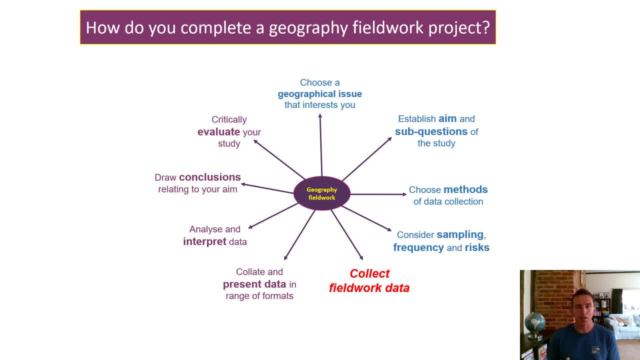 this would be a challenge. if you were just doing your study in your local area, you might think, well, there's a lot of probably going on around me. there probably will be, but i can- you know- confidently say that when you come to south pole, you're being brought to a place where there are a 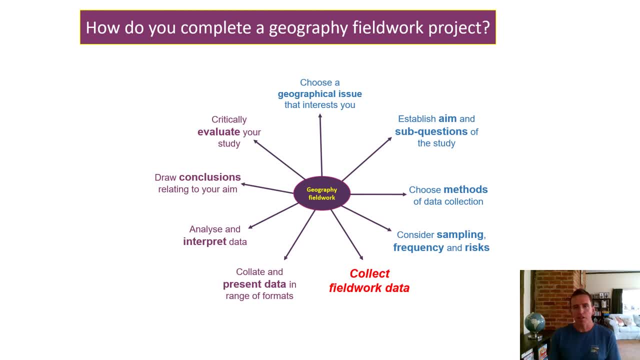 huge amount of geographical issues that you can focus on, which we've already touched upon. so this is your first challenge, and you will need to do this before you get to south pole. you're going to need to select the issue that i talk about today and that you perhaps might research. 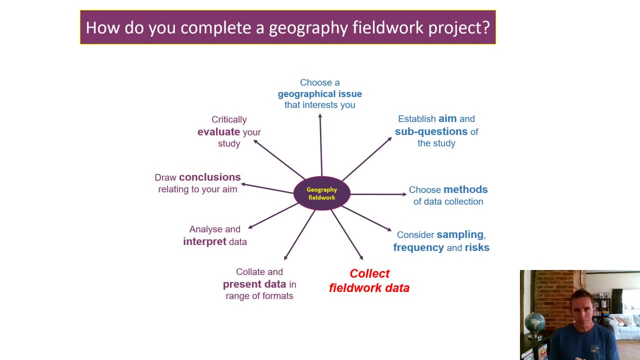 later interests you the most. that's your first thing that you have to try and do. from that point, then, your second challenge is to start to think about: well, what questions am i going to ask about the issue that i've selected? what is it that i actually want to investigate about total? 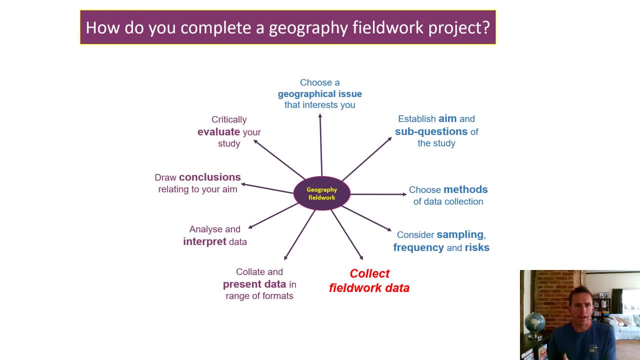 management, for instance, or what is it that i want to find out about the impact of gentrification in south pole, of second homes on on south pole? the second bit is where you then try to kind of extract a question from the issue that you've selected and that will probably require you to. 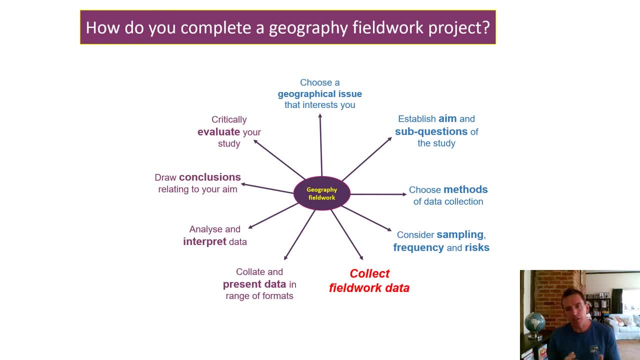 have a bit of backwards and forwards from your teachers and for you to perhaps propose an initial question, your teacher might say: well, actually i'm not sure about that, maybe we might need to scale it down a little bit, or maybe we might need to think a bit more about going down that road. rather, 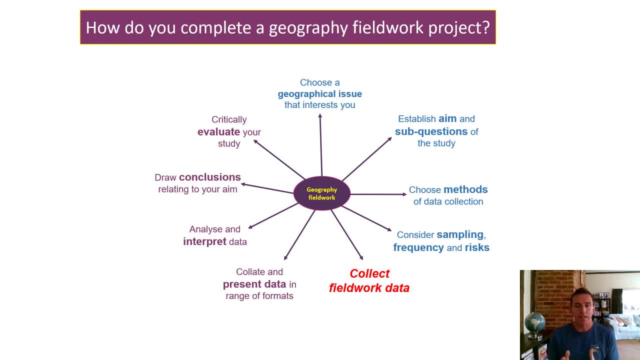 than doing that, because that might not be feasible. so inevitably at that stage you'll need a little bit of support from your teachers. if there's nothing, if there's no, there's a question that you like to ask me at that point, then you're welcome to to email me and say: look, chris, i'm thinking of. 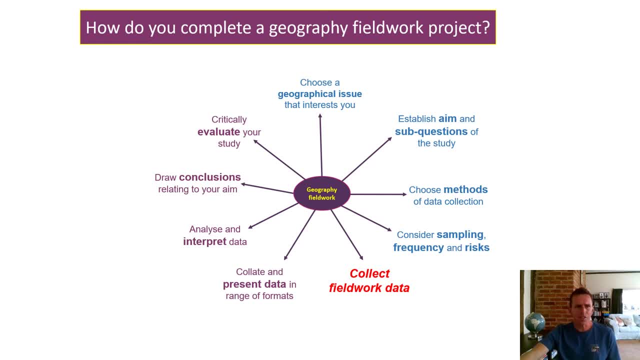 doing my study on this in south wold. do you think i'll be able to get information on this and how do you think i might be able to get it, or what do you reckon? am i better, perhaps, focusing on this angle of this? so that is a stage that is quite fluid and flexible and is essentially the stage 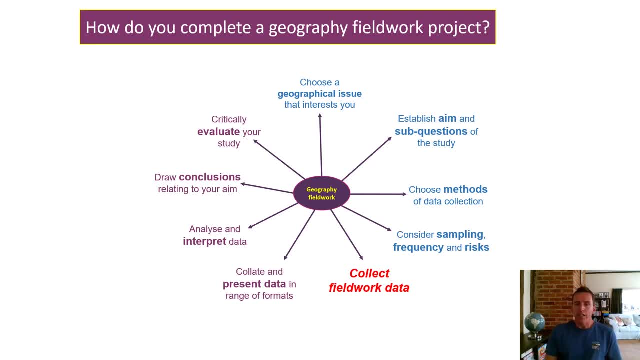 that you will be doing over the next few weeks. you will also then, once you kind of got the green light to the title that you have proposed, you'll then also need to think about how am i going to collect data to help me answer the questions i have set, and it might well be that at that point you think 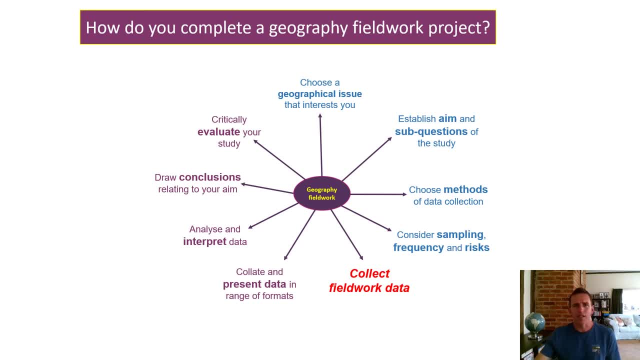 actually, yeah, i like the question, but i'm going to get any data for it and that then might ask you: it might require you to then go back to that second stage and think, okay, then maybe i need to re-dig my question a little bit, because i i'm going to need to get data to help me answer it. so 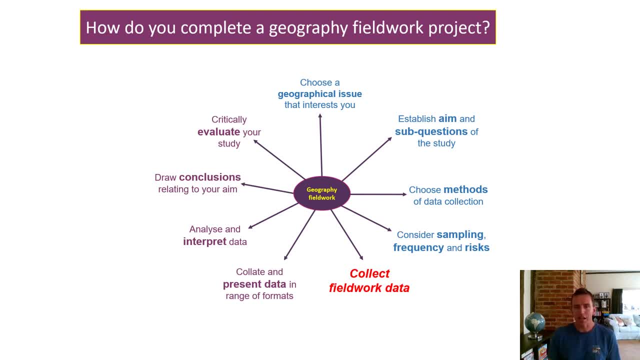 that third stage, there is quite important choosing the methods of data collection that you will use to collect your primary field works. primary field work is data or information that's been gathered by you and you only, and um, you're going to have to think about what primary 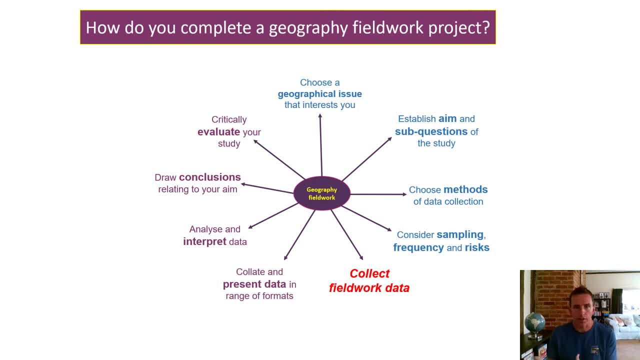 field work am i going to be able to collect with my study? so i'm going to hopefully introduce you to a number of different primary fieldwork methods as part of this video. the other thing that you'll need to do, which is less complex, is that you're going to have to think about how am i going to get? 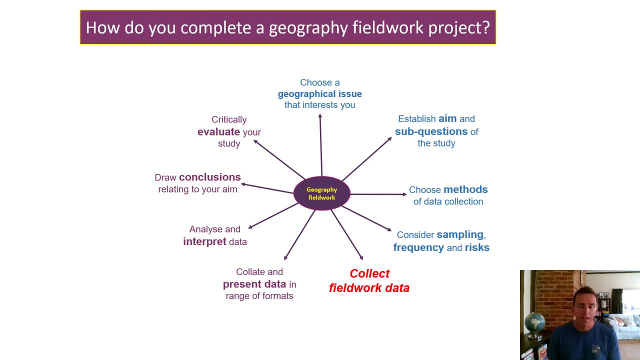 more of a kind of a hoop that you have to jump through really is this bit here where we're considering sampling frequency and risks, and so by sampling, what we mean by that is a kind of twofold really. firstly is, how much of a sample of data are you going to be able to collect? 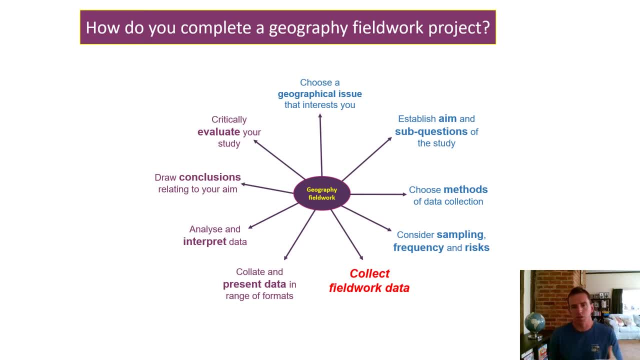 so if you're doing questionnaires- for instance, how many questionnaires are you going to ask if you're doing a pedestrian count on a high street, how many times are you going to do that? how frequently are you going to do that? you're just going to do it once? are you going to do it every? 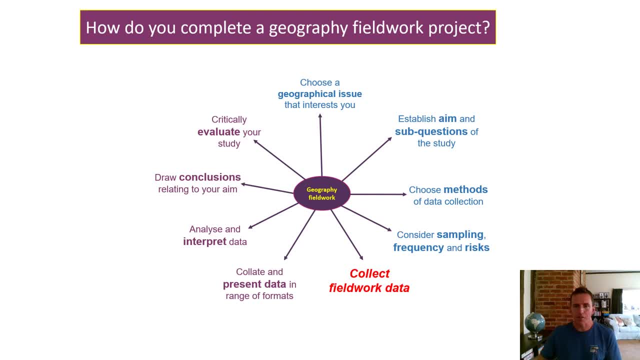 hour on the hour? are you going to do it just in one location? are you going to do it in several locations? so those logistical decisions that you have to take control for, and then, equally, there is an element of planning that needs to be considered about the risks associated with your field work. 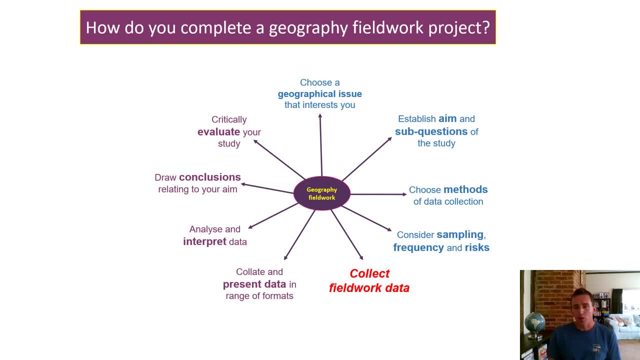 and also questions of ethical um, the ethical impact of your study as well. i will cover that later on in the presentation, so don't worry too much about it. but ultimately, those four bluish statements there are working for you and you're going to have to think about how you're going to. 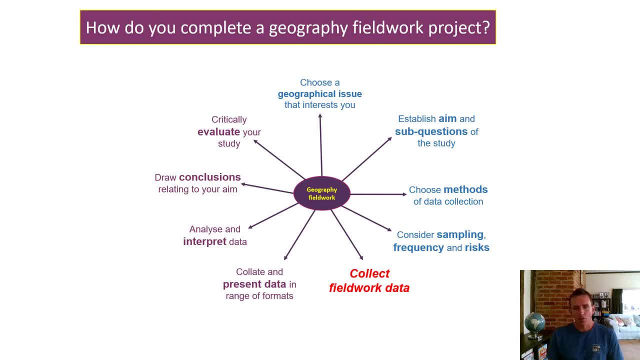 use that data and come up with your own personal data as well. so that's another example of a way of studying the skill set. so that's an example of a way to do that, and the way to do that is by looking towards the red statement in the bottom of that kind of mind map where you have the words. 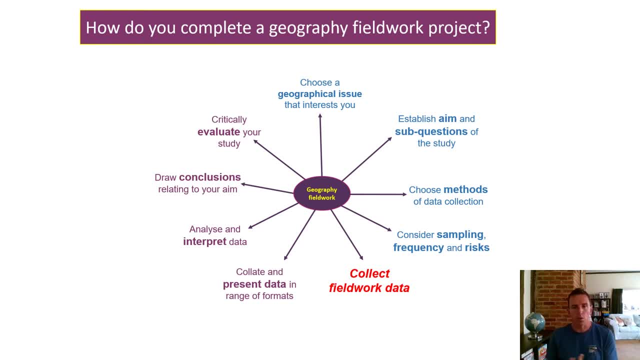 collect field work data. so that is then the fieldwork data you've got when you come to Southwold. if we get time at the end of your fieldwork day when you're in Southwold, i will help you and give you a little bit of guidance about how you can then move forward with your study and how you can. 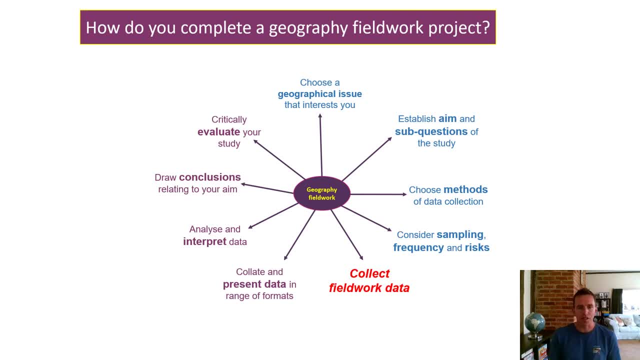 to you. but i can certainly give you some suggestions and show you from good places to help you presenting your data at the end of the day when you're with us. but we want to help you get prepared to get to that red statement so that you're ready to come and collect your. 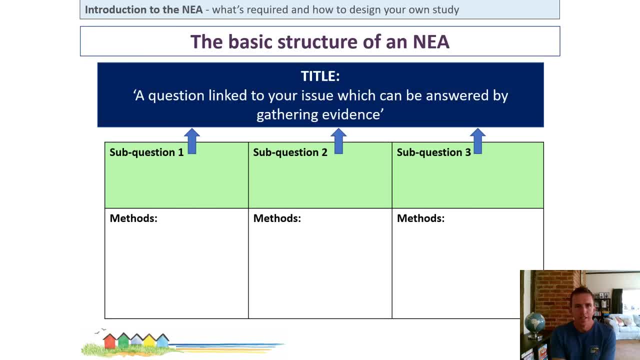 fieldwork data. all right, so we will go first of all onto this image here. um, you may or may not have been introduced to this idea of a proposal form, so one of the things that you'll have to do is ultimately submit a proposal form for your study, and your proposal form will have on it. 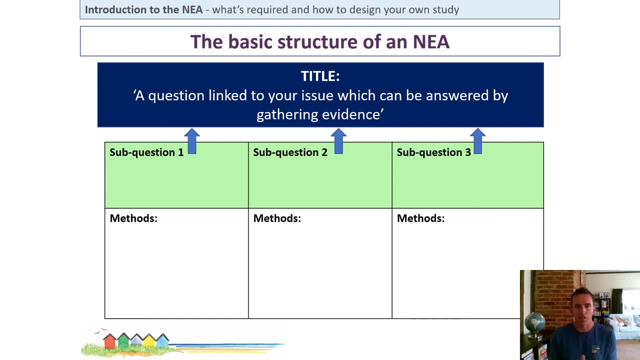 your title, your perhaps supporting sub questions and the methods of data that you're using, how your study links to the curriculum, and it is a document then that is submitted with your final nea report. now that document, i don't think it's particularly user friendly, so we've created 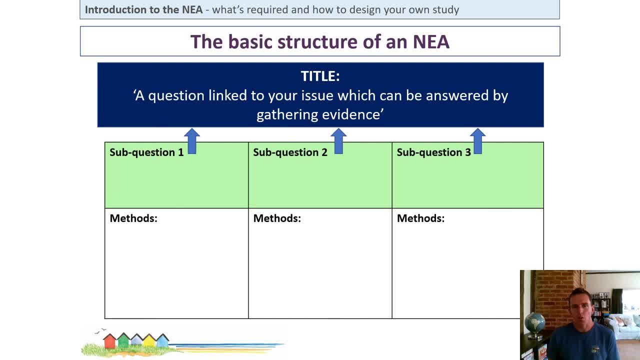 this as a way for you to submit a proposal form for your study, and you can submit a proposal form as more of a user-friendly format for what essentially is the fundamental footings, i suppose, of what you need to have for a geographical study. so get this right. 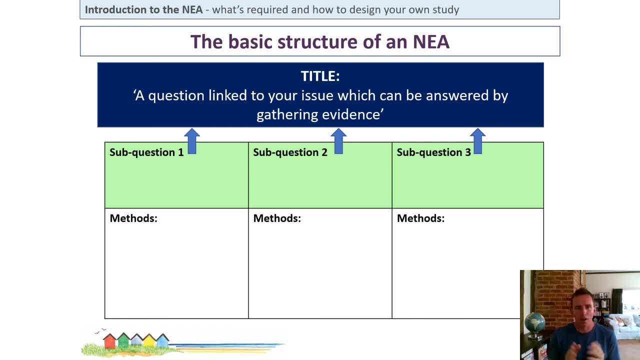 and actually you can have confidence that you are now off, you're away. so over the next couple of weeks, this simplified diagram here, i would suggest, is what you should be trying to work on. first of all, having picked your issue, you are going to need to devise and come up with a title, a title for your 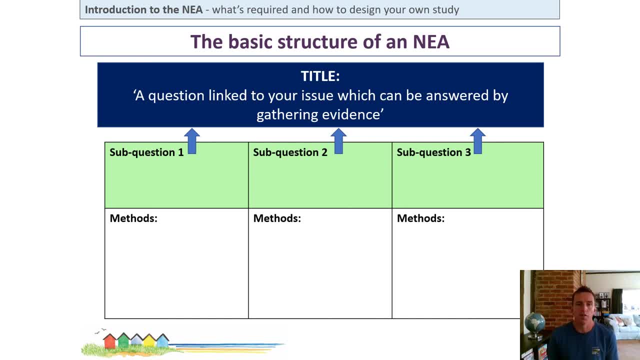 study and generally, i would advise that titles often work best where you are asking a question. say, for instance, to what extent are the hard engineering strategies used on south ball beach effective? that is a question, so a question which is going to be linked to your issue. so if my issue 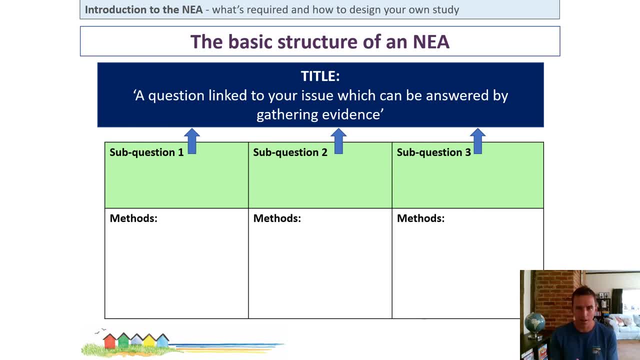 was coastal management, i'd say: right, i'm going to look at hard engineering, so the seawall and the drawings, and i want to ask how effective those different methods are. so that's my title. now, to help me answer my title, what i then do is i divide it up into smaller supporting sub questions. basically now, these sub questions: 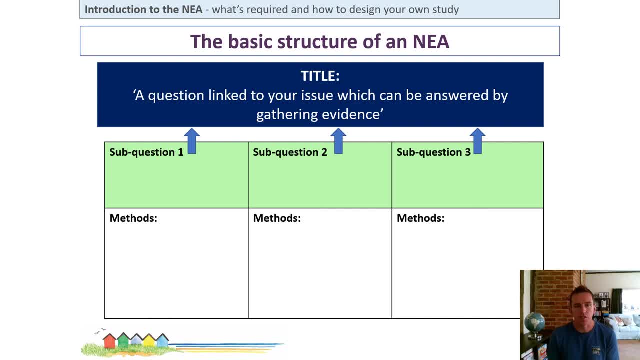 should prop up your title and, crucially, they should be relevant to your title. but what they help you do is to break up your study into smaller, manageable, manageable chunks. so your second challenge, having picked your title, is then to come up with three- normally three- supporting sub. 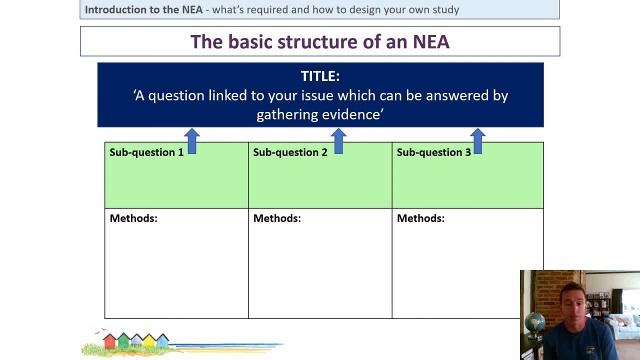 questions. it might well be that you have any two, although you might have four, but i would say that, of the neas i've marked in recent years, vast majority of people tend to pick three. what you then need to do, having got your sub questions, is you need to allocate and think about appropriate 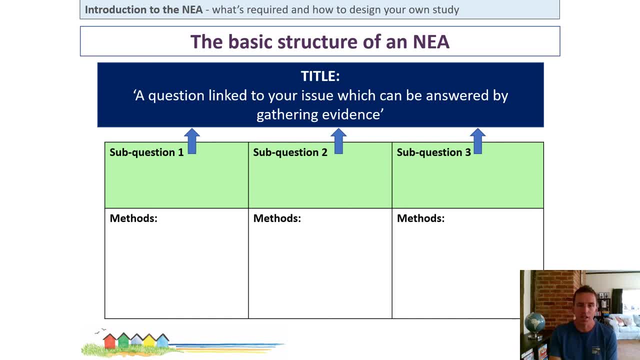 methods of data collection. that will help you answer each of those three sub questions, and In normal years, most people would probably try to aim for between four to perhaps six methods of primary data collection. Now this year across the country there's an acknowledgement, I think, from all exam boards- that that's probably not going to be possible for most people. 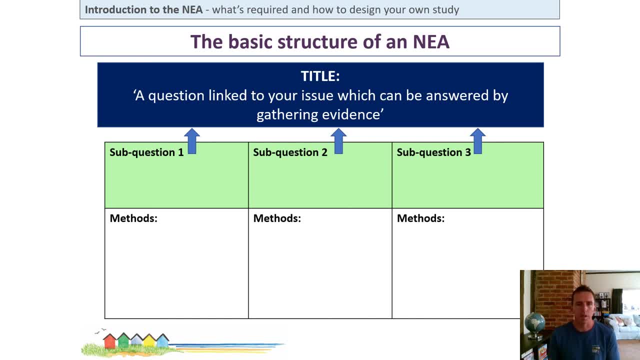 There's going to be significantly less primary fieldwork contributing to people's NEAs this year, And there's going to be more people who are reliant on using secondary data, and that's fine, But what you'll need to do is still make sure, whether it's primary or secondary data, 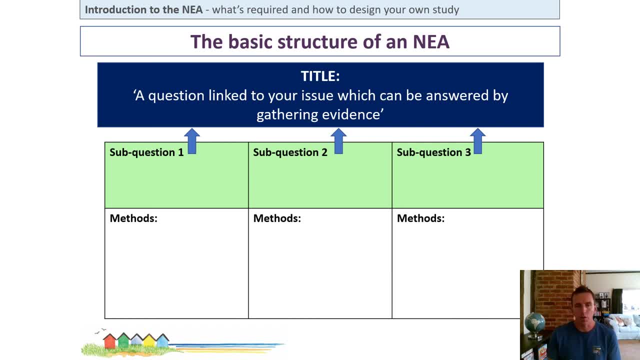 have enough methods of data collection that are going to help you answer each of the sub-questions that you've said. So that, then, is kind of like a holy grail. Get that right. Have conversations with your teachers about this. Maybe you've got lots of scraps of paper where you've got this kind of stuff on it. 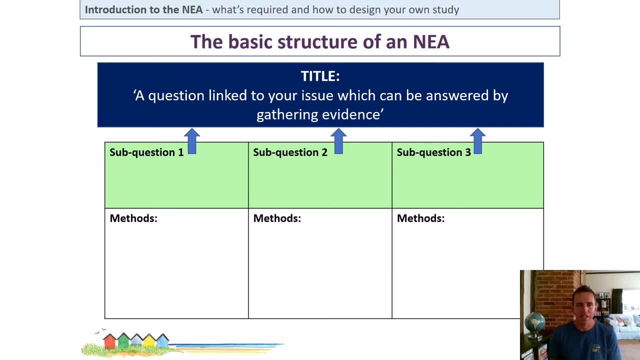 And you're saying: right, there's my question. It's a question from one, two, three. These are my methods. It's that that probably needs to be a bit fluid over the next couple of weeks, where you're kind of. 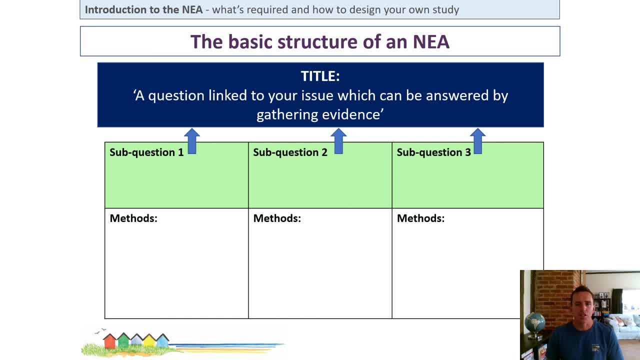 redesigning, rejigging, perhaps rewording some questions and make this bit the foundations of your study work. If you get that signed and sealed from your teacher and they read that and have that justified to them and they say: 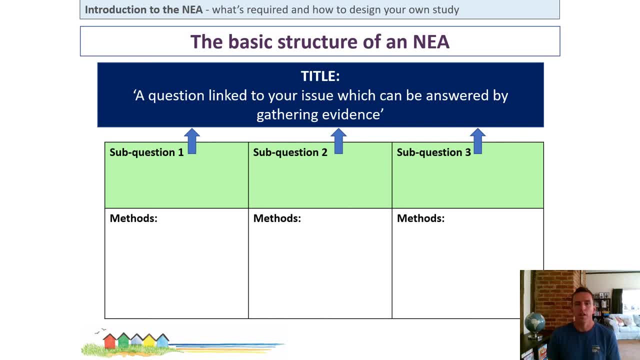 yeah, that sounds like a really good study actually. That sounds really feasible, really appropriate. all linked together then you can feel real confidence that you're getting started on the right foot. Here's an example On the left-hand side. 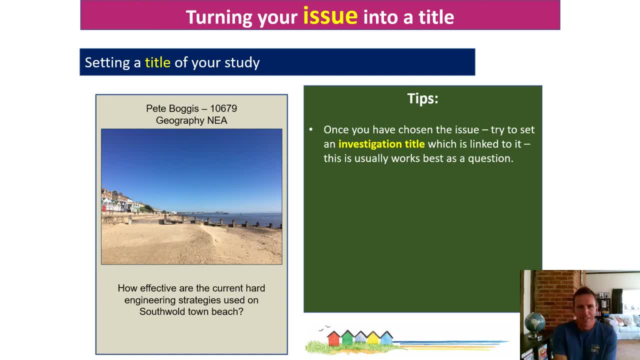 here a chap called Pete Boggis. This is an imaginary student, but similar to what I've just said. actually, he picked the study title: How Effective Are the Current Hard Engineering Strategies Used on South Old Town Beach? Now, the reason that I've used this as a good example of a title is because your title is best. 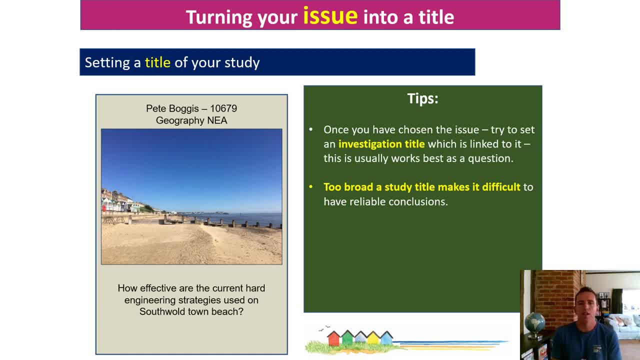 I would suggest if it is more concise, then more broad. So very often people try to come up with a very ambitious, which is obviously not a bad thing in a way, but generally overly ambitious in the scale of what they're aiming to do. 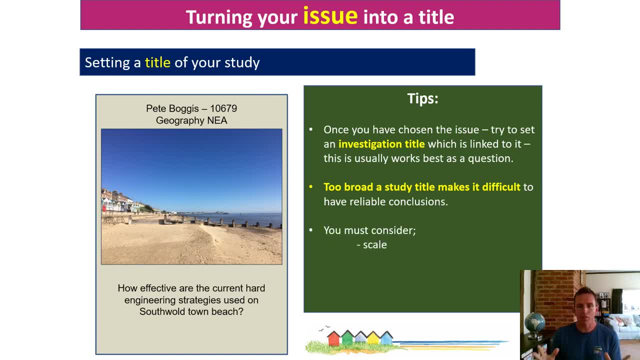 So one of the key things to consider with your study is the scale of what you're aiming to do. Remember that you're going to have one day of data collection. So this person here, Pete Boggis, actually, when he first went to his teacher with his idea of what he was going to do, 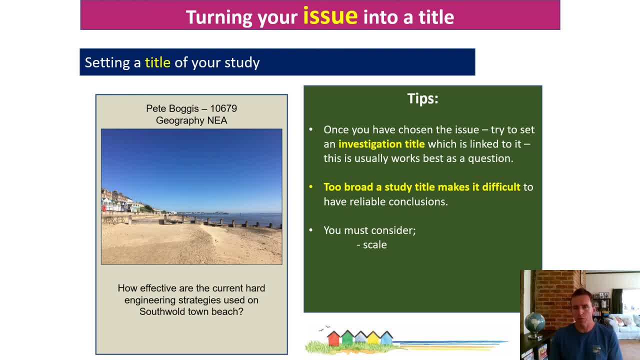 he may have said: I want to look at the effectiveness of coastal management on South Old Beach, and they might say oh. they might say okay, yeah, fair enough, But think about your scale. So, coastal management with a sample. 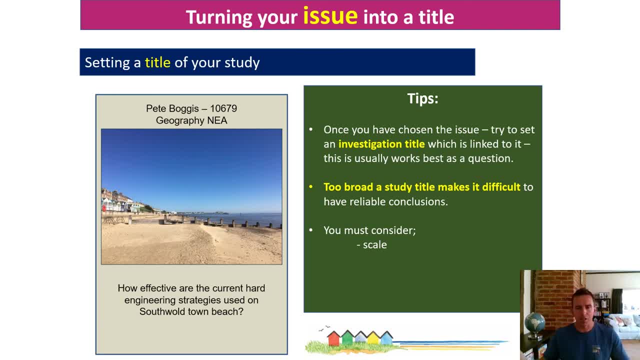 they've got hard and they've got soft engineering. If you do hard engineering, it's mainly just in the area in front of the town. You do soft engineering. You're going to have to go north to Eastern Badlands and look at managed retreat there. 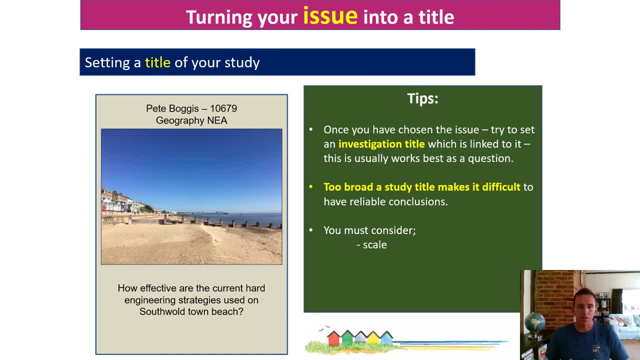 And you're going to have to go south and look at the dunes as well as looking at town, So you're gonna have to cover a wide area. So how about you actually just focus on the hard engineering strategies? You've got drawings and you've got a seawall. 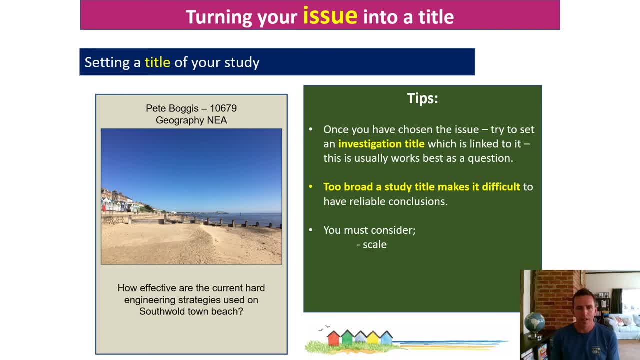 Why not Focus on just those two things? rain it down a little bit. And also then, rather than just saying South Old, why don't you just specifically say South Old Town Beach? We know that's a kilometre long from the pier to the end of the seawall. 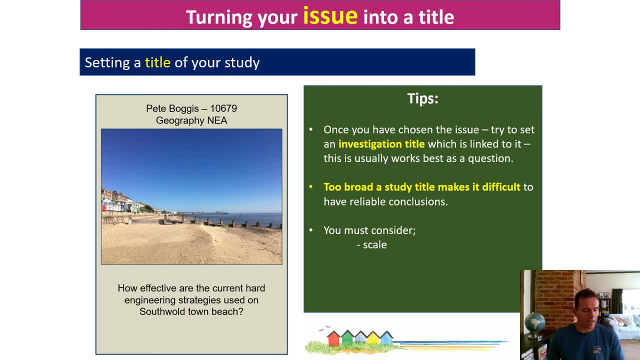 So you could focus your study on the hard engineering strategies one kilometre distance. That would make the scale of your study much more feasible, And it would also mean that you're able to repeat some of your data collection, which makes your data more reliable and your results. 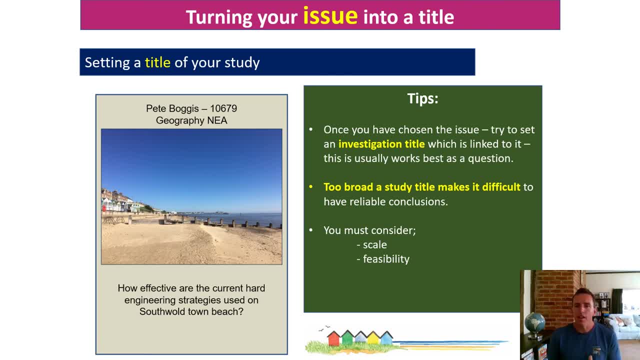 more accurate, So that student then has probably refined their initial idea to make their title much better And ultimately then their study will be more effective. So think about this. obviously initially come out of your plan, but then don't be afraid to be flexible in terms of refining the scale of what you're intending to do. 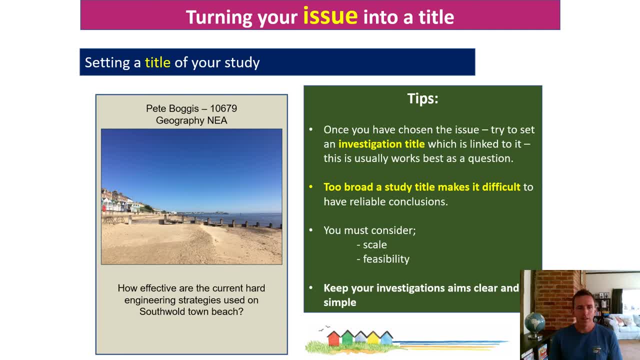 This one, I think it's probably worth saying. actually, your title can sometimes get lost in a bit of a fog when you're writing something that is fairly open ended. you know something that might be four or five, maybe 6,000 words long. where you're writing an extended piece of work like this, 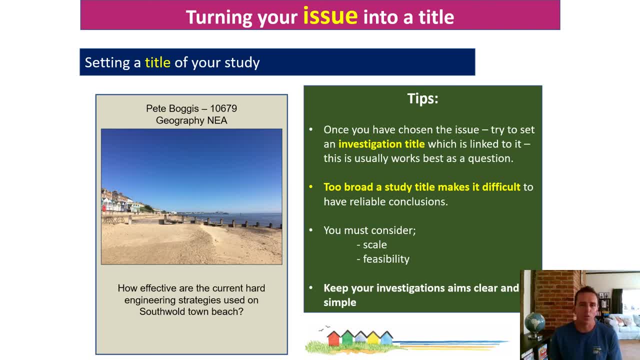 You can fall victim to waffle, and waffle in an NEA is not going to be great. It's not going to contribute very well to you creating a good mark at the end of this. So what you want to be making sure that you're doing. 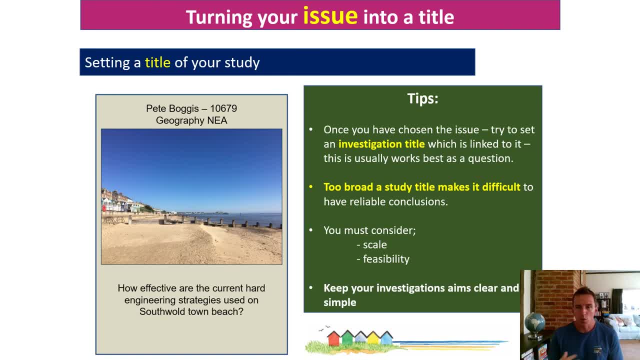 throughout your study is things that are relevant and talking about things that are relevant, and always relevant, to the questions or sub questions that you've set. So where you have a clear investigation title, like the one here for Pete Boggess, it's much more likely that the things that you write are going to be relevant to your title. 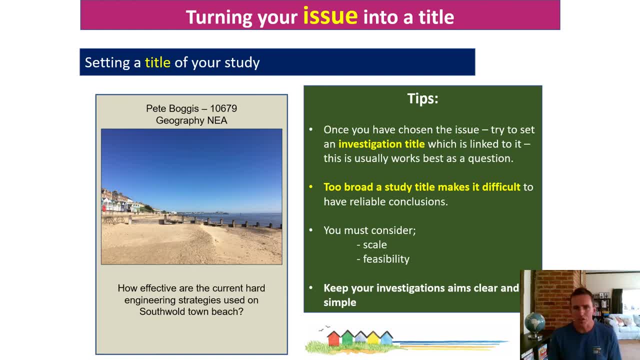 You're going to cut out that element of risk, including lots of waffle and talking about stuff which actually isn't relevant to your study and isn't therefore going to be scoring you any marks. So I would try to keep your investigation title clear. 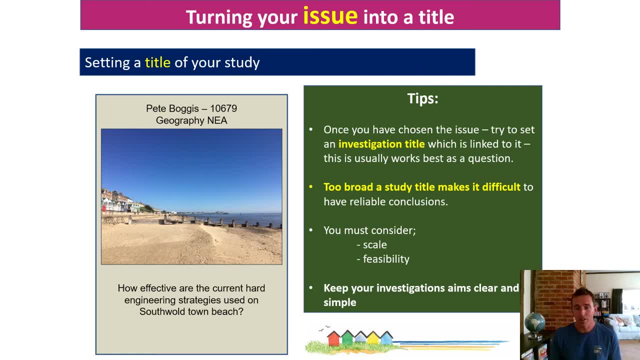 So all the time in your head, you know what it is you're trying to do and try and keep it simple. Okay, It doesn't mean that that is going to be a simple study. It just means that it's going to probably be an organized one, and one that is going to be relevant. 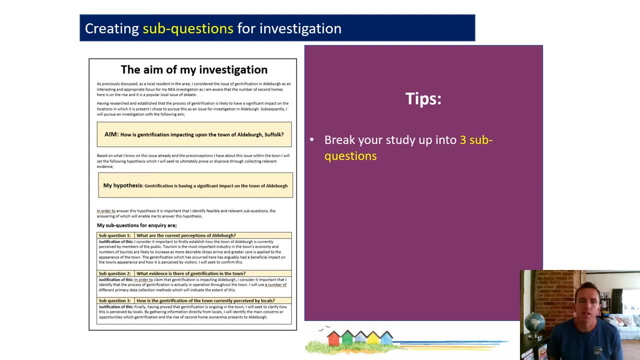 Okay, So for this, we've kind of covered this a little bit already in terms of structure of your study, but we would normally suggest that, having got your title, you then have these three supporting sub questions. I've already mentioned that These sub questions need to be relevant to your aim, and they should be relevant enough to your aim that you're able to kind of justify how each of these subheadings contribute to your title. 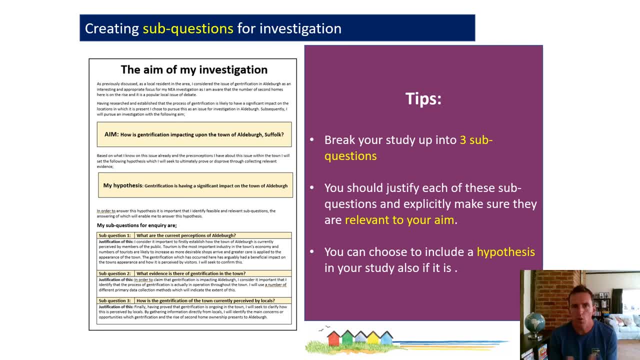 Now the third issue here is about hypothesis. There's nowhere anywhere on any of the NEA guidelines from any of the exam boards that your studies have to include a hypothesis. but hypotheses sometimes are useful to include because they give you a kind of a logical reference point to refer back to at the end of your study. 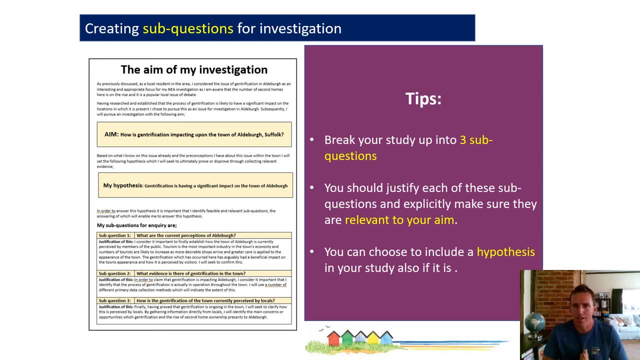 To ultimately say yes, I was in my prediction, because a hypothesis is essentially a prediction which you can base on your prior knowledge. So this person here is doing a study looking at the impact of gentrification in Albra and their prediction is that gentrification is having a significant impact on the town. might be again. 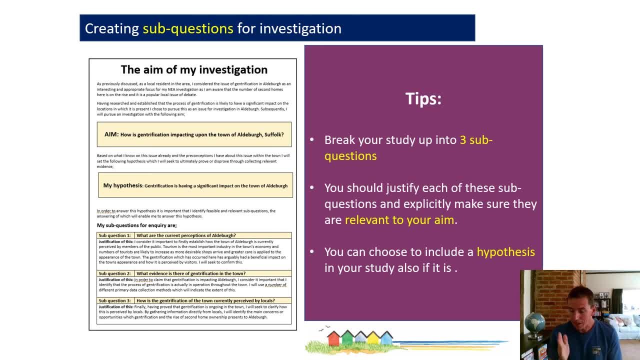 if you're doing the coastal management study that you're saying that you know um, hard engineering is having a significant impact on coastal morphology on South Oldstown beach. A hypothesis, then, gives you a logical thing to return to in your conclusion, where you're able to say: 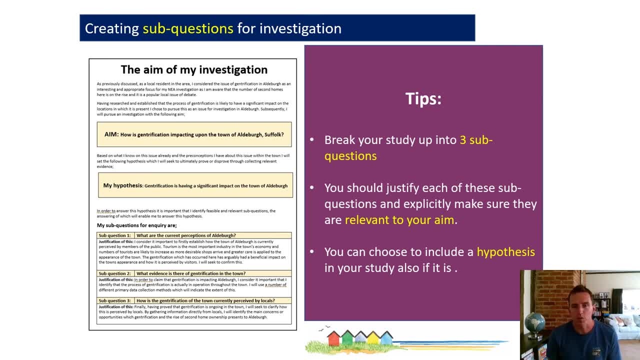 okay, at the start of my study, this is what I've said, and I'm now able to categorically prove this because my results backed up my assumptions that I made prior to my investigation. So it's not a bad thing to include. 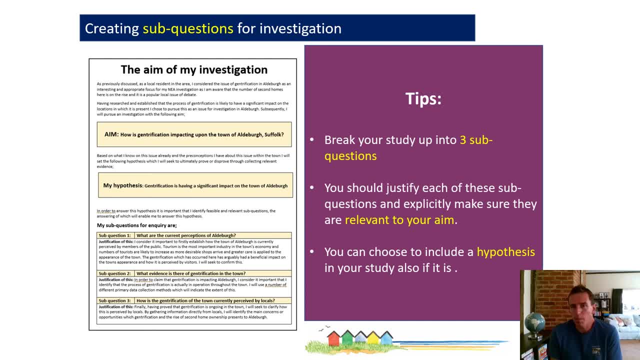 but I would say again, not everyone does and probably it's about 50: 50 split. Some people have studies that are more kind of geared towards having a hypothesis, Others perhaps a less naturally um needing one. So it's up to you. 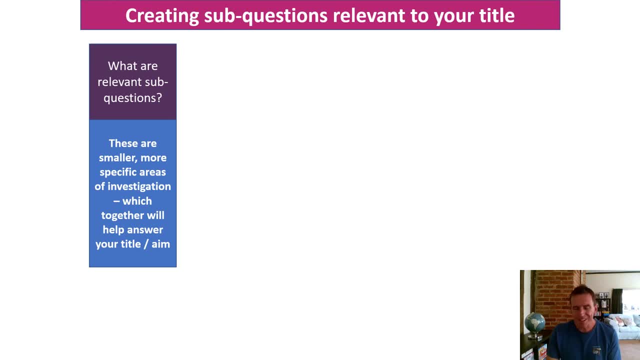 All right, So I'm just going to dwell a bit, actually, on the idea of sub questions. So this is an example of why sub questions are relevant and how you can perhaps use them. So we are recently working at a high school called Bungie high school. 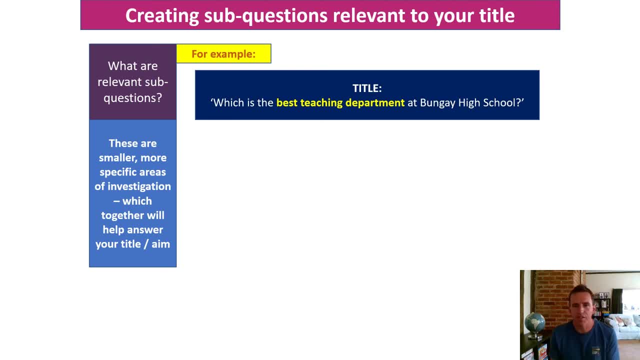 And one of the things that we said to them was right. Imagine if you were in your classroom at the moment and then the head teacher came to the door, have a little quiet word. and they pulled you into the corridor and I said: 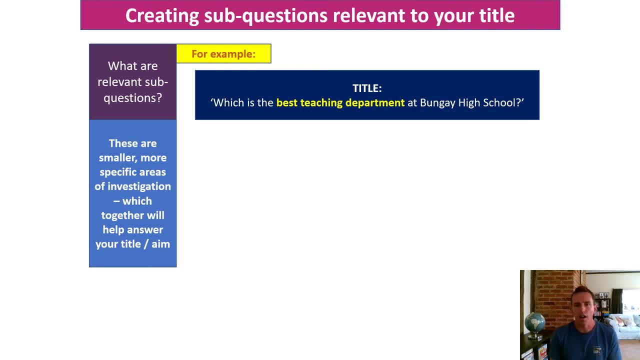 right, I've got a favor to ask. Um, I've heard you're good at writing. I want you to write me, from a student perspective, a 4,000 word report on which is the best teaching department in the school, You might say. 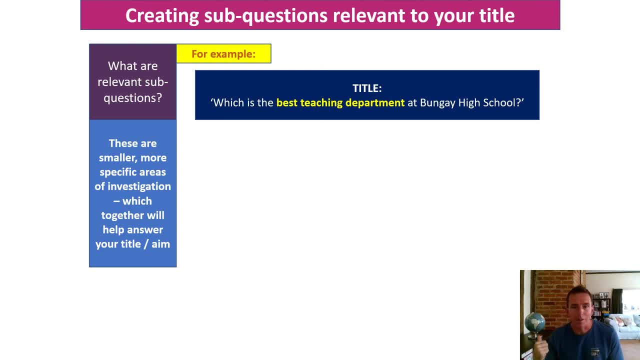 I'm actually very busy. Um, I'm trying to plan my job for the NEA, But a teacher is quite insistent and they say: well, you know, forget about that for a second. I need you to do this for me. 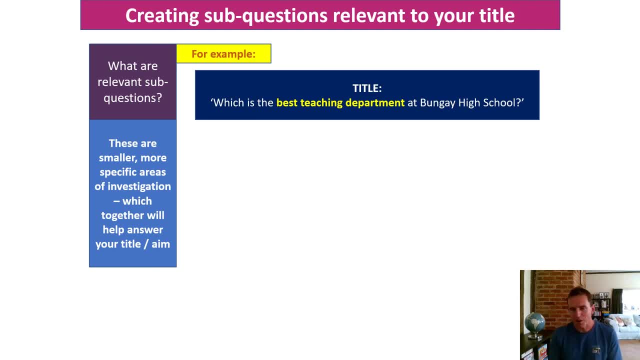 And you write this 4,000 word report on the best teaching department in the school. So, reluctantly, you agree and you say, okay, well, how am I going to do this? So you could probably tease out 4,000 worded waffled essay answer to that question and just write it as a big essay. 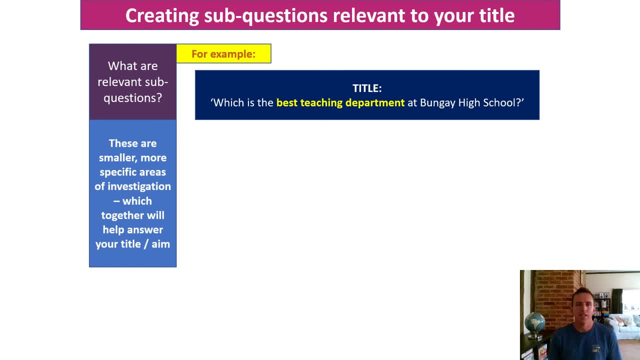 but it wouldn't necessarily be all that engaging or that inspiring, And you know that's interesting to read. So this is where a geography report is different for history or an English essay. You've got to think of this as a report, as a modern report, and not just as a big chunk of tech. 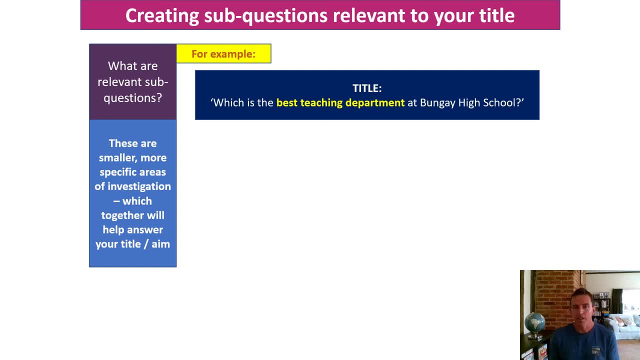 So geography NEA has got the potential to be really engaging and to be really kind of different in terms of the way it's structured. So to answer that question, then it would actually probably be a better idea to break it up into smaller, more manageable chunks. 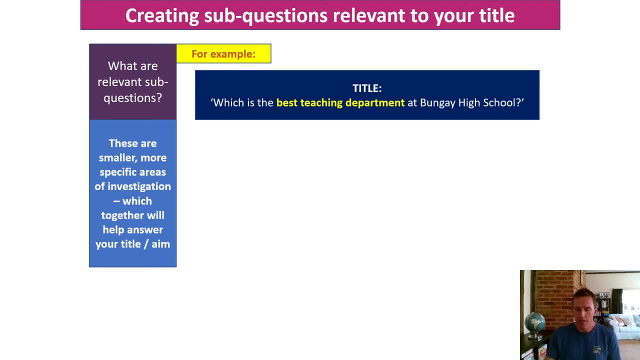 Give it a better structure as a finished piece of work. So the student then decides: okay, well, fair enough, we better do this. What I'm going to do to start off with is I'm going to have a first question, which is actually going to focus on what is here in this school. 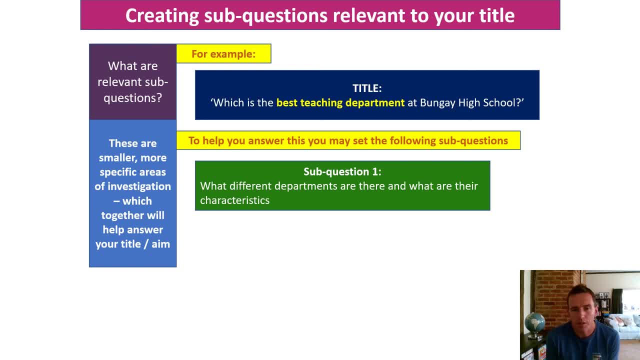 because actually, as a reader and you don't know this school, first thing that you might want to do is say, okay, well, what are the different departments that we've got and what are the characteristics? So what subjects do we offer? How many teachers are in each of those? 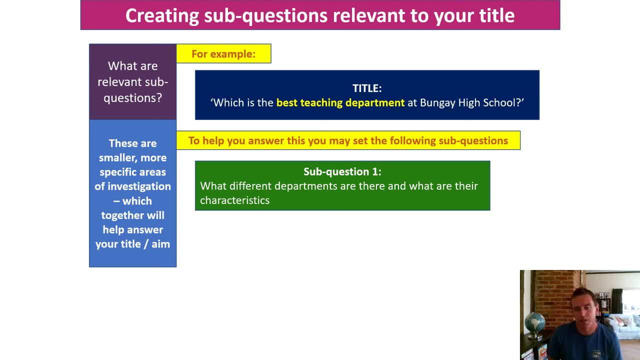 How many students actually opt for those subjects Which are the most popular in terms of student number. So you could have the characteristics, then, of the teaching departments. That's going to be relevant to this title. The title is: which are the best teaching departments? 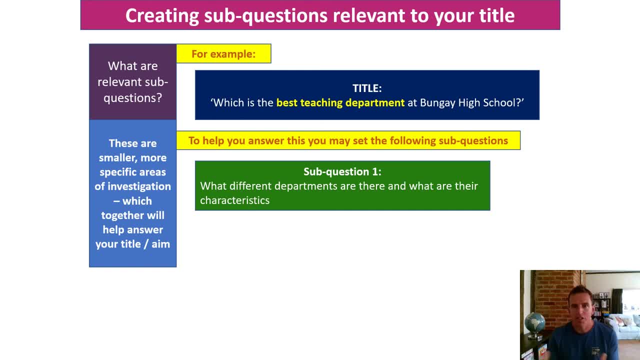 It makes sense, then, that the first question is actually saying: well, since we need to tell you what is the best teaching department, we're going to say, first of all, what teaching departments we've got and what the characteristics are. So, realistically, 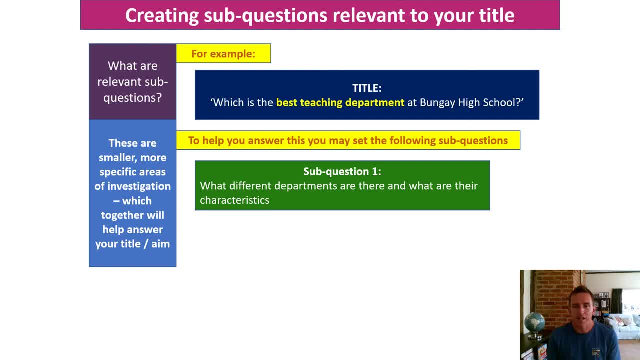 you could actually swap that title, for you know which is the most effective form of hard engineering on South ball beach. sub question One could be well, what hard engineering is on South ball beach and what are their characteristics? And you may do a. 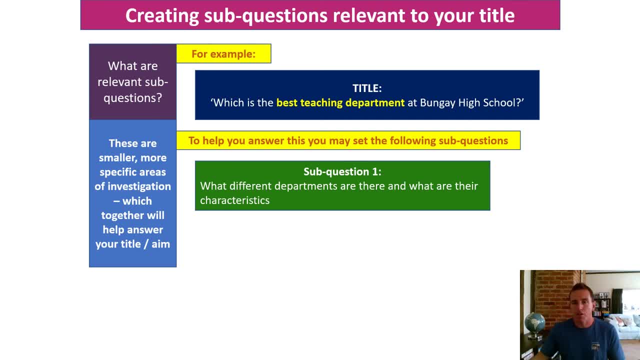 an annotated series of photographs. You may do a bipolar survey to actually show the current characteristics of coastal management. The second sub question is student has decided that they're going to use is how do the exam results of different departments compare? So they're actually going to do some quality quantitative. 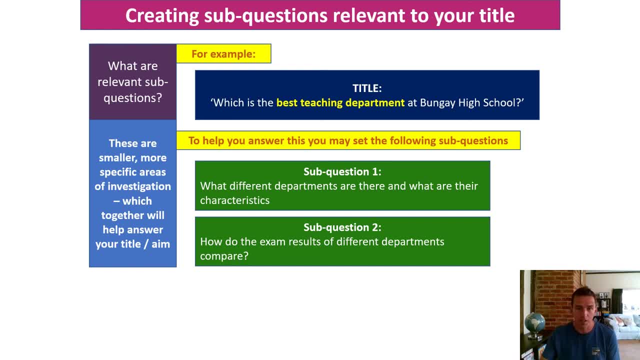 data crunching here and they're going to look historically at how these departments performed and what results they get at GCSE at a level perhaps. how many of these students go on to study a level in their subjects? how many of them perhaps might go into university to do it? 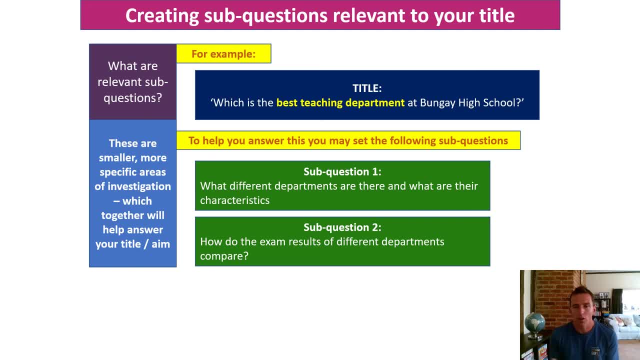 but historically looking at the data as well. So they would get a lot of quantifiable information from that, And again that's going to be relevant to the question. questions asking is: which is the best teaching department? So inevitably then we would have to consider this success. 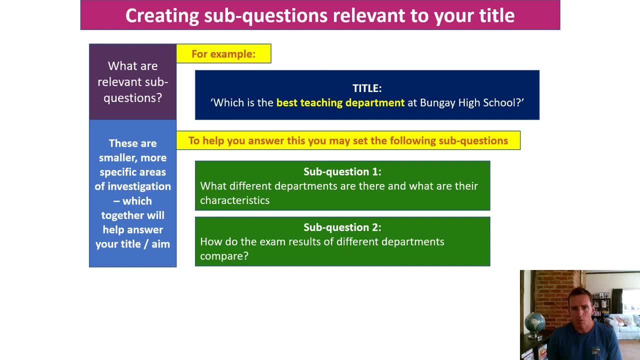 In terms of those departments and regarding exam results, So that sub question two is clearly linked to the title sub question three. Then we're going to try and get a little bit more qualitative data. So qualitative input into this study would include considering people's opinions and their thoughts and attitudes towards these departments. 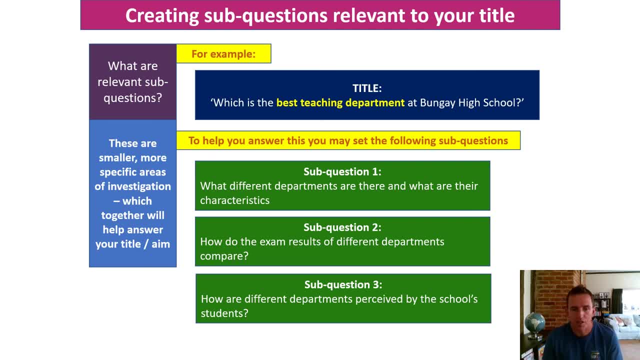 So some question three here says: how are different departments perceived by the school students? So could be, you know, a student survey where you actually ask people what they think. rather than physically, or rather than actually analysing the data, you actually are asking for people's opinions. 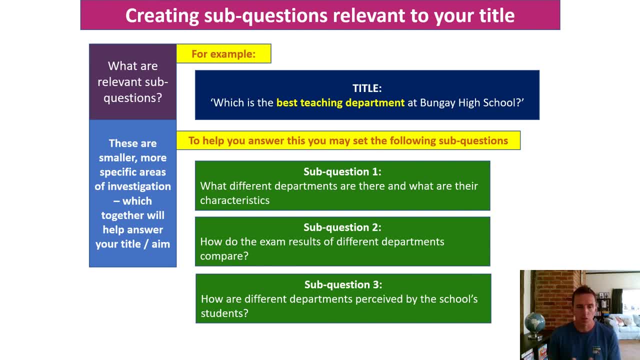 perceptions and thoughts about the school's teachers and their departments. So what this study ultimately has is a mixture between primary and secondary data, quantitative and qualitative data, but collectively, all of that data is relevant to the sub questions that are being asked and all of the sub questions is relevant or relevant to the title that's being asked. 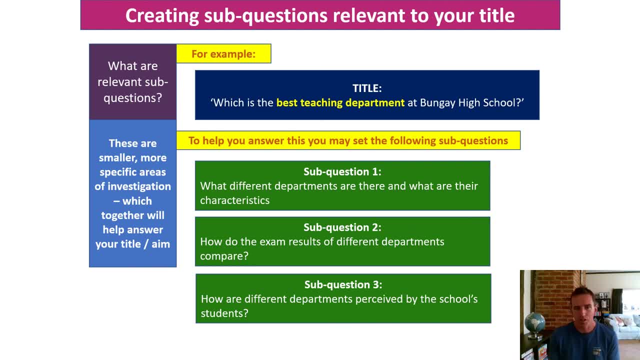 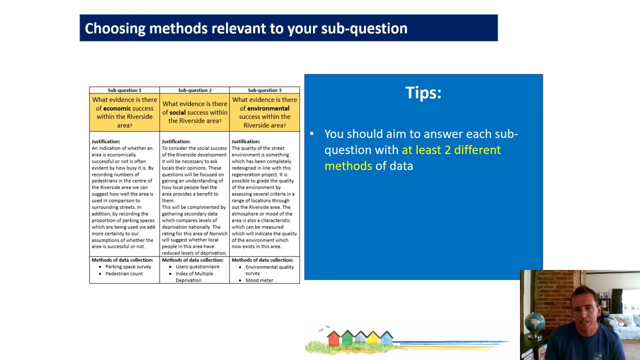 So that all ties in together and that's how the sub questions can be useful. So, in terms of your tips, I would suggest that you would have two different methods of data collection, whether it's primary or secondary, for each of your sub questions, and a mixture of quantitative and qualitative. 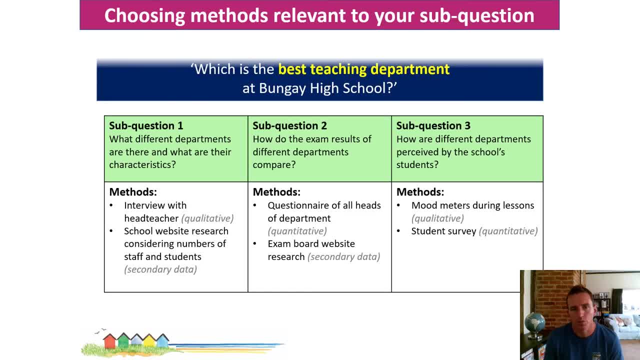 So if we could go back to our title here, that we looked at this person then, like we just kind of reviewed, has got their sub questions there and underneath each of them has added in the forms of data collection that they're going to use to help them answer those sub questions. 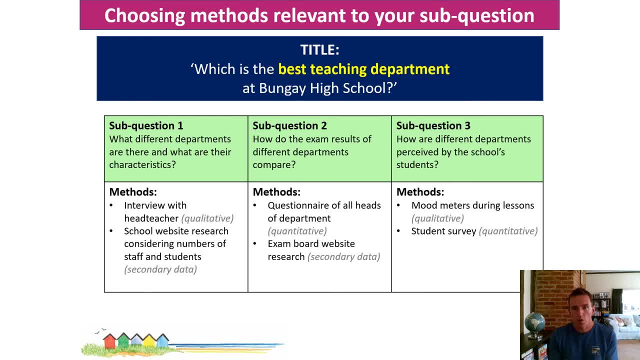 And if they were planning this, then imagine it was an NEA. they could then go to their teacher at this point and say: right, I think I've got my title pretty happy with my sub questions. I'm thinking that I'm going to use these methods to answer that sub question. 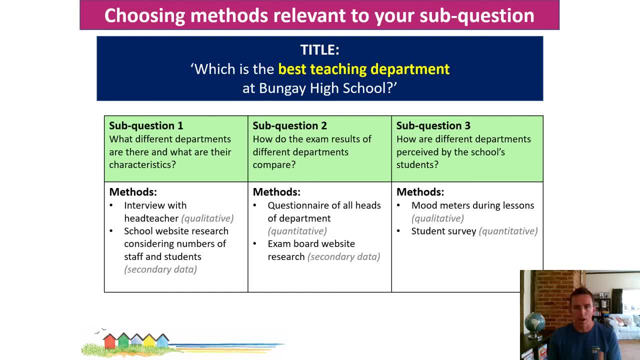 these methods for that one and these methods for that one, and they're going to be relevant because of this, this and that. If you get to that stage, then over the next couple of weeks, that, hopefully, is what you're going to be working on with this structure like that. 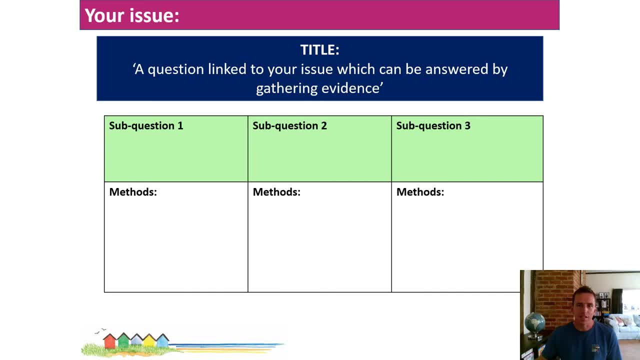 Then, as I say, you can feel confident that you're really getting started on an NEA which is going to work, which is going to be feasible, is going to be appropriate, It will be, it's going to be, it's going to be. 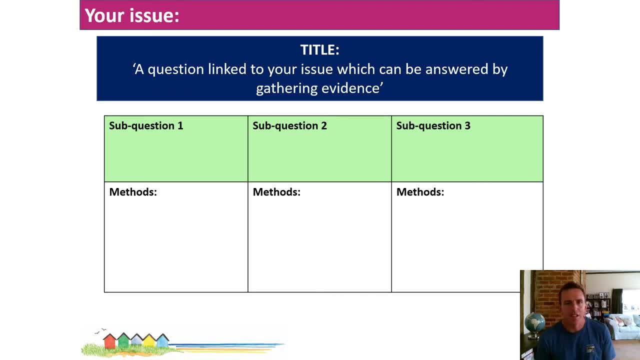 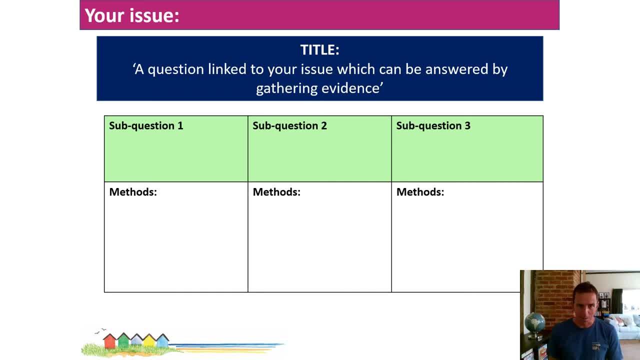 All right, Hopefully that not bamboozled you too much And hopefully that makes it clear as to the work that you need to do, So you might think, okay, well, cool, Fair enough, I know about structure, then that you're advising. 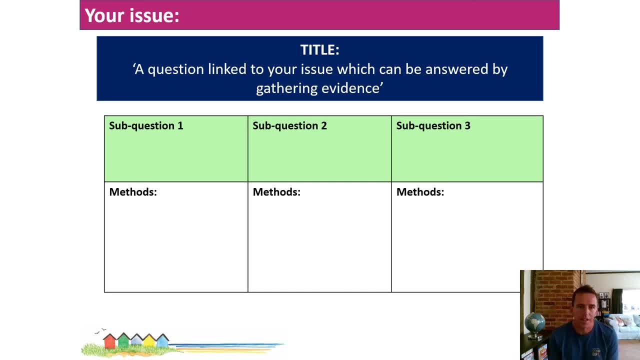 actually, what question am I going to ask, Which is fair enough, And at this point the questions that you could ask are probably going to be fairly limited, because I haven't yet interviewed the geographical potential of Southwold. So that now is the next thing that we're going to come through. 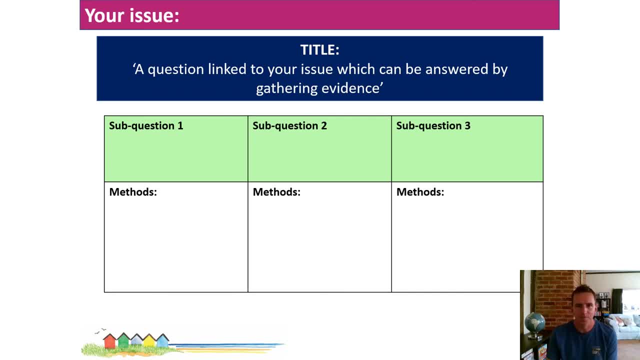 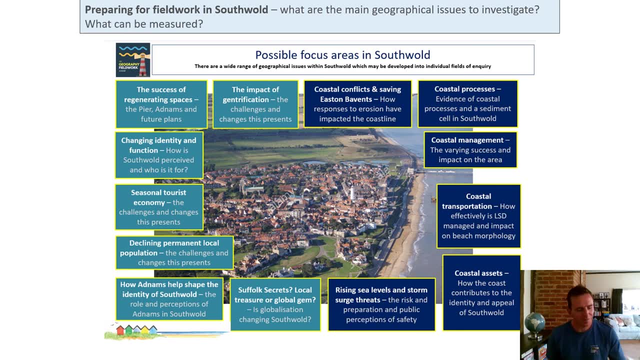 Hopefully it's the world. So back to this then again. this is in your booklet And, as I said, your challenge initially is to pick the issue that you think is going to work. You would like to investigate in Southwold And at this stage 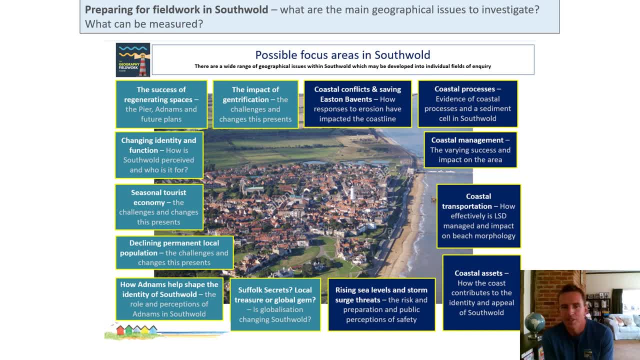 you may think I'm going to do that. I'm going to do on Adams, I love breweries And that is the thing that I am definitely going to do my NDA on. or you might think I love longshore drift. It's brilliant. 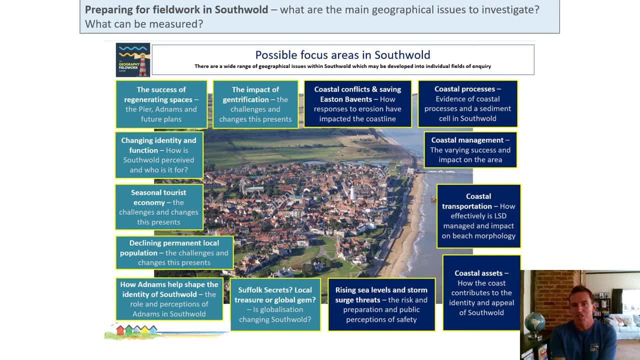 I'm going to do my study on coastal processes. I would suggest, over the next few minutes or so, have a bit of an open mind, listen to the different issues that are discussed And ultimately, when you've heard about everything, then make your decision. 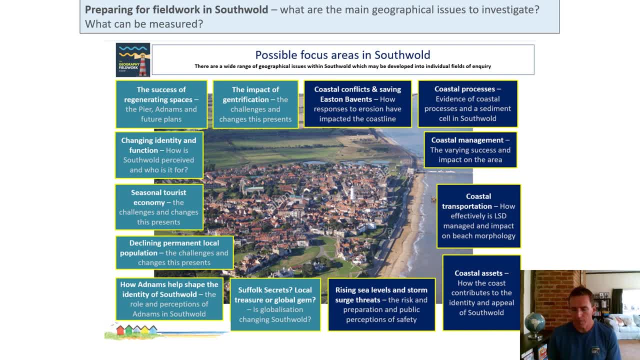 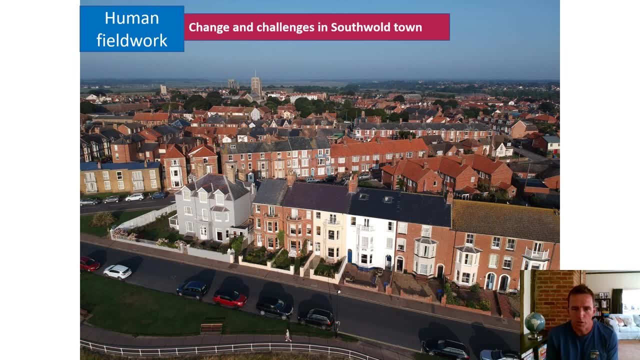 And when you've got more information in your head. firstly, then, what I'm going to do is highlight the geographical potential from a human perspective. It's a nice view taken by a drone hovering over the beach, looking inland towards South wards um. 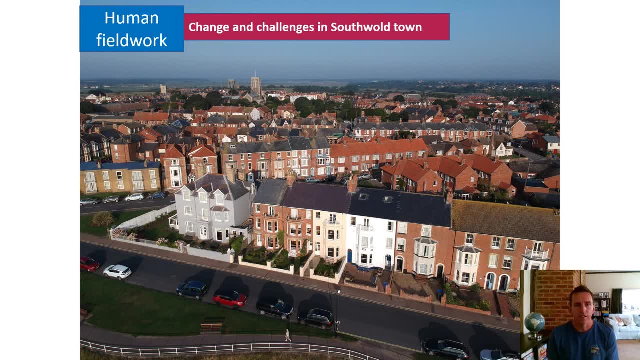 high street and you can see the church there and uh looking beyond into uh, the west as as kind of the uh, the, the pick it hands away Into the distance. You can see from um this image already, that South wards houses. 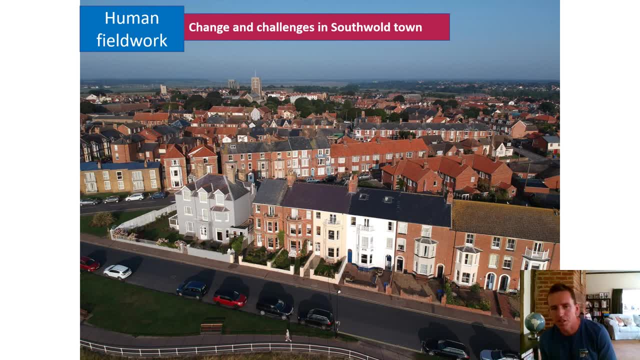 you know, pretty nice. I mean, those are seafront houses so those are going to be some of the most in demand. but you get the idea very quickly when you arrive into town as you walk along the streets that you know. 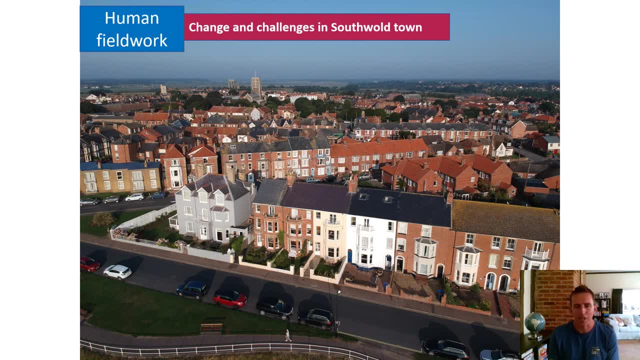 the houses here are nice, Um. there's lots of money that has been invested in them, Lots of care, lots of attention applied to them, or renovations that have made them look like they've ever looked before, Bigger than they've ever looked before. 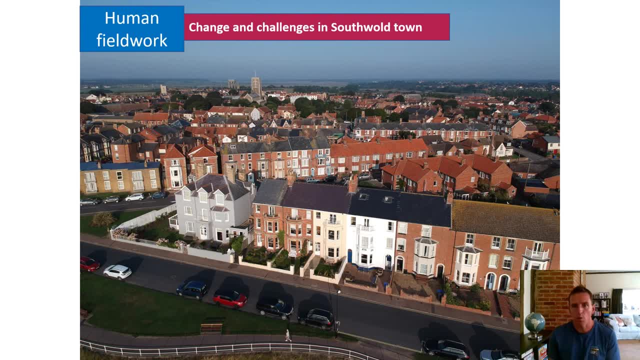 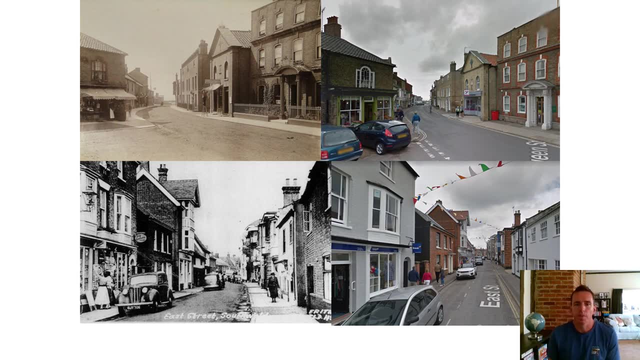 And you know you very quickly have this feeling of affluence and wealth as you're walking around the town. It's a place, then, that people come to as day trippers and holiday makers because, as I've said before, South wards has this nostalgic feeling of classic British coastal holidays and the seafront. 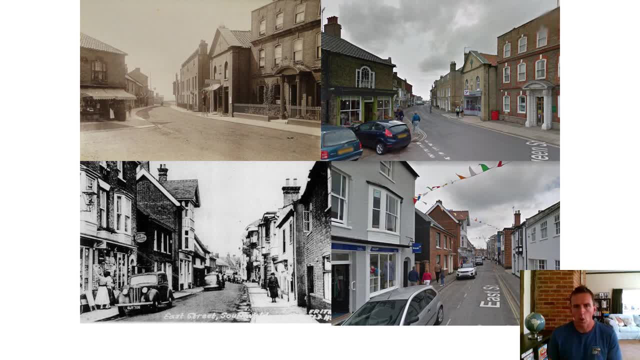 the high street, the lighthouse, the pier, all adds to this kind of- um you know, nostalgic British holiday vibe that South board does quite a lot to promote and preserve. And physically, there are a number of people that we've been coming to South for decades now, for years and years on returning family holidays. 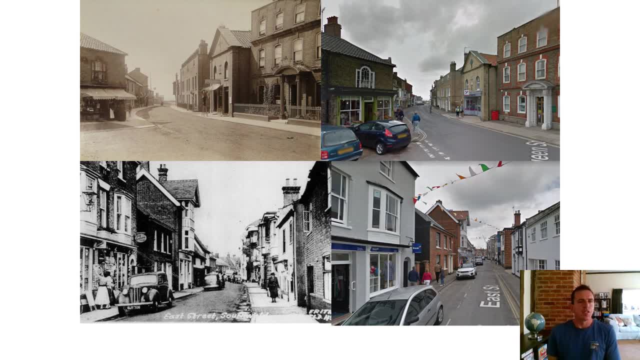 And physically, they will probably say to you that you know South holds great because it's a place that's very timeless and it hasn't changed at all. And when you look at the buildings, physically the buildings in most places haven't changed. 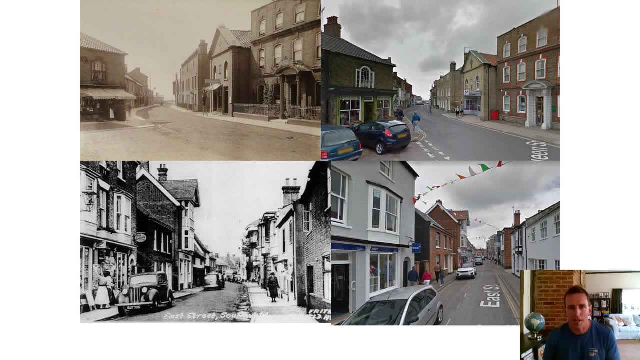 An awful lot And the streets. I've got the same architecture and the same layouts and the same look to them as they probably would have done 40,, 50,, 60,, 70 years ago, And that is one of the appeals of South ball. 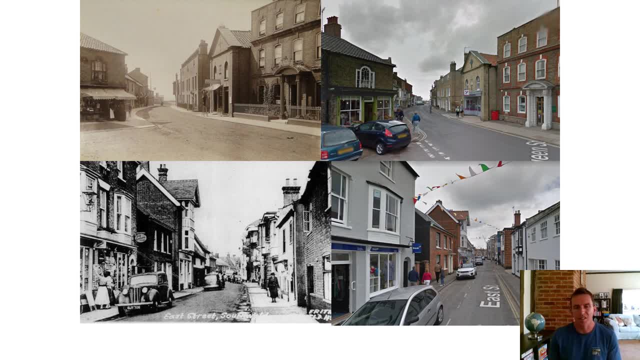 So you might think: well, this is a strange place then, to be looking at it's idea of change. Change is one of these big themes currently in human job changing places, because South boards landscape, from a human point of view, hasn't changed. 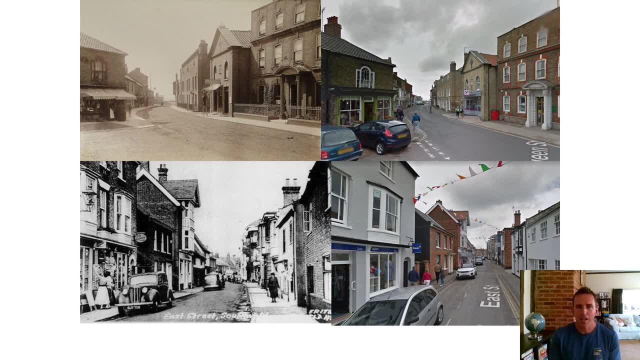 It's here. It hasn't really changed, but the change in South board is definitely real but is definitely discreet- Well, so discreet that most people would miss it in a window. here a little clue to the change which is happening in South ball. 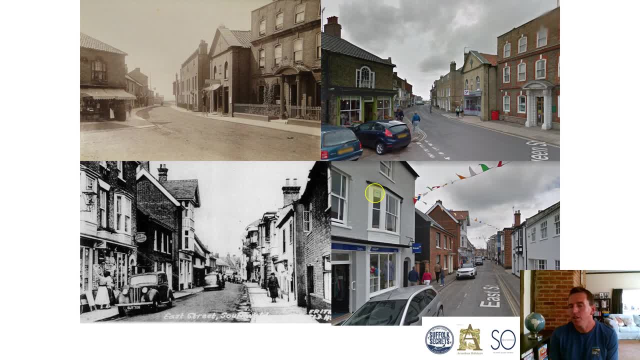 These little logos that have, over the last 10 to 15 years, been popping up in most residential houses windows or on the doors of a lot of the buildings, These residential properties, these things are the logos for the towns letting agents, and the letting agents are responsible for looking after property that are available to rent to holiday holiday makers. 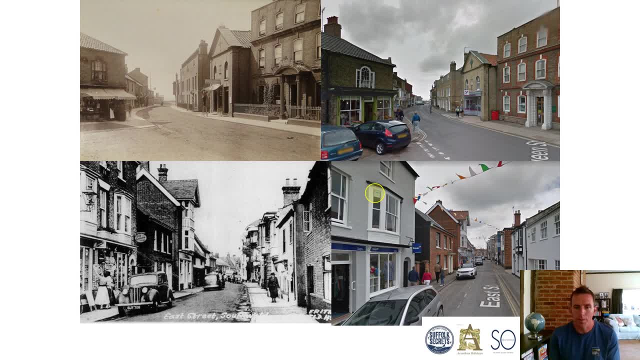 These properties are normally owned them by second homeowners who bought them up. It may stay in them for a few weeks a year, but for the remaining time rent them out as holiday rentals And, as I mentioned previously, South board as far as I'm concerned. 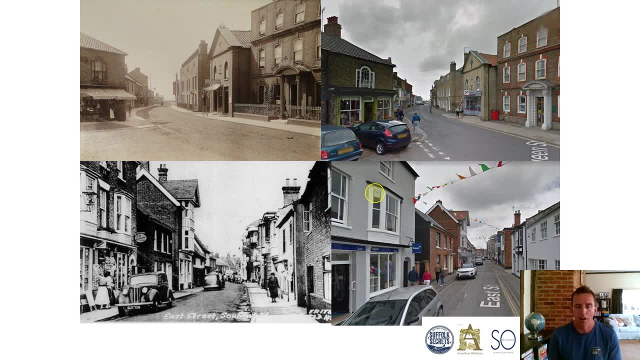 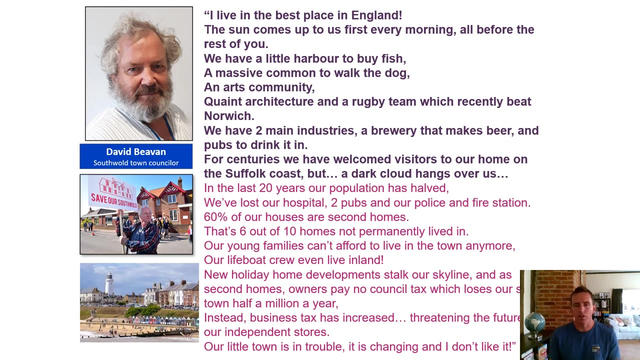 I'm aware in a country is probably a town, which currently is most affected by rising second home ownership in 2011.. I might skip to the next slide. 2011, South board had a census, where the whole country had a census, And at that point it was noted that 60% of houses in South board was second homes or holiday rentals, houses that were not lived in local people. 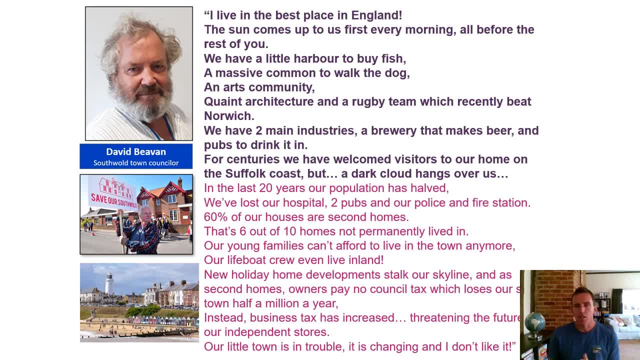 So it is a major issue And it's an issue that has prompted lots of national attention, but it's also prompted, you know, response from local residents and the local council. So this chap here, a chap called David Bevan, represents South board. 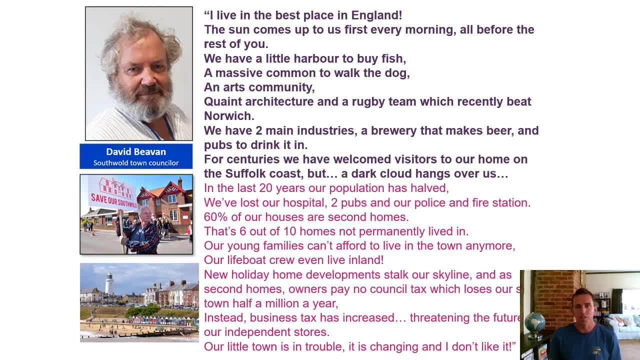 you know, in the in the local area, but also occasionally goes to Westminster and speak to Arbor hearth as well about the issues in the town, And he did this a couple of years ago, And this bit of text here on the screen is an extract. 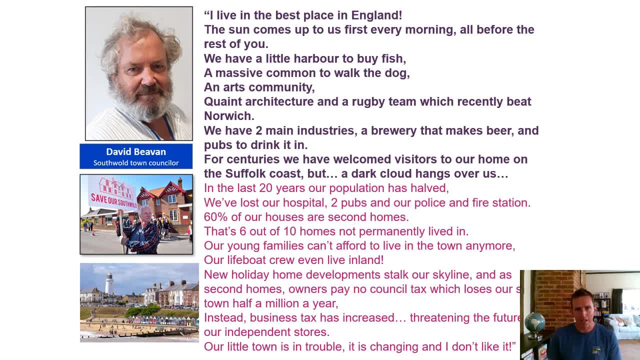 a text. a text here on the screen is an extract. a text here on the screen is an extract. a text here on the screen is an extract, an extract from one of the speeches that he gave at Westminster about his life in South board. 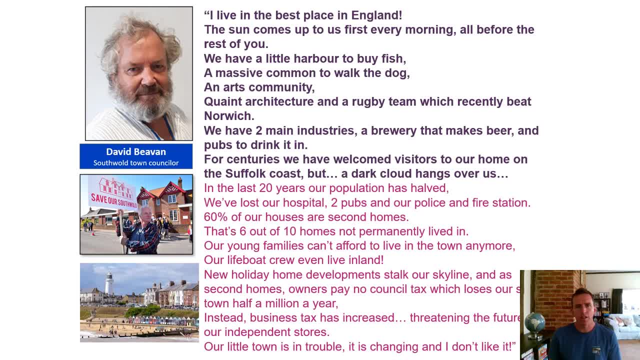 And the first part of it, the purple part, is generally fairly positive, talking about why he loves South board and why it's a great place to live with lots of space, place to buy fish, You can go to watch the arts in the theater and you know. 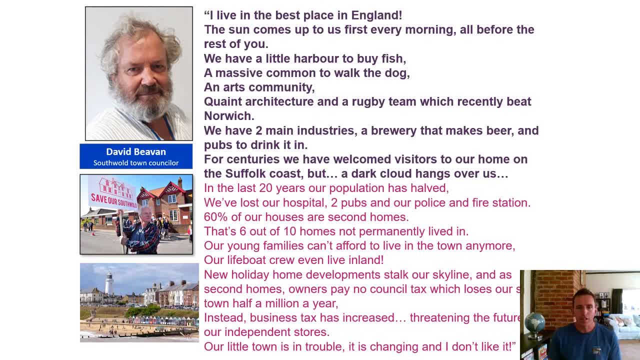 he's a keen sportsman. He goes and watches the rugby and the cricket team And we've also got, you know, this beer that makes this brewery. It makes wonderful beer And you know there are wonderful kind of old school. 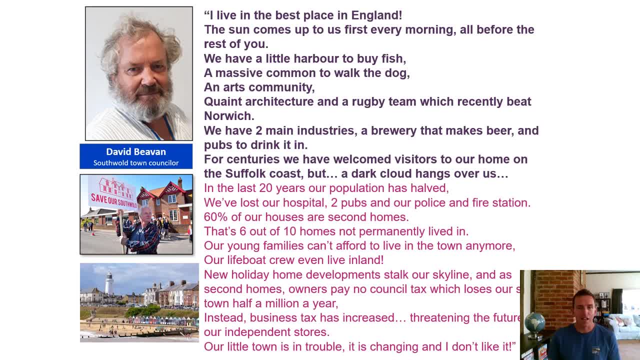 old time pubs in South board and lots of nice cafes and things like that. But he goes on to say: for centuries we've welcomed visitors to our home, but a dark cloud hangs over us And the second part of this speech here was more about the negative change that has occurred in the town board in recent years. 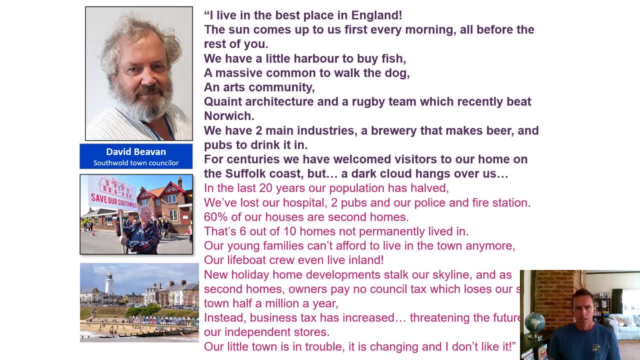 Does in the last 20 years, our population is half. We've lost our hospital, two pubs, our police and fire station. The library in town is also in the threat, for the primary school is also in a threat. that ice high school has closed. 60% of our houses are second homes. that's based on 2011 data. six out of 10 homes not permanently lived in. even the lifeboat crew of South board can't afford to live in town anymore, because the issue is that when a property comes up for sale in South board, it is normally in such high demand, The house prices are inflated Massively. local people can't afford to buy the property generally bought up by people that can afford to pay over the odds, and they then use it occasionally, but generally rent it out as a holiday rental. 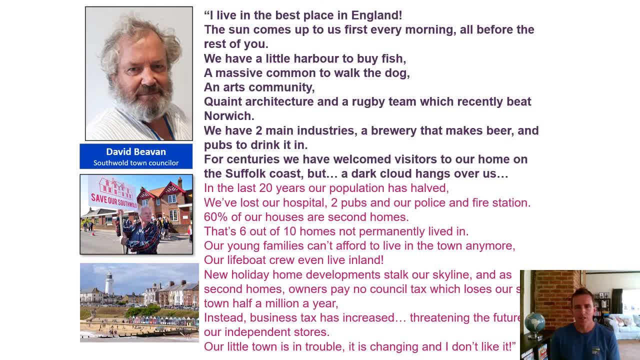 So this is something that is creating a massive social economic challenge to town board goes on to say that our little town is in trouble, It's changing and I don't like it at all. I'll refer back to a couple of the other things that you'd said and speak in a while. 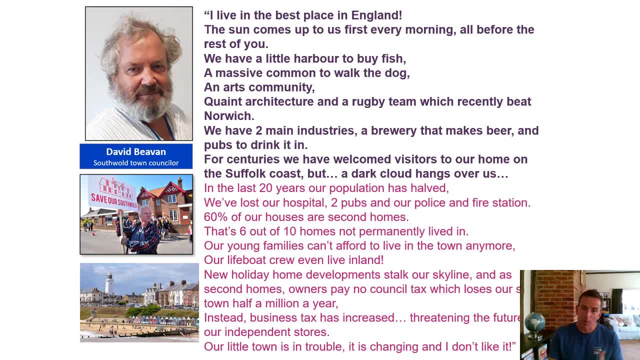 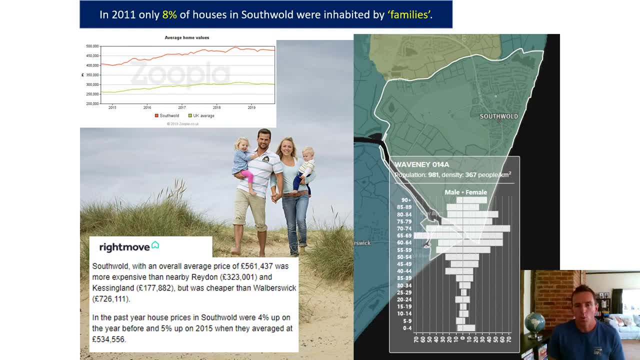 but it is a changing place From a human perspective, even though that might not physically look the case, and the change is evident when you do a bit more digging. amazingly, South board has only got 8% of its houses occupied by families. Only 8% of the houses in South board are occupied by families. 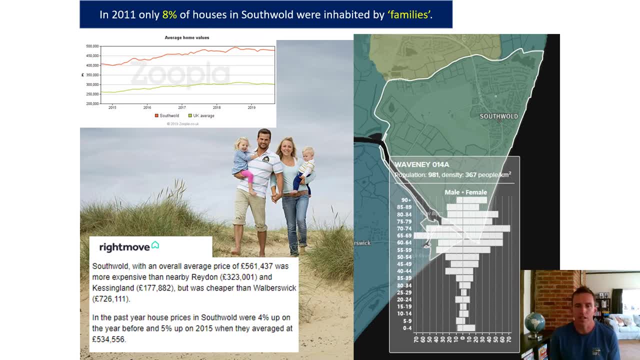 When you look at that population perimeter there on the right hand side of the screen that represents the South board area chain by the white line on the map above it. That is probably one of the most distorted population pyramids for any community in the UK and you can see that very. 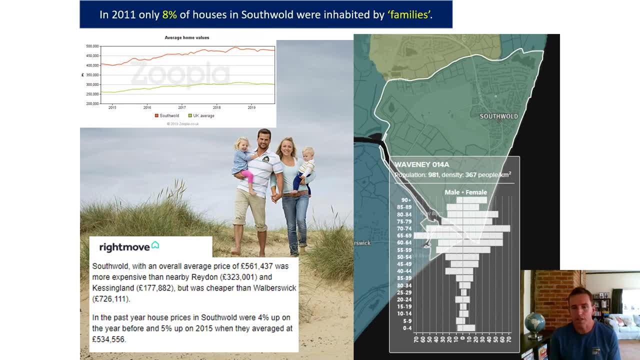 very few people under the age of 40 are fortunate enough to live in the town board. The local primary school, which is next door to where we're based as a role of about 58, currently only have three permanent teachers. They have classes one and two together. 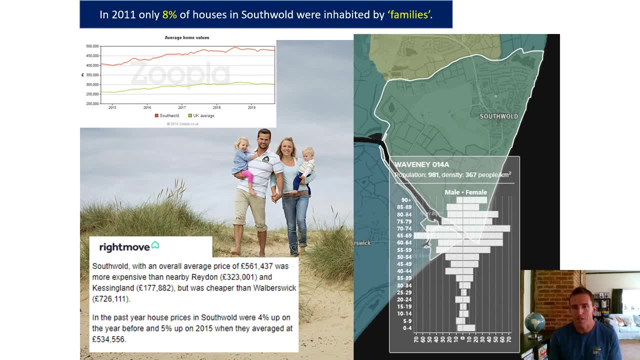 three and four, five and six together. It's under threat and it potentially in the next 10 years, may not exist. South board has this distorted permanent population of older people, So these residents that appear on this population pyramid here are the permanent residents that were locked in the 2011 census. 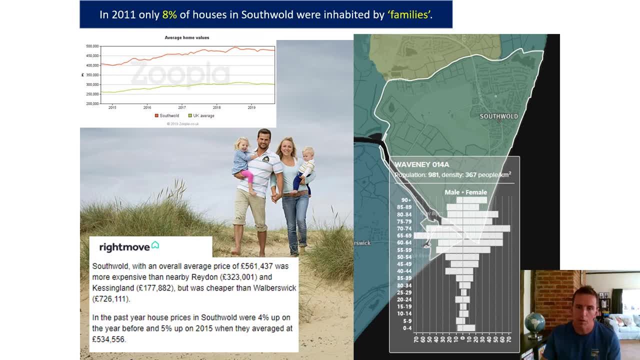 So the second home owners are not represented on this graph. They will be represented on wherever they live locally. So you can see that of the permanent residents, a huge amount of them are retired people. There's a significant amount of people over the age of 80 and 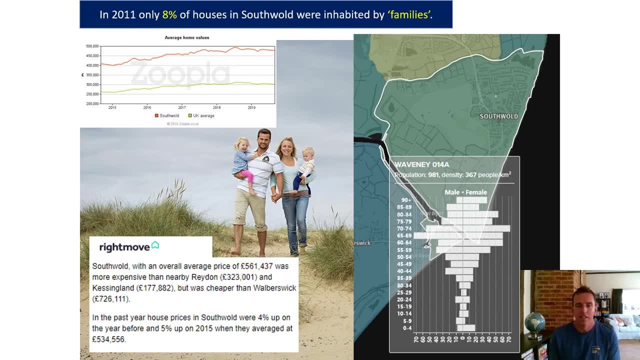 uh, very hardy group of females over the age of 90.. Now, unfortunately, in the years that have passed since 2011,. inevitably, some of those people will have passed And, um, that is not a sustainable population pyramid for any community. 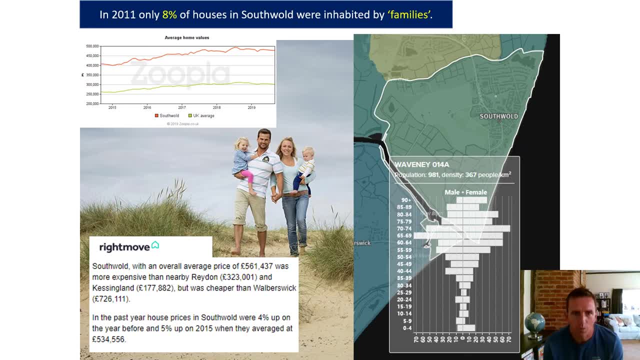 As I say on the left hand side. there are a couple of things before I move on, And one of the problems then of the second home ownership is this: inflating house prices. You can see the graph provided by Zoopla on the top shows the UK average house price with that kind of line. a little green color and the red line representing Southfold's average house price. Southfold's average house prices is almost about £200,000 more to buy the equivalent house in Southfold than it is generally in anywhere else in the country. There's data from Rightmove this year saying that Southfold has an overall average price of £561,000 or out in the town. 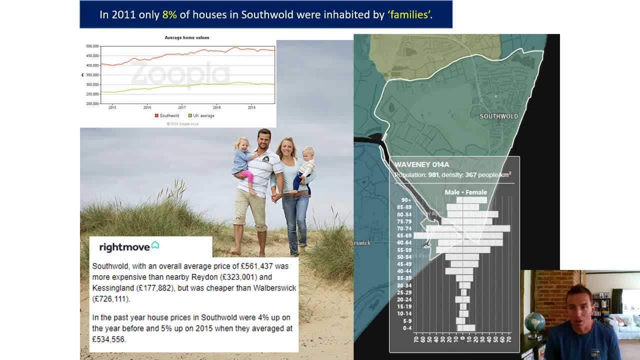 Now, most houses in Southfold are terraced houses And they're not actually anything special that you'd find them in any town or city up and down the country. There are some fairly grand ones, but most of them are pretty ordinary And 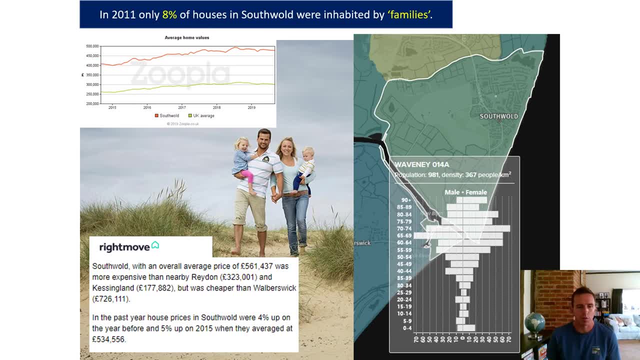 um, you know it's by two houses in nearby Ipswich, probably three for the same amount, for one price for one house in Southfold. So it's hugely inflated. This is one of the problems. So in your booklet here, fourth page, 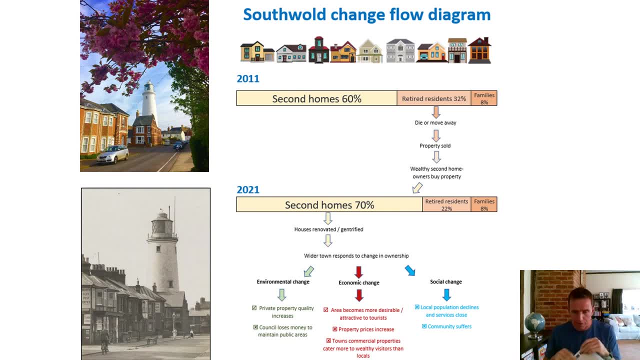 I think, but David Bedden, the speech on the fifth page, on the fourth page, in fact the page afterwards. Now it's a fairly simplistic flow diagram, but we put it together and use it with students just to kind of reiterate this change that's going on in the town. 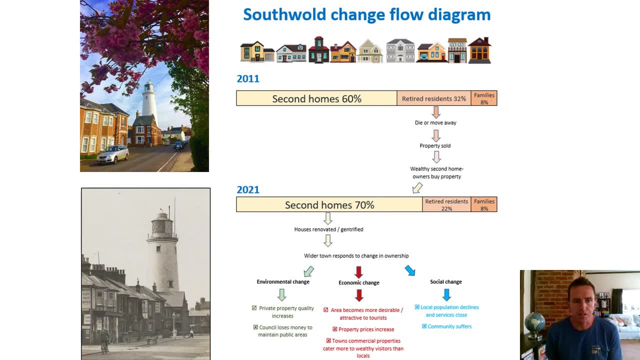 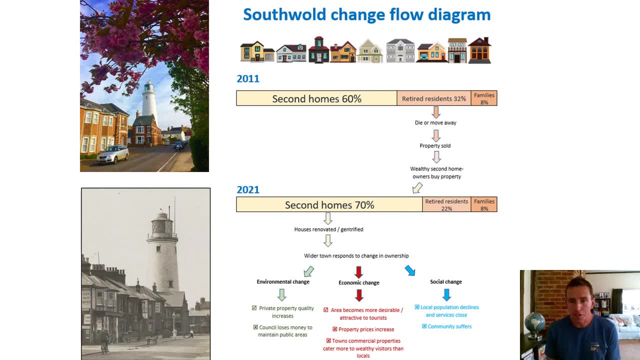 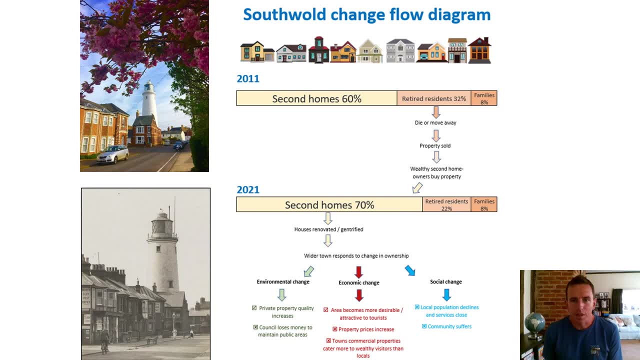 Now we know that over the nine years since then there has been a significant change to the numbers of retired residents because, unfortunately, a number of those people will have died or will have moved away, And it's those houses then that come up for sale. So there's not many houses in Southfold that are for sale, but houses that do come up are normally the retired elderly residents that have passed on or moved away. 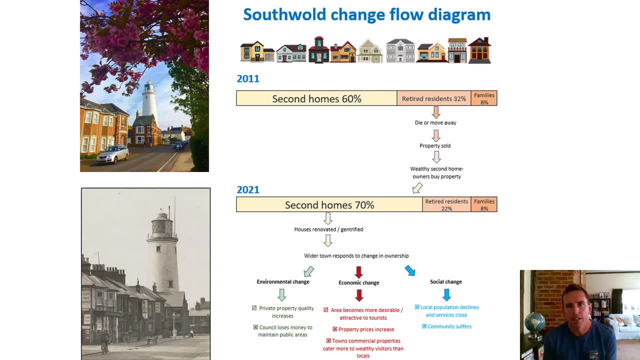 And if you, for instance, have an elderly relative that lives in Southfold and they do die and you inherit their property, you've then got kind of two choices really: You could either stick to move yourself and your family to Southfold, or you might choose not to. 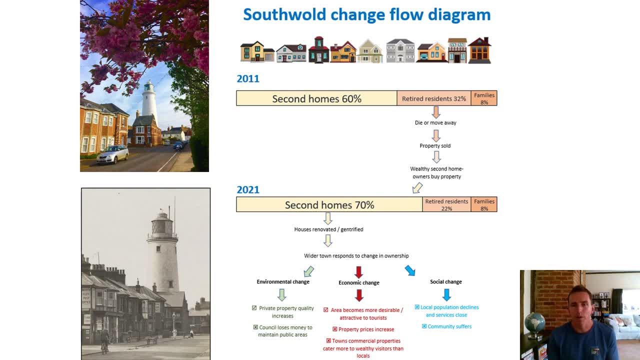 You could either do that and to sell that property- and, bearing in mind this is probably one of well, it is definitely one of the country's most prestigious and expensive places to buy coastal property and the average house price here is over half a million pounds. you might think, well, that's a no-brainer. 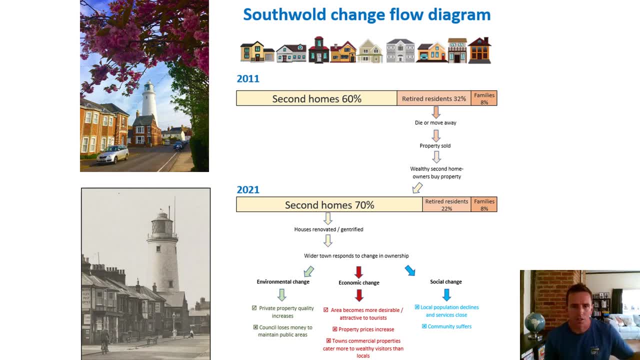 I'm going to cash in, we're going to put the property on the market, we're going to sell it and we can use that money for whatever else in where we live. So what generally happens then is those properties are, are sold, and in Southfold, you will notice, I don't know for whatever reason- very often in the autumn we see this kind of cycle of gentrification happening. 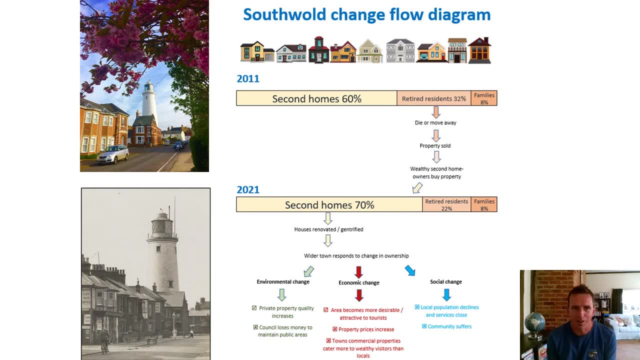 So the first thing that you normally see are the for sale signs going up around the town. Eventually- and it doesn't take long for those houses to be bought- we'll then see the for sale signs coming down And the next thing that happens is you either then get a skip, or you get scaffolding, or you get both going up outside the house. 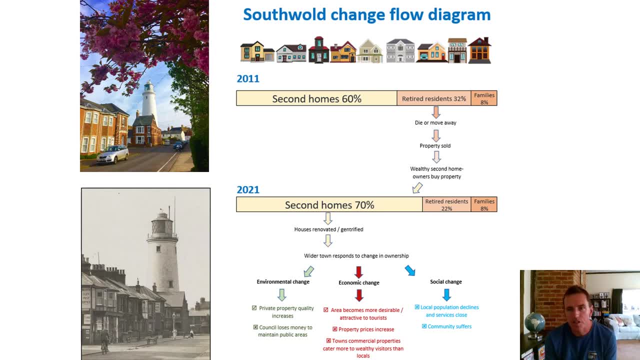 You then get the arrival of the white vans and the builders, And what normally happens with these properties that are being occupied by elderly residents is that they're completely gutted, they're completely renovated. The interior of the houses are completely refreshed- I might put in new kitchens, new bathrooms, have an extension at the back. 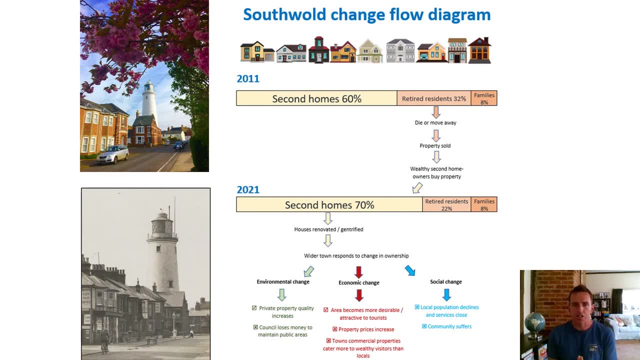 and what's happening is what's called gentrification. Gentrification is where the process whereby properties are improved and they are improved individually, not overseen by a council or any kind within the call of the council. gentrification is where the process whereby properties are improved and they are improved individually, not overseen by a council or any kind of council or any kind of council. 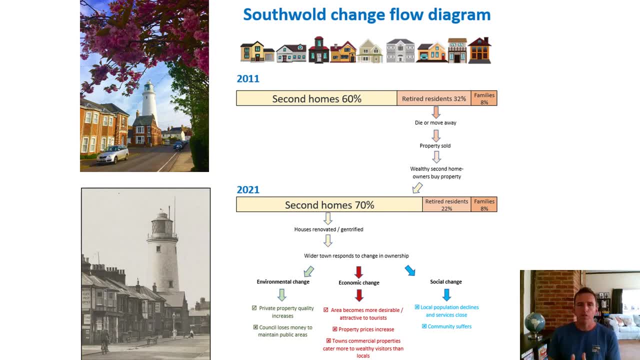 of a larger plan, but they're improved on a localised, singular basis. Gentrification as a process will often have a consequential knock-on effect. So if you have a few properties on a house on a street that get renovated, a street can quite quickly become more desirable and more. 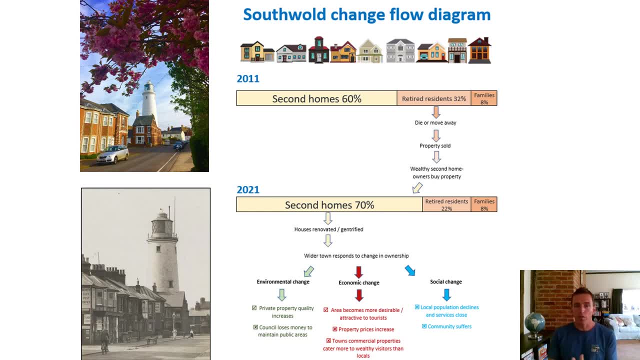 fashionable and house prices there might go up, and before you know it, in the space of 10-15 years the whole street may be gentrified. and not only then does the property on that street look better, but actually the services in the surrounding area then may change to cater for the people. 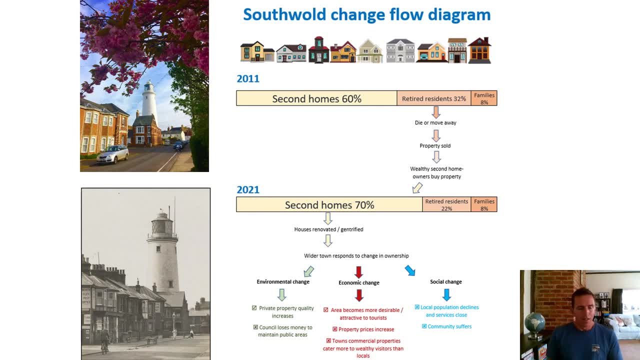 that are now there rather than the people that were there previously. So this street is a street called Stradbroke Road, where the lighthouse is. Stradbroke Road is a fantastic example of South Wales gentrification. You walk up and down this street. the properties are lovely, the level of 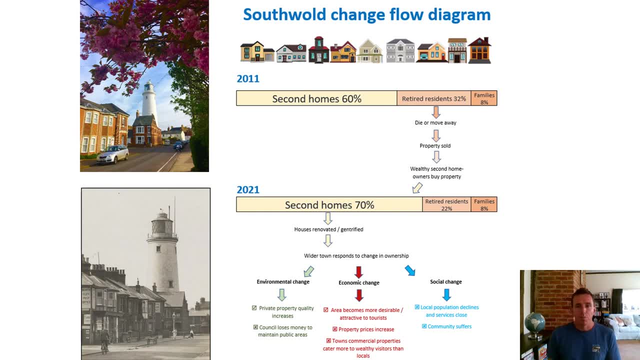 maintenance applied to them is second to none. you know they're pretty good, But you'll notice that most of them have got a holiday home ticker in the window or have got a key tape on the door, because the vast majority of them are second homes that are rented out to. 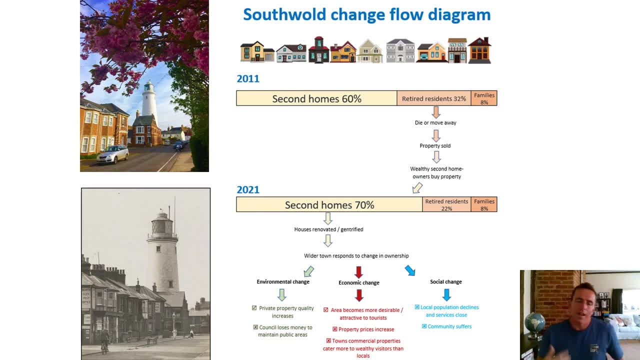 holiday makers. So what we are expecting to see, and we actually completed a report on behalf of the South Wales Town Council this last year, in the winter of 2020, where we actually did a study looking into what the current rate of expected second home ownership was in the town, based by what's currently available to rent On Airbnb and a number of the other main holiday rental websites and we estimate that currently we're looking more at. about 70% now of the homes in South Wales are second homes. The retired residents have inevitably reduced over the last nine years and the families we're 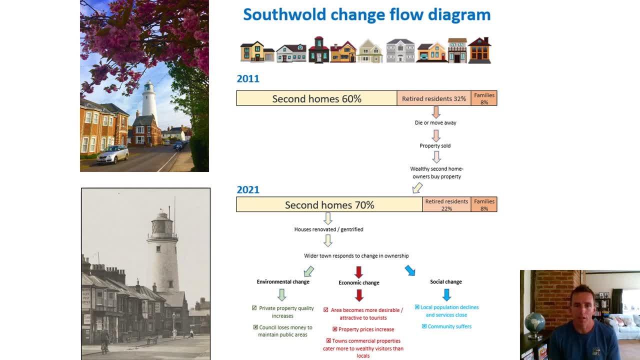 estimating to be kind of fairly consistent in the same. but the change has been in a reduction in the amount of retired residents. We've seen an increase in the number of second home properties. so below that then on the flow diagram that we've got here, is the impact of that increasing proportion of second homes. 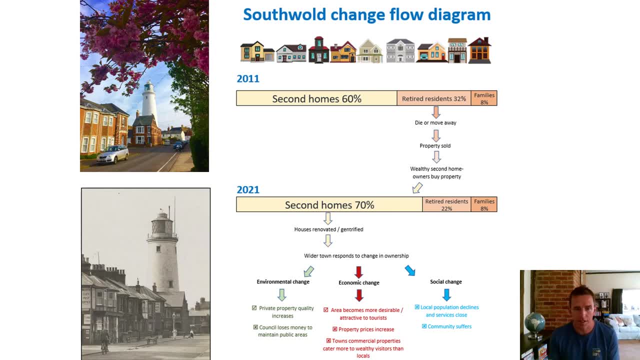 So the obvious consequences is that the houses are renovated and gentrified, like I just said, and then there is a wider town response to this change in ownership. So, from a physical, environmental change, things that you would you know more obviously see, then, is that the property quality? 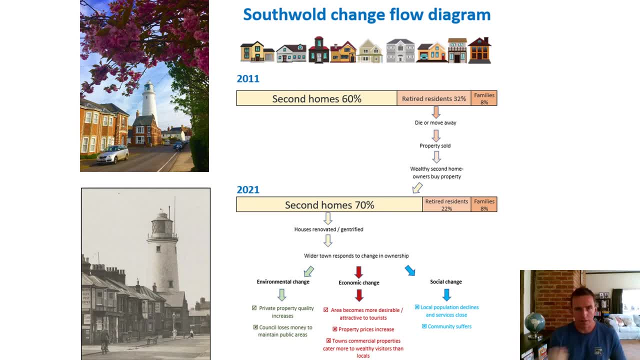 on these buildings increases and as you walk around, as I said in South Break Street, you will get the feel this is an affluent, nice place because the houses are lovely and are well maintained. So the private spaces in South Bond are very high quality. The problem is that the council is losing out, so 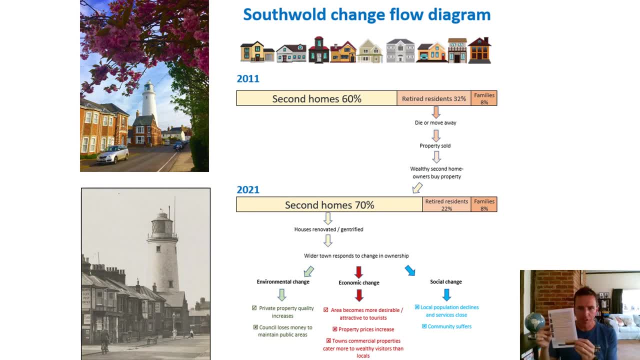 one of the things that I'll refer back to- Mr Evans speech here kind of towards the bottom- is that he second home owners pay no council tax. apparently this is the legal loophole: you pay no council tax on a second home property that you own and that then in a town where 70% of the properties are second homes is a major issue and in 2011 that cost Southwold half a million pounds a year in terms of lost income that they would normally get through second home council tax, so that will be even more. now it might be 600,000 pounds a year that they're losing out on, so that's money. 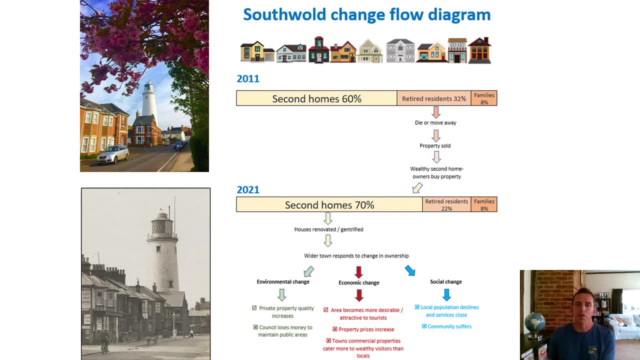 that would be in the town council's coffers that they would normally be able to use maintaining the quality of the environment locally. and this is one of the strange contrasts. in Southwold you've got a town full of very nice, very well maintained private houses, but public spaces, public money is. 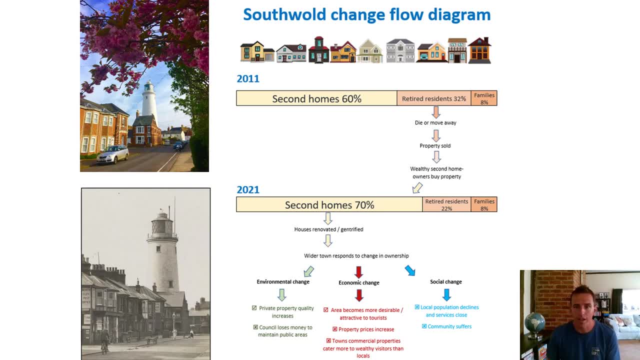 needed to maintain those spaces, such as the park, the seafront, the railings, the benches, car parks, things like that are actually pretty tatty in Southwold and are not very special at all. you'll notice that the grass and a lot of the parks is not cut. there's very kind of rough edges to Southwold's seafront behind. 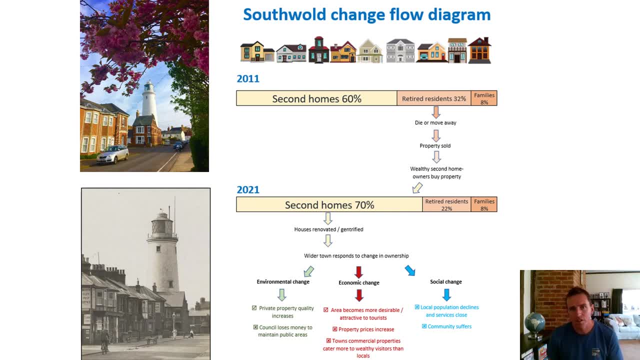 the beach huts. we have you know what could potentially be a very nice kind of rock gardens, cliff face, that kind of back the beach, and in lots of places like Felixstowe and Alborough that is the case. but in Southwold we've just got a huge collection of nettle and bramble. 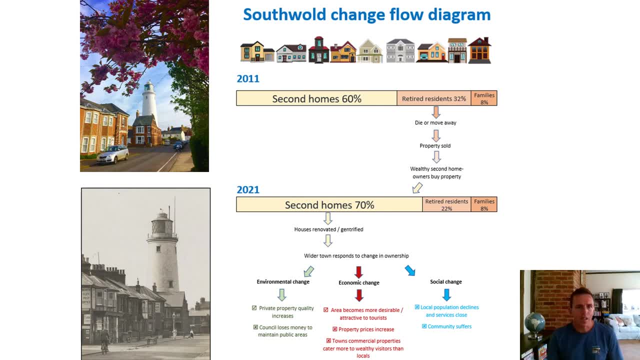 and actually they have a problem of rats there as well. a lot of the paintwork on the railings is flaking and definitely needs some love and tlc, and actually a lot of the benches are pretty hazardous because they've got broken wooden slats and they're just not that nice at all. so there is a 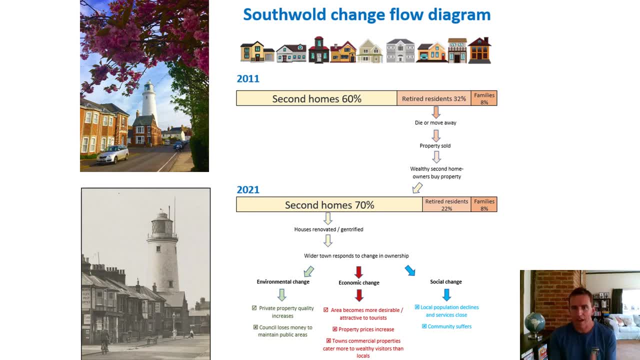 definite contrast between the quality of care and the quality of investment between the private spaces in Southwold and the public spaces, leading from a consequence of Southwold town council having less money to spend on these maintenance jobs due to the fact that there's so many second homeowners. 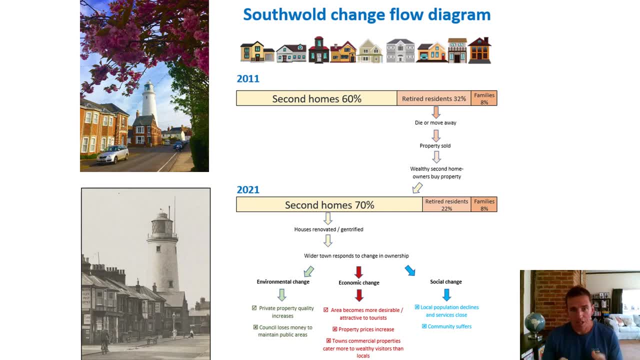 not paying council tax. so some students use that- that issue as the sort of their nea and they look at you know. so what impact has the increased amount of second home ownership in south wold had on the town's environment? more obviously, the economic change is one of the major consequences of this rising tech and home. process, the area is much more desirable, um so house prices here have skyrocketed. like you said, it's become much more desirable for not only second homeowners but also for tourists. so house prices increase, but also that price of pretty much everything increases. you can go into some shops in south wold and expect to get a sausage roll for. 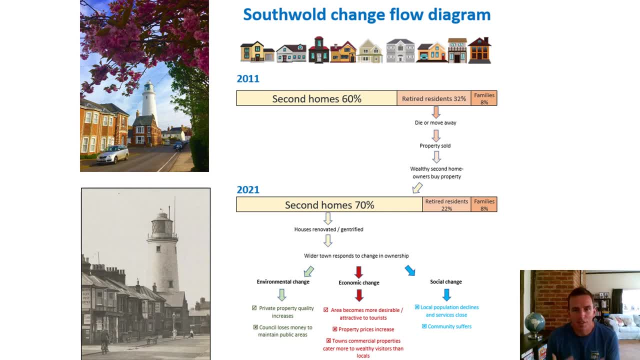 lunch and pay over five pounds. um, you know, some of the things that you buy in the town shops are massively inflated because you're having to buy them from posh delis rather than greg's, for instance, so there's no greg's in south. 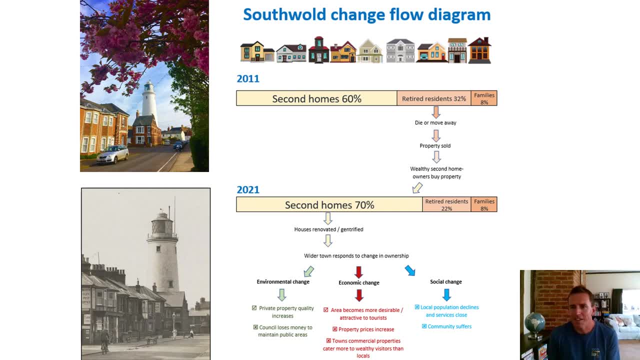 wold, because these affluent second homeowners don't want to be getting their lunch from greg's and getting it, you know, a sausage and bean slice. they would rather get something that is a bit posh and a bit, you know, more, more elaborate. so there is a, an economic 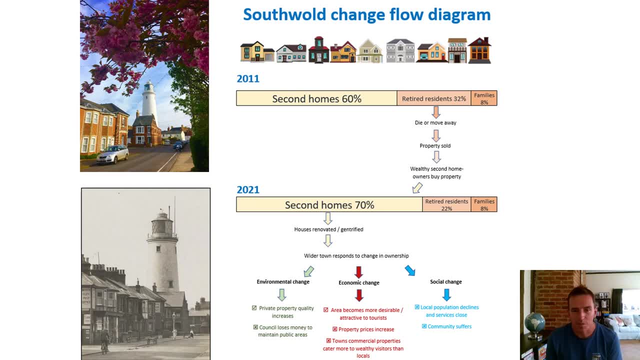 impact, um, not just in terms of the housing prices but also in terms of things that you can buy, so that the high street has responded also to the change in um. you know who is in south wold, so this is something again that's perhaps not necessarily obvious. gentrification impacts upon the physical. 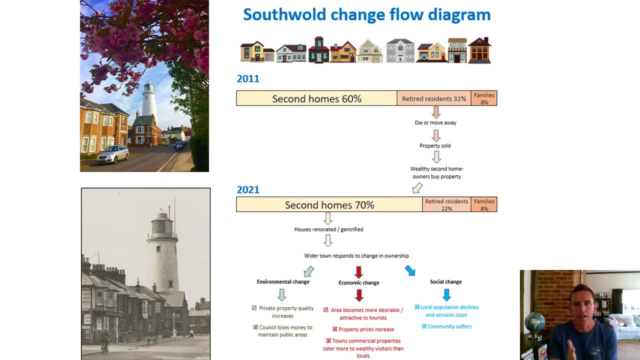 buildings that are changed. gentrification also then has this um knock-on effects on the high street and the services for a town, and south wold services and shops are actually now no longer for local people. south wold services and shops are catering now to the affluent visitors and the holiday. 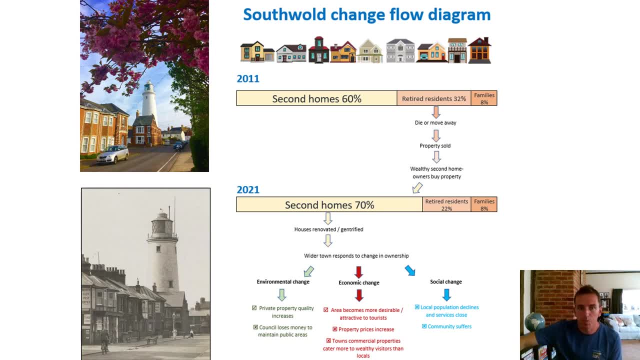 makers that come to the town and the high street is full of nice boutique delis and cafes and you know these antique stores and high-end clothing stores and jewelers and stuff like that, and there are actually very few local stores for local people, um, and the things to buy in those shops, particularly those kind of sandwich. 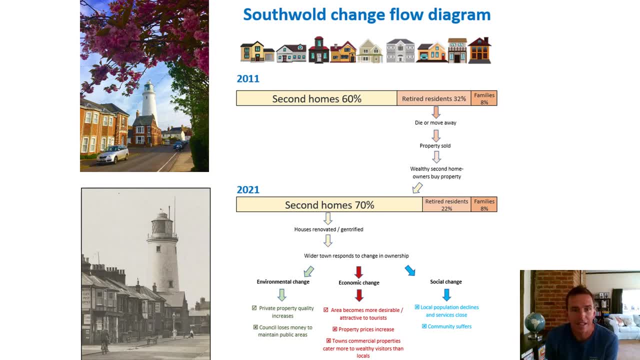 shops in delhi. they're actually really expensive. so if you are planning to, you know, have lunch in south wold and bring an extra couple of pounds, although there are. to be fair, there is a tesco and co-op and you can get your meal deals from those places. but 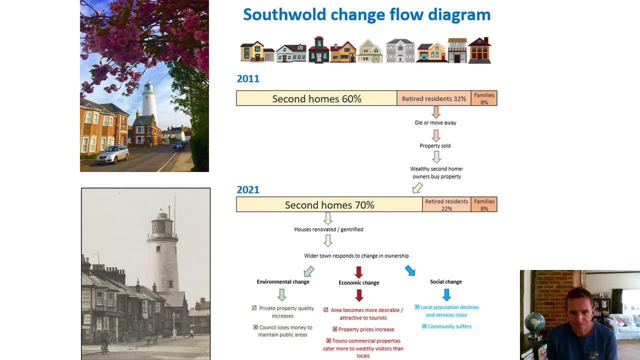 you know, the bakeries especially are kind of high-end. finally, the social change of its second home process has led to a declining local population and actually south wold can be a really boisterous bustling place in a sunny summer's day or sunny summer's months, but it actually is a very bizarre place in the winter and particularly midweek. 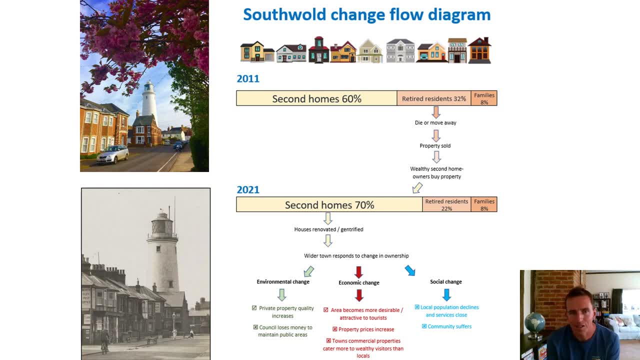 we have um in the uk very few places that are considered to be resorts, to be places that purely serve a tourist purpose. in places like france and spain they have lots of these tourist resorts actually shut down at the end of their summer season. they pull down the shutters and lock the 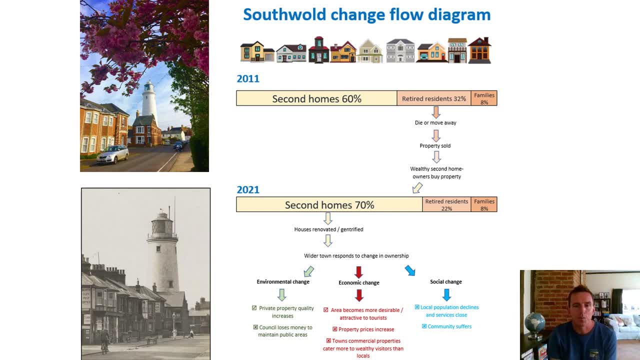 doors and they go away for six months or so. they open up again in the spring. well, in the uk we don't do that. we don't have these kind of purposeful resorts that are just have this sole purpose of being a, you know, holiday destination. but south wold is getting like that and um, in the winter, particularly midweek, it can be. 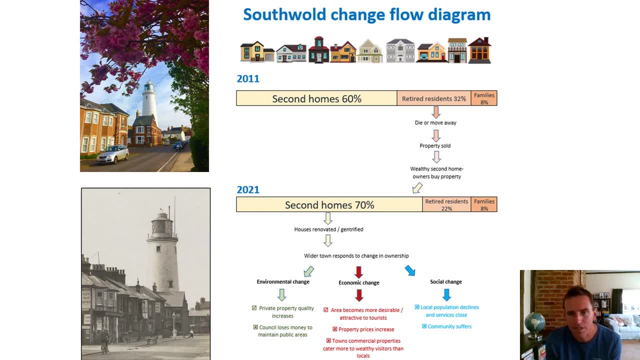 pretty much abandoned and i can walk back to my car at the end of the day and there'll be no cars parked up on the residential street that i parked and, bizarrely, no lights on in any of the houses because they're all empty. no one lives there. um, we were in south wold for the beast in, beast from. 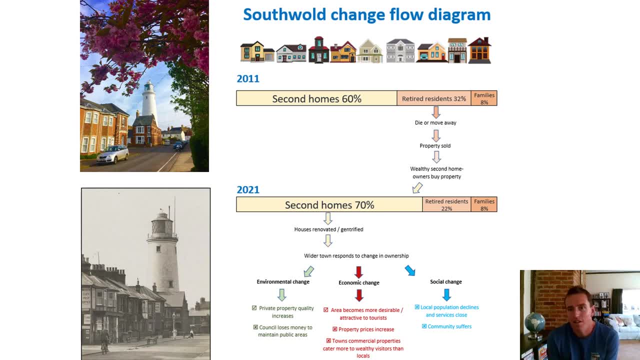 the east a few years ago and it was like a kind of a uh horror film. there's no one around and the streets were just kind of had snow drifts and, um, you know, walking down the streets there were no footprints in the snow because there's no one around. 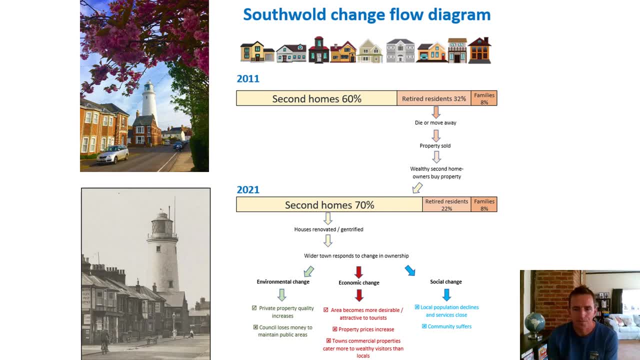 at all. so it was a bizarre place. um- and this is one of the things that we're doing- is it's it's massively impacting upon the local population and the local services. so the things like primary school- the numbers are falling- things like the library are under threat. 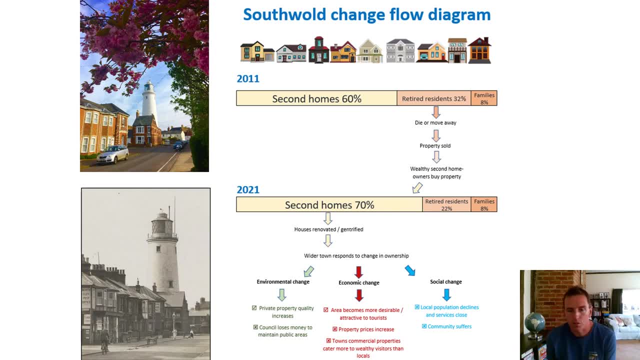 we've already already had the police station and the fire station closed, high school closed in the 1990s and in 2015, Southport Community NHS Hospital closed too, so the community suffered significantly as a result of this process. Even things like Southport's. 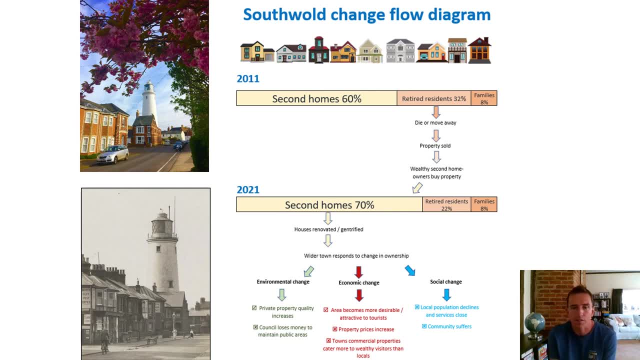 rugby team only had one player from Southport. the rest of the players are actually kind of driven in from other surrounding towns and villages. So again, some people may look at this idea about the social change that the second home owner process has resulted in. I'm sorry to spend so much time dwelling on that. 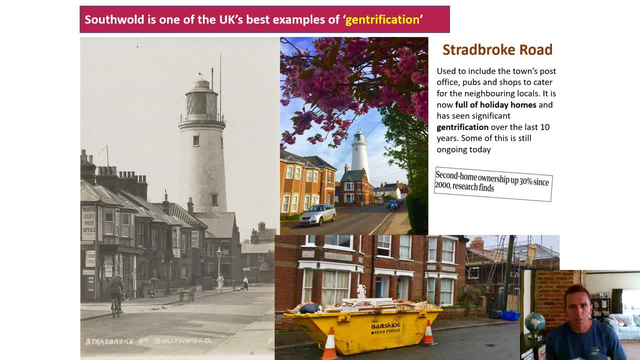 one. So in Stradbroke Road. I've kind of already mentioned Stradbroke Road and I've mentioned this process about the skips appearing and appearing on the pavements and gentrification process happening. but Stradbroke Road is definitely worth knowing about. It's one street away from where we are. 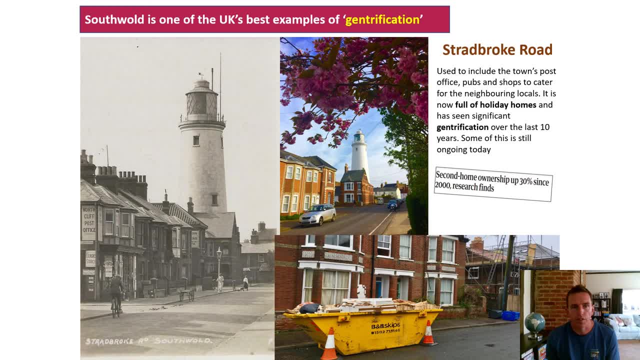 it's a street with a lighthouse on, and if you're doing a study on gentrification, I would say the street on Great Barrierage Road is a street with the lighthouse on. the suggest that this is one of the places that you focus on. it may even be that 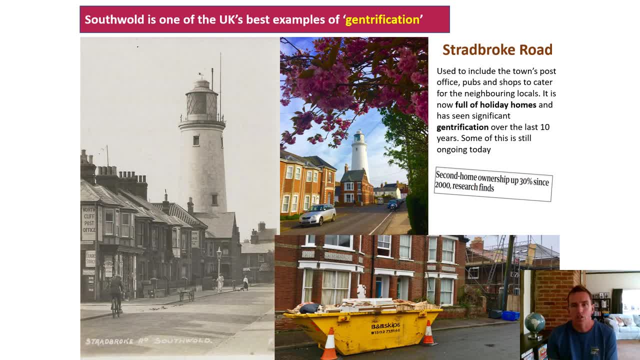 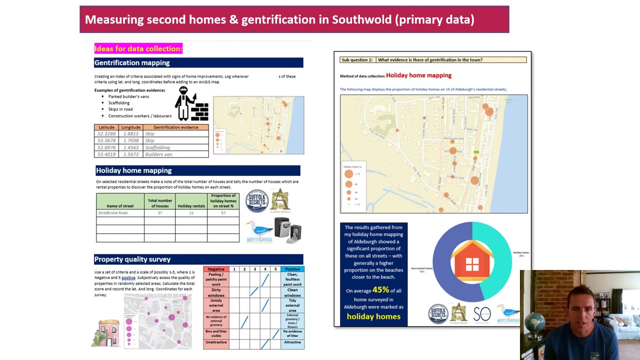 you actually say: right, I'm going to do a study on gentrification and my study is purely going to be around the changing identity and function and the impact of gentrification on this single street on Stratford Road. so some of the things that you can do and again, I think I've got these in the booklet- some of the 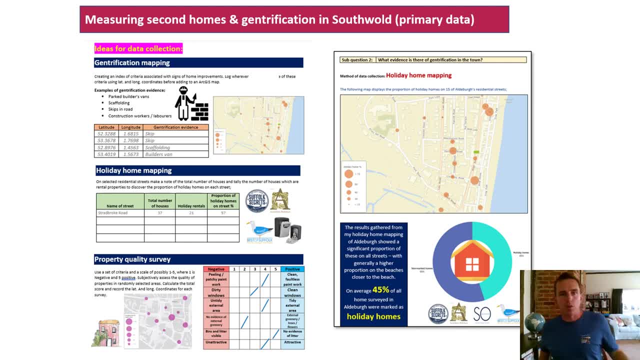 things that you can do to measure second-home ownership, the extent of the holiday rentals and the extent of gentrification in and around Southwold are gentrification mapping, holiday home mapping and property quality surveys. now I would suggest that you download the app called Jogit, and I'll talk about Jogit. 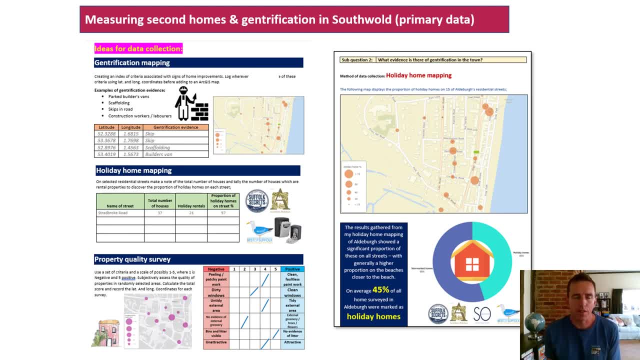 a bit later, because on Jogit there are 35 different methods of data collection that you can use and you can collect on your phone. the other thing that you can do to measure second-home ownership is to collect the data, and the other thing that's useful about Jogit is it gives you. 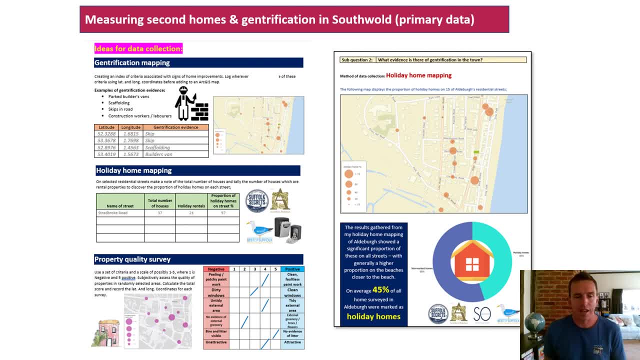 a suggested methodology. it tells you how to collect the data, and what I don't really want to do is suspend, you know, four or five minutes talking through the methodology of each of these different methods, and so, if you're interested in doing a study on second-home ownership or gentrification, what I am going to, 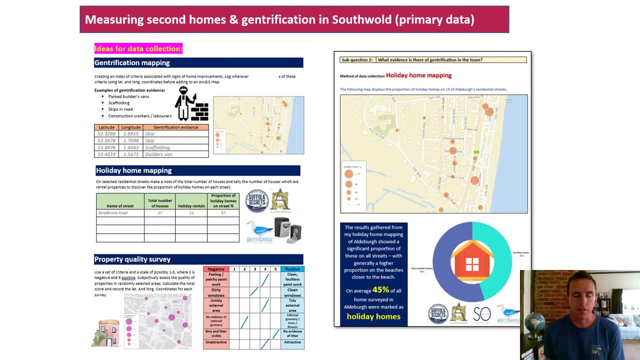 suggest is that these would be the methods that you would then look into, but what you'll then need to find out is: okay, well, what is gentrification mapping? how do I do it and where should I do it? then? but, yeah, I would suggest that these are that the 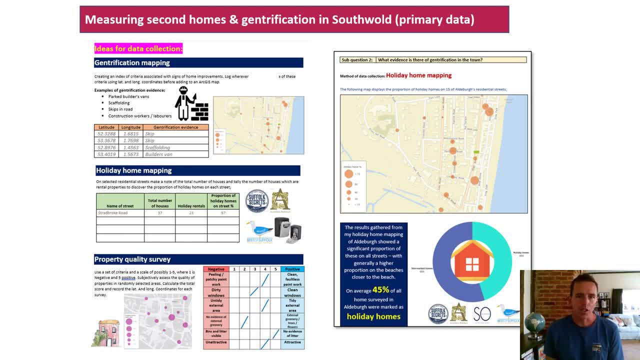 methods that would be nicely linked in with that, if you. one of the things that I'll say at this point as well is that a number of the methods of data collection that you can do on jog, it will do something called geo stamping your data. so geo stamping is whereby when you collect your data, you actually collect. 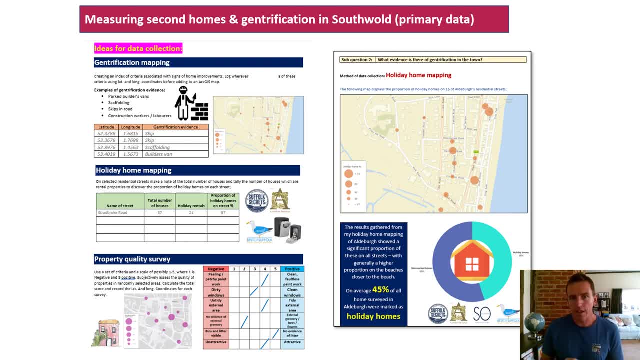 it alongside the coordinates of where you've collected that data from. so they лет. you're a latitude and longitude. So if you're collecting data on your phone, your phone is sending out, you know, a GPS signal and you can physically collect. I don't know a number of pedestrians. 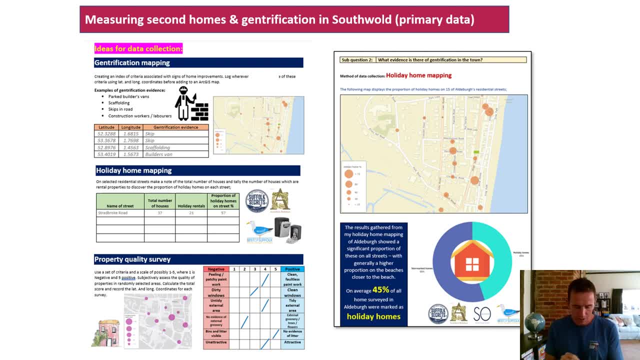 you've spotted on a particular street and then, rather than traditionally where you might write down what high street I spotted- 15,- your phone can actually record the latitude and longitude, give you the exact point that you've spotted those 15 people. So in this instance, here on 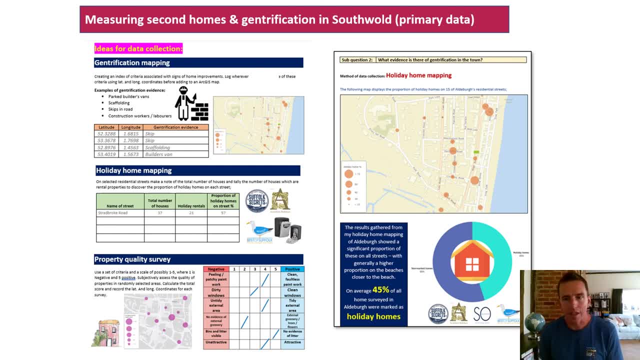 the screen. you've got gentrification mapping. This person here is logging any signs of gentrification that he sees in and around Southwold and they've logged skips and scaffolding and construction vehicles and whenever they do that, the latitude and longitude is logged. What ultimately they'll. 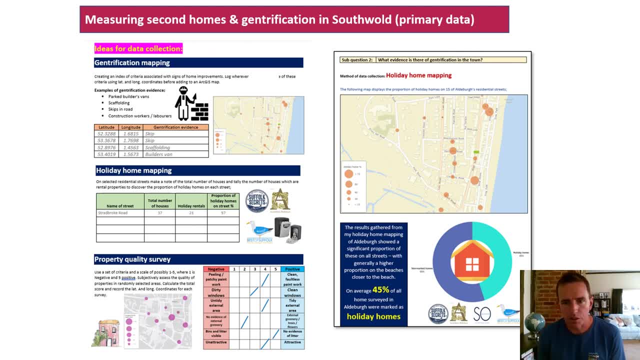 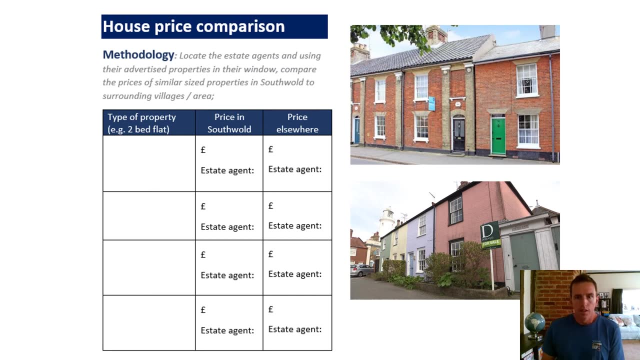 then be able to do is to create a map like these two that are on the screen here, which actually show the data that they've gathered in the actual physical location from which they gathered it. So it's worth just getting familiar with that too. Okay, any studies looking into gentrification? this is a really easy method of secondary data. 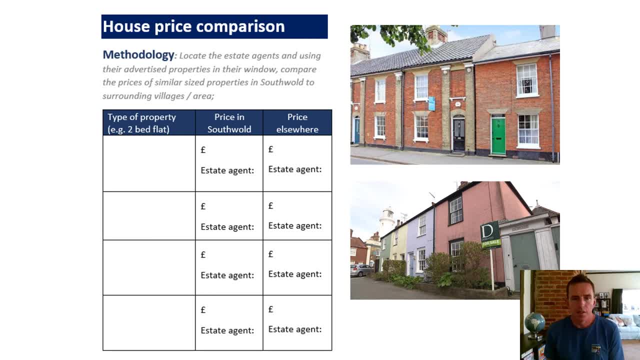 collection that you can gather house price comparisons. So, for instance, looking at websites like Zoopla or Rightmove, they give you lots of information about what houses are currently for sale and, obviously, the price of those houses that are for sale. So one of the things you could do. 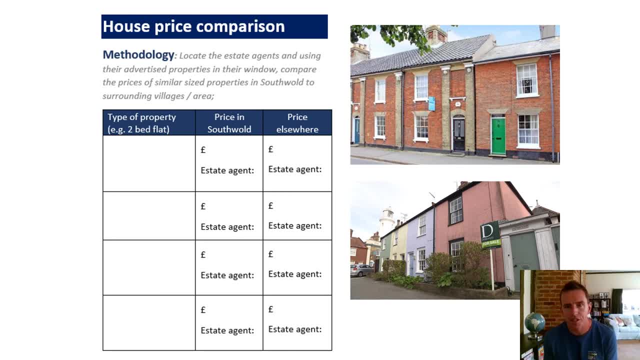 you could perhaps survey 10, 20 different houses that are currently for sale in Southwold, write down some of their characteristics. So for instance, are they a two-bed flat, are they a four-bed townhouse? write down their price and then somewhere else that's, perhaps I know somewhere that's. 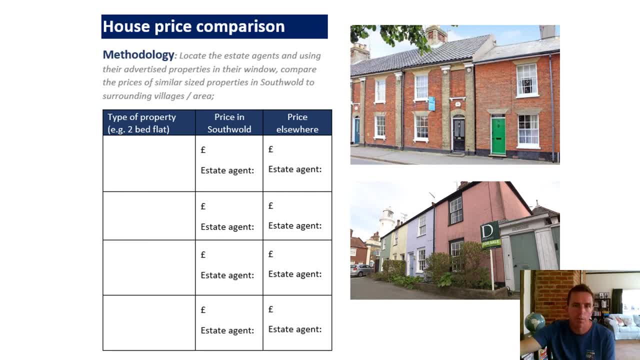 local to you or somewhere that's perhaps not affected by tourism. that may be more inland. you could try and find similar comparison properties. So how much is a two-bed flat generally in Ipswich, for instance, or how much is a four-bed townhouse in Ipswich? 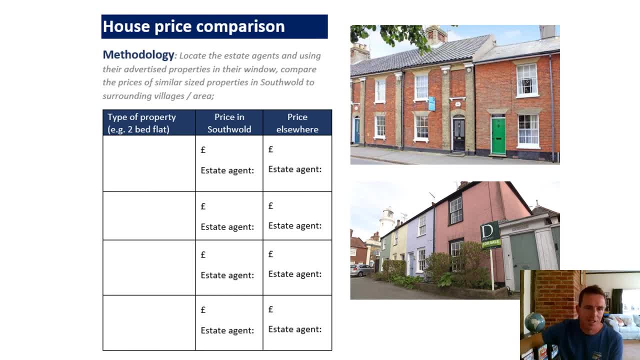 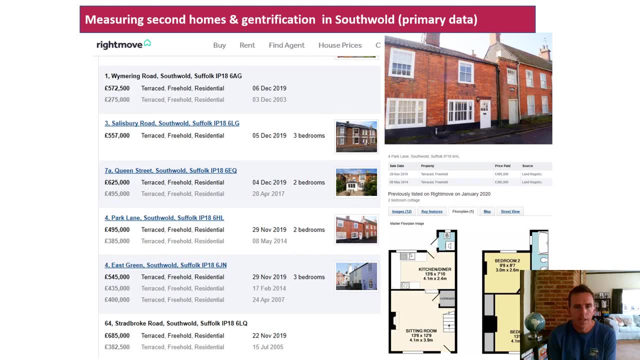 You can then work out is how inflated the prices in Southwold are for the same type of properties. The house price comparison is a really nice way of using secondary data. Rightmove and Zoopla have a huge amount of historical data as well, and actually, if you 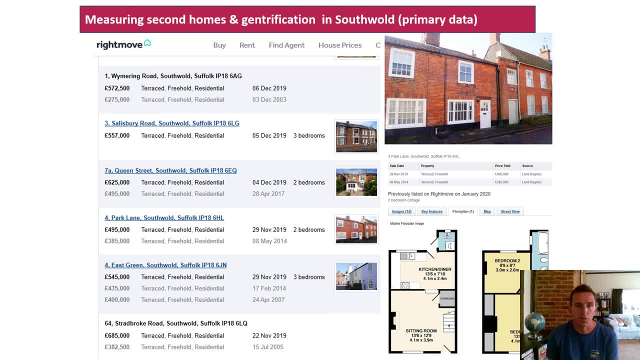 dig around a little bit, you'll be able to find lots of stuff that's really useful. This is a great feature of Rightmove, where you can click on properties that are for sale currently and you can then see historically what they've sold for in previous years. 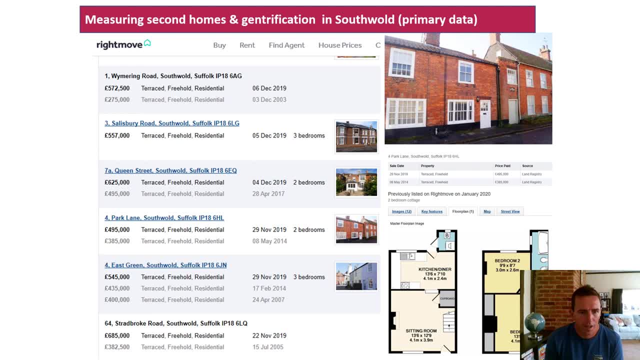 These properties that are listed on the left here. let's look at that one for East Green. so that's been on Rightmove's books three times in the last 13 years. It was sold in 2007 for £400,000, it's now being sold in 2019, so 12 years later- for £545,000. 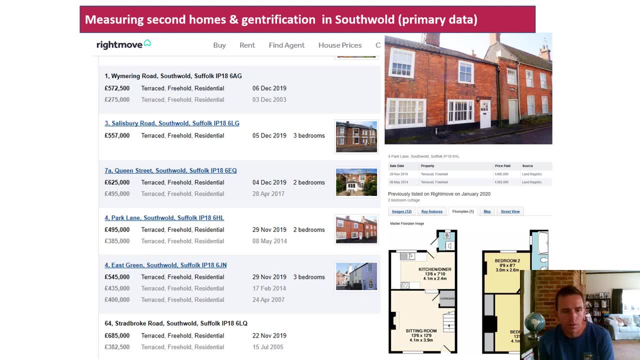 So in 12 years the value of that property has gone up £145,000.. Now it may well be that that's been significantly improved and renovated and extended, but in lots of cases there probably won't have been a significant amount of change. 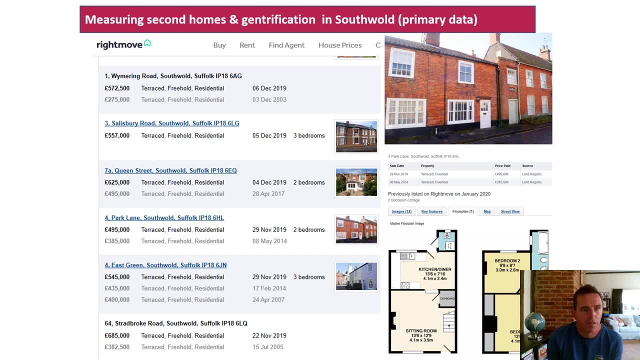 That one at the top there, Wimmering Road, that sold for £275,000. That's more than doubled. if I've got the maths right, that's now currently for sale for £572,000.. The one at the bottom as well, Stradbroke Road. look at the inflation there, the rise in the. 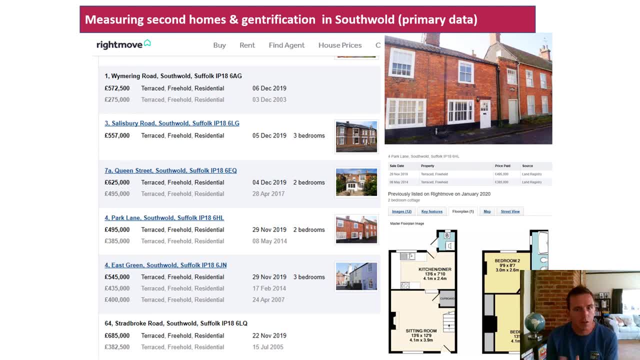 house price. So again, you could perhaps do some analysis of the data, look at how that's changed, proportions, what percentage change has been, and really kind of interesting data. One of the other things that that perhaps suggests as well is that one of the things 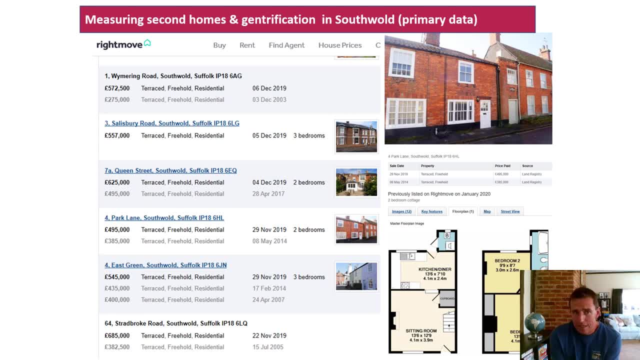 that happens in London I know especially, but is increasingly happening in Southwold, is that some people who've got a huge amount of money will buy up property with no inclination at all to use that property to rent it out but to just have that as a store for their cash. Because actually the property market in some places 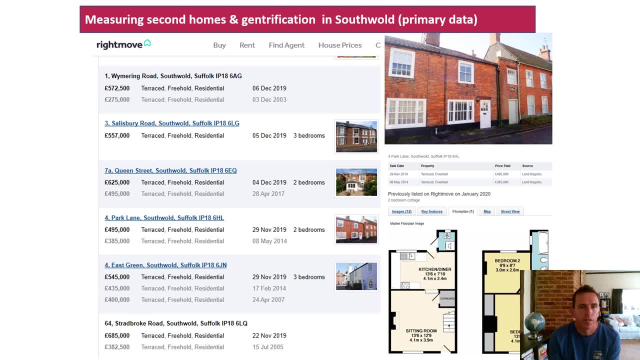 is increasing so quickly that if you've got £500,000, you would get a better return from your £500,000 if you bought a house in Southwold, sat on it for 10 years and then sold it than if you put that £500,000 into a high interest bank account. 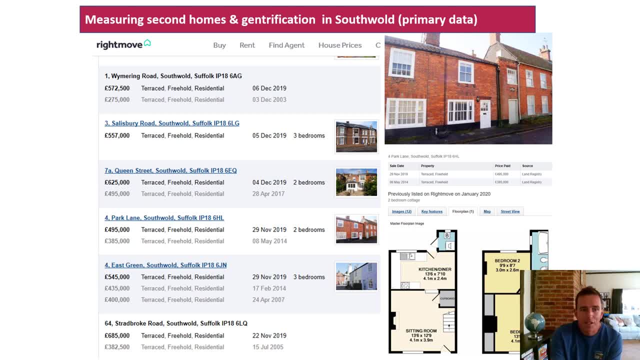 And that's what happens across the country in areas where there's significant demand for properties. So there are a number of properties in Southwold that are clearly empty, that have been bought several years ago. there's been nothing done to them. the owner of them is just sitting on them. 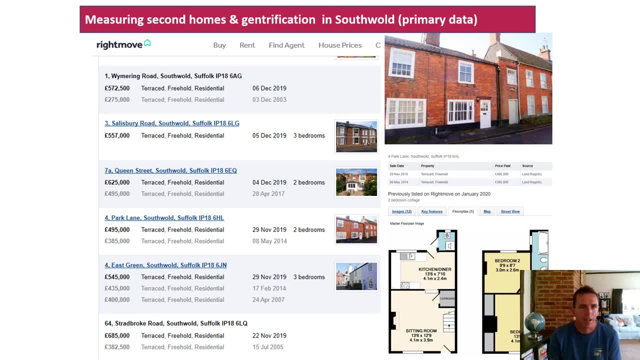 and when they feel like it they'll cash in, they'll sell it and they'll have probably made a couple of hundred thousand pounds. So if you can afford it, it's a very easy way of making money, but obviously to a community it's a disaster. You can't afford to have numerous empty houses. 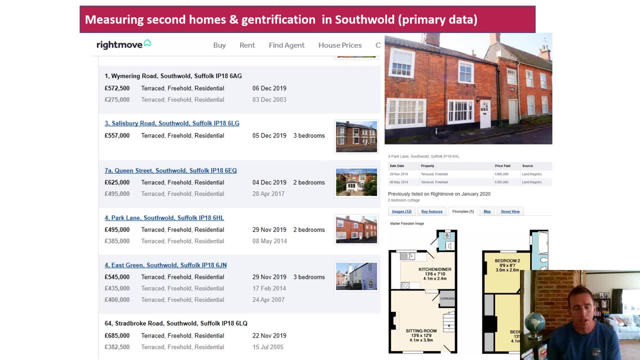 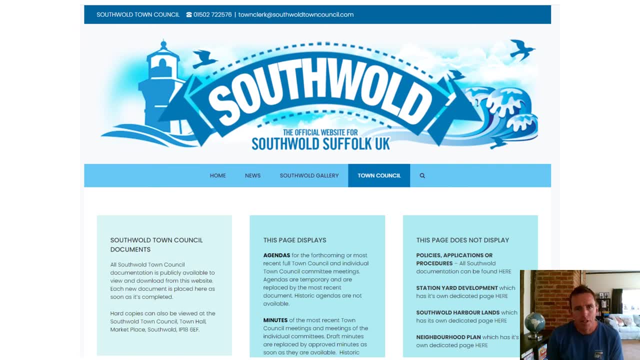 just essentially bank accounts for very rich people. So that's interesting and it's something that's definitely a problem in Southwold. This is a great source of information locally and not often something that people would perhaps look into, but in terms of gentrification, 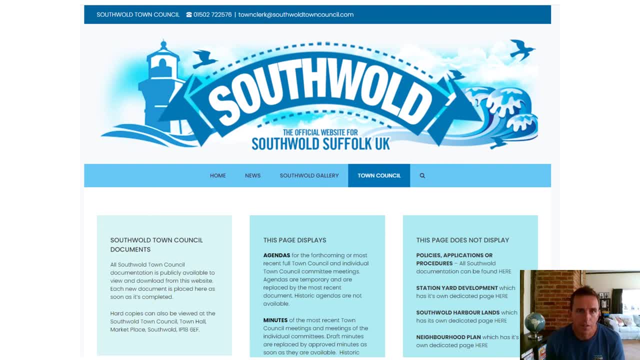 and amendments of properties. then people have to apply for planning permission to make often physical changes of any kind of significance to their houses. So they have to apply to the Southwold Town Council in our instance to get their planning permission granted. So they have to apply to the Southwold Town Council in our instance to get their planning permission grant. 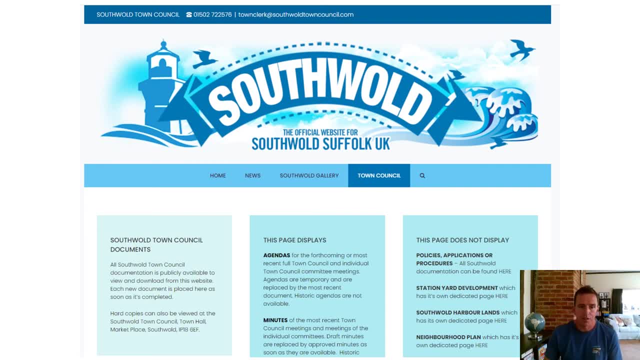 to get their planning permission grant. to get their planning permission grant. So the town council will meet regularly and as part of their meetings they have somebody who is taking minutes and they have a public agenda as well, and they also have to publicly present and disclose the discussions. 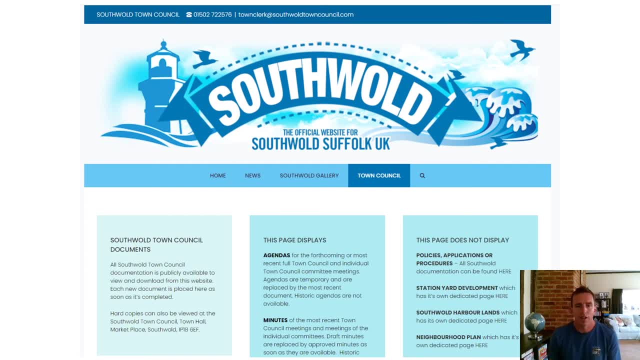 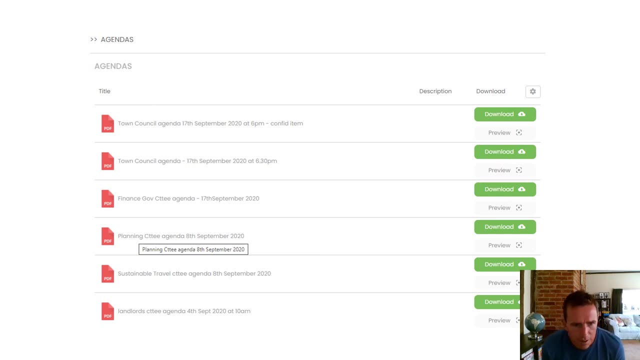 So on Southwold's Town Council website you will see that there are the agendas and minutes for all of the recent Town Council meetings. uh, those are just organized into pdfs and you would scroll down to kind of see that the newest and the latest ones here. one here: planning committee agenda 8th of september and then 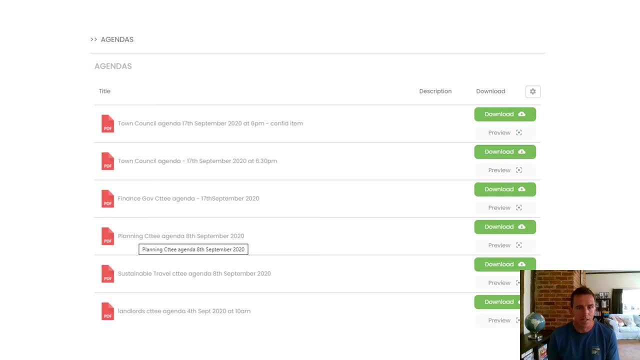 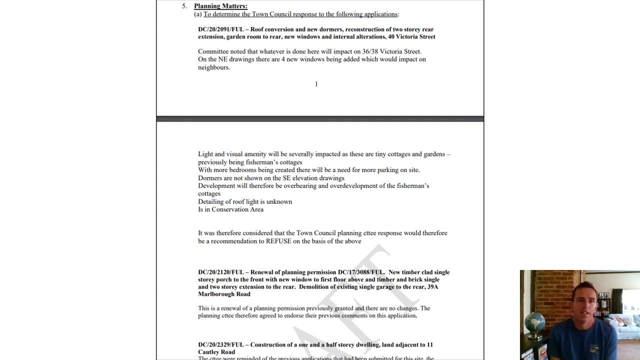 further down on that list is a planning committee minutes, so if you click on those pdfs you can then see what has been discussed. so this one, then, about meeting on the 8th of september. item number five on the agenda was to discuss planning matters, and you can see the first one here, a roof conversion. 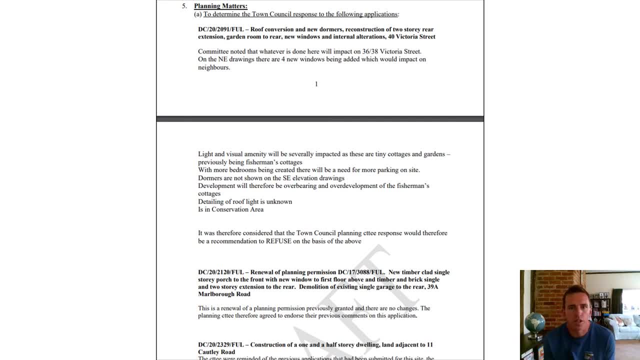 new dormer windows, a reconstruction of construction, food story extension, a garden room to the rear, new windows and internal alterations. so that is all gentrification, you know, extending, improving adaptions, and that was happening on 40 victoria streams. it says there that this might. 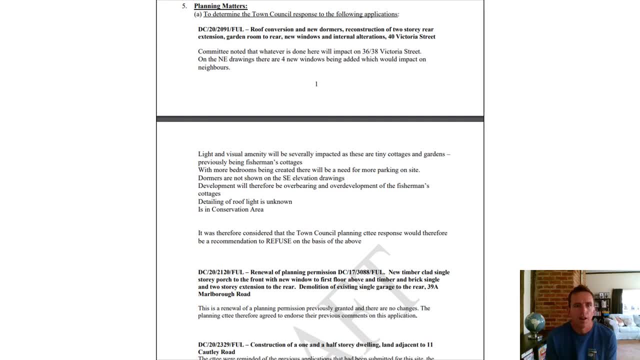 impact 36 and 38 Victoria streets. but what you can do is you can scroll down these minutes and you can look back and see what has been discussed and what has been discussed and what has been discussed, and you can look back at historical minutes, maybe over the last 12 months, to actually see which. 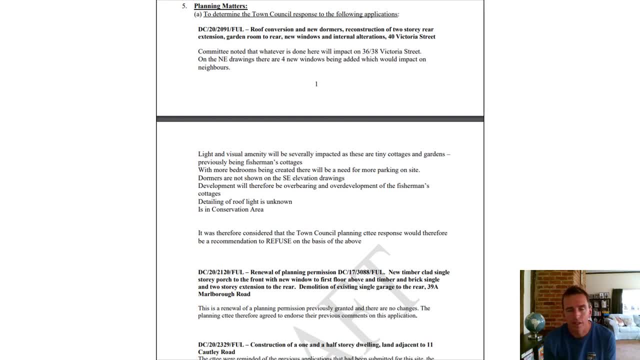 properties in southport have been gentrified, because they will all be on the town council's minutes, because they will all have to have been approved at some point by the council. so this is a really good sort of secondary data where you can look at the planning commissions. 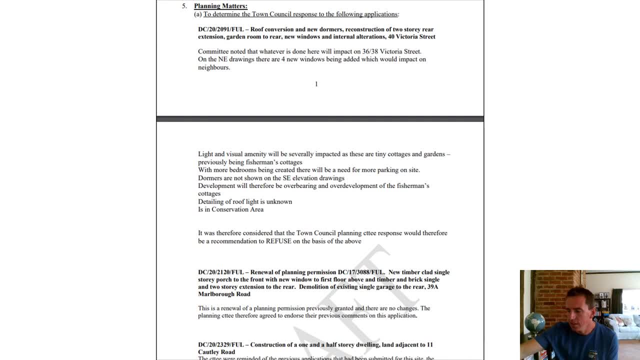 that have been granted so you can actually confidently say yep, from these streets have had planning changes or had, um you know, gentrification changes in this last 12 months, so this is a very good initiative. to do this, i would say. i think there'd be very, very few people. 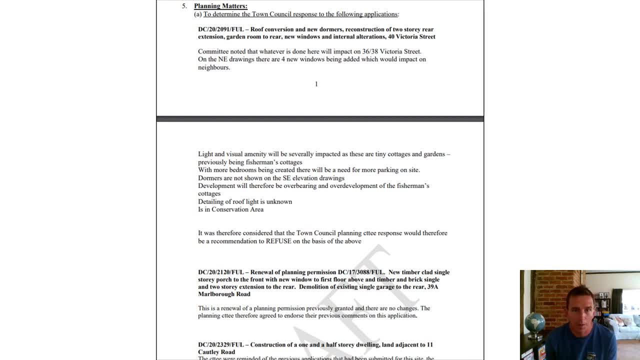 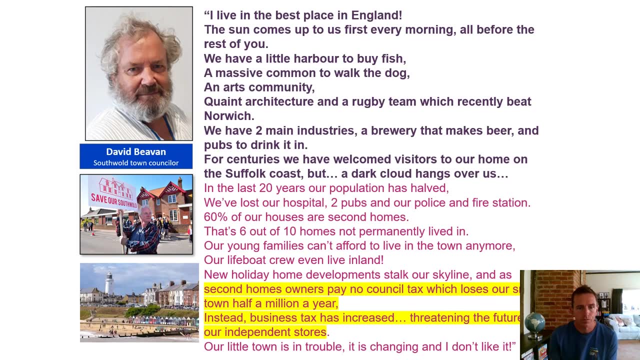 that would be doing this, but this is a very clever, effective way of using secondary data that is publicly available to reinforce your understanding about the extent of gentrification in southport. uh, we mentioned, didn't we, about Mr Bevan in his speech there saying that councils 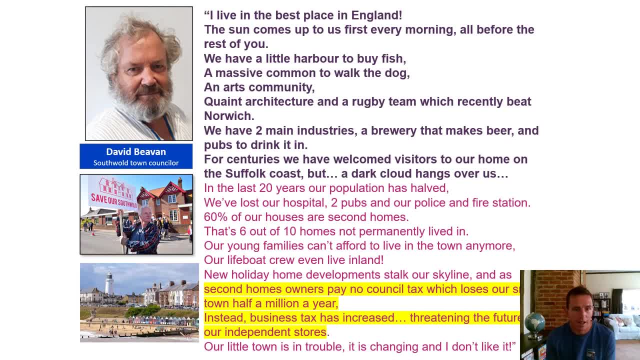 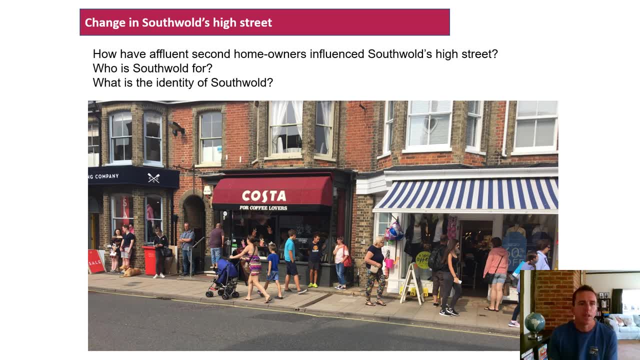 were losing out as a result of the reduction in council tax being paid. now, one of the problems then in southfold is that, because they are not getting enough money from their residents because of the limited amount of local residents, southfold town council has responded by taxing the businesses on the high street more, and they're actually using the 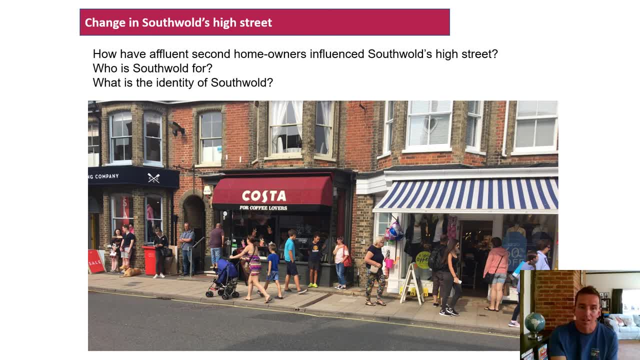 businesses for their source of income because they can't get that income from the residents. so over the recent years business tax on southport's high street has increased and as a result a lot of the independent small shops that southport's high street is kind of. 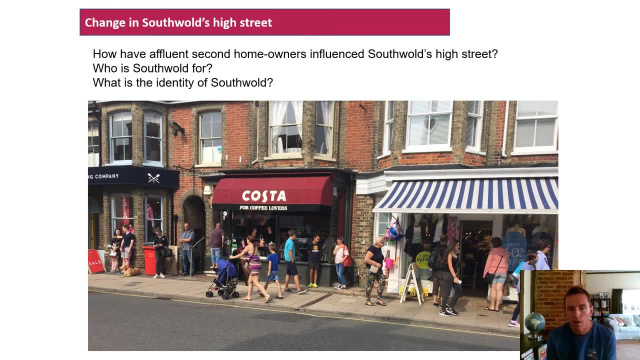 famous for locally have not been able to remain viable and have closed, and increasingly, chain stores are arriving. in southfold costa, for instance, um wh smith's, tesco's, um have arrived, and this is one of the things that is unique to southport: it's it's high street is actually one of. 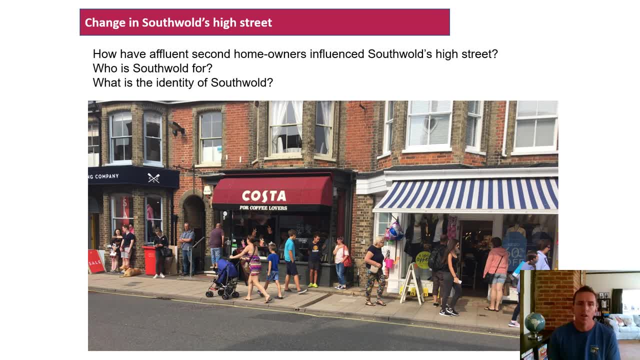 its key attractions, um, but the second home ownership process has completely changed and influenced the high street. not only has the high street responded by kind of having these delhis, which are, and these higher stores which are kind of catering towards these more affluent tastes, high street has had to change because independent stores have been priced out of being on the high 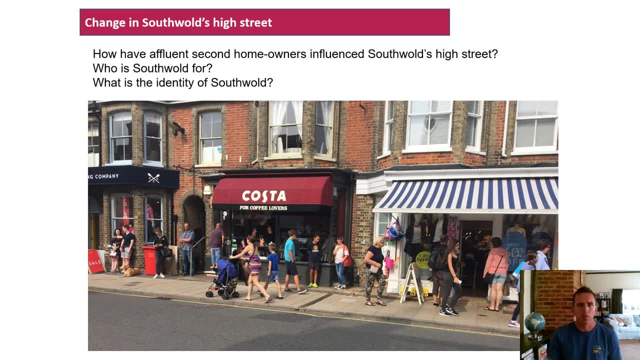 street because of these hikes in business rates too, so there's been a significant number of reasons as to why the high street has changed. onions was really a key part of the intersection with costos, VA, which were constantly miten mobile businesses have changed over the years and costos 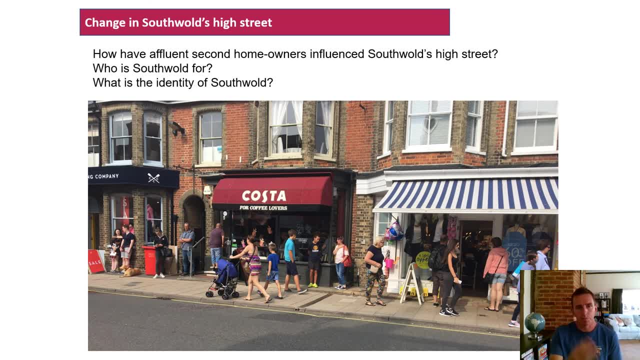 and that's one of the things that people can look into. so some students have looked at these issues. you know how has second-home ownership influenced the high street, even the wider question of who is Southwold for? what's the identity of the high street? again, those questions in terms of study, you might 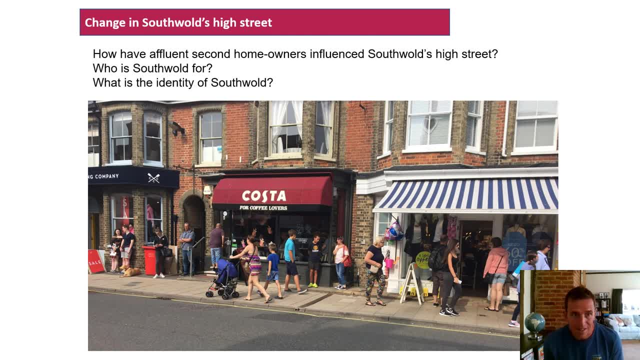 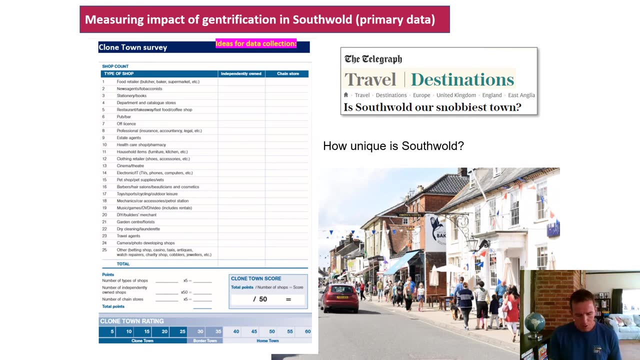 probably want to kind of focus that down into who is Southwold's high street for, who's it catered for? is it a local high street, or is it now this tourist resort high street or affluent visitors? okay, so again, I think this is in your booklets. 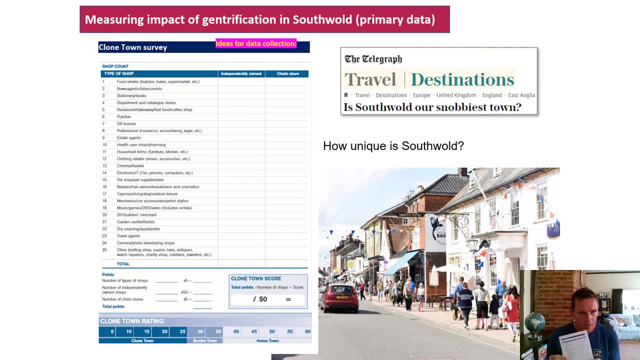 and there is a whole page here with the title clone town survey, and a clone town survey is a nice method of data collection, which is essentially kind of a development on land use survey. if you type into Google clone town survey PDF, this is the one that comes up first. I think you can just print it off. it's a 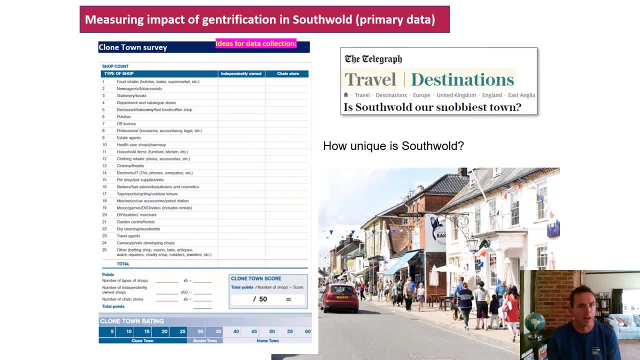 two-page document and on the second page it actually tells you how you complete. but ultimately it's a. it's a tally chart where you tally up the number of different stores there are on a high street and you kind of make a distinguishment between it whether the ownership of those stores is. 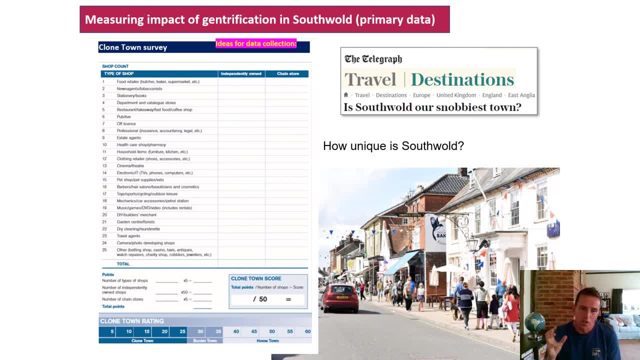 independent or whether they're chains, and then ultimately you can create a little equation or you complete an equation which gives you a score for your town and that score then tells you how unique that town is in comparison to other high streets up and down the country. so if you go into your local town or your local city, wander down the high. 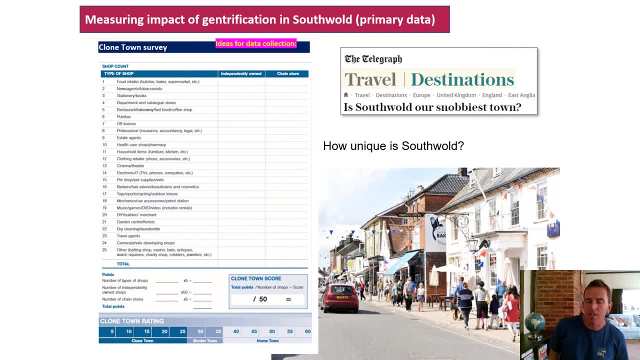 street. there are going to be the same shops there that you would expect to find in any other town city and there's going to be probably a Boots and a lush and a HMV, for instance. I don't know, is still HMV around, but you know what I 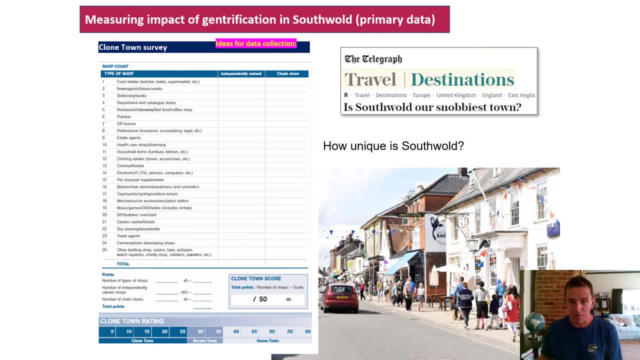 mean that you get those type of stores that are kind of permanent fixtures wherever you go in the UK. now that isn't necessarily the case in the Southport. like I say, there's no fast food, you're not got Gregg's. you're not got McDonald's, you've got 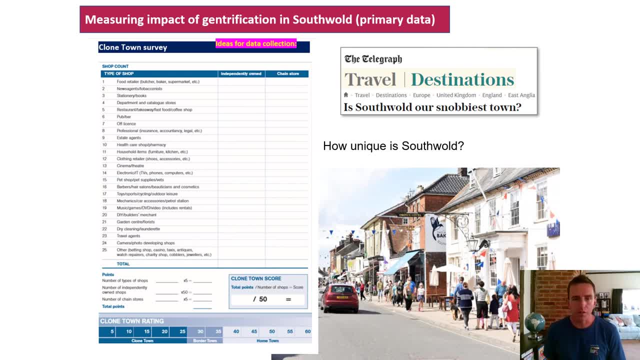 not got any of these kind of major chains really, apart from the odd few, and so one of the things that you could do is you could complete a clone town survey for Southwold to see what Southwold's current clone town score is now. as I say, 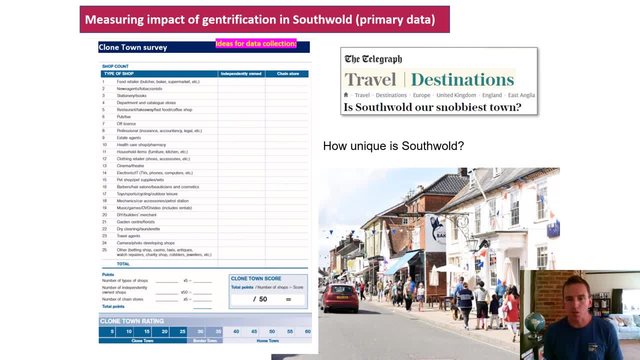 business rates have increased in recent years and independent stores have been lost and more chain stores are arriving. so actually, if you were to complete a clone town survey of Southwold ten years ago, you'd probably find that it was much more unique ten years ago than it was ten years ago, than it was ten years ago. 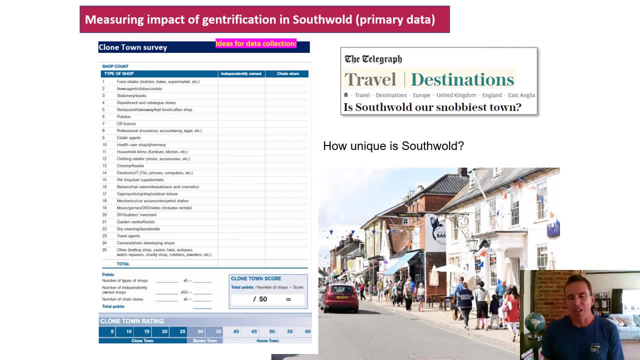 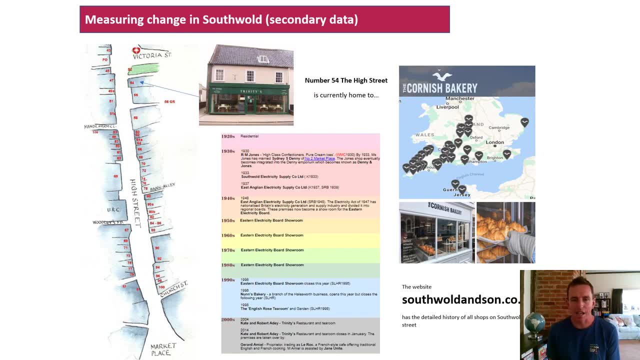 than how it is now. Jamie can't do that but actually you can, which is great. so it is possible to complete a clone town survey for Southwold historically as a result of this wonderful website called southwoldandsuncouk. southwoldandsuncouk is a kind of a labour of love between two local residents who have 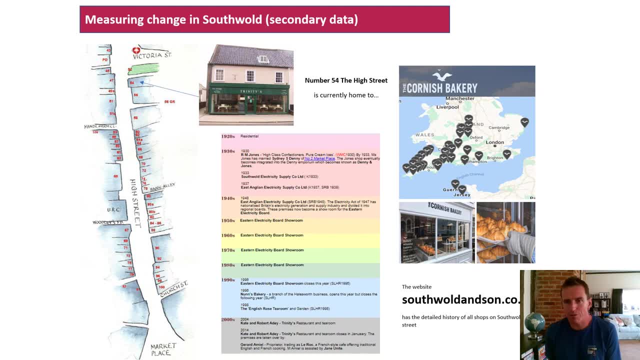 spent a huge amount of time in recent years putting together just an incredible resource to create a clone town survey for Southwold and the rest of the UK. I would also like to give a shout out to the Goodwill Trust, who have worked with every building, that we've been doing a lot of this research for a while, to show. 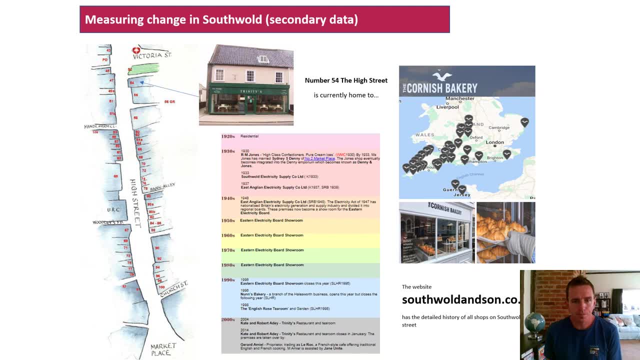 Southwold's changing human picture over the last 60, 70 years or so. what they've done is they've made this website that is basically full of lots of different street maps, and you can see on the left hand side the screen there, an example of 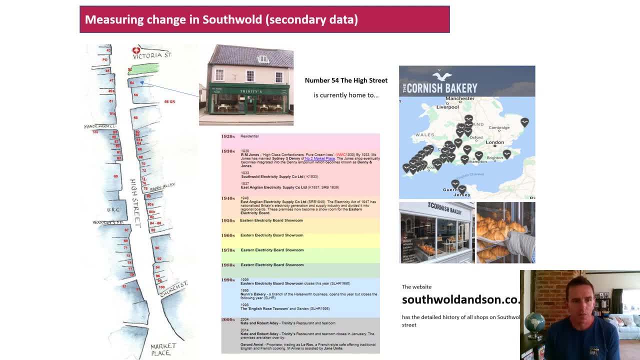 the High Street street map on the website with lots of little red numbers on each of the individual buildings. you can then click on any of those red numbers. it pulls up the kind of the rainbow chart that you've then got in the middle of the screen here to see how they are doing over the years. 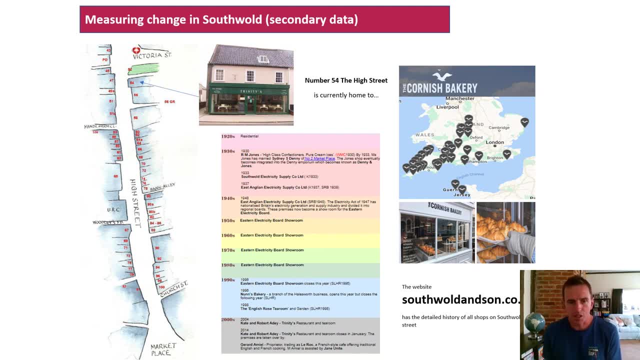 And this chart shows you the historical uses of each of those properties, going back as far as records belong, So in the 1920s, the building that is shown in the screen here, where it says Trinity's, that's number 54 on High Street. 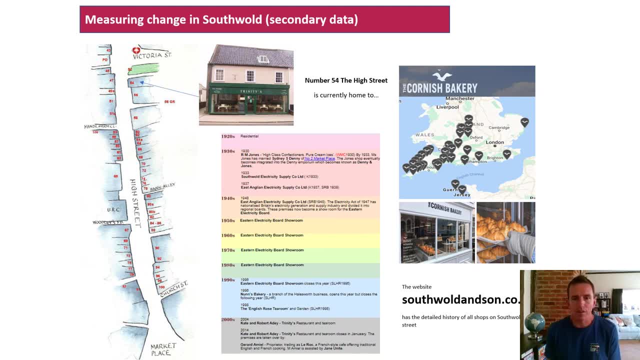 In the 1920s that was just a house. it was a residential property. It was then owned by the Eastern Electricity Board for a long time and it was a showroom. It then became a tea room and a restaurant and it was owned locally by a local couple. 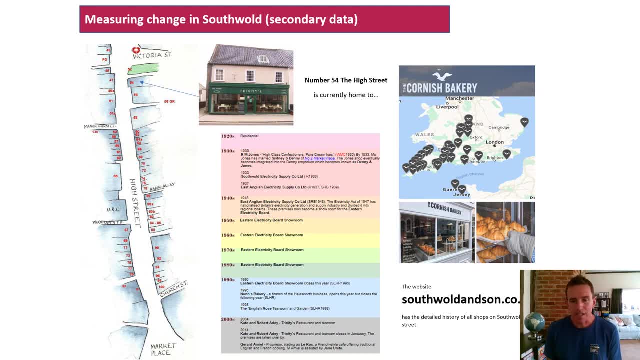 But in early 2019, it then changed and is now the home to a Cornish bakery, which is a nice shop and it's worth knowing. but it's not unique to Southwold And you can see the map on the Cornish bakery's website there of their stores and their outlets. 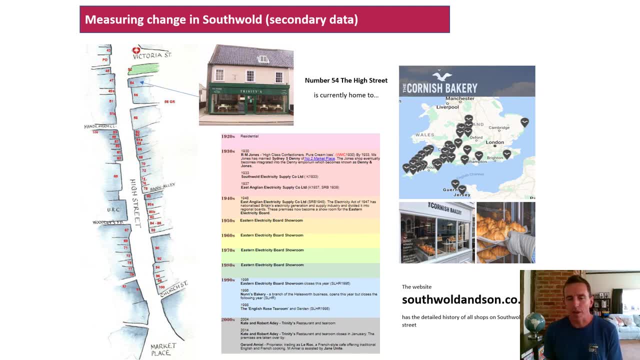 They are a chain store, obviously predominantly based down in the southwest, but you can see that on the east coast, there that's their Southwold store and they're branching out. So, having had, You know, a local use for so long and being a local restaurant run by local people, this is now a multi of, not a national. but this is a much bigger company that owns this and the profit for this won't necessarily be benefiting Southwold whatever. 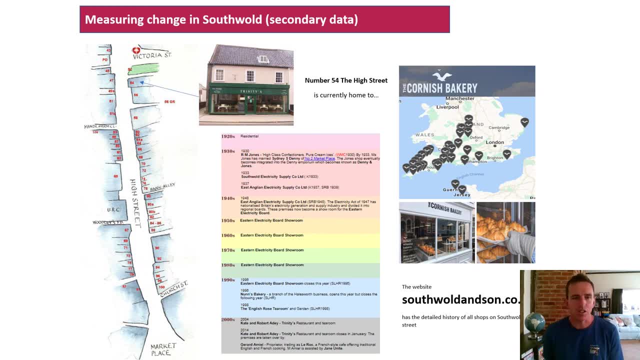 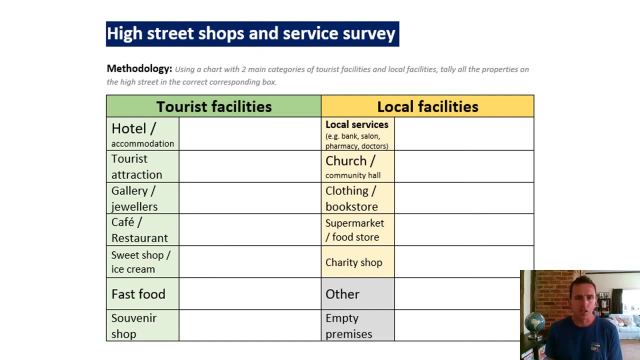 So it's changing to represent the changing nature of the High Street, where there's more chain stores. Other things that you could do on the High Street: if you didn't want to complete A loan to town survey, you could just create your own High Street shop survey. 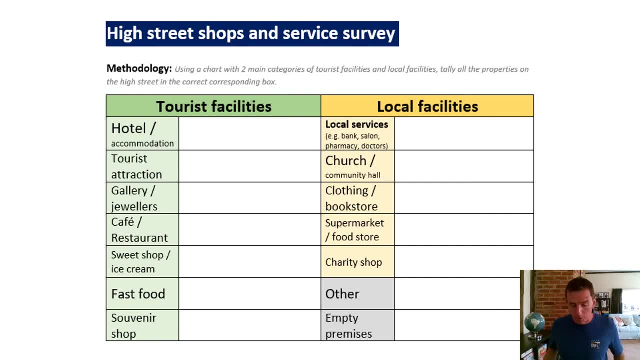 Maybe that you were doing something to show how or who Southwold is for- whether it's for locals or tourists, And therefore you could perhaps create something as simple as this: you know what shops on the High Street are for locals, What's which of tourists, and you could simply do a tally like this and then come out of the ratio afterwards. 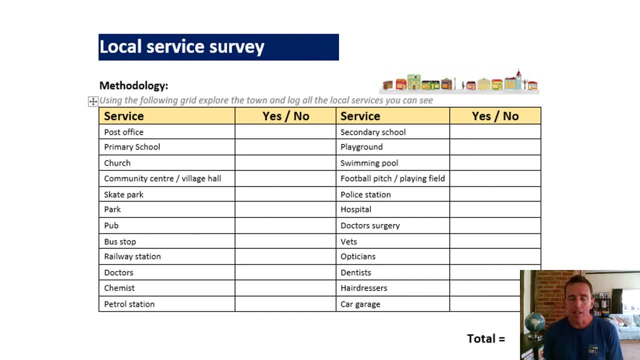 You may choose to do a local service survey, in addition to perhaps doing a shop survey. What services are there for local people in Southwold? and again, this you might be able to do just using Google Street View and Google Earth and looking at how many of these things that you'd expect the town to normally have does Southwold actually have, and you could then perhaps do a comparison with other towns locally or look at ones local to you. 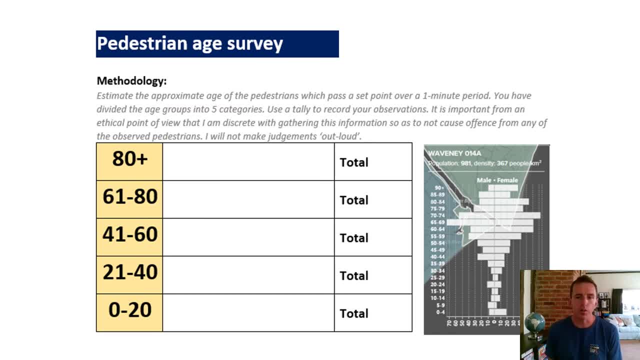 Pedestrian age survey. this is a useful thing to do if you're trying to prove the identity of the place. There's a number of limitations to it, but we know that that population pyramid there represents the local Residents who are here permanently. how much does the actual daily population of the High Street represent the fixed population of the residents here? 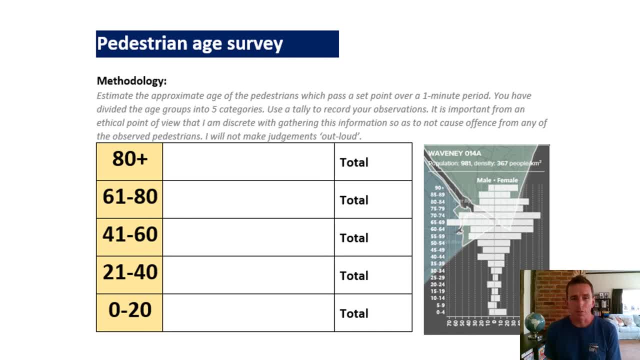 So you could actually, if you're doing a study based on who is Southwold for, consider that this may be a useful thing. or you know, as I say who, what is the identity of Southwold currently? So an age survey is where, essentially, you'd need to find yourself a discreet spot- not too discreet that you look like a stalker, but perhaps 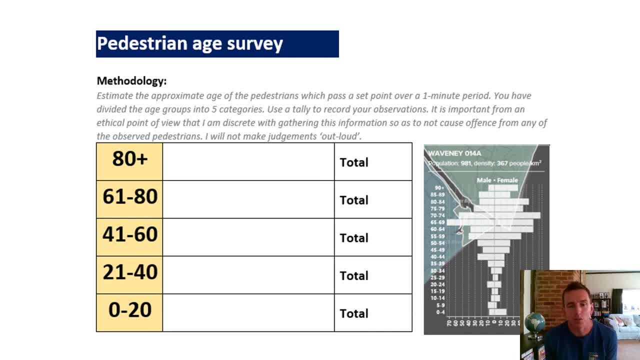 A nice spot on a bench- often good if you can sit down and do your survey- A spot on a bench where you've perhaps got it on your phone or you may have it on a clipboard and you perhaps create categories like this and you're simply over maybe a five minute period, but it'd be up to you recording the number of people that would fit into those categories. 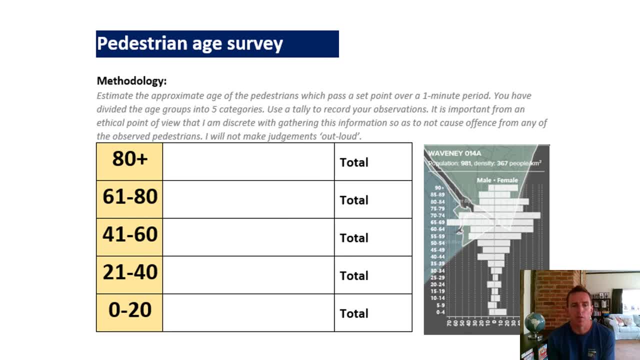 Now, the reason that we've chosen to do those categories- and we use this sometimes for our GCSE students- is because age distinguishment can sometimes be quite tricky, especially when you're doing a survey, When you get kind of middle age and above. 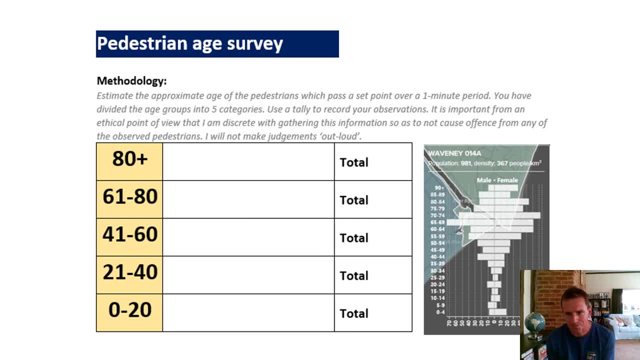 So you know, when people get into their mid thirties, sometimes quite difficult to make an accurate guess of their age. So rather than actually ethically going up to them and asking them how old are you, You would do this method of making an estimate using an appropriate scale like this: 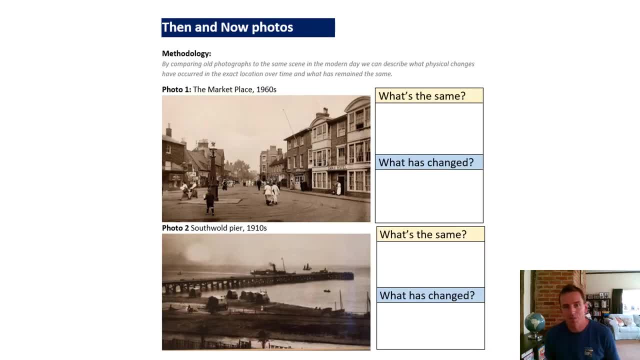 Okay, Very easy, nice method to do And again, you can prepare this before you come. But if you go on to South Oldham Sun, you'll see a huge archive of old photos for every single street, But equally probably if you just type into Google you'll find archives of lots of the streets. 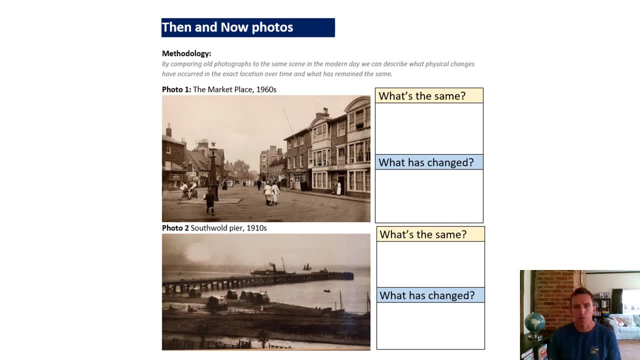 And pick any kind of photos. This photo here is of the marketplace. You've also got one of the pier too. There'll be lots of the lighthouse, lots of the high street, lots of the adnams and lots of the seafront. 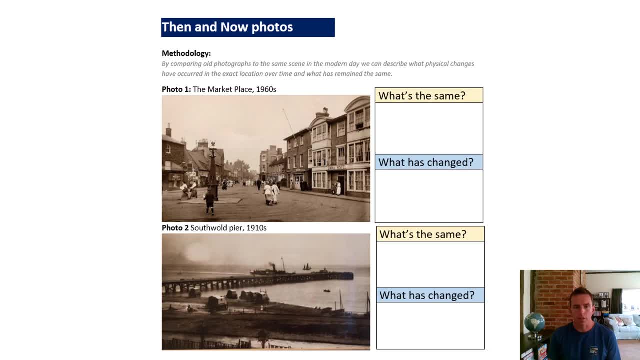 Historical photos- And this would work also for a physical or a human method study- Gather maybe three or four historical photos And then, when you're in Southwell, try to find where those photos were taken and kind of repeat the photo, but from 2020.. 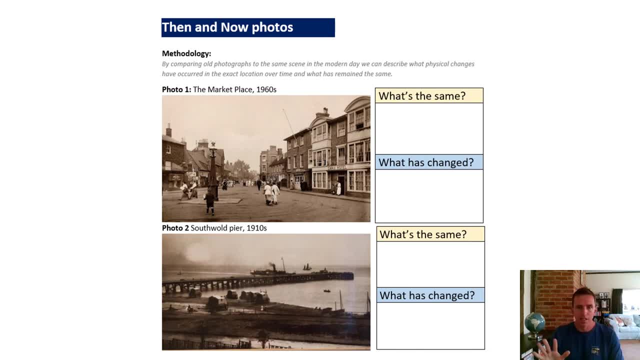 You could then present both photos side by side and simply annotate them with. what's the same, what's changed, What change is obvious in these two contrasting photos. Really straightforward things to do, But really really easy, Relevant And, you know, absolutely just form of data presentation and data collection. 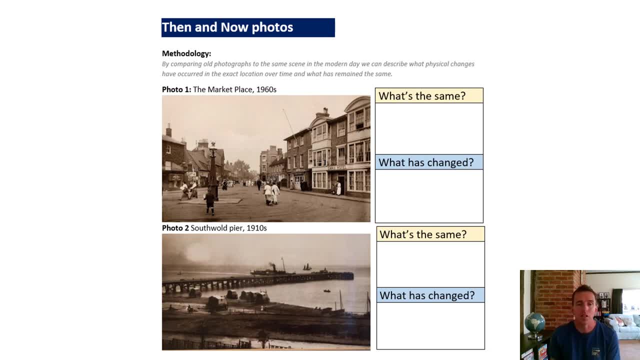 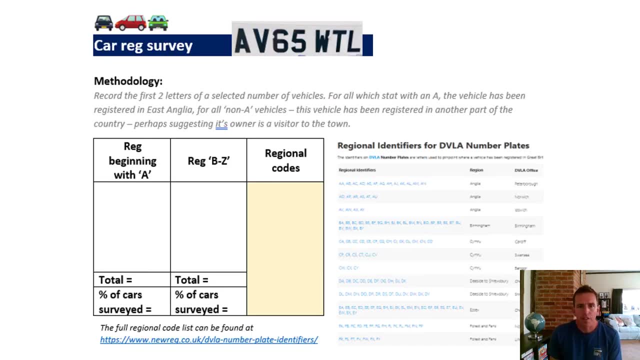 So I would suggest that that might be something that all of you can do, if your study is linked to this idea of change at all. Okay, A couple of things that you can do with cars, particularly if you're doing gentrification or if your tarp is four, or you know the kind of the idea about second homeowners in the town. 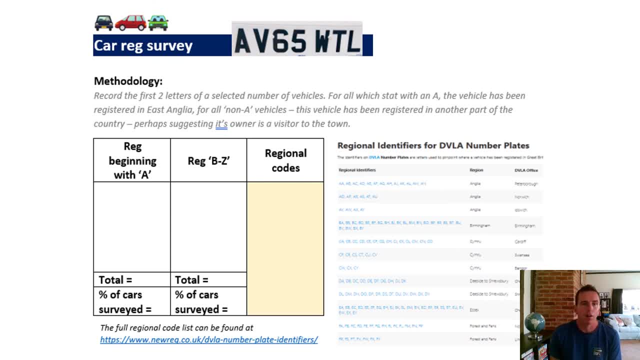 One of the things that you may or may not be aware about Car registration Plates is that the first letter of the registration plate represents where that vehicle has been registered, And any vehicles beginning of the letter A have been registered in the East Anglian region. 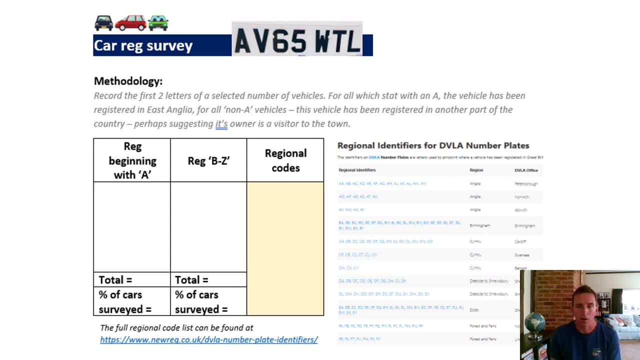 So Norfolk and parts of Essex as well. So if you spot a vehicle in Southwell with an A registration plate, chances are that that vehicle belongs to somebody who lives relatively locally. Anything with the registration B to Z, More chance that it belongs to somebody who is from further afield. 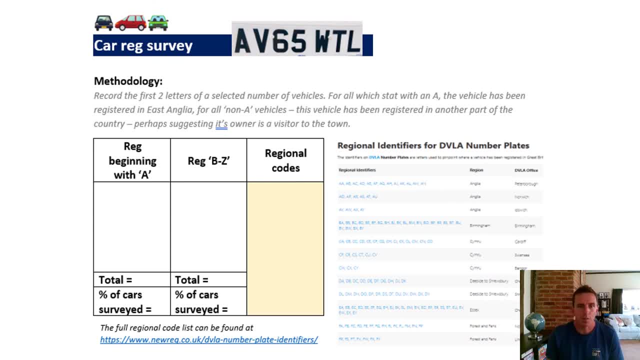 Now that gets less reliable the older the car is, because there's more chance that the car might have moved on to somebody else and now is no longer owned by the person that registered it. So sometimes people choose to do this by actually just hoarding cars that are maybe only two years old. 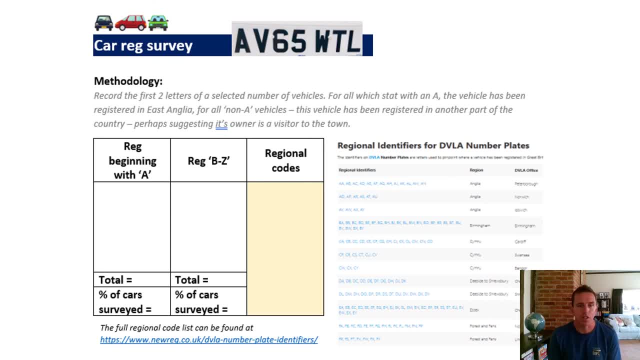 And again, you can find the age of the cars by looking at their registration plate. You may choose to survey, for instance, 50 vehicles at random And work on that And work out the proportion of those vehicles that are local and a proportion that are further afield, to again get an indication as to who it is that is in Southwell and who it's for. 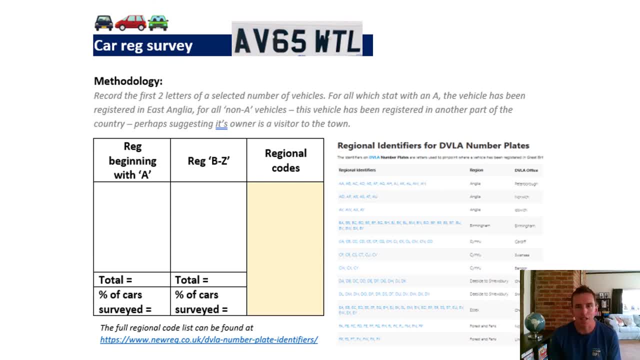 The DVLA, the kind of national licensing agency, has a huge list of these different numbers And you can simply just type into Google DVLA regional lists and you'll get the screen that I've got there with all of those different codes And it will tell you where those people have come from. 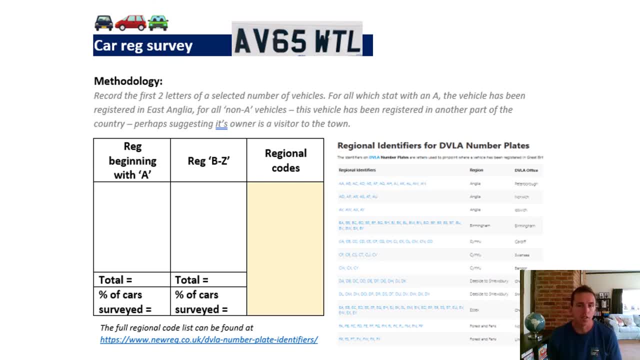 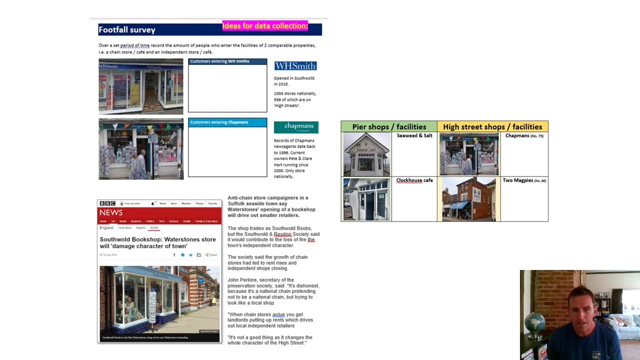 So you may then ultimately choose to present this on a Coropath map To show the sphere of influence of Southwell and where people are coming from to be in the town. Footfall survey is kind of essentially an elaboration on a pedestrian count or maybe even an age survey. 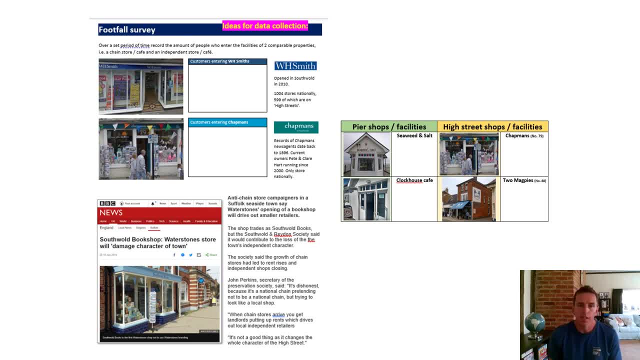 There's a number of things you can do in terms of, you know, recording and measuring people and their characteristics, other than just counting them. So footfall surveys may be useful if you're doing a study that then lends itself to looking at the impact that second home vehicles have. 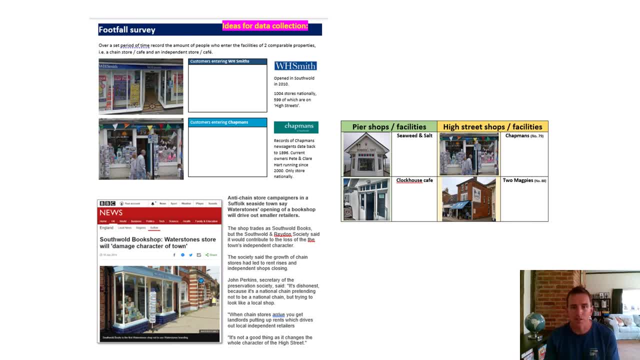 To looking at the impact that second home ownership is having on independent stores, Because there are a number of independent stores that have an equivalent chain store on Southwell's High Street, So by that I mean there's a. you know, there's a shop called Chapman's on Southwell's High Street that has been there for over 100 years. 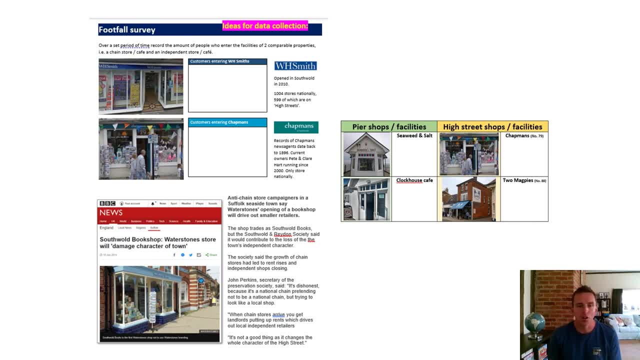 It's owned by a couple called Pete and Claire- I used to teach their son Josh- And they've run this news agency. essentially They sell cards and magazines and newspapers and drinks and things Right in the middle of Southwell's High Street. 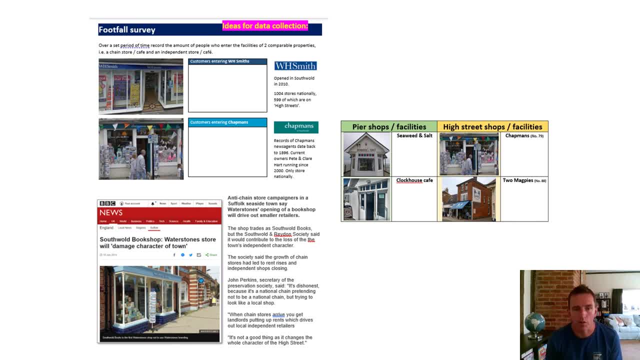 They've run it for years. They've been, you know, in the family for a long time as well. It's the only one in the country. Ten years ago, almost opposite them, WH Smiths arrived and started selling exactly the same things. 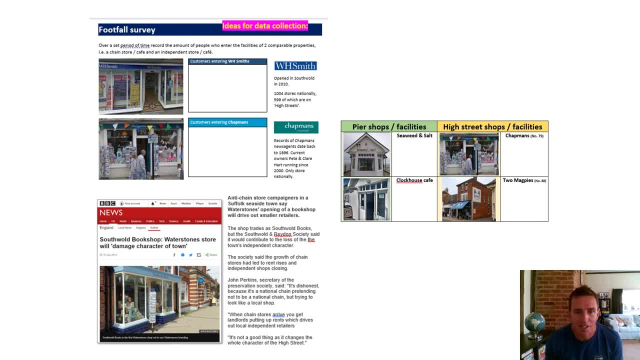 You know a much bigger brand of over 600 stores on UK High Street, Over 1,000 stores and things like train stations and airports and stuff like that up and down the country. It's a much bigger brand And because it's a more reputable brand, sometimes people are inclined to go and shop there because they know what they're getting. 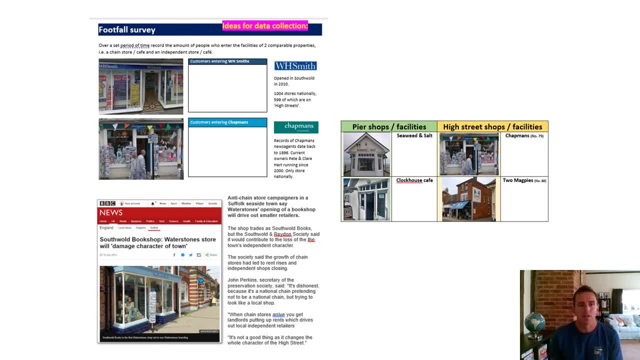 And perhaps not so much. They're more inclined to support the independent store because they're perhaps less familiar with what they would expect to get in that store. So you could perhaps look at the impact that this increasing amount of kind of chains on Southwell's High Street are having on the independent stores by looking at physically. is there a difference between the amount of footfall in to those shops? 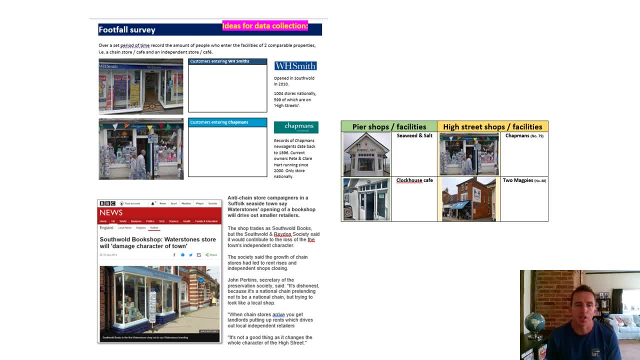 So potentially you could again discreetly locate yourself maybe five minutes or so outside Chapman's, at a sensible distance, and outside WH Smiths And literally tally the amount of people that are going into those shops. Is there a significant difference? They're essentially telling the same things. 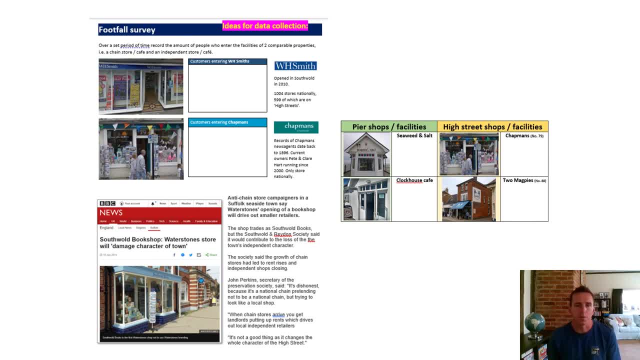 Is the High Street store that is the national chain WH Smiths, you know, taking away a significant amount of trade from Chapman's. Another thing that is kind of quite unique in Southwell is that you know a number of these national chains arrive in Southwell and recognize that there are a number of people that will shop in independent stores only. 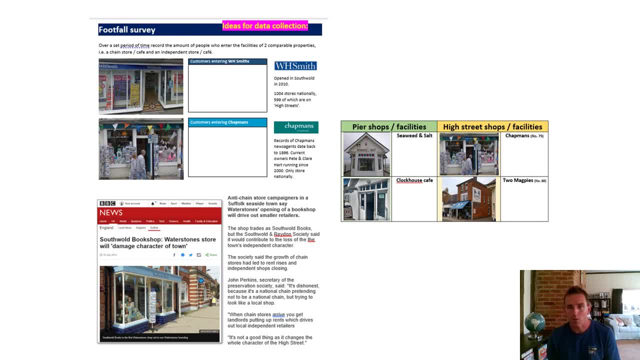 Because they want to keep up Right, They want to keep them going and they want to support them. A few years ago, Southwell had a Waterstones that arrived on the High Street, But discreetly- not discreetly, probably more nastily- manipulatively- Waterstones changed their shop front and changed their entire branding to make the shop look like an independent store. 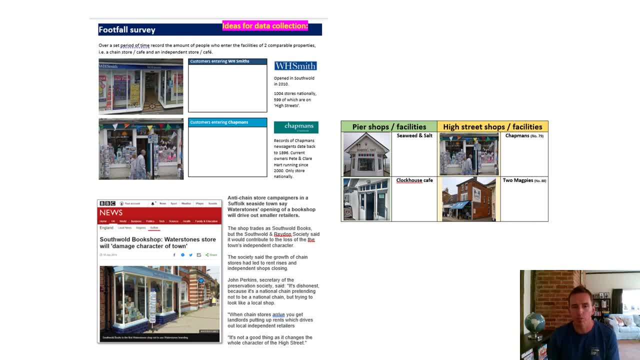 So the store is called Southwell Books and it stands loud and proud still on Southwell's High Street And it looked like a nice independent store. When you go in there and you go to the till and buy something, you are asked if you have got your Waterstones card and you get a Waterstones receipt and a Waterstones bag. 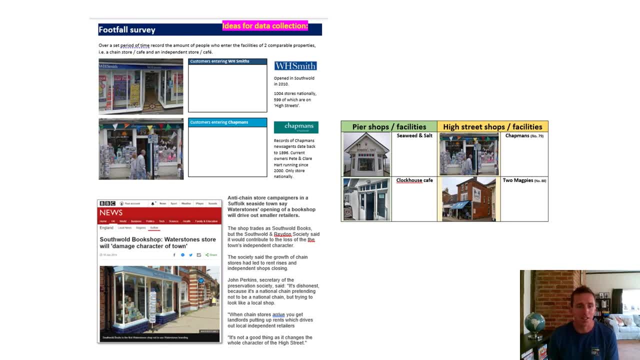 And you can kind of come out of that shop, having bought a book, feeling like you've actually just been done and you've had the wool pulled over your eyes, Because it is a Waterstones shop in every single sense of the word, apart from the fact that it's got the words Southwell Books on the front of the store. 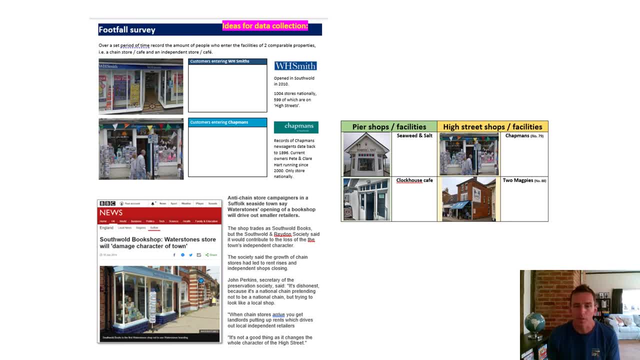 People are aware, Businesses are aware- There are a number of people that are aware of this issue- that independent stores are threatened, And sometimes the High Street stores use that to their advantage by dressing themselves up in wool clothing. I don't know if that's the right analogy, but there we go. 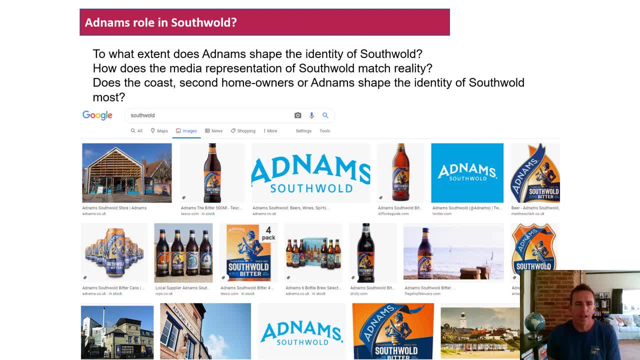 Okay, A number of you may be interested in the brewery and the role that Adam's Brewery plays in Southwell. It is, as I said before, an absolutely fundamental key player in Southwell, And without Southwell I think it would be a – sorry, without Adam's Southwell would be a very different place. 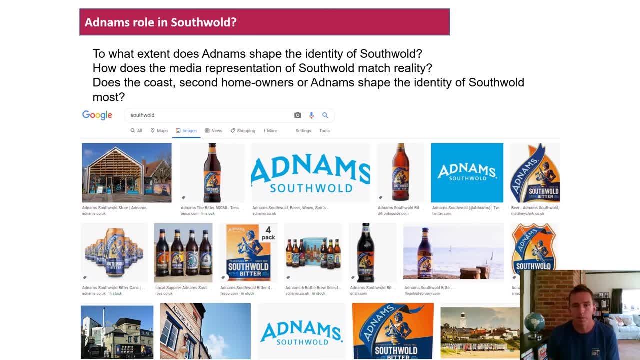 And I think both of them really need each other. But you wonder whether actually Southwell needs Adam's more than Adam's needs Southwell. The brewery has been in the heart of the town for over 100 years. It owns some of the key properties in town: the main hotels, the main pubs, the biggest shop in the town. 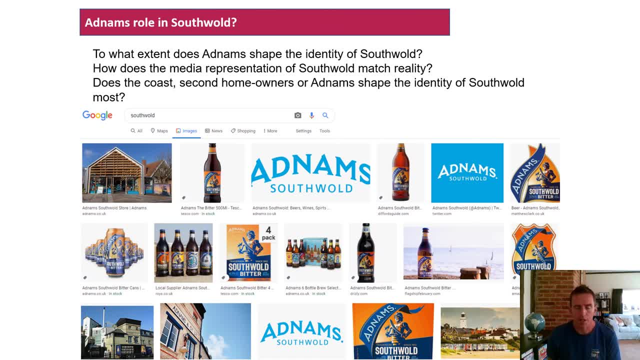 It's the biggest employer, It's the biggest inn, It's the biggest influencer. Southwell used to have a tourist board, a tourist office, on a tight street up until about seven or eight years ago. They now no longer need it. 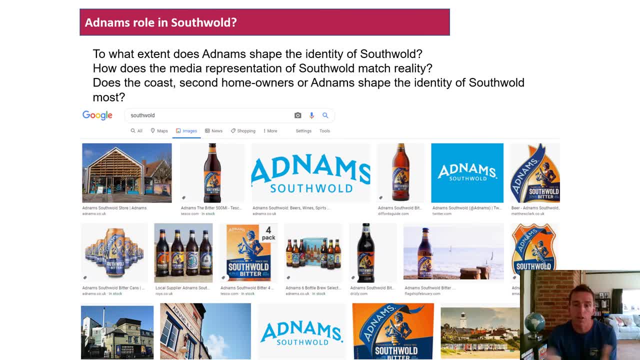 They closed it because Adam's does so much marketing for the town. Its logo has even got the word Southwell underneath it. They sponsor national events, They have a huge social media following And they create this brand of Southwell And people, when they come to Southwell, often want to go and sample the local beer in the local place that it's brewed. 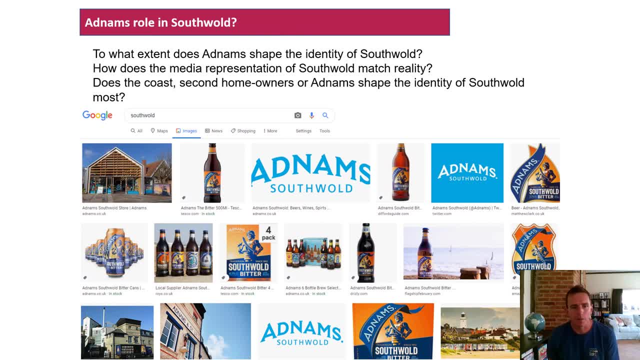 like kind of a Guinness in Dublin. They go on Adam's tours And they end up at those tours at Adam's flagship for where they can buy all sorts of things. So it has a huge role in shaping the economic prosperity and the economic future of Southwell. 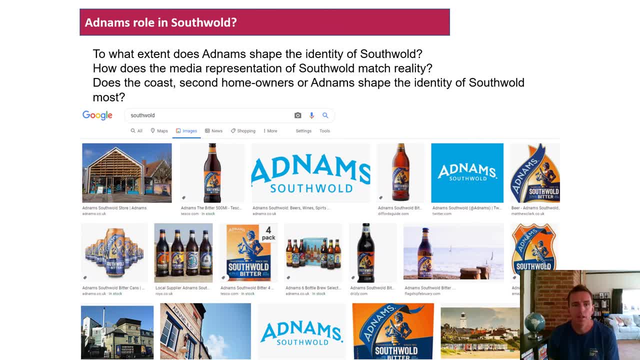 But it has a huge role in shaping the identity of it as well. It oversaw Southwell's biggest regeneration project, which I spoke about. when you have the tour, the virtual tour, It also has this relationship in terms of the media. It also has this relationship in terms of the media representation of Southwell. 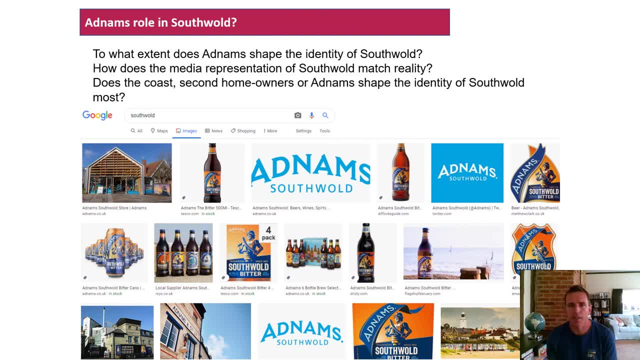 How does the media representation of Southwell, which is promoted by Adam's, actually map to reality? So if you're more of a media student, there is this kind of focus that you could look at as well, which is quite a nice idea. 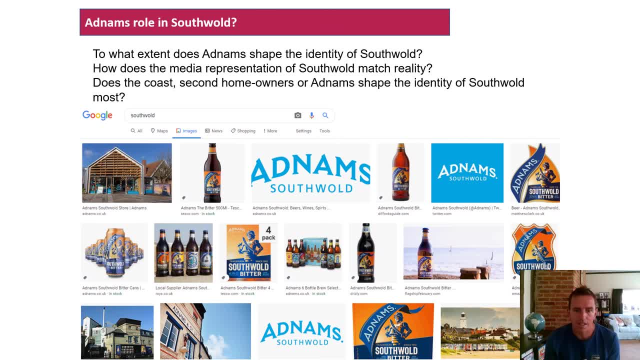 Perhaps looking at collecting information from media sources initially, before you come in, and actually collecting information in the field in Southwell, How much is the kind of the, How much is the kind of the identity which is created online by Adam's actually a true representation of what this space is like? 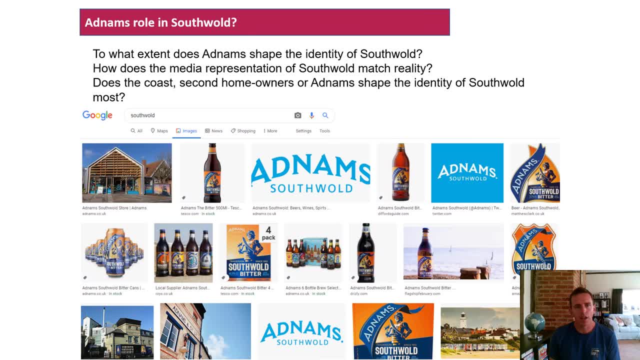 And then the other idea there: does the co-second homeowners, or Adam's, shape the identity of Southwell Motor? Who are the biggest players, And which of those is actually the one with the most significant role in terms of shaping Southwell's identity? 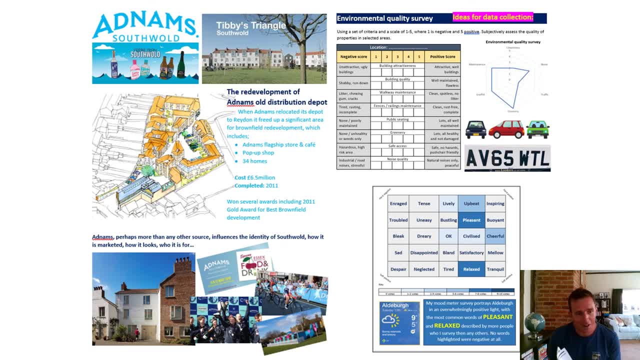 In your booklet you've got this information. I recognise that I've already talked for an hour and a half. This is a colossal Introductory video And you'll do well if you watch it all, But hopefully there'll be bits that are relevant and useful to you. 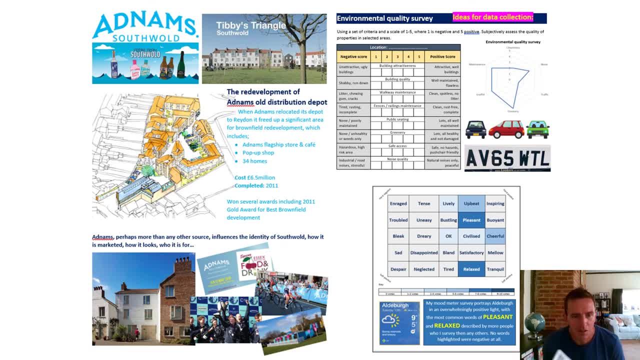 This bit that is in the booklet about Adam's is on your screen now. Have a look at that. So I've talked about this a bit more in the virtual tour. The Tibbys Triangle, part of Southwell, is an area of regeneration. 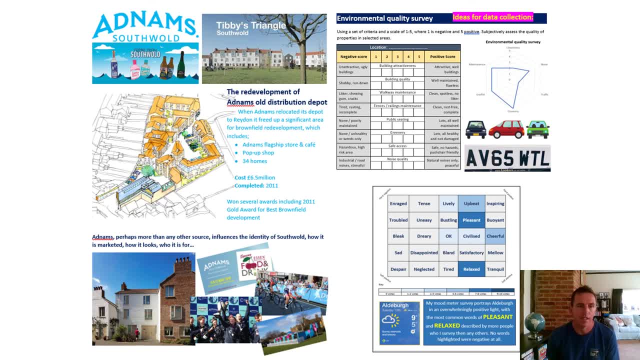 It's essentially Southwell's brownfield redevelopment site. It's now very nice, very successful In a certain point of view. It's not necessarily successful in terms of benefiting the locals, but it looks much better, much improved, And some of you may choose to focus on its regeneration project as part of looking at Southwell's overall role in Southwell. 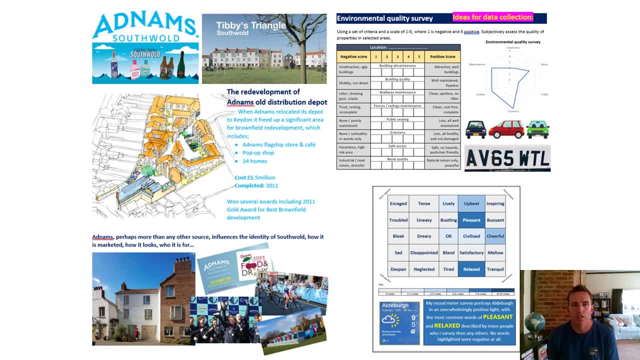 Or you might just look at it in terms of the regeneration success within this area. Kind of six and a half million pounds was spent renovating this place, turning an old industrial site of lots of warehouses and funerals And functional buildings for Southwell's brewery into what is now a large modern housing development, but really kind of cool coastal properties rather than, you know, just your box standard housing. 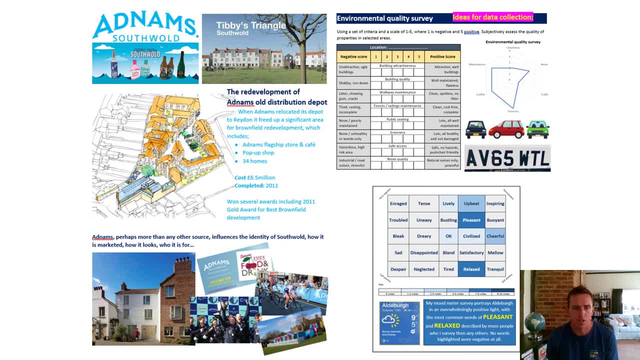 Thirty four properties were made as a pop up store as well, which is currently home to a nice quirky kind of stationary shop which teachers may enjoy this thing, And there's also a really nice cafe and the big kind of homeware store as well. 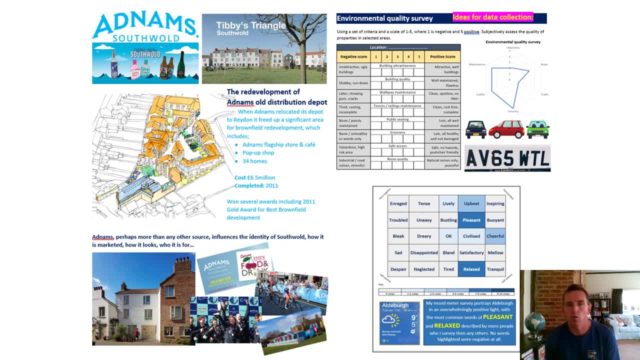 Plus, Adam's is main. Yeah, Yeah Right, vermeiglolis, Great place, in quite a really kind of stale outlook, for all of their beers and their wines and their spirits. On this screen I'm just going to flag up the mood meter down the bottom here. 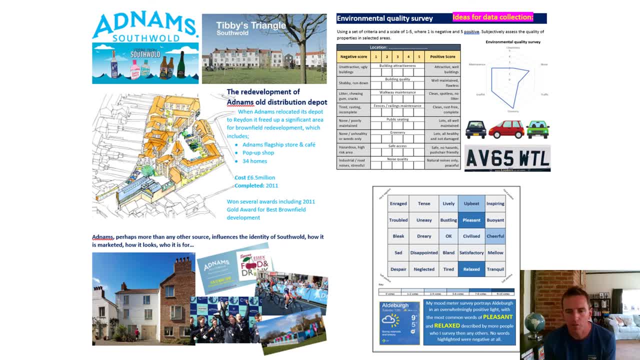 The mood meter is this piece next to my head, but that way, This way, there it is A mood meter again. if you look on Dog Gottes das Verden, There'll be an explanation of mood meters. It's the idea of trying to accept the kind of that. 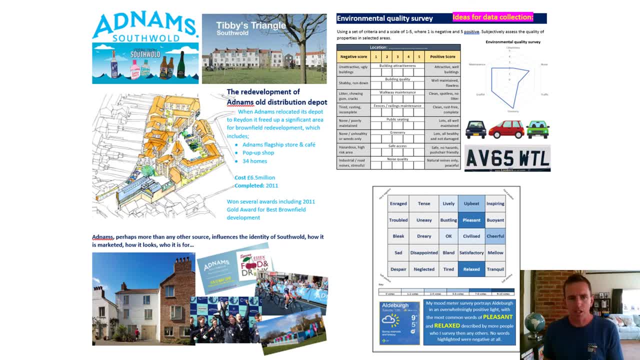 and where you have regeneration. not only do they physically want to change the appearance of the place, but they want to make sure that the atmosphere created in that regeneration project is positive and it's pleasant and it's, you know, suitable for people to want to call that place. 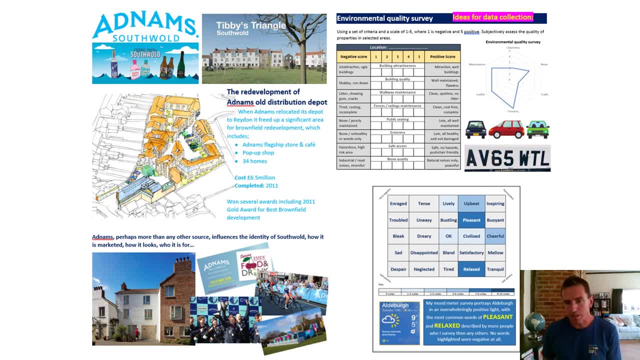 their home and the atmosphere within tibby's green, i often think, is very relaxed, very mellow and chilled out, and so it may well be that doing a mood meter is something that you consider it's a nice form of qualitative data collection. you can also do, perhaps, the mood meter on the pier. 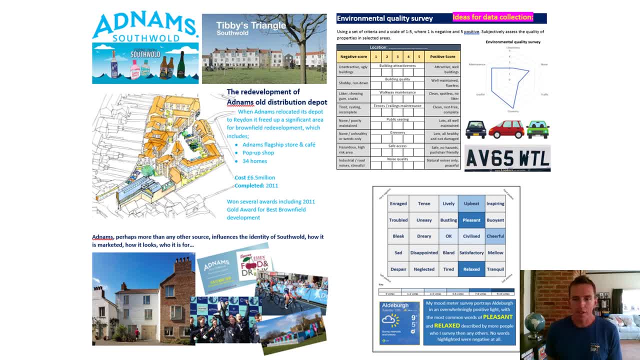 on the high street, maybe on the sea fronts. obviously it's weather dependent. so if you're doing a mood meter, that's going to be influenced by the conditions on the day, which are external factors. but it doesn't mean you shouldn't do it and it just might mean that there's limitations. 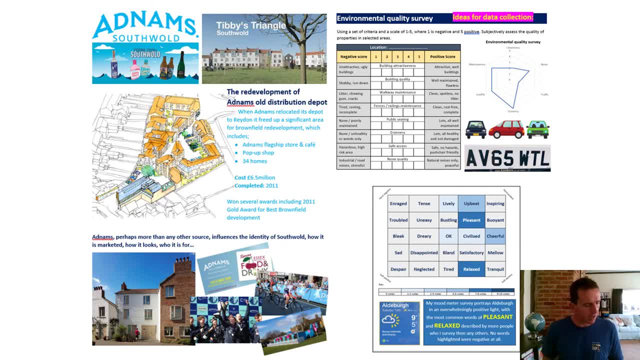 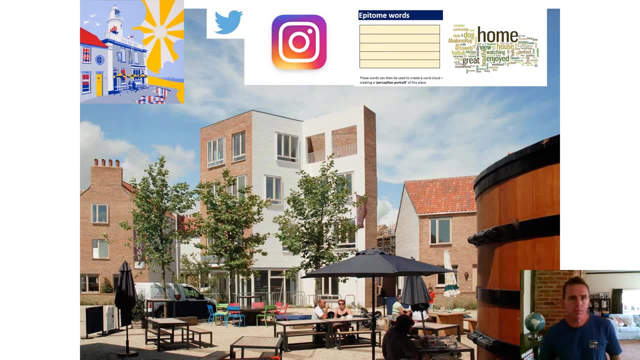 to reliability of your method when you did it. so have a look at mood meters on jogit to see how you go about completing it and whether it might be relevant to your study amount. there's just some nice pictures of tibby cream. the instagram and the twitter um logos there. 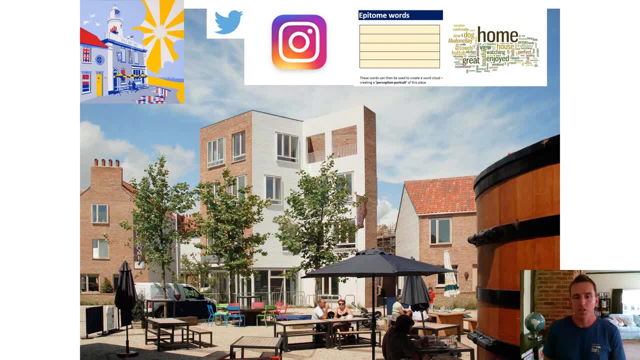 have reminded me that actually one of the things that you could do is you could do a method of data collection using um social media sources. you could eventually look at um posts about south world. how many posts about south world have actually also got the hashtags adnams in them? 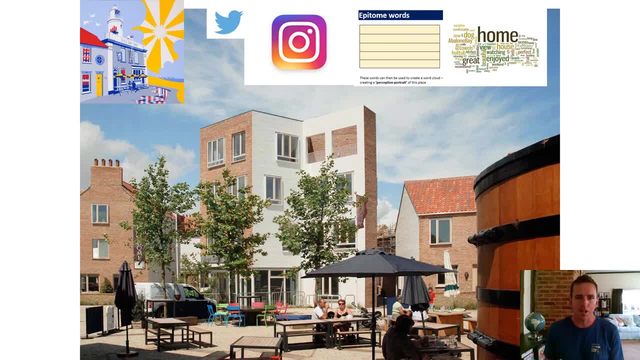 i imagine there's a significant proportion of pictures and posts that are relevant to south world from holiday makers that actually in some way are connected to adnams, whether it's actually somebody literally holding a beer or being on the adnams tour or being in one of the adnams hotels. i reckon there's a 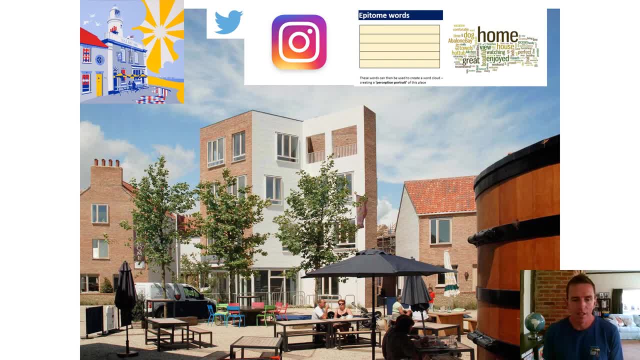 significant proportion of houses- oh, sorry, posts about south world that are linked to adnams, so you might try and work that out. one of the other things that you could do is create one of these word clouds that you can see above my head there in the top right hand side of the screen. 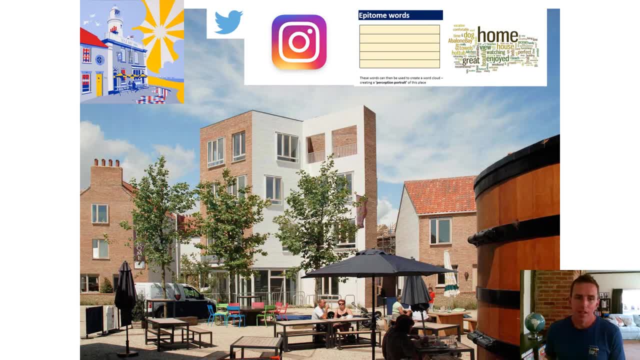 and a word cloud is where you represent the kind of descriptive words that people are saying about a place. so again, perhaps, using instagram and twitter as your source of information, you could extract from those posts anything that is descriptive about south world, so any descriptive words. you could create a list of those and then put them into the website. 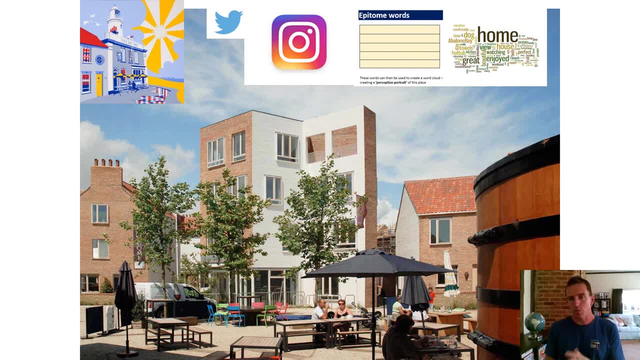 called word art dot com and they then create these word clouds for you. you can fiddle around in the settings to make the- uh, the actual cloud shape a relevant image to south, or so you could do the cloud kind of in the shape of a seagull, for instance, or a boat, or a pier or a lighthouse. 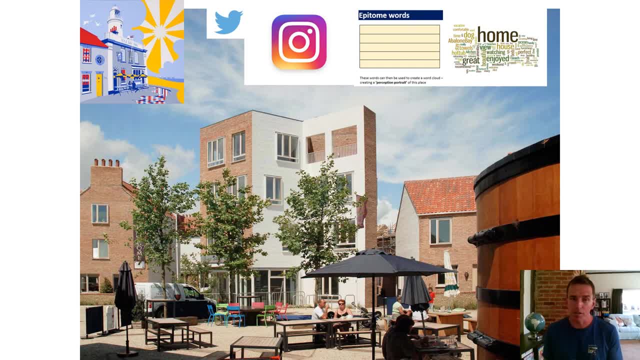 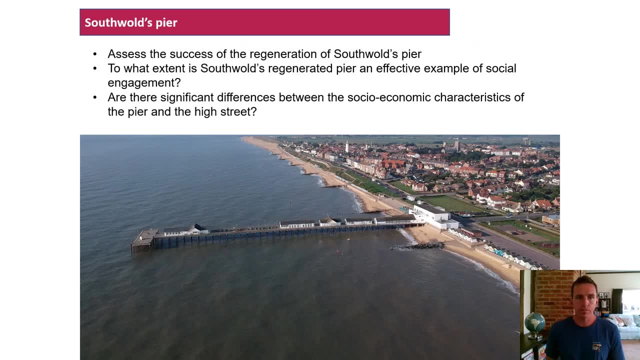 so have a look at that website: word art. think about how you might use social media to create one of these word clouds. again, it's a good form of qualitative data presentation. all right, so we're kind of heading towards coastal geography a little bit more, um, but before we get there, the pier is a kind of a mixture between coastal and human geography. it's. 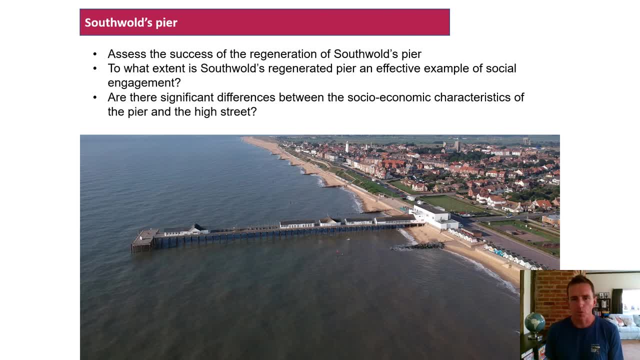 a really, really good example of successful regeneration. the pier and um in a fairly twisted way as well. um southport pier is independently owned. it's one of the few piers nationally that's owned by a private family and they've overseen the renovation of it and had 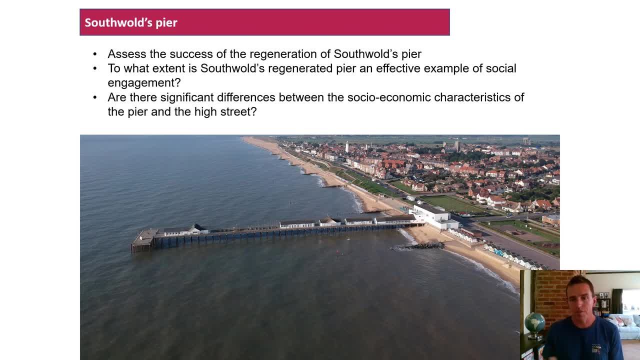 unique ways in which they've done it. so some students choose to focus their studies on the pier, because the pier is nice and compact and there's lots of information on it that is um applicable and to suitable for field work. so some students look at the success simply of south wold's. 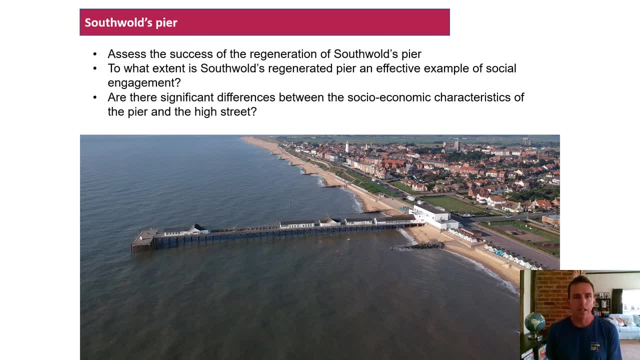 pier and the success of the regeneration of it. they look at whether the regenerated pier is an effective example of social engagement- i'll talk about that in a second- and they look perhaps either, whether there are social economic characteristic differences between the pier and the high street. so is there a difference between the economic success of the buildings? 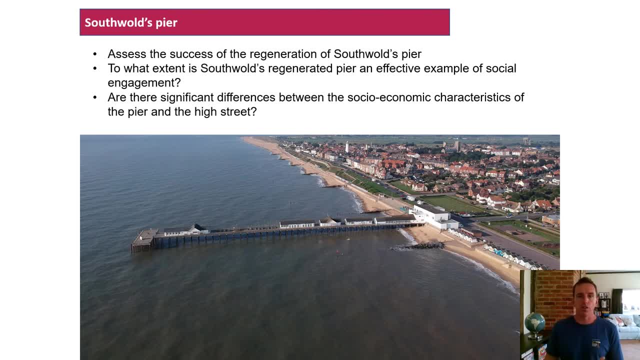 the cafes on the pier. as a footfall in the pier, in contrast to the high street, are less people going in and out of those properties in in comparison to the high street? um is there a different age um bracket to people that are on the pier in comparison to high street? so you could do a comparative study looking at the differences. 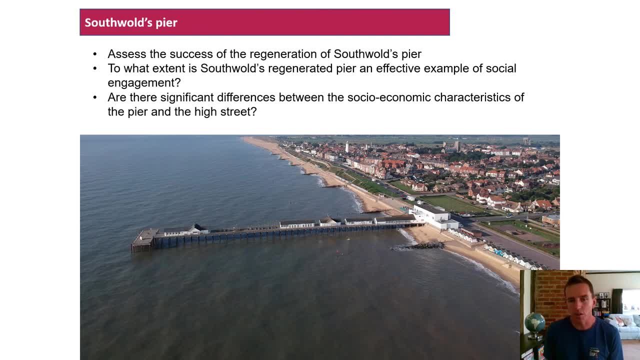 between, yeah, and the high street. either way, the pier is a really good place to investigate one um, the one thing that is perhaps worth noting is that occasionally, maybe six or seven times a year, if there's high winds and stormy seas, pier is shut. that would be a disaster if you had your study completely based around the pier and unfortunately, 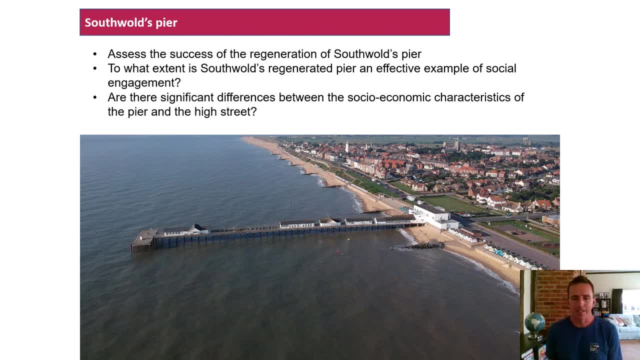 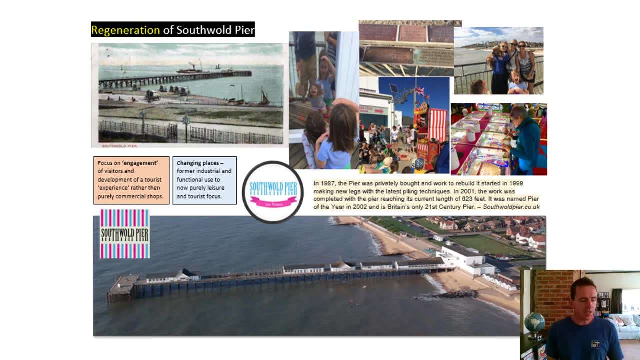 on the day that you came it was really wild weather and the pier was shut. then we'd quickly need to think of a plan b. that shouldn't indicate be really bad. so in your book that you've got some information about here, again, read through this. it'll give you an introduction to it if you're. 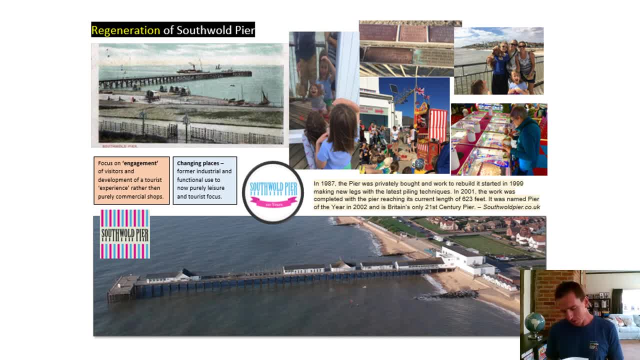 interested in doing, uh, some work on the pier. i'm sure this is in here. there is, um, some work on the pier and some work on the south pole pier and some work on the south pole pier, and then there's lots on the south pole pier website about the history of it. but, uh, what's good about here is that when 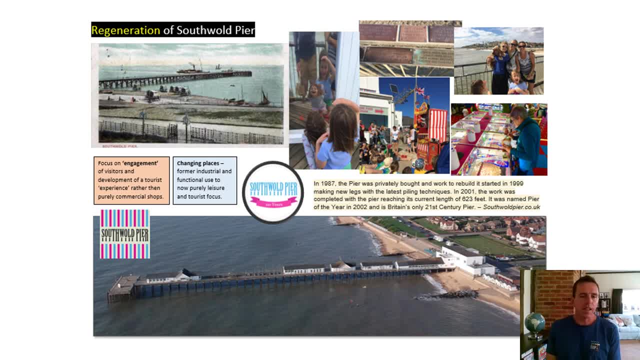 it has been regenerated. it's been regenerated with a plan and a vision, and the vision for this pier was that they didn't want it just to be a classic here with slot regimes and ice creams and has all those things. but it's got other things too, and the vision was to actually make it a. 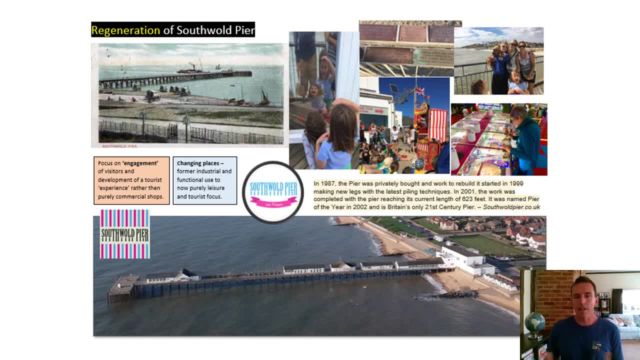 nostalgic, quintessential experience that people went there and they engaged within the pier, rather than just going there for their chips and then going somewhere else and to fund the regeneration of the pier. one of the things they've done quite uniquely and very successfully is they have used 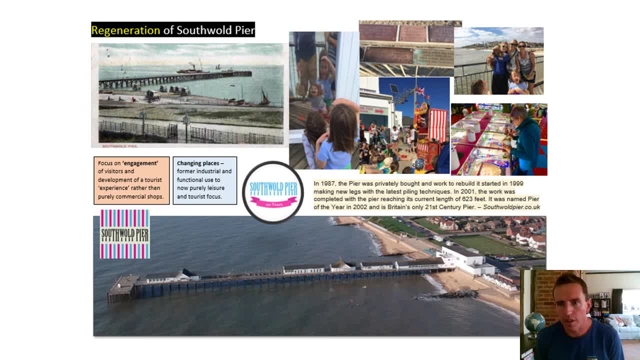 the railings that go all the way around. you can see there's a picture top right there of a group of ladies and stood on the pier. behind them is a metal fence, and that's the fence that separates the three parts of the pier, which is a space that is actually a big square um layer. there there are. 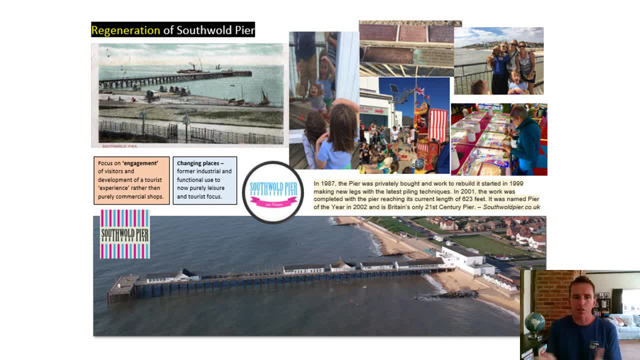 plaques that are mounted against the railings and actually now on most of the parts that here there are three layers of plaques and these plaques are all inscribed and all unique and they are independently um unique to the people that have paid for them. so you can pay to have one of these. 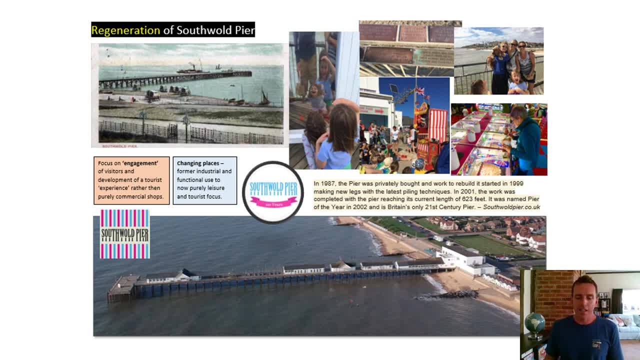 facts. you have a small one, it's 300 pounds. i think a big one is almost about 500 pounds, maybe a bit more, uh, and these plaques are individual, sometimes memorials of people's people that are on the pier might have died and used to come to south wolding up here. 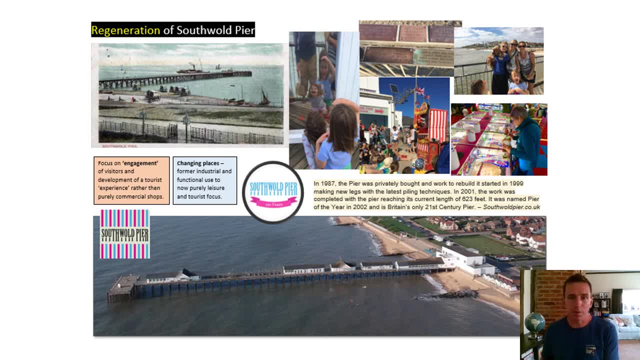 sometimes they're testimonials. sometimes schools have actually put like a year group levers on there, and there are some from businesses. there are lots of very personal messages. there's even some kind of proposals that you'll see as you go around. but one of the things that these things do is they engage you, they draw you into. 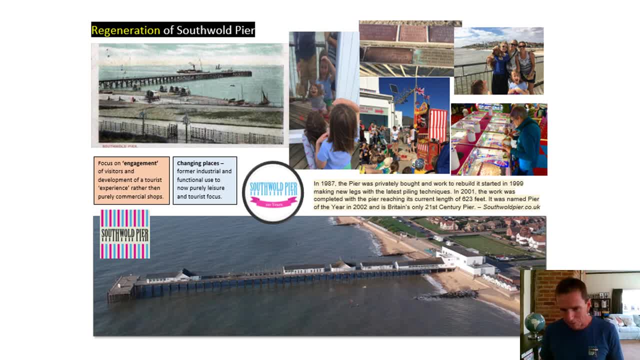 reading several of them and many of them, and you see people walking around their peer. the peer heads down reading these plaques. um, cleverly though those, those plaques are paid for much of the regeneration of the pier. a huge amount of money has come from these plaques being installed on the pier. 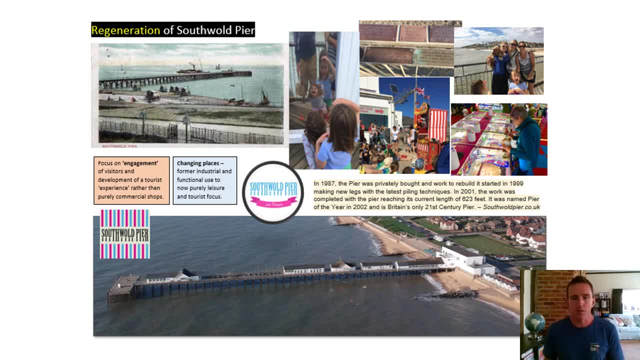 and they've enabled the redevelopment to continue um since the year 2000 and 1999, when the pier was reopened um. it now has cafes. it's got um a really cool building called the under the pier show, and in the under the pier show there are um. 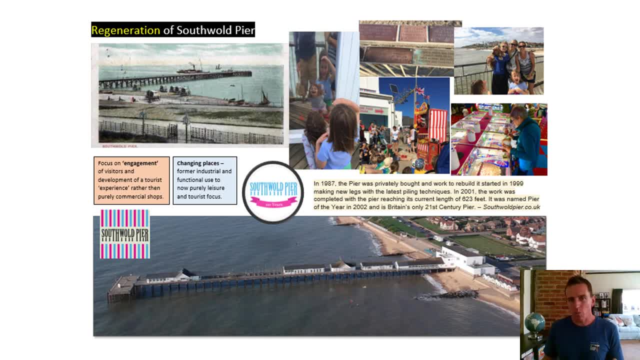 really alternative forms of arcade games. there's one where you can walk a dog on a treadmill, where you can- uh, yeah, there's all sorts of things you can shoot at, some of bin laden's and all that. so there's all sorts of random games that you can play in the under the pier. 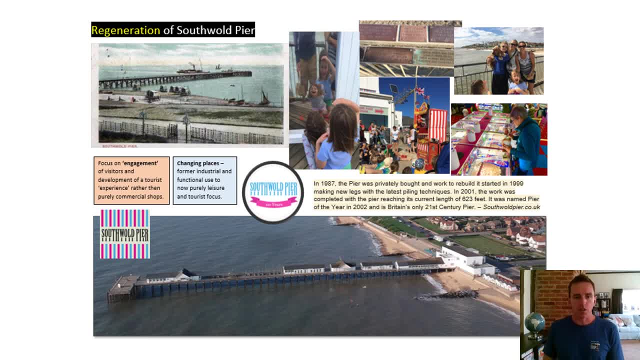 show. there is, um, you know, some nice cafes and restaurants too. there's a wall of wavy mirrors. there is the classic kind of picture where you can put your head through that says we've been to south wold here and you can all line up. line up and your body is represented by some kind of weird clown. 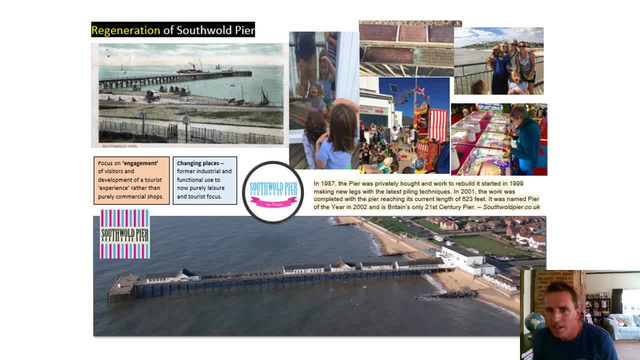 um, there's a water clock and the water clock on every quarter of an hour reduces this kind of random show. it's, the water clock has all these different kind of metal features on it and part of the the artwork of this water clock is it is two men. 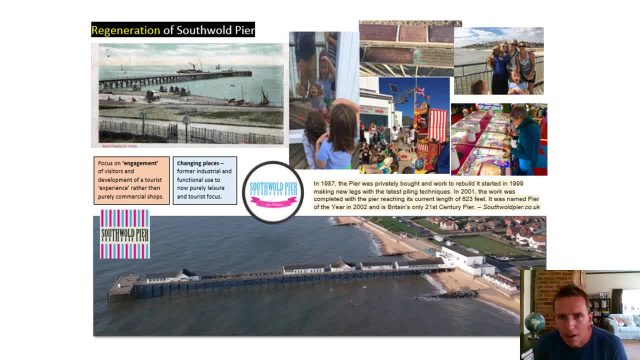 two metal men uh in a bath and every 15 minutes they stand up, they pull down their trunk to their wearing and they wee on over the edge of the bath and then these kind of roses grow up. it's very bizarre, um, but people of all ages love the water and I can't believe. 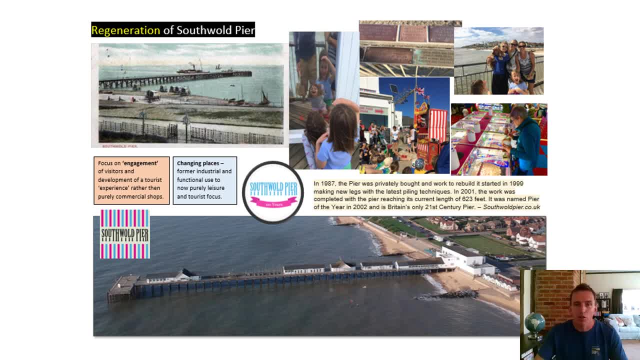 that's all that you've seen in this show it and they wait around in groups to watch it. you can see people waiting around in groups to watch the punch and judy show there. so the pier, the regeneration of it, has been geared around this idea about engagement and i know that's one of the issues that has covered this kind of idea of 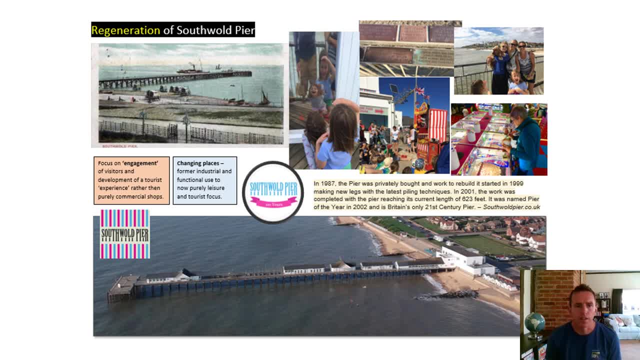 social engagement, uh, in human a-level geography. so you could look into whether you know to what extent, assessing the extent to which social engagement has contributed to the effectiveness of the regeneration sample. yeah, so lots of people choose to look at the pier because it is a really good, unique example of it. also, on a wider scale, there are 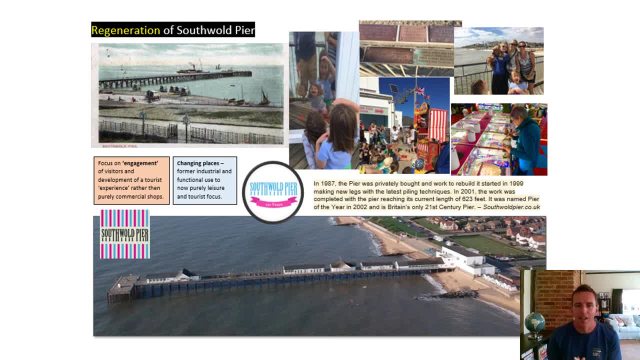 websites that rank peers and nationally, as i say there's, there's a, an award called the peer of the year and on that website it actually kind of has a criteria for what makes a successful beer. so you could use that perhaps to drive your study in the introduction. 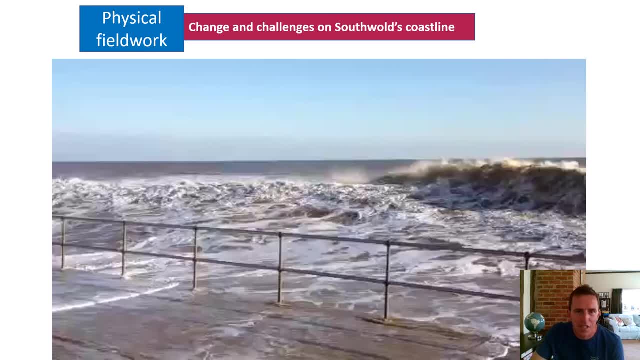 oh, okay, we're getting there. so, in terms of the physical geography along south wales seafront generally, you might look at south wales sea in the picture on the page that i had before, where, um, the sea looks quite benign, quite calm, and you might think, well, there can't be a huge. 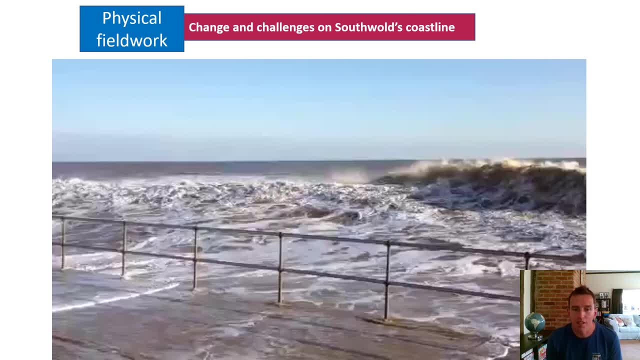 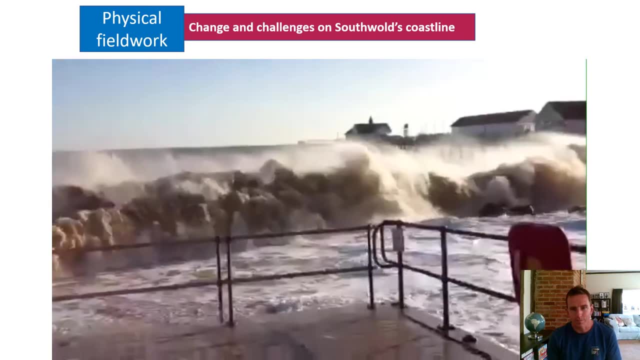 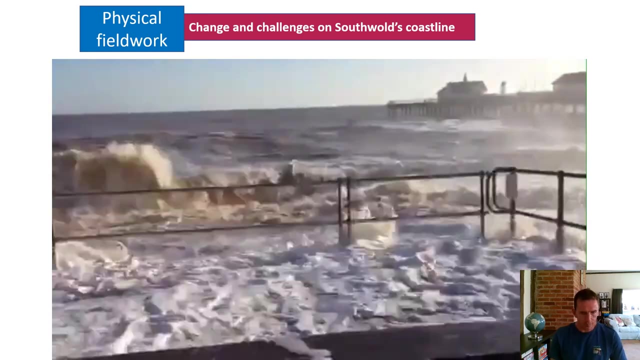 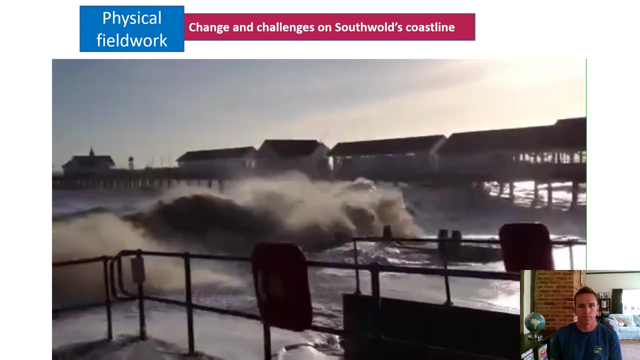 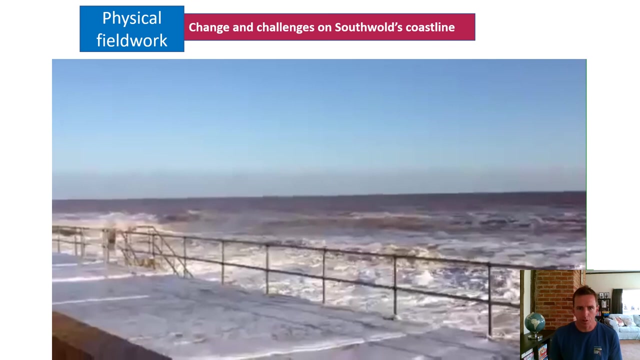 amount of erosion going on here and a huge amount of action, and on most days you'd probably be right there isn't, but on some days the sea can look like this: okay, pretty dramatic. so on a day like that, you can see that the sea has got the potential to be very 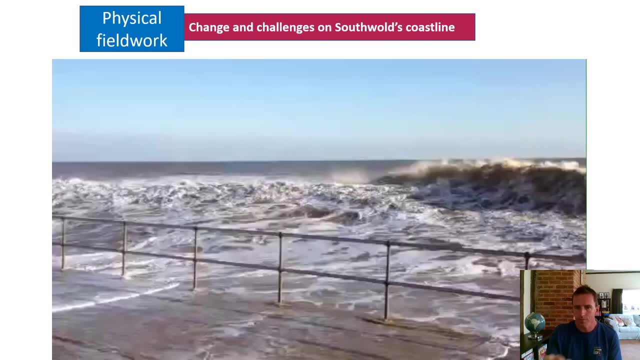 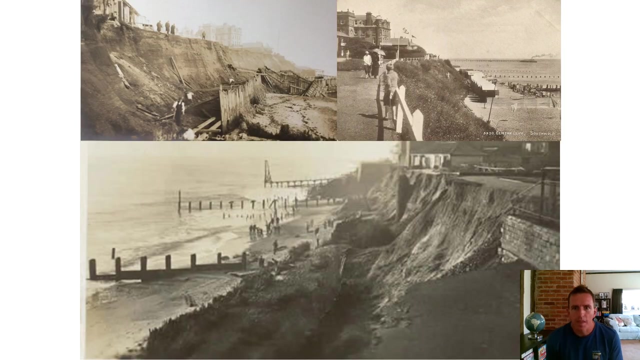 destructive banana. okay, so south wold is a place where often you turn up a nine times out of ten. the sea looks very sleepy, very calm and pretty mellow. but if you've been to the seafront for years you know some of this season has got the power of глубbing. the shall mean, if you have ever gone out in Careful that, if you have gone out there and you can just go straight up the seafront and you can see some pretty big water sands there, you can see the daylight up there, you can see the Undertaker right here, southern sea, nice TOADS and sandburnish waters around it too. that's good. 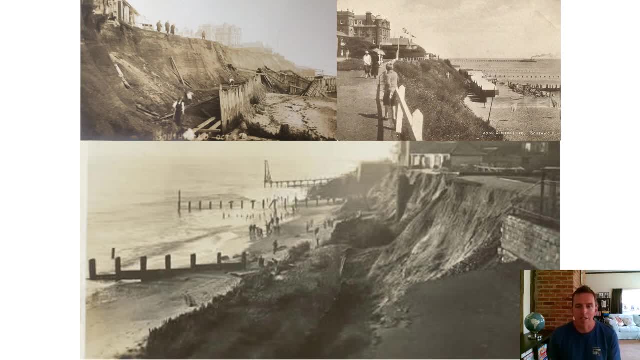 that is vulnerable primarily because of the geology of which the town sits on. so the cliffs that south wold stands on are made simply of sandstone and clay, and neither of those give any real resistance to total erosion. um, historically, then, the biggest storms, and we do- 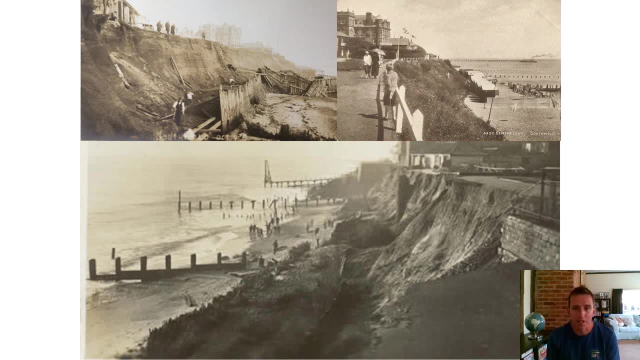 get the occasional big north easterly that brings big storms to south wold. occasionally get storm surges as well. those storms historically down years, have caused great damage and, of course, significant amounts of erosion to happen over the space of 24 hours when you get the sea really. 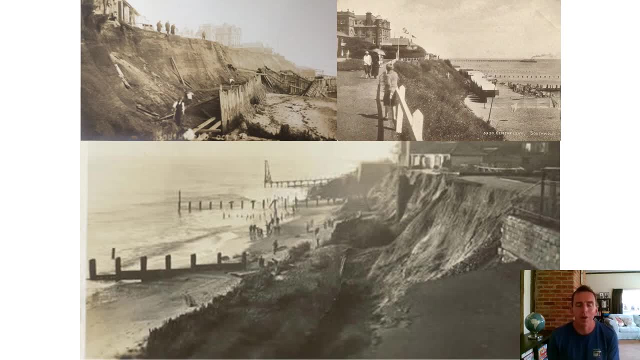 whipped up into a frenzy and previously along most coastlines in the uk, before any kind of more formal hard engineering was invented, most cliffs that were vulnerable were just kind of protected by a layer of timbers that were basically a kind of a wooden sea wall. and you know, very often we 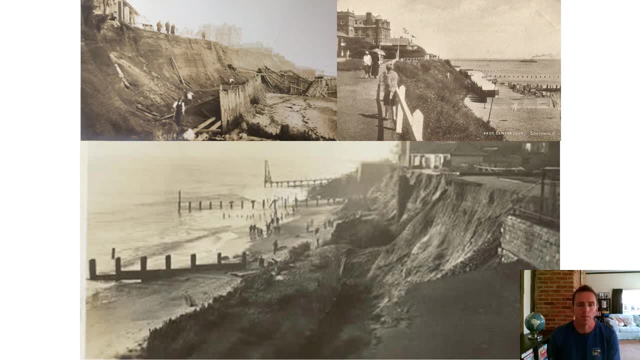 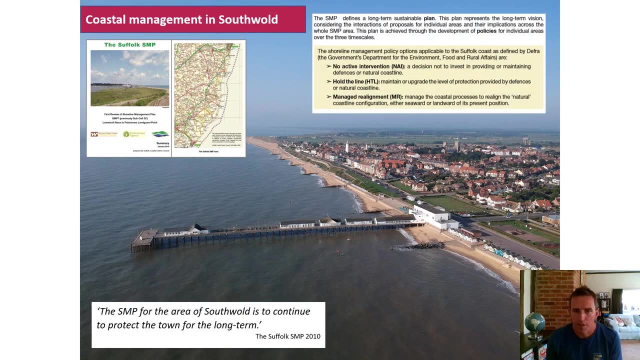 would see a storm that would breach those barriers and cause um significant coastal damage. generally then in the uk, one of the things that happened that acted as a significant kind of mark in the sand really was um the 1953 um floods, um, you may or may not be aware of the 1953 storm. 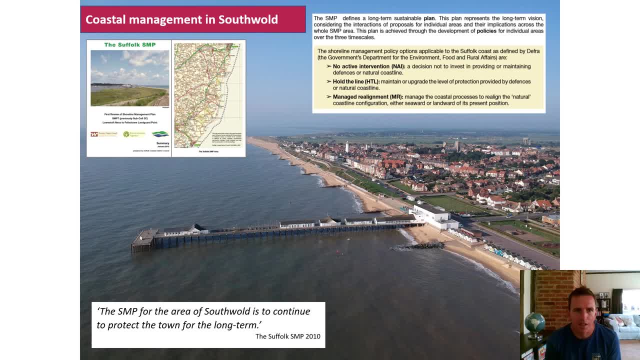 surge in the uk we're not affected necessarily by significant natural disasters. you know we're not likely to have volcanoes and tsunamis and things like that here. but the one natural disaster that we are prone to and vulnerable to, particularly along the east coast, are these things called storm. 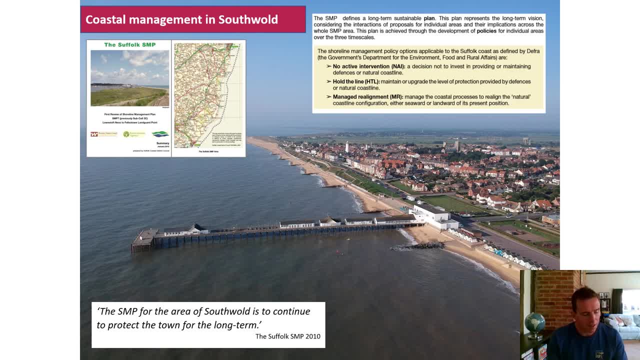 surgeons. the storm surges are where you have these kind of unique weather events, where they normally coincide with a number of things culminating at the same time: normally a high tide, normally a very low pressure system and normally onshore winds as well, which all three coincide to essentially whip. 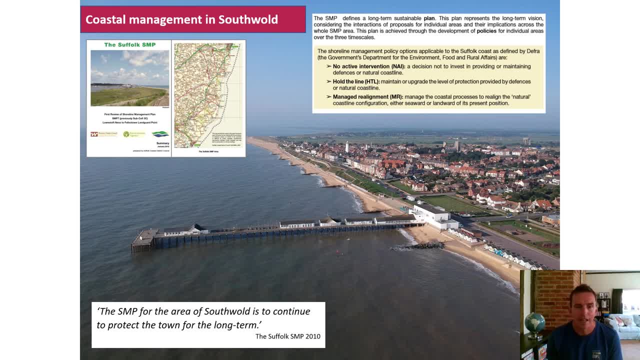 up a frenzy, make it bigger and more aggressive than it normally is and give it the potential to be destructive. in 1953, south bold had a significant storm surge event and um towards the the southern end of the beach there, where you can see the dunes, beyond the pier, where the groins run out, there's. 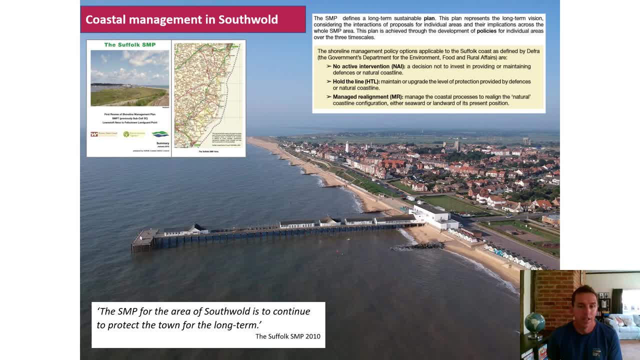 the dunes there are in front of the street called ferry road. five people were actually killed overnight in january in 1953 when a storm surge inundated south boulder water and absolutely battered, and to the north of town as well. all of the marches were flooded out and people had to be. 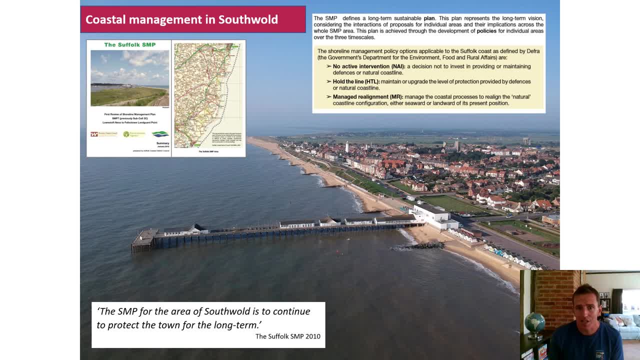 evacuated and rescued from their houses up and down the east coast. over 350 people died in one single night and across the way- kind of opposite to us in the netherlands- hundreds of people also were killed. so storm surges, particularly this storm surge in 1953, acted as a real kind of 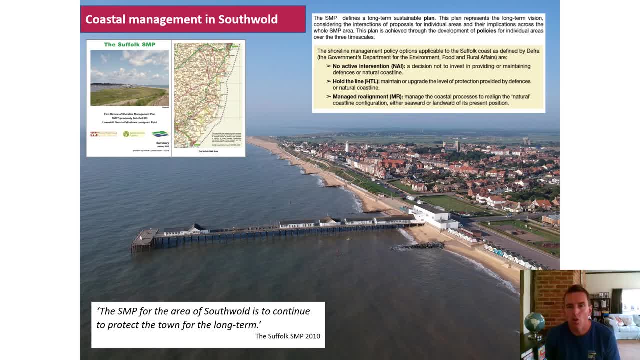 trigger point for the government to come out of a more solid, consistent, robust way of defending the coastline. so one of the things that we now have are these things called shoreline management plans, which i'm sure you're probably familiar with, and shoreline management plans document the localized strategies for defending or protecting, or it's actually 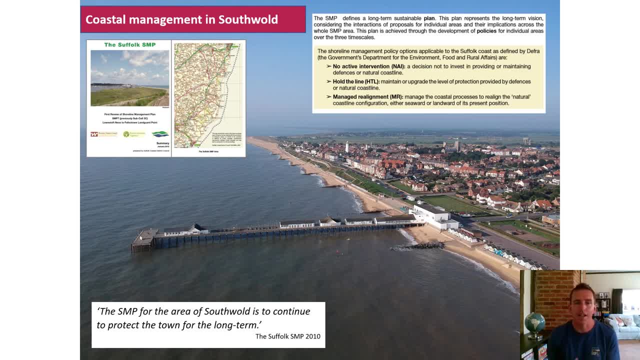 managing the coastline. the whole uk coastline has got a plan, whether it's defended or not. there has been a decision taken about how that coastline in that section is going to be managed. well, you can see from this picture here that very much of the coastline is being managed by the environmental agency, which has already 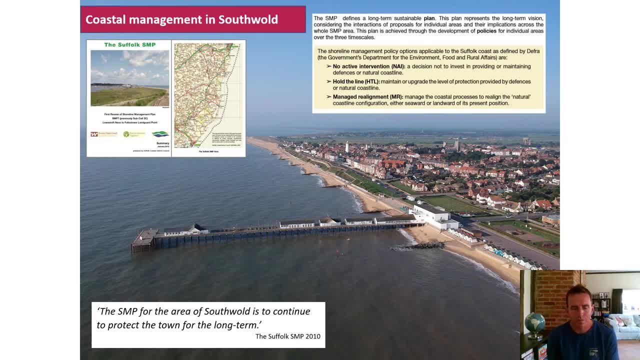 installed the line, and the most obvious form of defense that southport has is this big strepti concrete that sits in front of it: the sea wall- a seawall here- is about one and a half kilometers long. it's worth- the environment agency values it- 20 million pounds- 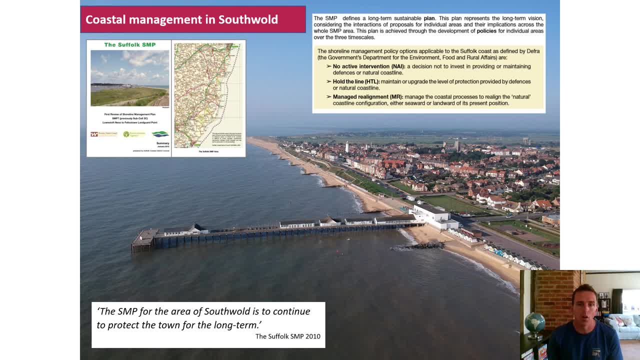 it hasn't all been completed and installed at the same time, but since the 1960s, south boulder had a seawall protecting it, a solid concrete seawall, and it was extended in the 1980s, which i'll tell you about in a little while. 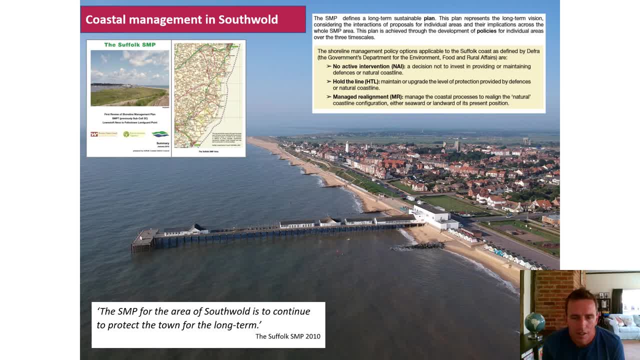 is to hold the line south and north of the town. there is a plan of managed retreat, particularly north of the town. to the south the plan is more of a natural um engineering approach where the the idea is to have um, a kind of a managed section of sand dunes. but the north of the town we have 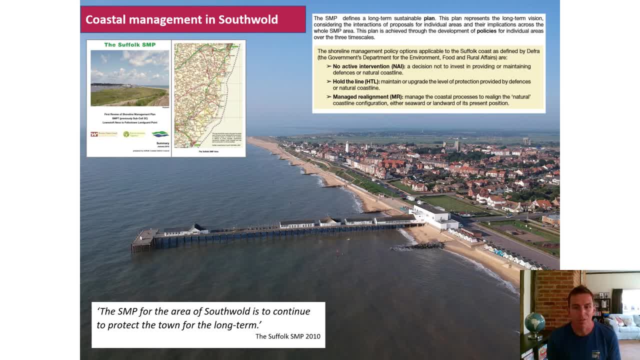 this, this area called eastern badlands, which is actually being allowed to just erode and, uh, that will create this kind of coastal conflict and issues um. but if you're looking at coastal geography and doing a study on the physical aspect of south waltz, um coastline and awareness of the 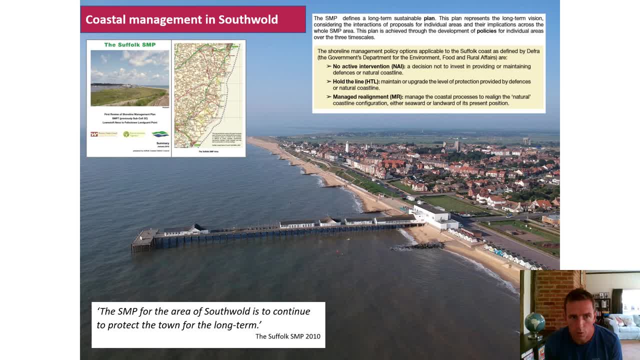 south wold shoreline management plan would be useful and looking at the suffolk shoreline management plan, particularly for using in your introduction, would be wise. but just to give you it the nuts and bolts of it at this point. long-term plan is to try and protect the town from the risk. 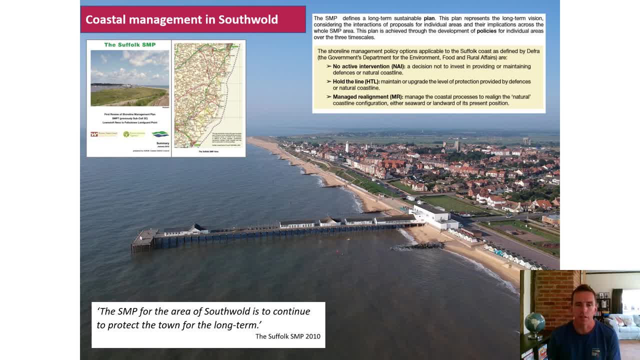 of future flood strikes, and there's a lot of history behind the development of the south waltz, and this is a story that we're going to be going through now. so the south waltz has been used for four years, and this was built in 1913. 60 years after the storm surge in 1953, south wold and the 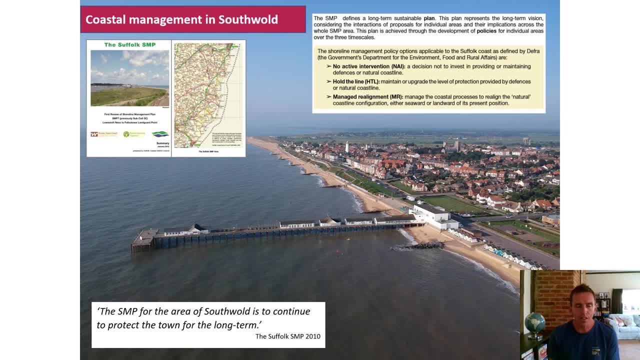 east coast had an even bigger storm surge events, but in the meantime, sea defences had been installed and, although the storm surge was actually bigger in terms of the height that it reached, it didn't breach the the sea defences that were in place. nobody was killed, nobody was injured, and there 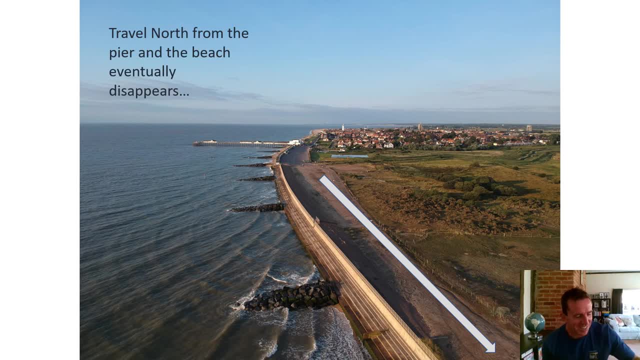 keeping the same place. oh, all right. so i'm not sure whether that video will have played or not. if it did play, you can just mute the song if you don't like it, um, and just watch the images. but what it does do is it gives you an overview of south wold shore from the south to the north. 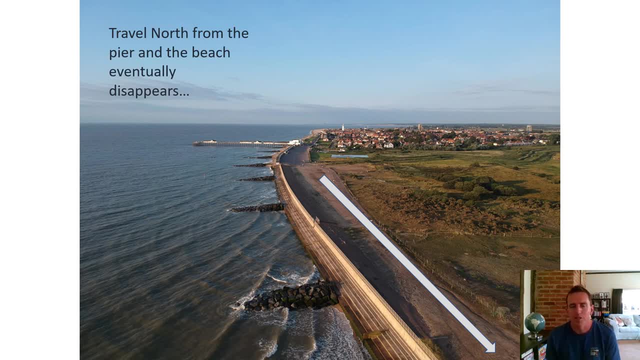 flying over the pier. for the vast majority of you, i suggest the best place for you to conduct coastal field work is from the area from the pier south towards the start of the sea wall. that one kilometer stretch has got everything you need in terms of coastal defenses and, if you need, 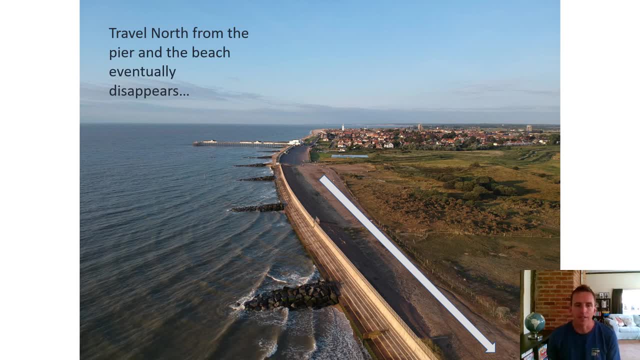 to go further north from the pier, then that's fine, but particularly beyond, the pier car park is a place that i'll need to accompany you with because it does get a little bit sketchy in terms of access and health and safety. you travel north from the pier in the pier car park, the beach. 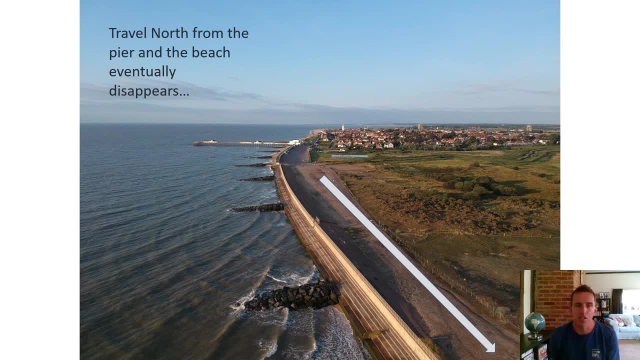 eventually disappears. you can see here, despite having a nice sandy beach south of the town, to the north of the town there's no beach at all and at high tide the sea comes right up to the sea wall here. if you swung this camera angle around and looked to the north rather than to the south, you would then see this and ultimately, the sea. 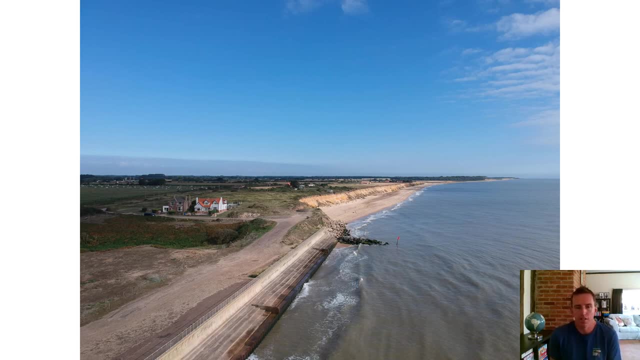 defenses and the sea wall that protects our world has to run out. the environment agency and the local authorities don't have indefinite- you know, unlimited- funds just to keep them betting in um sea wall and extending it and eventually had to make a decision as to where it would limit to. 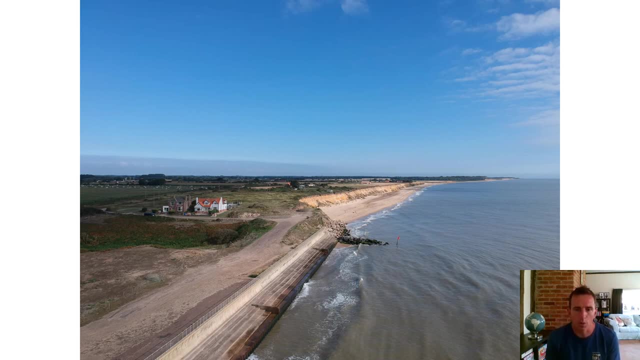 and where it would stop. so this is the end part of southfold sea warning. you can see we've got rock crawins north of the pier here. the last one there is in line with the end of the sea wall. so those sea defenses do the job and did the job of protecting the town from storm surges. 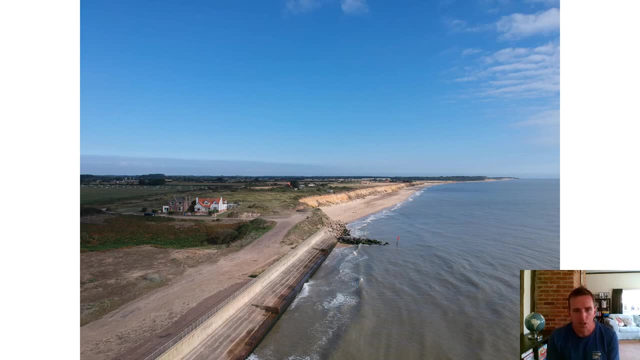 and ongoing coastal erosion. however, it would be frustrating if you live beyond the extent of those sea defenses- and unfortunately people do- and those two properties- there are both properties owned by chapel mr peter boggarts- and a lot of the land that you'll see beyond and behind those. 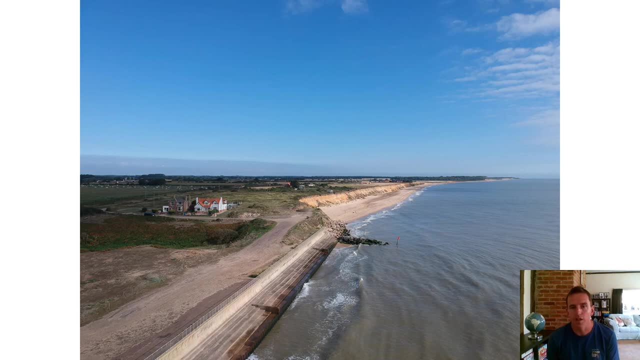 houses are also owned by the boggarts family, who farmed and owned the land up here for over three generations. so you can imagine in the 1980s, when this extension to the sea wall was installed and the sea defenses were improved, that the boggarts family were a bit miffed because 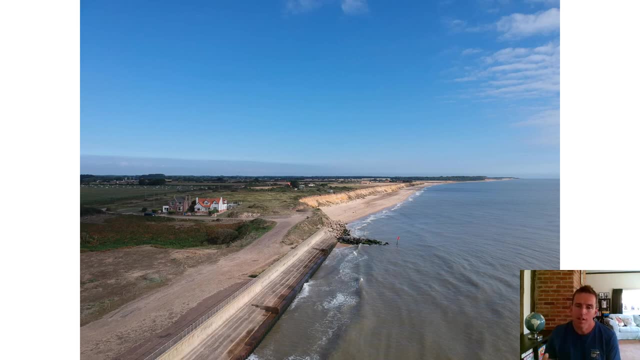 actually their houses, and the vast majority of the property that they own has not been protected by southfold sea defenses. they live about 10 meters beyond the end of the sea wall, so actually any future erosion would have affected those houses. so this is one of the 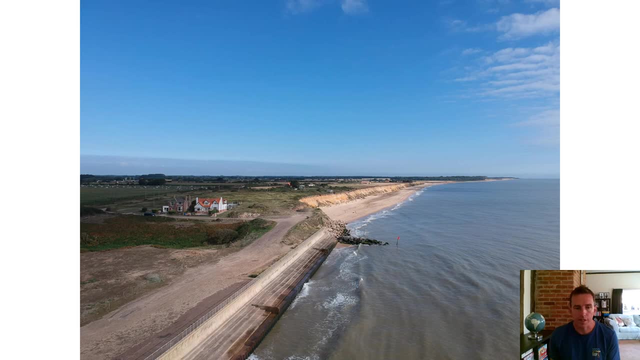 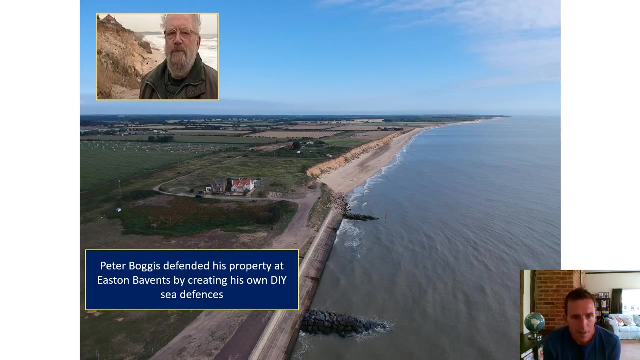 unique stories in southfold. it's an idea of coastal conflict and, linking to this, this cat, peter boggarts. there he is. peter boggarts was an engineer as part of his career and um one of the things that he was adamant about was that the sea defenses of southfold should 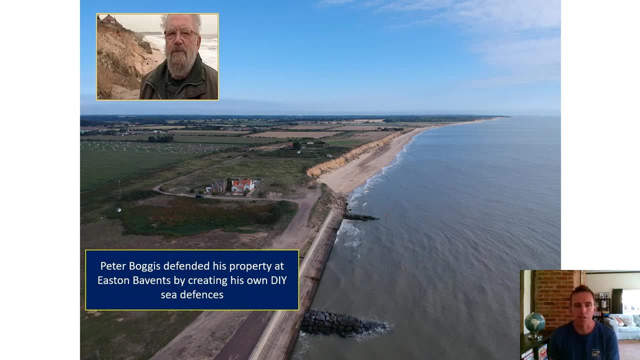 be extended to at least cover the protection for those two houses there, house that he and his ex-wife lived in. mr boggis then campaigned for a long time, through the late 1980s and throughout the whole of the 1990s, to try and get these sea defenses extended. 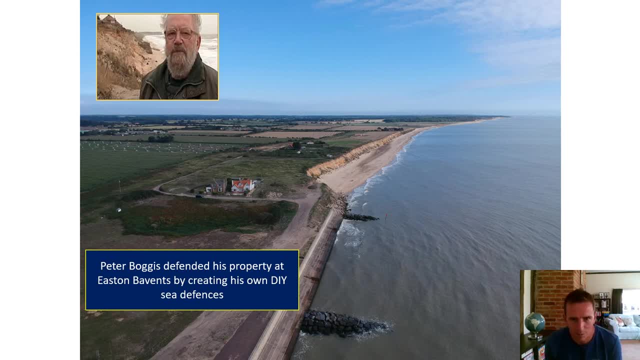 but unfortunately the local authorities, the environment agency, said: look, just haven't got the funds to do that and their decisions are based mainly on having um high value lands to protect. so normally their, their investments are places where there's a significant amount of people or where there's a significant value to the land. it's a significant land to protect. that's their investment. to protect. so normally, their, their investments, are places where there's a significant amount of people or where there's a significant value to the land, and it's a significant value to the land and so, in the form of the real estate, and the real estate as an example of the land, has been introduced as a national. 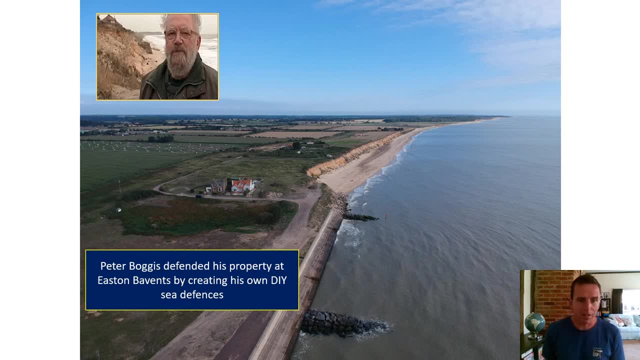 targets and i've looked at some of those partners in order to build the, the land i've included a few years ago and the land And, unfortunately for Mr Boggess, the value of the land here and the amount of people at Eton, Badlands, just wasn't enough for them to justify spending more money on protecting his 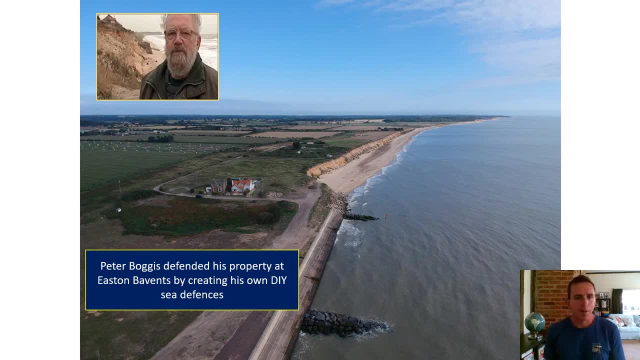 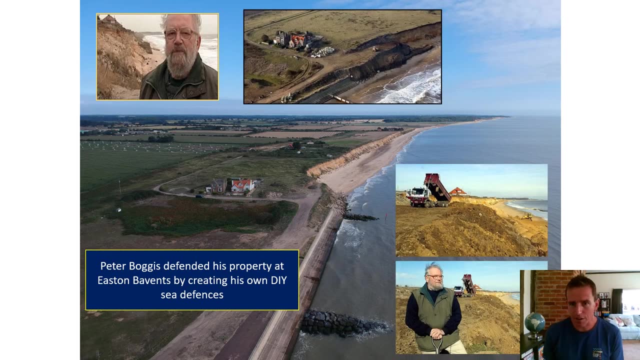 property. But he said: well, fair enough, then, if you don't do anything about it, I will, and I'll take matters into my own hands. And he was good to his word. So Mr Boggess created a very unique. 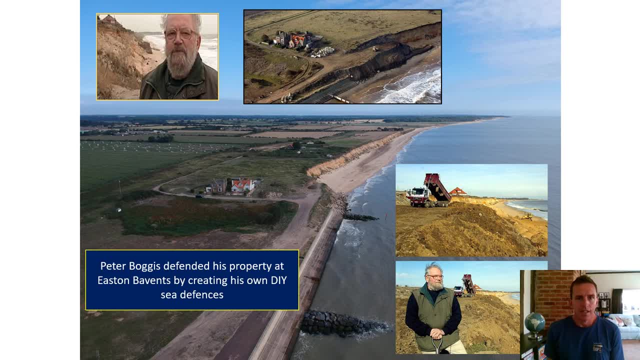 example of DIY cedar fences. He actually was very resourceful and he contacted lots of local construction companies in the late 1990s and said: look, I've got a problem and I think you can be my solution. I'm looking to create my own defences and what I need is rubble. I need material, I need 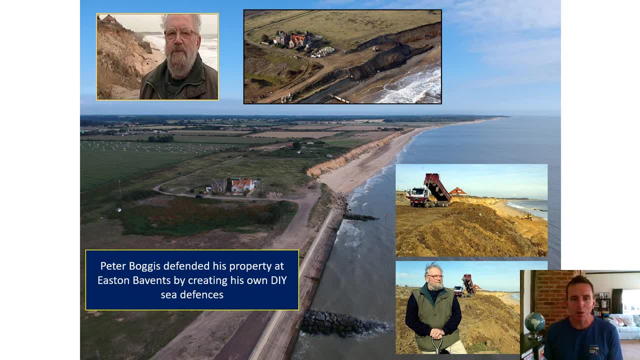 any kind of stuff that you don't need from any building projects that you're doing. I need it on my beach, And so lots of construction companies have to actually work in demolition before they construct. whatever it is that they're building And they often deal in and have to dispose with. 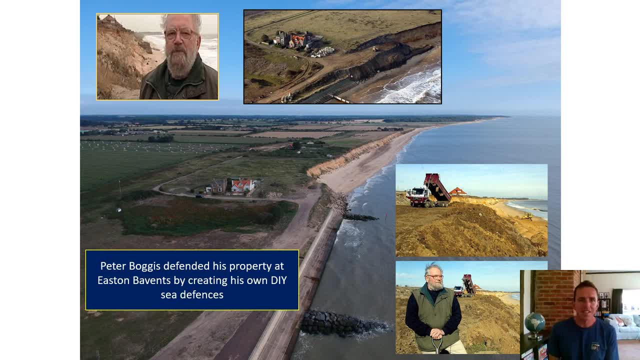 lots of rubble And lots of waste material. So this is what Mr Boggess wanted And he kind of publicly said: well, I'm dumping soil on the beach here and it's all good quality stuff. But the reality was that 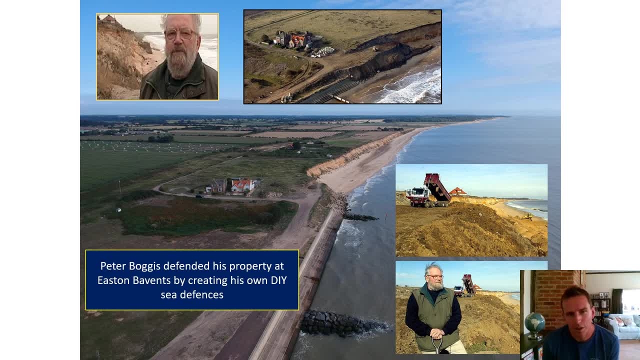 actually he invited all of these local construction companies to dump stuff on his beach, but none of it was regulated by anybody at all. He created this rough track that went up the back of the seawall here. Lorries used to come up there, reverse and then tip to let their loads onto. 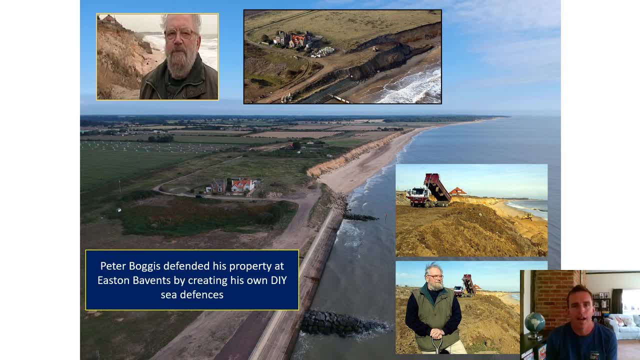 the beach And he, Mr Boggess himself and a couple of his friends, had bulldozers that they used to align the material and compact it and to drag it and to put it in place along the beach in front of the cliffs there, with the idea of 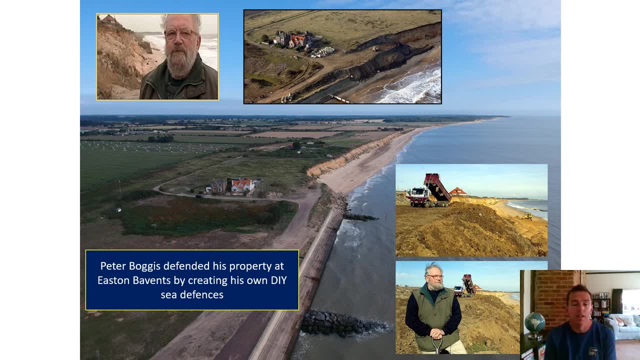 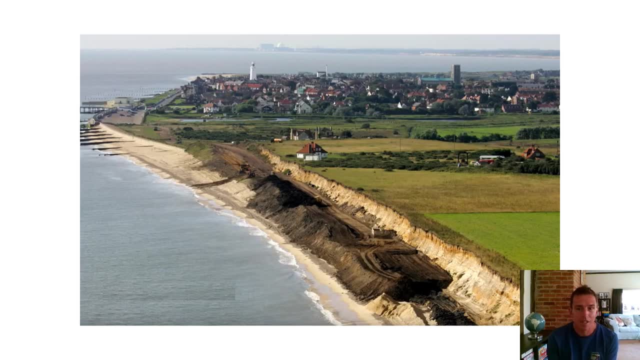 basically adding a reinforcement to the cliffs and to prevent future ongoing erosion. Amazingly, Mr Boggess did this for nine years. This went on between the year 2000 and the year 2009.. And it's just an unthinkable, colossal amount of material. 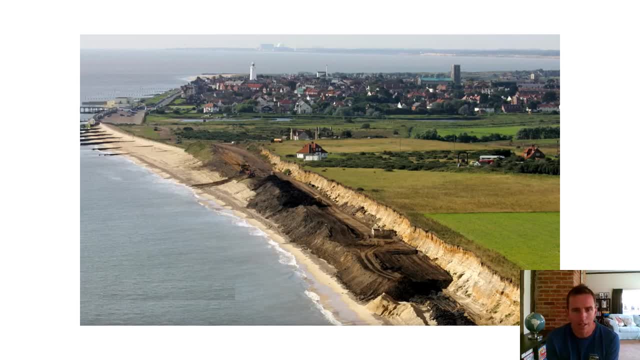 Rubbish was added onto the beach- unregulated material. If you've ever watched the Coast program on BBC, one of the first episodes in series one of Coast actually has a chap called Nicholas Crane who walks from one of those houses across the fields to the edge of the 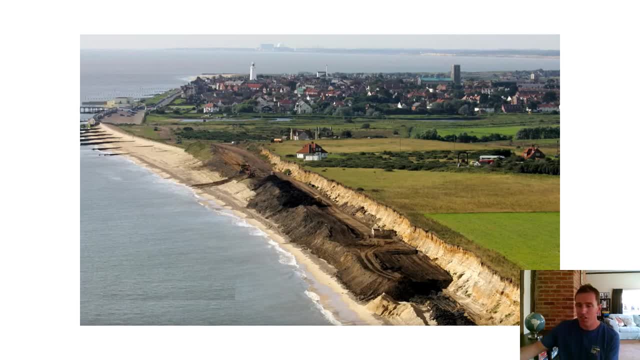 kind of natural cliff. and then they look out over the cliff and they see this huge work site of all these lorries and bulldozers coming and going and material being dropped off and then compacted And it's an unbelievable scene and it's well worth watching. 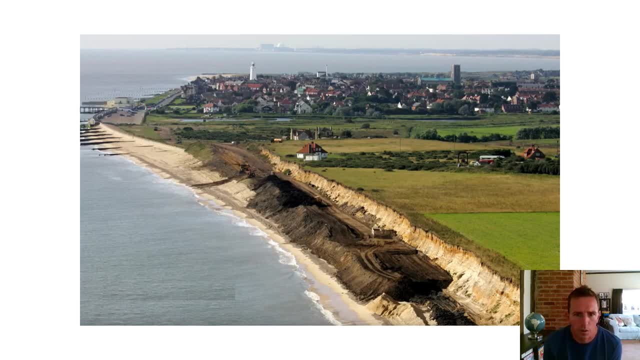 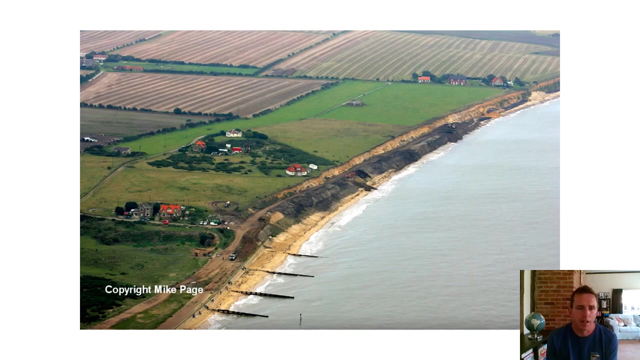 And I'm looking at a few. if you think about this is one of the issues that you want to look into. But yeah, incredibly, over this period, Mr Boggess dumped an unbelievable amount of material onto the beach. The material at its peak stretched over a kilometre north, 25 metres deep, and 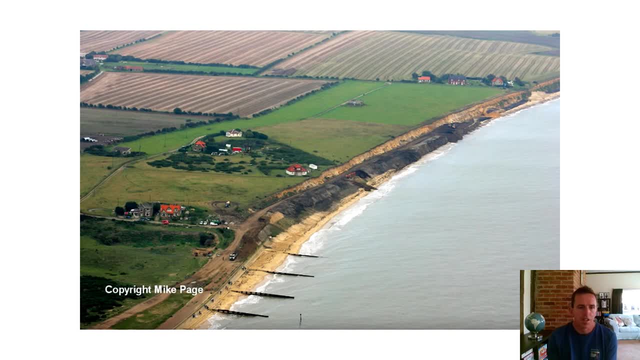 roughly probably about 10 metres high as well. So you know an unbelievable amount of material was added onto the co-time. You can imagine locally a huge amount of concern about this happening And inevitably Mr Boggess faced a huge amount of local opposition and he was 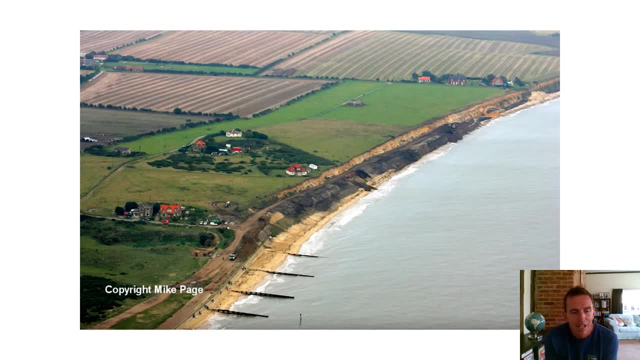 actually taken to court several times. Amazingly, he was able to win those court battles because legally he was able to claim that actually, historically, this property, this beach, was his land And it was his land before coastal erosion had taken away the top part of it, But the original. 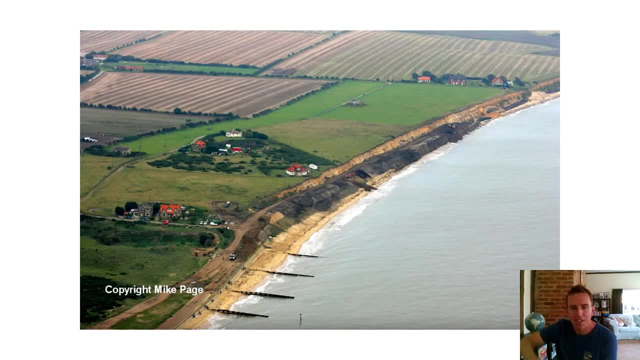 deeds to his property ownership stretched way beyond the beach, actually into the sea, and were actually now underwater, So he was legally able to argue that he owned this land. he owned this beach and it was his to do with what he wanted and to defend with however he liked. Ultimately, in 2009,, he was pulled into court again and he lost the. 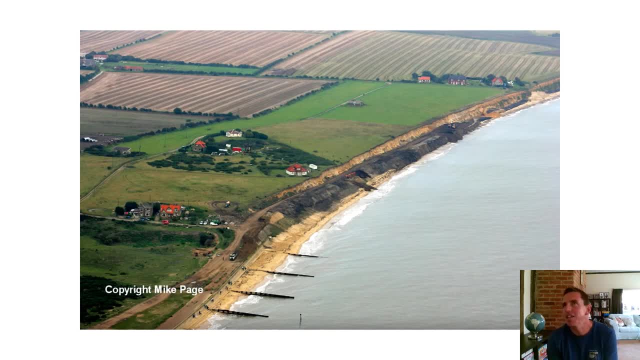 court case On this instance. I think it was English Heritage or English Nature that presented the case against him and said that what he was doing was actually preventing a natural exposure of fossils along this co-time here and it couldn't be allowed to continue and he had to stop doing it. 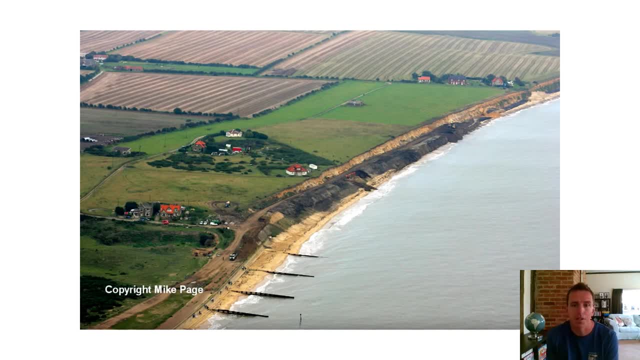 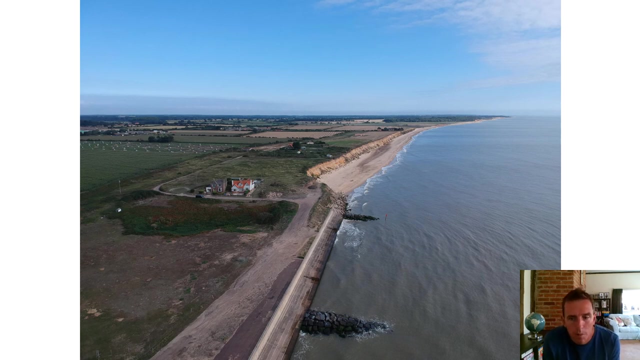 Crucially, though, they didn't say to him that they had to remove the material that they placed there. They just said that you just can't add any more. So in the years since that material has gone- And it hasn't gone because it's been removed by man, it's gone because it's been removed by the sea- the sea has claimed that material, has dragged it, has eroded it and pulled it into the North Sea. 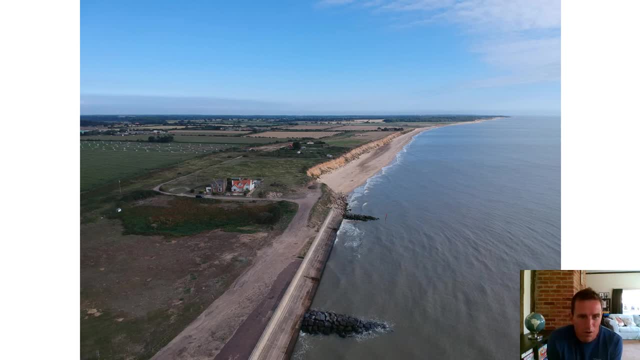 And the worrying thing is is that material is a mixture of all sorts of horrible stuff, So it's now most of it under the water, But increasingly a lot of it washes up onto South Wales Beach as well, And as you wander along South Wales Town Beach you'll notice little kind of red stones. They're not stones, they're just kind of smooth bricks that have been sculpted into the kind of pebble-like shapes. So there has been this legacy of 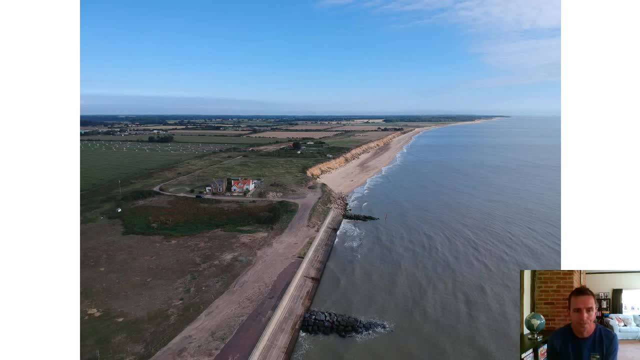 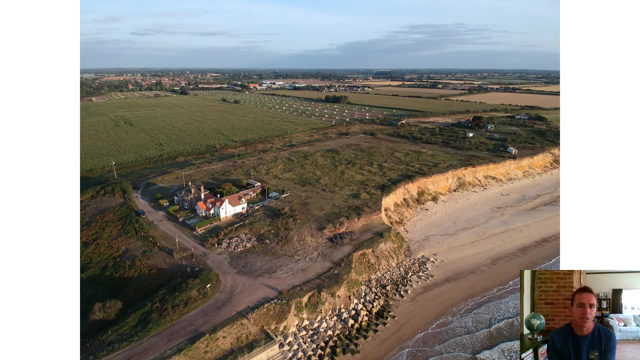 you know a huge amount of material now being out in the sea that shouldn't be there, But you can see that Mr Boggs's house is still there When you zoom in a bit closer. the reason for his house still being there is because in front of his house he added an extra layer of enforcement of what you can see as those kind of triangular- what are called tri-blocks- made out of concrete. 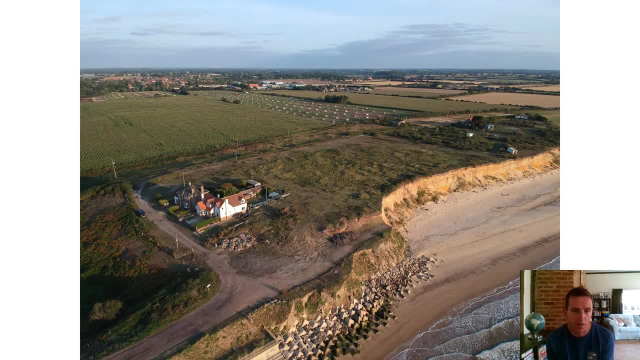 Allegedly he spent a further £60,000 on installing those in front of those properties, who essentially act as a second layer of defence to kind of disperse the energy of the sea out into the North Sea. And that's what we're seeing here is it broke against the cliffs And they've been hugely effective actually, And the coastline there hasn't retreated at all And they've done their job Beyond where he put those extra tri-blocks in. all of that material has now been returned to the sea or ended up in the sea, whereas the bit in front of his house has remained there. So in the 20 years or so since those were installed, the coastline has not been able to touch that part of the coastline. 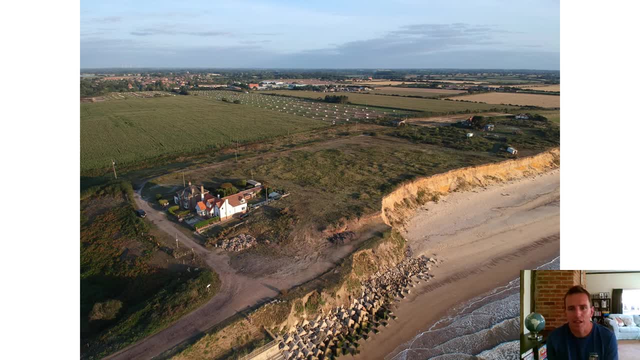 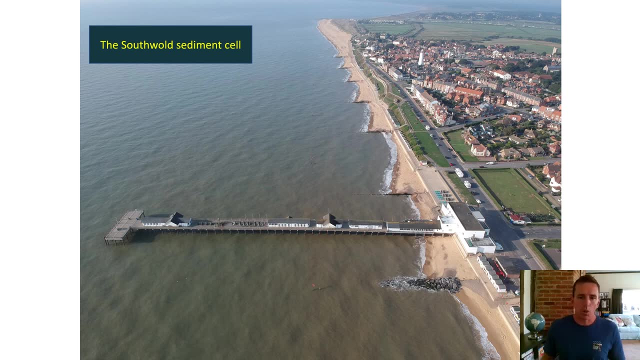 The erosion rates here are about three to five metres a year and they're very, very rapid. So one of the things that we have at Southwold, which is quite unique, is potentially evidence of a mini sediment cell. Sediment cells normally operate on a much bigger system. 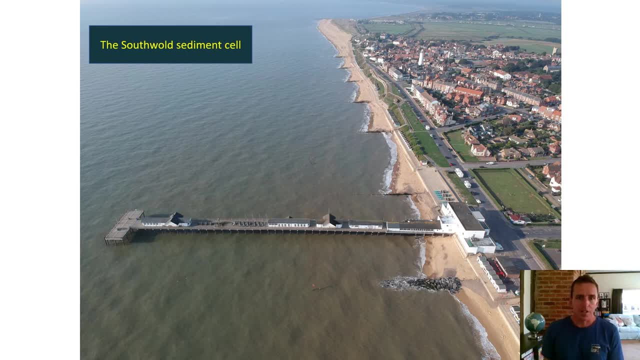 One of the things that we do every year is we walk up and down the coastline with the Environment Agency representatives and we talk about the changes that we've both spotted along the coast And we kind of compare our evidence and our theories And our thoughts about what's going on, because one of the things that's difficult about measuring characteristics of the sea is that a sea is a dynamic beast. 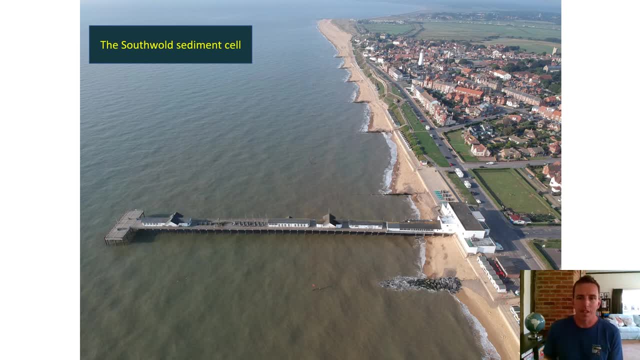 It's full of energy, and it's energy that can be whipped up by winds and weather systems, And it's constantly changing and it doesn't always fit the black and white system that you would expect it to, But there's significant change and uncertainty about the way in which any coastline behaves. 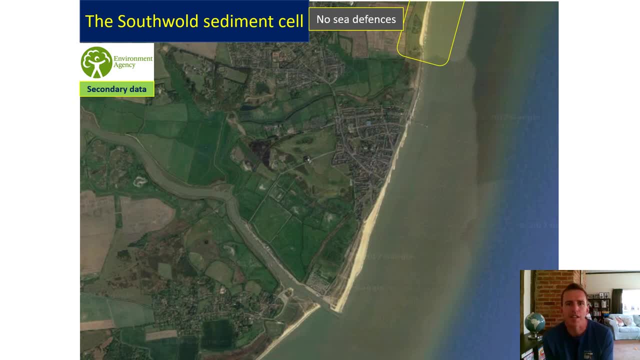 So, in terms of what's happening at Southwold, this, we think, is our kind of best way of summarising the patterns that we observe on a seasonal basis and a long-term basis along the coastline here North of Southwold. as you can see where that highlighted area is there on the map, there are no sea defences at Eastern Badlands, the area where Mr Boxer's house is. 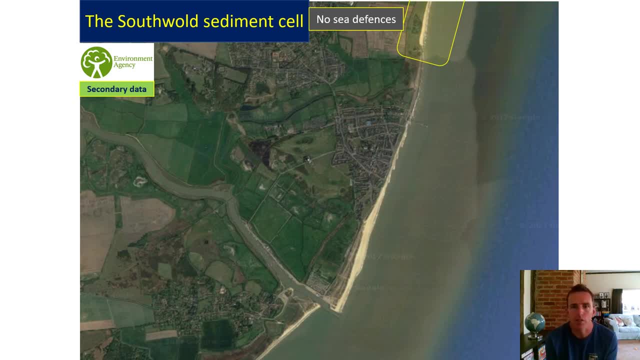 So we know that this is an area where there's significant rates of rapid erosion. What happens here, then, is that material is easily eroded And collected by the sea- the majority of that are small fragments of sand granules- and that sand is then worked into the sea system and normally then joins this kind of north-to-south conveyor belt drift which operates along the general East Anglian coast. 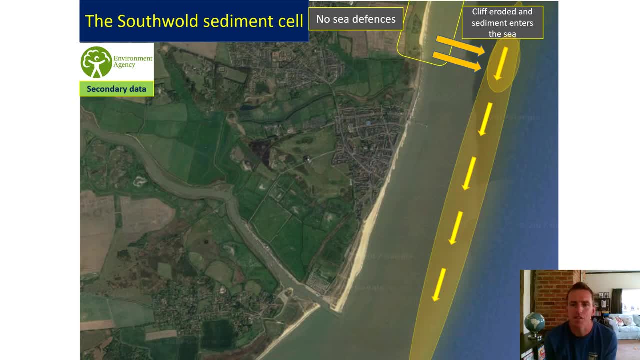 Going north-to-south along the frontage of Southwold offshore is this general drift of current which moves material towards the south. It then passes in front of Southwold town but is then intersected by the River Blythe river current, which then flows out into the North Sea here. 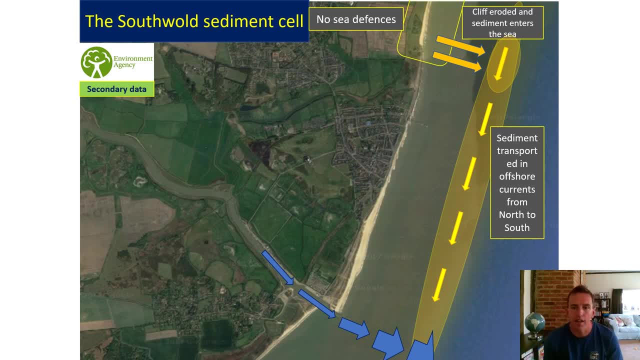 So a lot of the material that is essentially trying to move south can't get any further than this river current here And what we end up having is an area of accumulation offshore of Southwold of kind of quite shallow and not very deep water here. 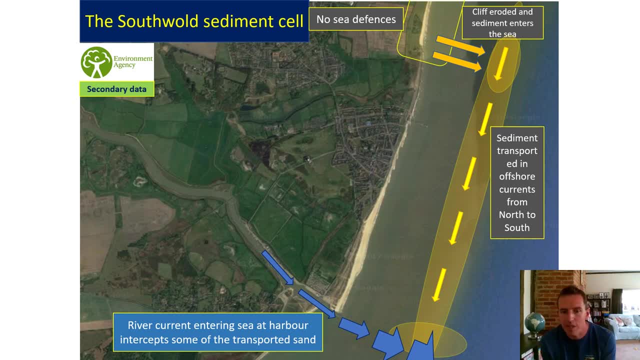 because there is a significant collection of sand material that hasn't been able to shift its way past the river current. What happens, then, generally, is that Southwold, as we have our weather systems approaching from the south and we have waves and winds coming to us from the south. 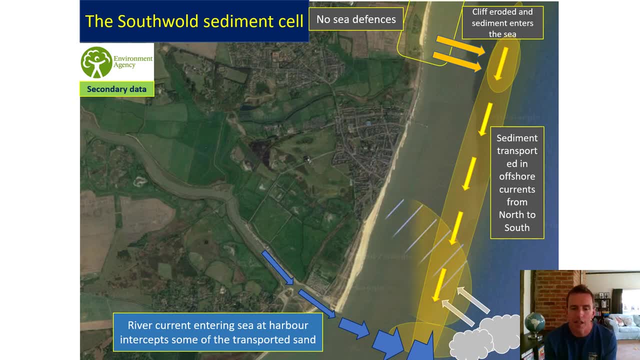 and that system of waves moves over the sandbanks that we have and brings ashore the material that is eroded from the north of town. It brings ashore, in the first instance, generally south of the town, which is why we have a wider beach at this end. 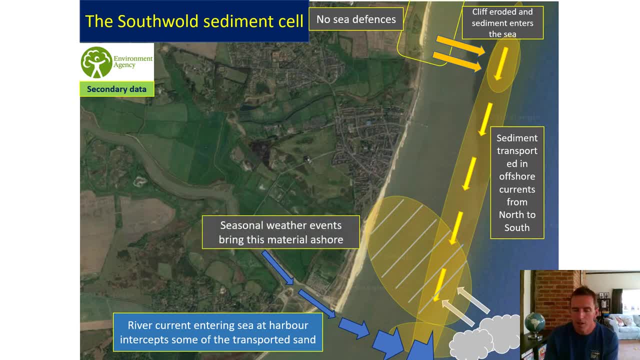 Then progressively that material is then moved north again by a longshore drift towards the pier and towards, ultimately, the eastern Bavon. So you have this kind of cellular system that's in operation and it works in almost like this clockwork system. 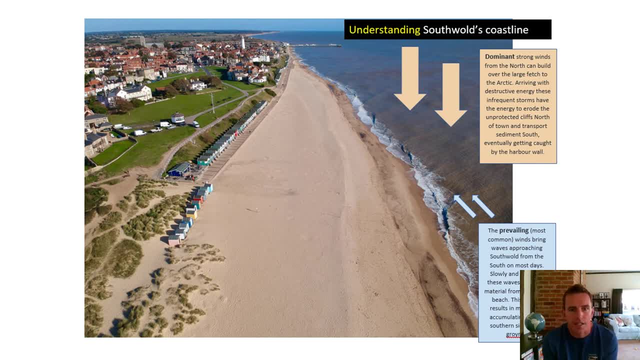 So that explains why Southwold's coastline looks like this. We have one end of it where the beach huts are on the sand dunes, where the sand is nice and wide. The beach is nice and wide up to about 30 to 35 metres at this point, with a sand dune system as well. 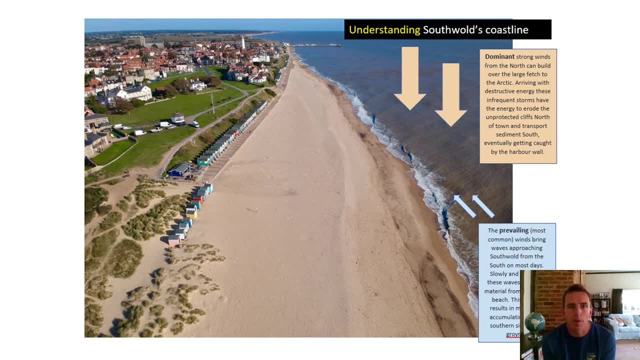 And then very quickly, as you make your way towards the pier and beyond the pier, the beach declines and it kind of truncates itself and becomes much smaller. So this is a result of two major things, And the major things that shape the morphology of the beach are the waves that affect that coastline. 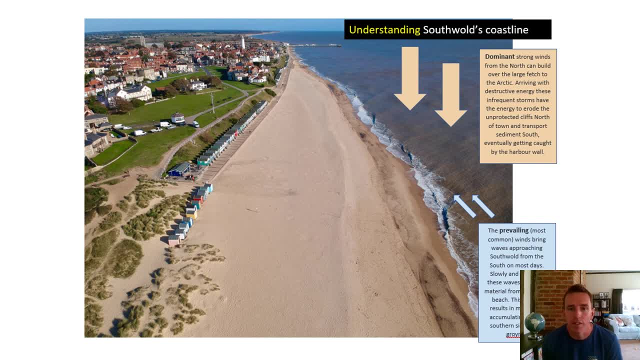 And the waves that we have are determined by two different factors, and those factors are both linked to the winds that we have. So you will have probably all heard about prevailing winds, and I think you've got this diagram in your booklet as well. 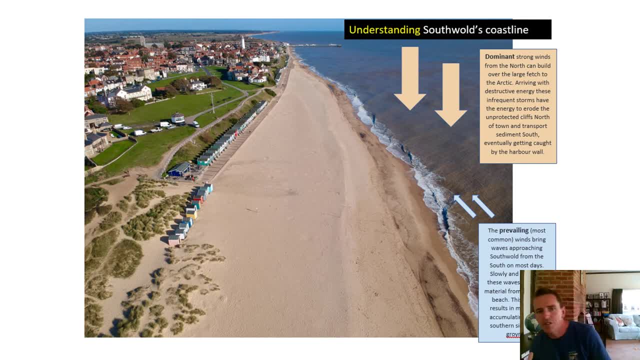 Prevailing winds refer to the most common, the most frequent and the waves that you and the winds that you would normally see on any given day. So most days at Southwold, when you come out onto the seafront, you'll see that the waves are approaching Southwold from the south in the same way that you can kind of see from your picture. 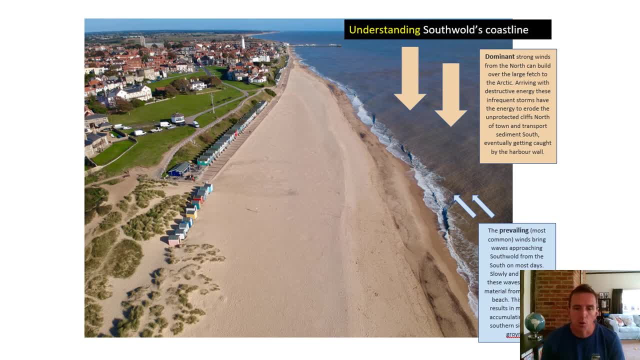 Where those little blue arrows are. the waves are approaching the shore at an angle from the southerly direction, And what that slowly does is it progressively moves that sand material towards the pier, towards the groynes and towards the northern part of the picture. 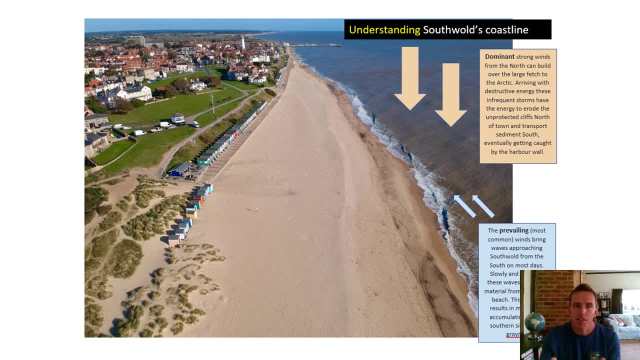 What that will do then over time is it will build up sand on the southern side of the groynes because that sand is being trapped by the barrier that the groynes are forming. So you can see that longshore drift is happening regularly by measuring the accumulation of sand against those groynes. 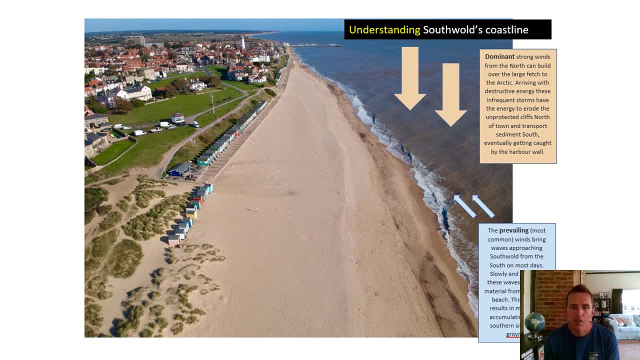 However, these prevailing winds haven't got a huge amount of energy to sculpt the broader coastline, and it's actually the dominant winds that affect the coastline here probably more dramatically. The dominant winds are winds that we get much less frequently, perhaps maybe only a handful of times a year. 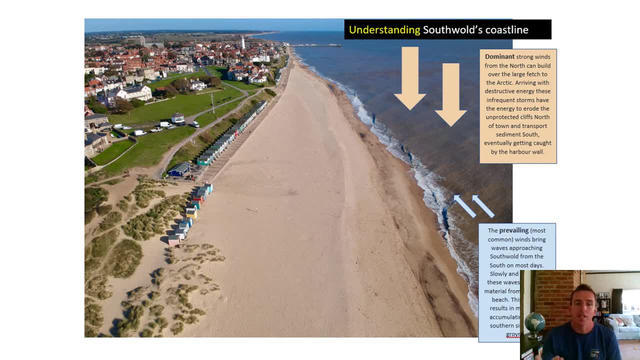 when we have weather systems that approaches from the north- And between the Suffolk coast and the Arctic there is a considerable fetch. So if you have a weather system coming from that direction, the waves can actually get to be much bigger, much more powerful. 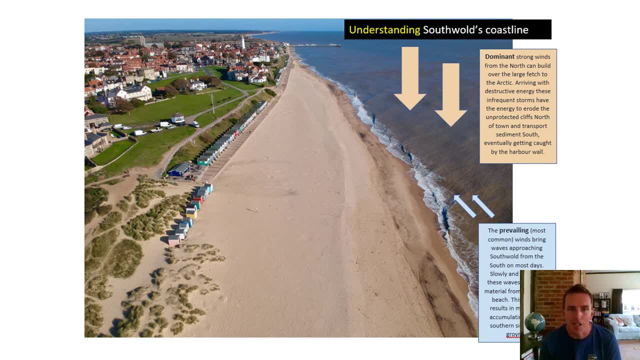 like the video that you saw earlier of the waves breaking really hard against the seawall and underneath the pier. So when we have waves approaching us from a northerly direction, they are much more dominant and much more productive at creating erosion and creating more transportation and more movement along the coastline. 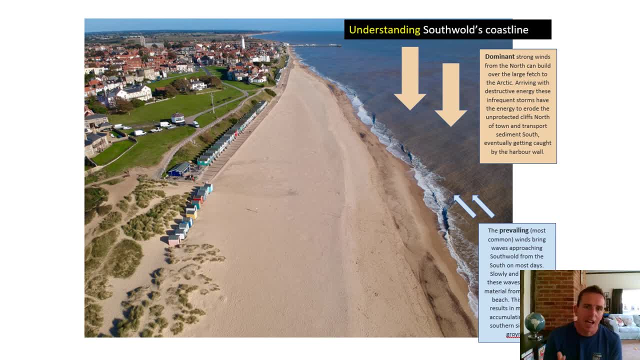 So that happens much less frequently, but it does happen sometimes, And that then explains why we have this kind of system along its outboard shore, where we have more sand at the south and we have more erosion going on at the north. The erosion generally only happens maybe four or five times a year. 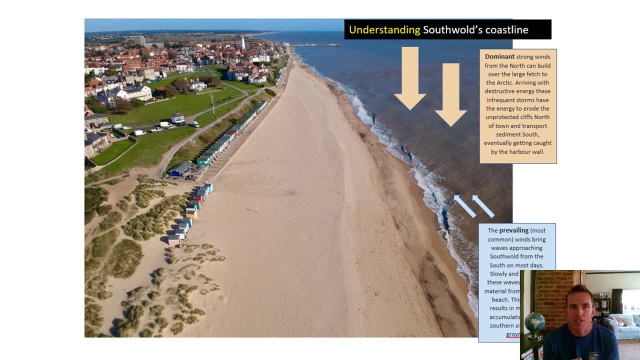 but when it does happen, it's there where the material gets collected from. in the eastern Badlands area. The process of longshore drift normally operates in reverse of that, and referring back then to that sediment cell hopefully gives you a bit of a broader understanding. 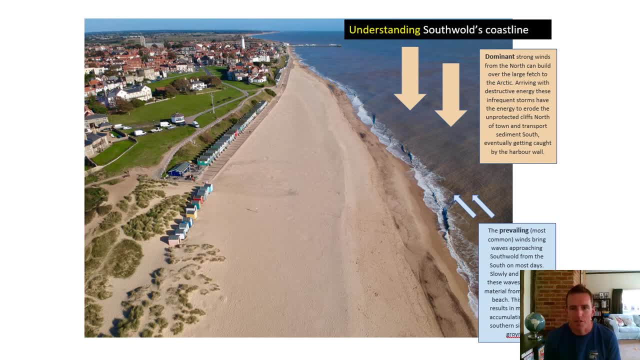 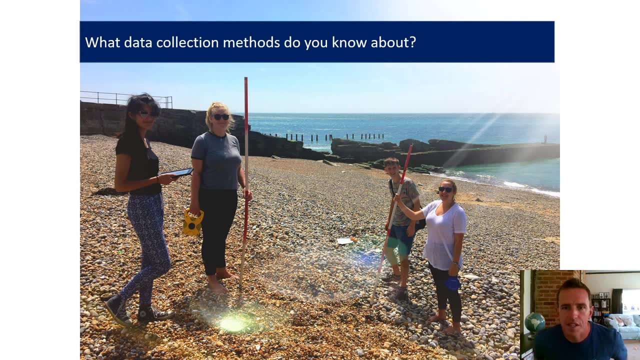 about why the coastline here looks as it does. So if you are to conduct a study on physical geography in Southwold and coastal geography, you're going to need to be aware of the different methods of data collection that are available to you And, as I said earlier, 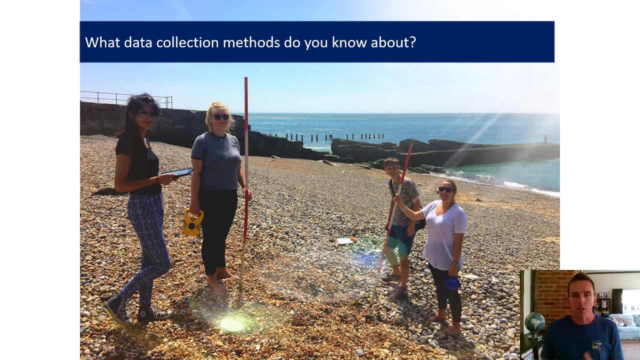 I would suggest that one of the things that you should do is to look at Jogit and look at the suggestions that are available on Jogit for you to record your data on that app and using your phone. A couple of things that are useful in Southwold. 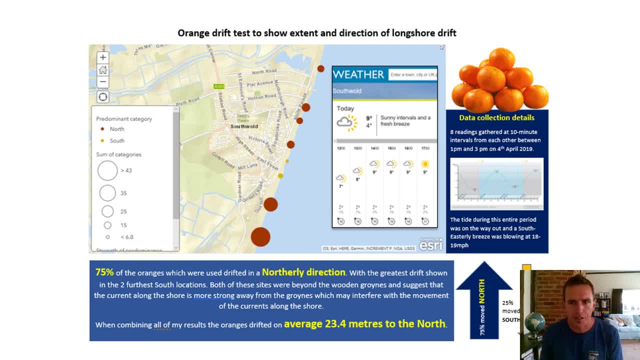 and this thing here: a longshore drift orange test. So this is where you release an orange into the shore of the sea and then you time over a set period and later then record how that orange is and how far that orange has moved. 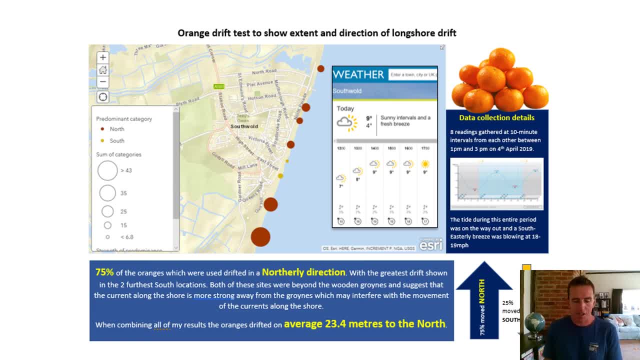 So to do this, it's up to you really, the methodology, but normally I would suggest that you use a marker, perhaps a ranging pole or a significant stone, and you place that in line of where you throw the orange into the water. You then start timing for the set amount of time that you want. 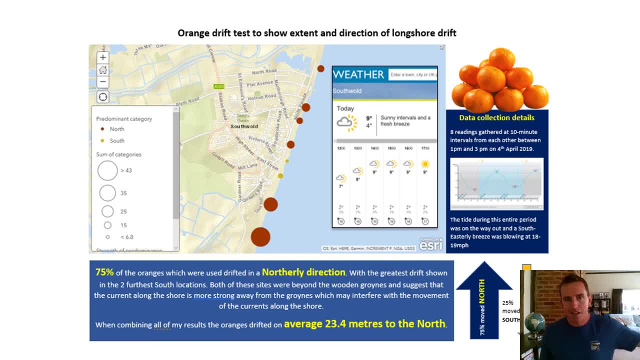 and then, at the end of that time, you press it up again, and, with a second marker, you mark the point, in line on the beach, of where that orange is drifting. You then need to measure the difference between those two points, and that, then, is the distance that the orange has moved. 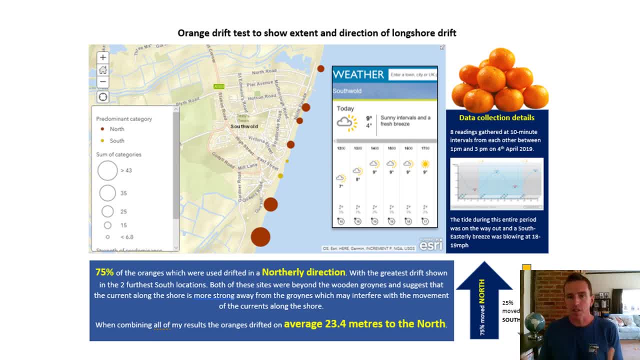 and because you've then got your time as well, you can divide your distance by time and you can create the velocity there of your orange. What this person has done is they've got the latitude and longitude for each time that they threw their orange into the sea. 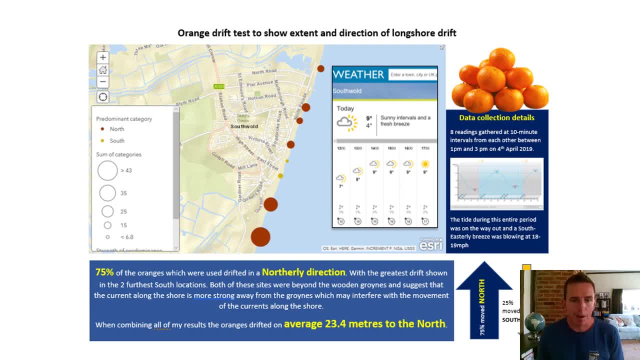 and that has meant that they've been able to produce an ArcGIS map to show how the velocity of the orange changed in the different locations that they did their longshore drift test. Colours that they've got there as well represent the north and the south flows of the orange. 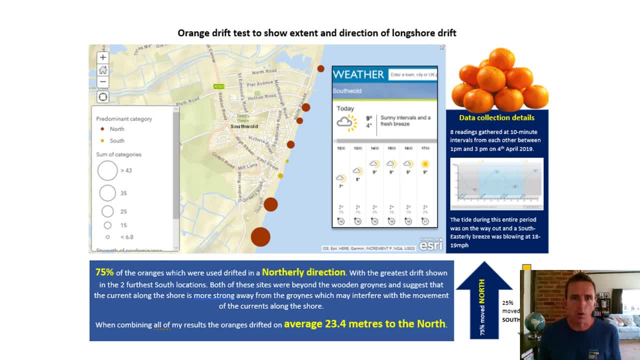 and most of them have gone north there. If this is something that you're interested in doing, let me know when you get to South Ord and I'll show you how you can present this material. But one of the things that you'll need to think about then 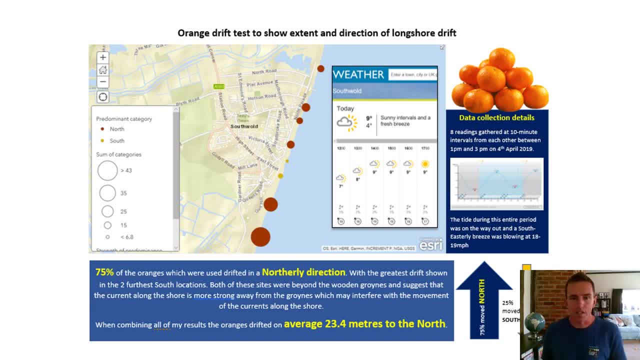 is the methodology of how you're going to conduct the different bits of data collection that you're wanting to do. So again, the sampling size, the sampling frequency, the equipment that you're going to use all of these things, the locations where you're going to do your actual fieldwork. 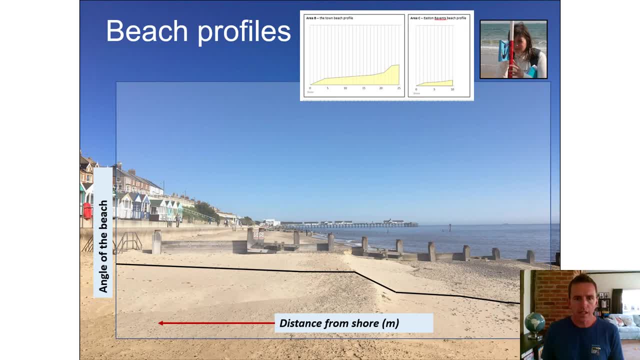 it's going to be down to you. Another thing that you could do is try to assess the impact of the coastal defences on the beach morphology, and very often the most traditional way of doing it is a beach profile. Beach profiles are essentially a way of measuring. 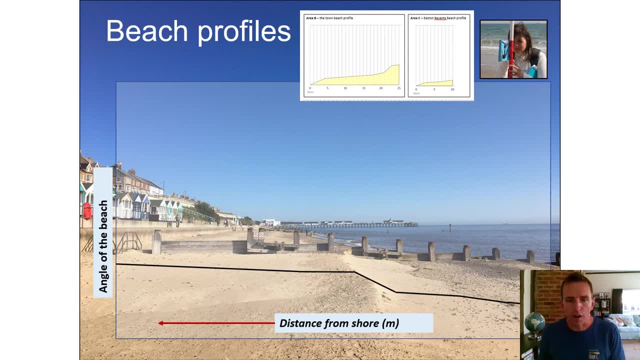 the changing gradient along the profile of the beach, and you can either do it from the shore up to the seawall or from the seawall down to the shore. it doesn't really matter, but ultimately you'll produce a graph that shows the gradient of that beach. 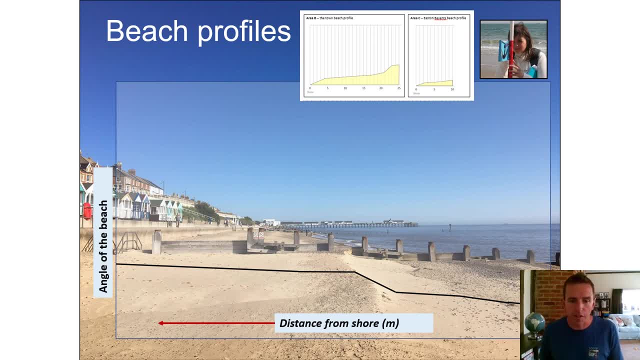 Yes, there were a number of the different methods you were doing, particularly coastal geography, but it makes sense to take a picture as well of your fieldwork site. So you know, a graph can be fine and it's a bit more scientific. 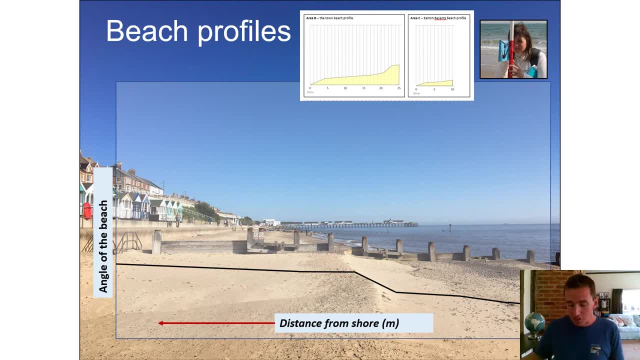 but actually if you're doing a study or trying to make a point about the changing morphology of the beach, it would also make photos. You can see here this person's actually layered their graph onto the actual photograph that they have of the beach, so it's kind of an effective way of integrating the two. 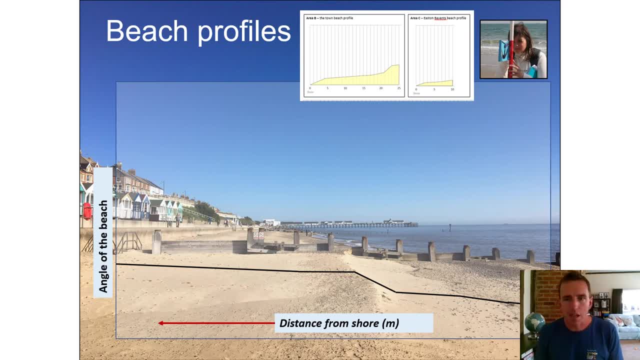 Beach profiles require two ranging poles, a tape measure and a clinometer device which measures your gradient, and it also normally will require at least two people doing it. So if you're doing a beach profile, you might want to think about who you could perhaps team up with. 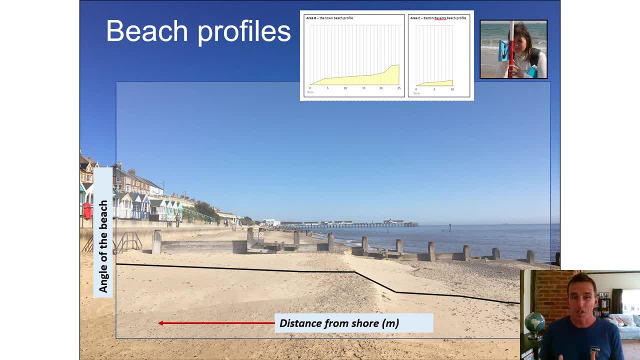 to make yourself more efficient. One of the things that I would say about a beach profile is that, generally, of all the methods of data collection, they are one of the most time consuming things to do, So really make sure that if you're intending to do this, 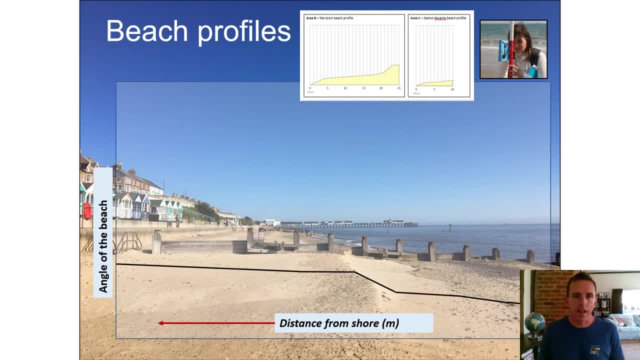 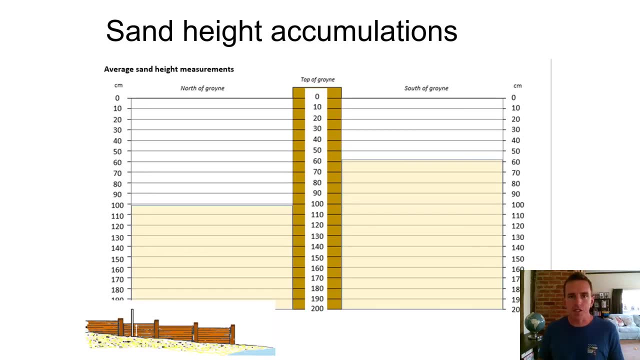 that you're completely clear that the results of this are going to help you and are actually really useful. An alternative would be doing something such as beach size measurements or sand height accumulations, or seawall measurements In terms of sand height accumulation for this one. 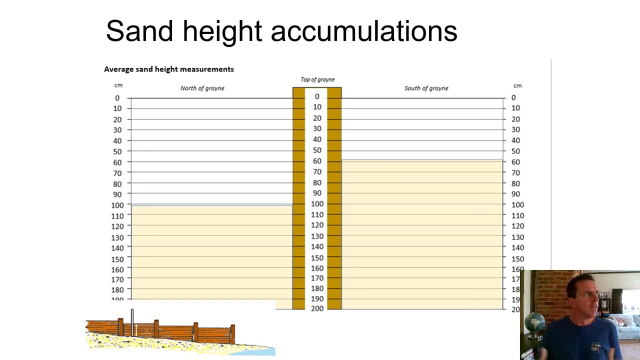 what you're looking to do is to try and prove the effectiveness of groins or maybe the evidence of longshore drift. So you can do this by measuring the sand height accumulations that you have either side of the groin. I've got a little sketch of a groin there on the bottom of the picture. 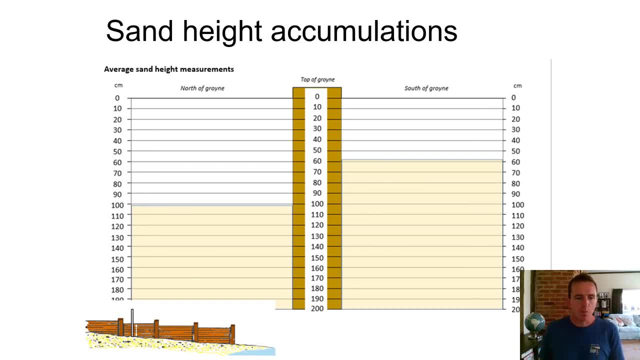 What you'd need to do is, then, using a tape measure- and we can give you these- is to measure the height of the sand that is accumulated against the groin, And to do this, you measure from the top of the horizontal beam of the groin down to the sand level on one side. 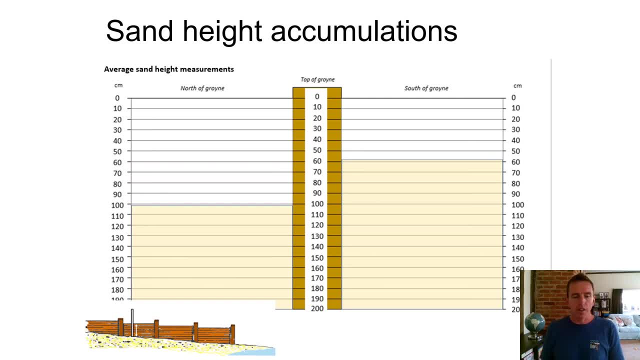 and then, in exactly the same location but on the opposite side of the groin, you then do the same. So you have a north and a south reading. You'd need to then see whether there is a difference. So if there is more sand accumulated against one side, 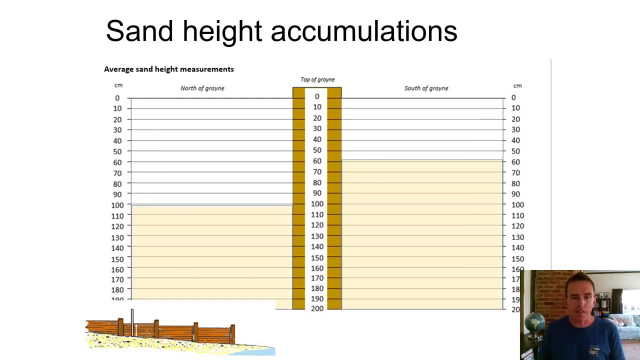 that suggests longshore drift, then, is kind of trapping the sand on that side and suggests that the groins are being effective and also can tell you which direction longshore drift is operating in. However, to make your results more reliable, you'd need to make sure that you did probably more than one measurement. 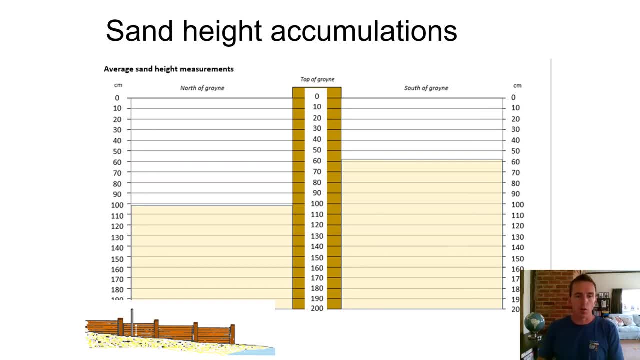 along that groin and then perhaps maybe five measurements along the course of the groin. And because we've got seven groins in Sandfold that are measurable, these wooden ones, then it might well be that you choose to measure all seven. I will say that sand height accumulation measurements are very difficult to do. 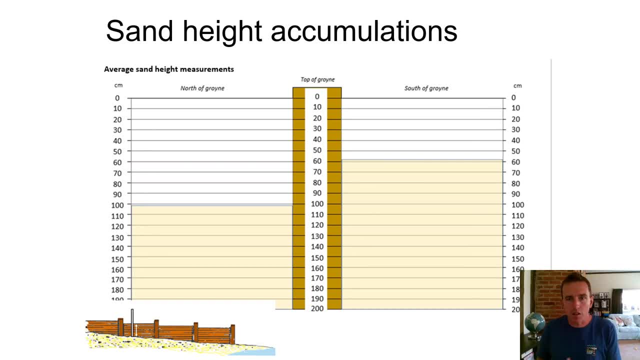 against the rock groin, so don't worry about doing them there. One of the things you could do is to take a picture of those rock groins and then annotate that to show why you haven't measured the sand height accumulations here, And it will show that it's very difficult practically to do it. 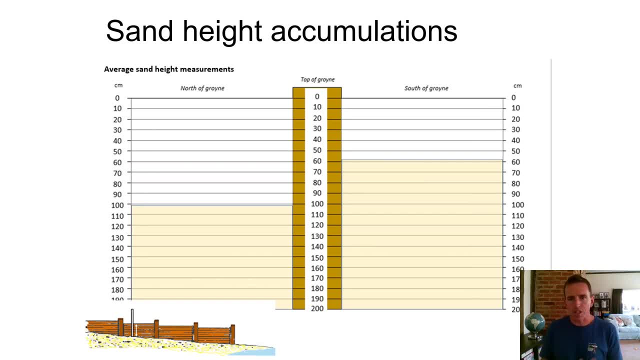 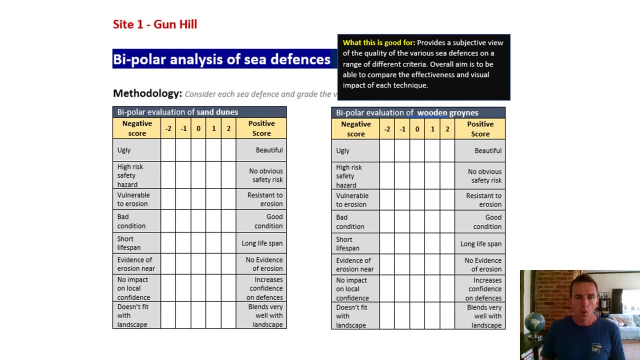 also there's a hazard involved because a lot of those rock groins are covered in this motty algae, which makes it very difficult for you to actually get on to them, One of the things that you can do with all of the sea defences that we have. 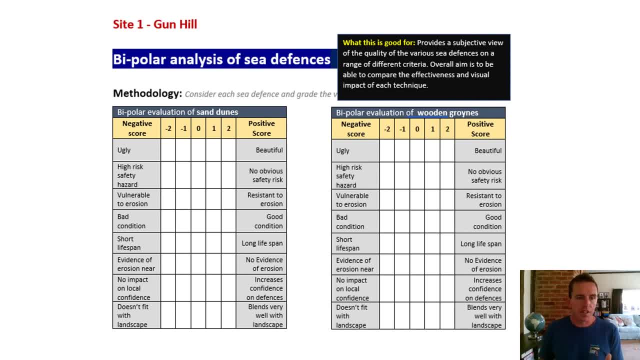 is a very simple bipolar survey. Here we've got criteria that we have come up with, but you can make these customizable and bespoke to you. But essentially the job of a bipolar analysis is to compare the current state of maintenance and level of kind of quality that these sea defences have. 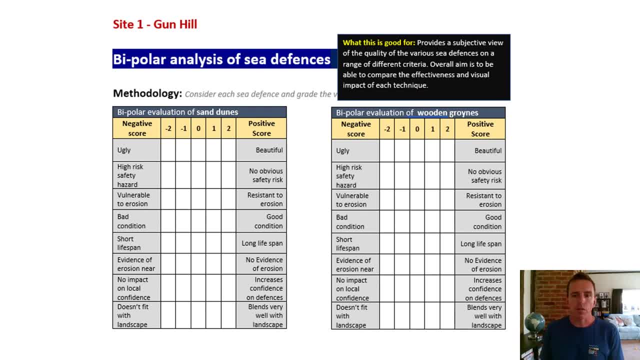 So along the left and right hand side of these boxes you've got a range of criteria ranging from negative on one side to positive on the other, And then in the middle you have this kind of scale. The one that we've got here has got a minus and plus system. 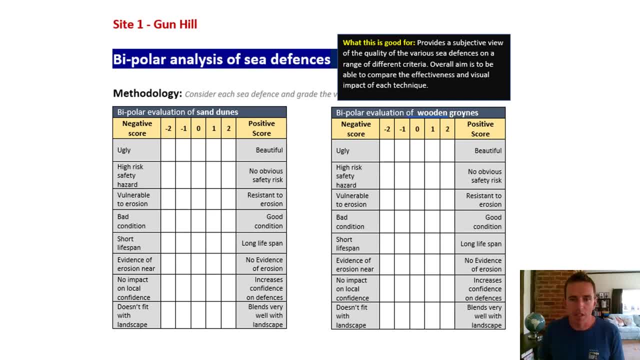 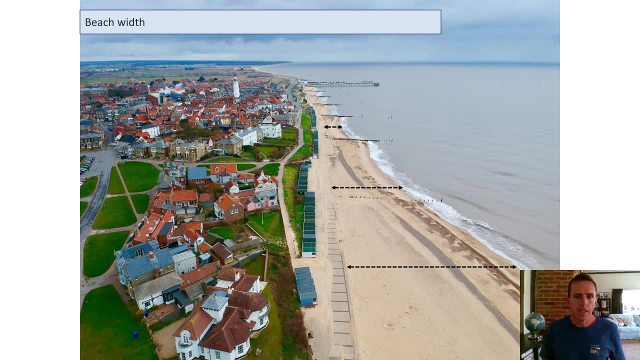 but you might well have a zero to five or a zero to ten system, It's up to you. It's the same scoring system for each of your different methods of sea defence, And then you can compare, using something like a radar graph, which ones are in the best state or which ones are the most effective. 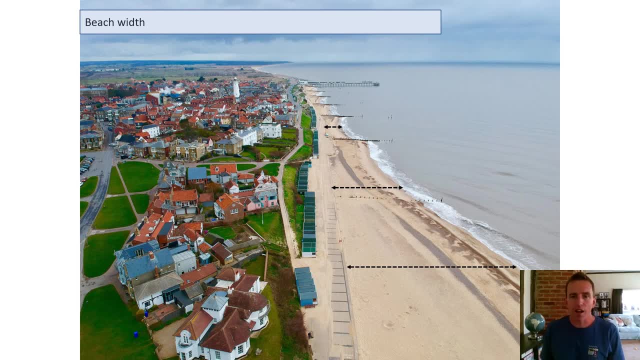 Beach width I mentioned just a second ago. this is a kind of a quicker alternative to a beach profile. with a beach width, You're literally measuring from the shore back to the seawall and potentially doing this systematically down the coastline, As I said, from the pier down to the end of the seawall. 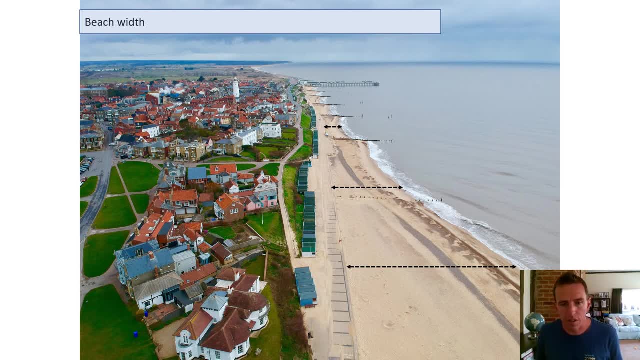 it's one kilometre, so you could naturally do this in 100 metre inflows. The beach width, then, will show you how much the groins are intercepting the sand as it makes its way in one direction or the other, and also show you where transportation and deposition has created a wider beach. 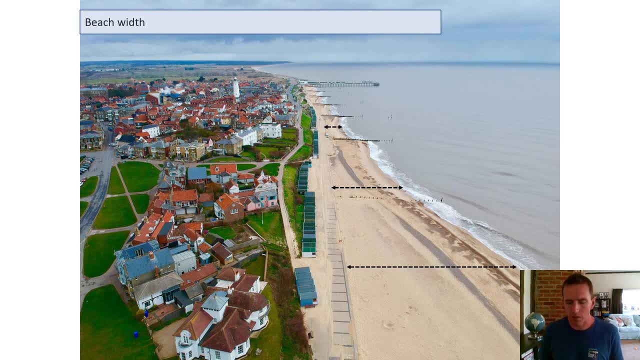 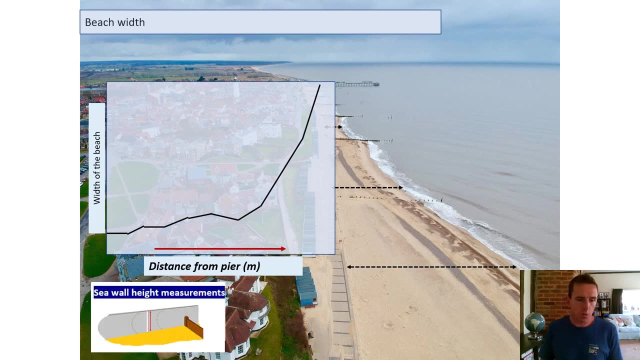 and how the characteristics of the beach change during the course of that steeper. An alternative to beach width or an addition to beach width could be doing a seawall height measurement, And for this one you can literally stand on the beach and just measure the distance. 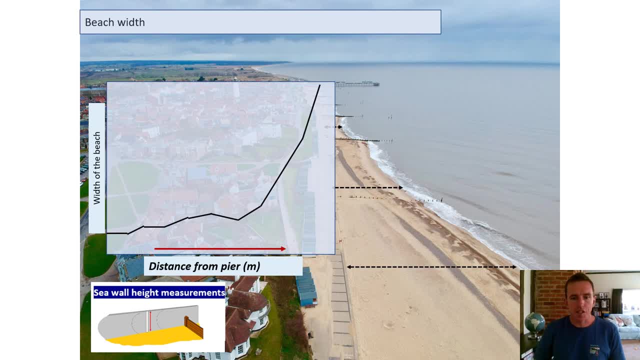 from the sand up to the top of the seawall and again, perhaps do it systematically at each interval. So it might make sense to do a seawall height measurement and the sea beach width measurement in the same location. Ultimately, both of these things you could present on a line graph like this: 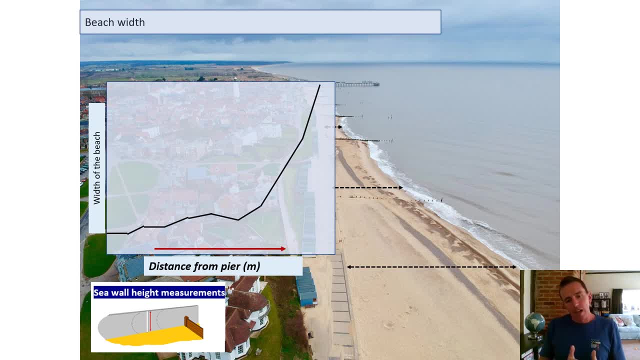 or a scatter graph to show how, as one of those changes, so as distance from the pier changes, whether the width of the beach changes and whether the seawall height changes as well, You could, and this would be good planning if you took ten measurements. 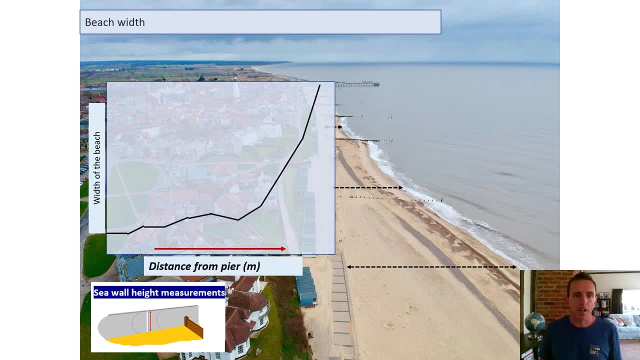 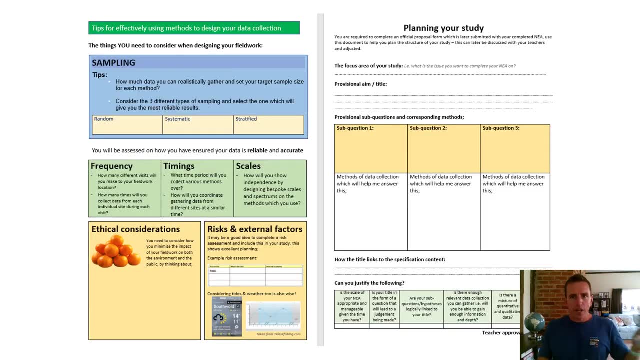 you would then be able to do a Spearman's rank test to show whether a correlation existed, if it wasn't clear from the graph that you've presented. Finally, we're getting there. We're going to talk a little bit about the page that you have here. 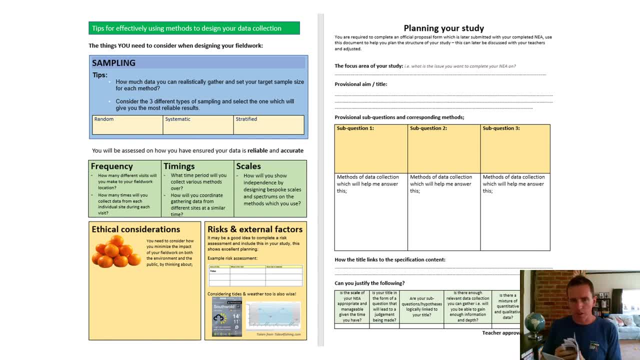 and the page that you have towards the back end of this book that looks like this, And this is just us talking a little bit about sampling. So sampling is one of the things that you're going to need to consider. I'll briefly mention that and I'll briefly mention the other things in this page here. 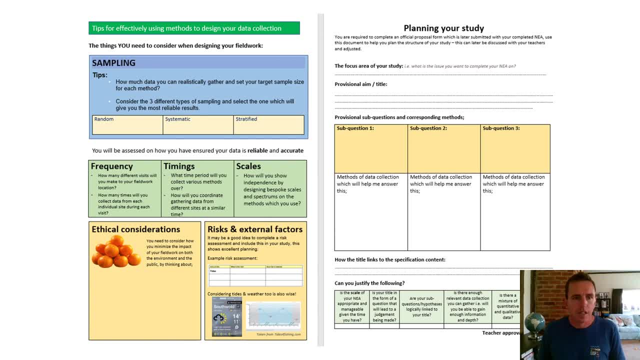 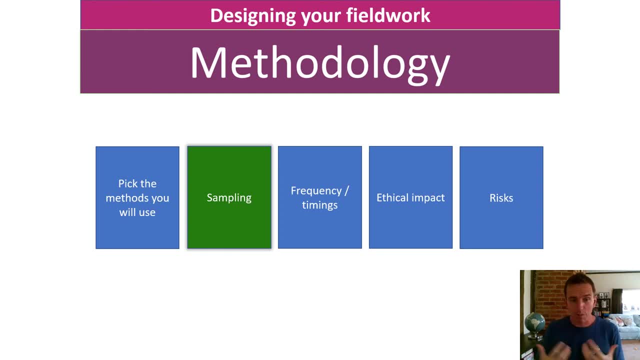 But these are the type of things that your teacher will be able to tell you a little bit more about. In terms of sampling, then, well, we have different types of sampling, but there's also different meanings to sampling. One of the things that we mean fundamentally about sampling is that field work in its very nature. 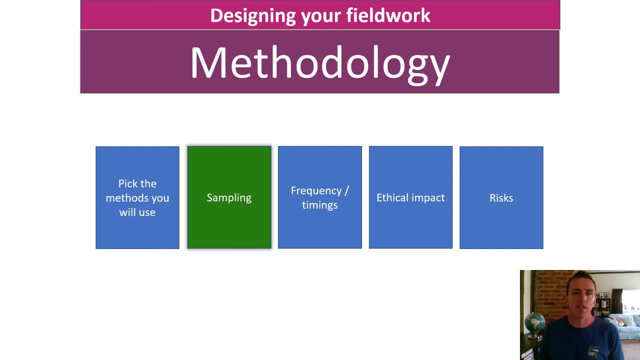 you're only collecting a sample and a limited amount of the overall data that is available. So when you do a study, you're only able to collect data for one day. Obviously, the best studies are the ones that are available for one day. 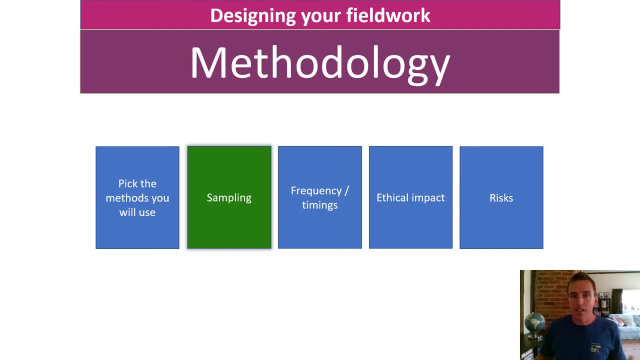 The studies. you know much more data And you know if you can collect data over every single day, then that would be more reliable than one that's just collected on one day. So you are collecting a sample. You're also not going to every single type and sample. 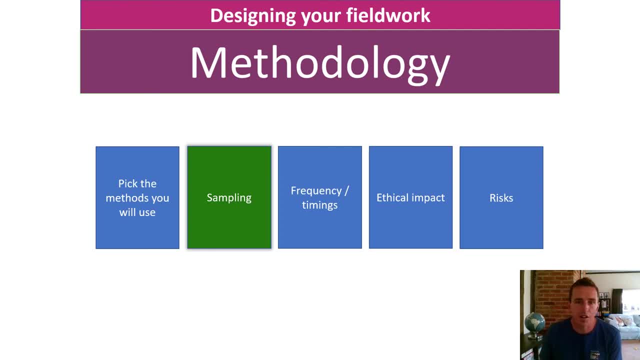 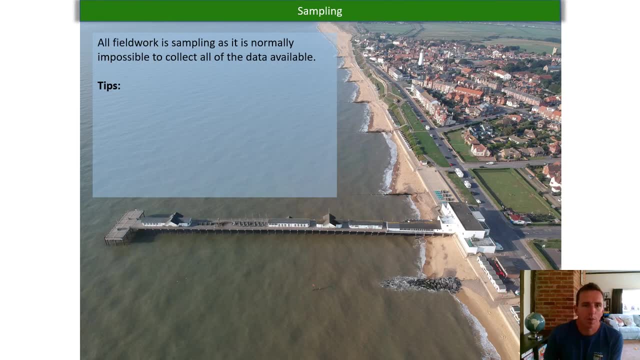 It's not going to be feasible that you do that. So you're choosing which sample sites you go to and give you a good reflection of the total picture. The other thing to think about are the sampling types that we have. So there are three different types of sampling and I'm going to go through them now. 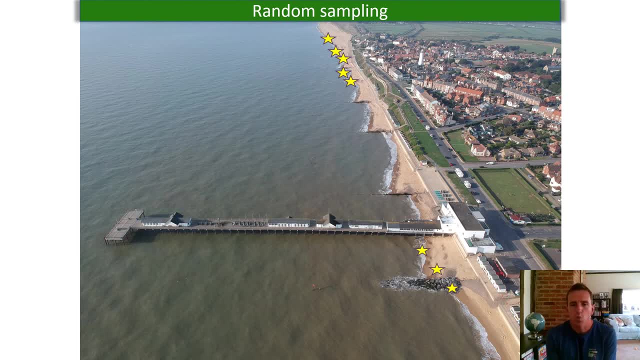 For you, Random sampling is where you can use something like a random number generator to completely remove bias from selecting your sampling sites And perhaps is therefore the least biased sampling For this. then if you were to take that one kilometre stretch of seafront along Telford Shore, 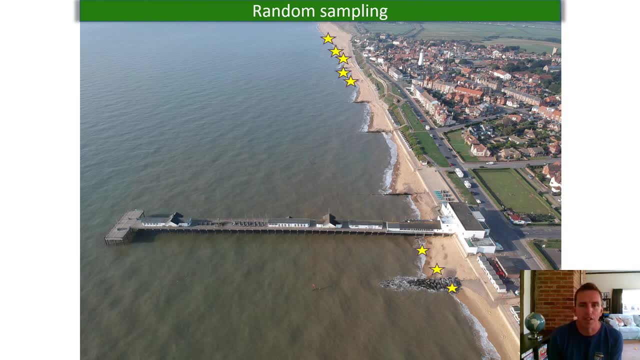 a random number generator might then select five sites that are all towards the beginning of the seawall And the other sites that are perhaps towards the end of it. So you might end up getting an overrepresentation of one particular section and what's called clustering of sites, which isn't particularly useful. 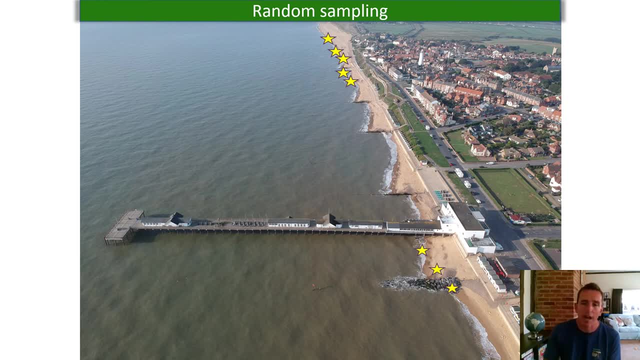 So for most instances random sampling isn't all that useful, but perhaps for some of your surveys it might well be. Systematic sampling is in effect probably the best form of sampling, because it is where you systematically divide up an interval like a kilometre and have 100 metres. 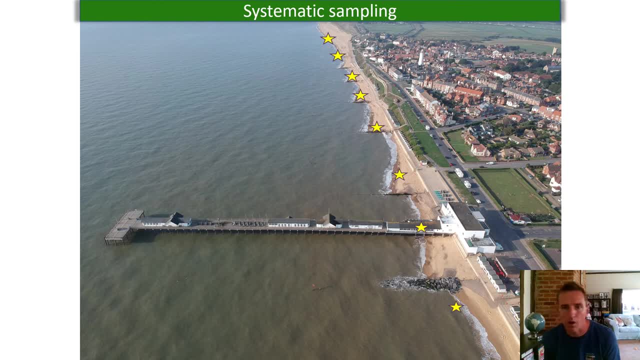 However, the reality of that may be difficult to pull off. It might well be that your 800 metre mark is literally on the pier and you can't physically get to that point, Or it may be that at 600 metres on the beach. 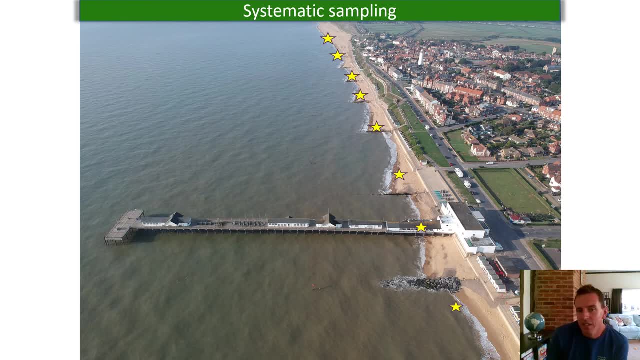 you've got a family that having a picnic and you can't simply go up to them and ask them to pack away their scotch eggs and pork pies because you were wanting to measure the beach in that exact location. So in reality you'd have to kind of move around them and be kind of sympathetic to their situation. 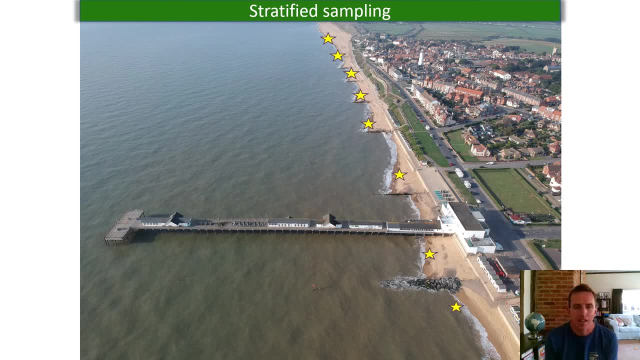 And therefore stratified sampling is often the sampling technique that most people use. This is where you try to kind of use systematic sampling to get a fair representation of the overall area, but you've got the freedom then to move your sites to sites which are going to be accessible. 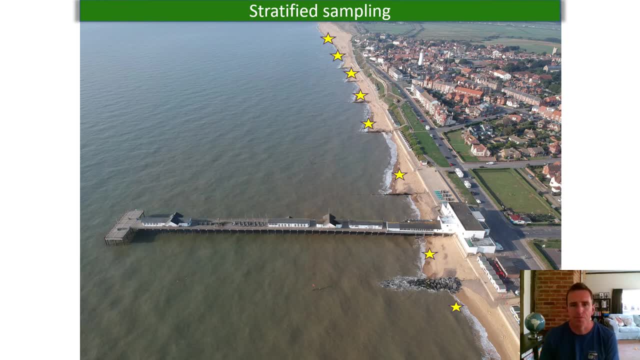 appropriate, safe and better for you to use. So when you're writing up your study, you will have a section called your methodology section, which is where you're essentially kind of writing a recipe or kind of a step by step guide to each of the data collection methods that you are using. 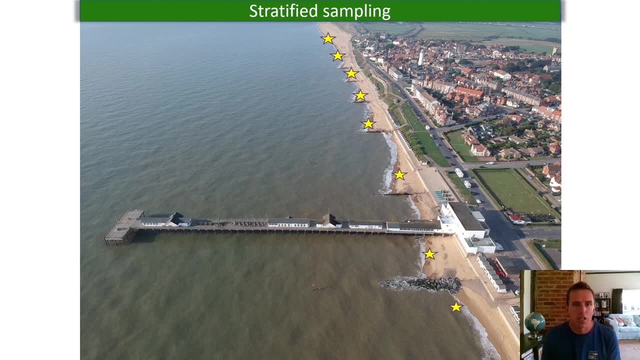 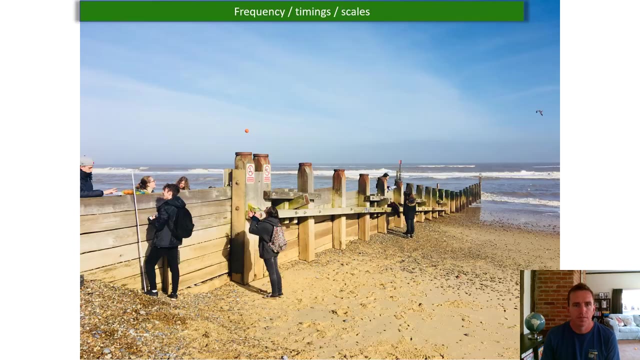 And one of the things that you'll need to do in that methodology refer to the sampling techniques that you used and the sample sizes that you used in order yourself to get the marks for that section: Frequency, timings and scales. What we mean by this is that there's a number of things that you'll need to consider again with your methodology. 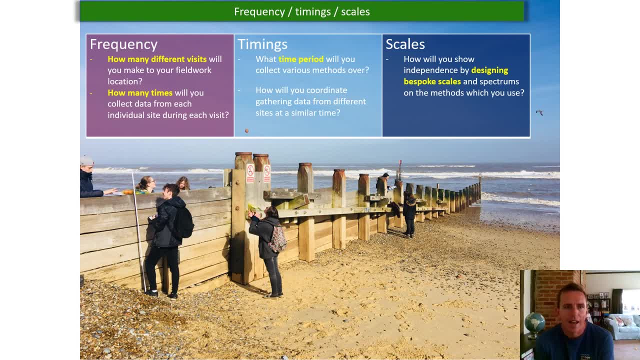 So, in terms of frequency, it's going to be your decision about how many different sites you go to, how many times you might return to those individual sites. very often, teachers are asked the question: how many questionnaires do I need to do? 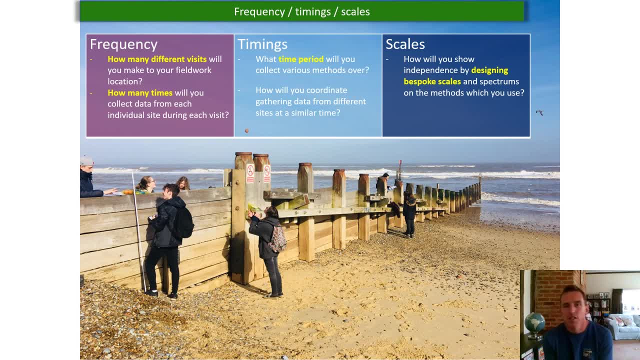 How many streets do I need to go to, How many times do I need to do this and repeat it? How long do I need to time this for? All of those questions can be answered by you, So you're the one responsible for this field work. 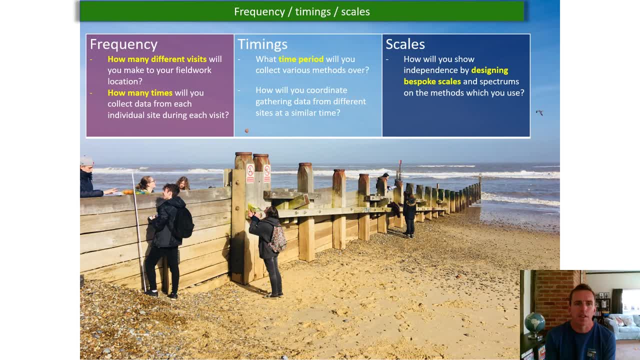 You're the one that's going to have to come up with your own itinerary and to think about where you're going to be and what you're going to do there and how long you're going to be doing it for. So how many surveys is enough? 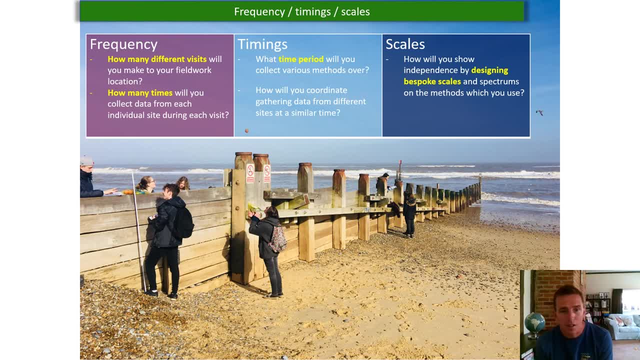 How many streets is enough for you to go to. One of the things that you can do is you can efficiently work with other people who are doing the same methods of data collection of you. There's nothing to stop you sharing the data that somebody else has gathered that's been collecting the same way in which you're doing it. 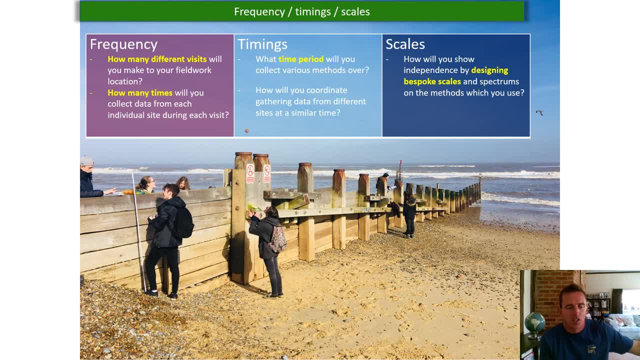 So it might well be that you're doing three beach profiles at the southern end of the beach and you know somebody else is doing beach profiles as well. There's no point in them doing that in the same location as you. Why not send them off to the north? 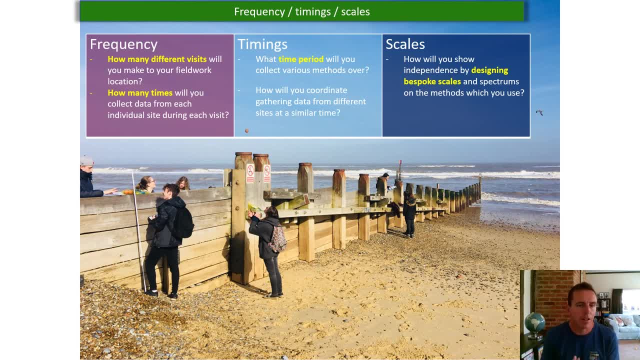 you to the south and then you share your results. So think about how you can be efficient with your data collection. All of these things, then all of the scales, the data collection grids, the way in which you're measuring, collecting your data, has to be your decision. 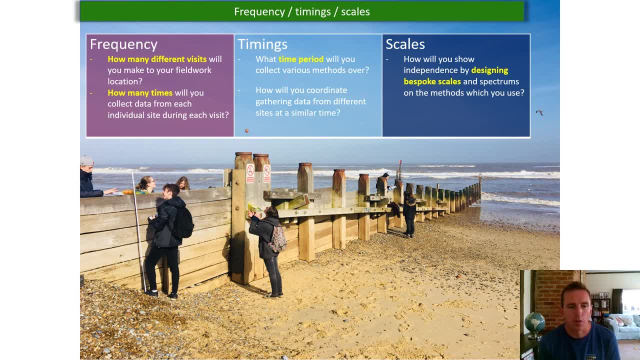 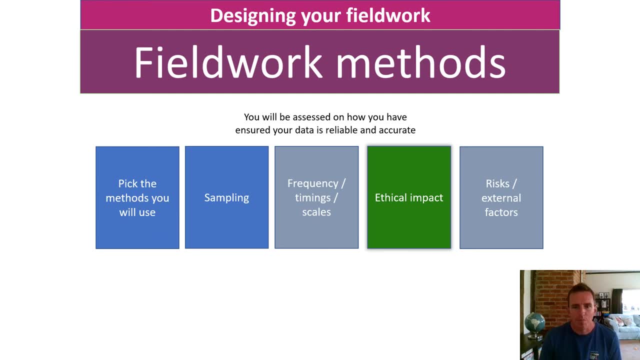 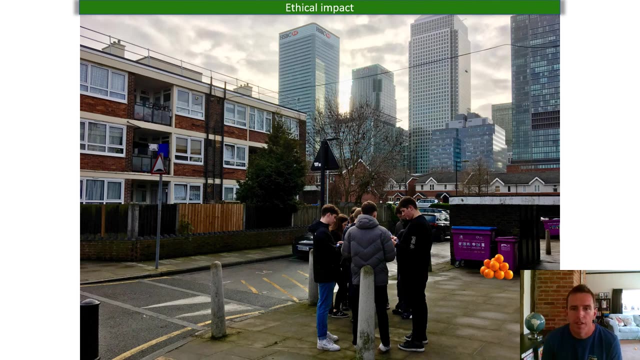 So you're going to be thinking about practicalities of the field work that you do, making those decisions, about the methodology yourself. Ethical impact: This one is one which you perhaps may not logically think about, but in terms of things that you can do to impress the examiners. 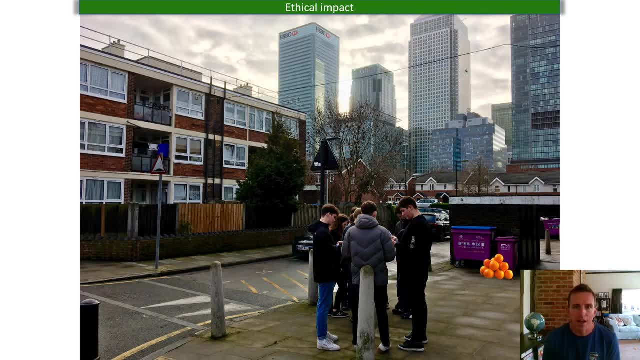 impress the students marking your study. Ethical impact is something that's worth considering, and there are marks available for The field. work that you complete should not have a negative impact on anybody in terms of a member of public or any animal or any aspect of the environment. 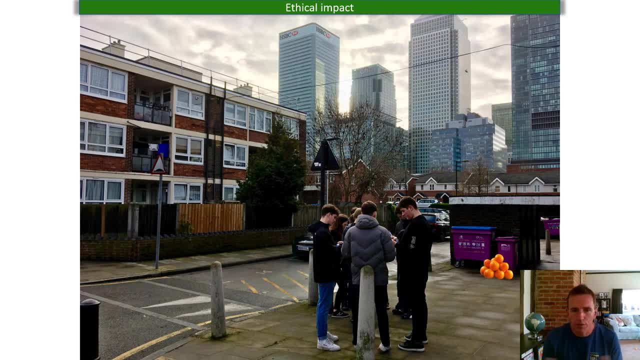 So what you're doing in terms of your field work should have no footprint, should have no negative impact. So you shouldn't make people feel intimidated by completing questionnaires. You shouldn't inconvenience people by taking too much of their time. You shouldn't prevent a business from making sales by kind of 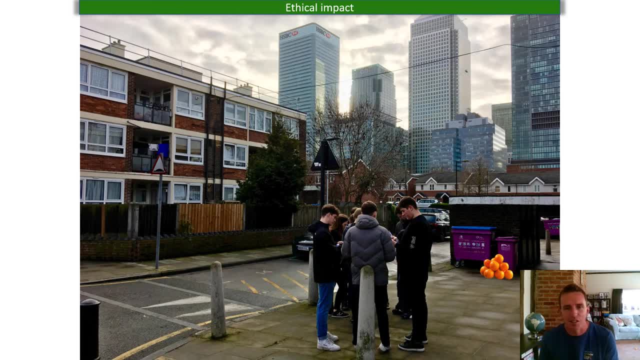 you know doing something to the detriment of that business by standing outside and counting aloud and stuff like that. You shouldn't be throwing things into the sea. that's going to have a negative legacy on the sea. You should be doing things that are going to have minimal impact as possible. 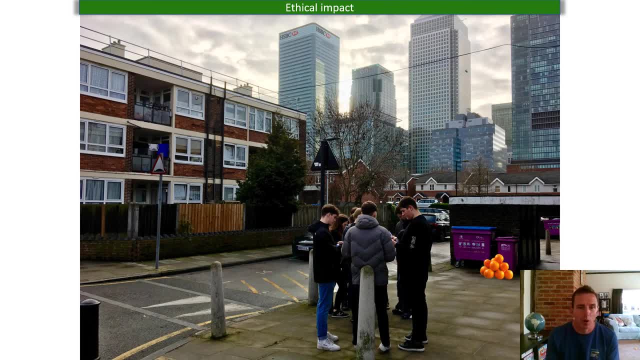 Now you'll be doing these things anyhow, naturally, because that's just how people operate. You know you're not going to do a beach width measurement through somebody's picnic or over somebody's sunbathing towel on the beach. You're going to naturally move your sampling site to somewhere more appropriate and more safe. 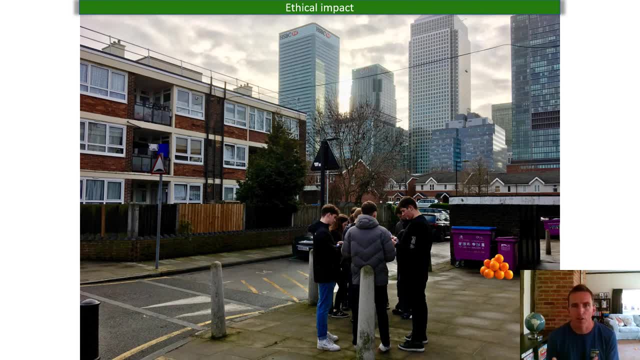 But each of these things are actually subconscious ethical considerations that you're taking. So for any of those things- whether it's using an orange instead of a plastic bottle to do your drift test measurements, or whether it's doing questionnaires online rather than actually going up to people and making them perhaps feel a little bit uncomfortable in this current climate that we're in- 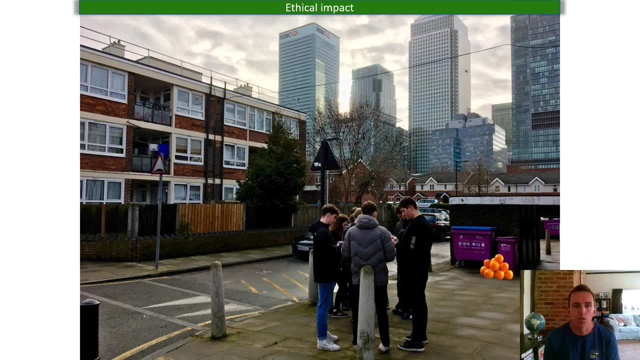 All of those things are considering the ethics of your data collection. So make a note of any of those things, because those are things again, if you can flag them in your methodology, will jump out at the examiners and they'll say: 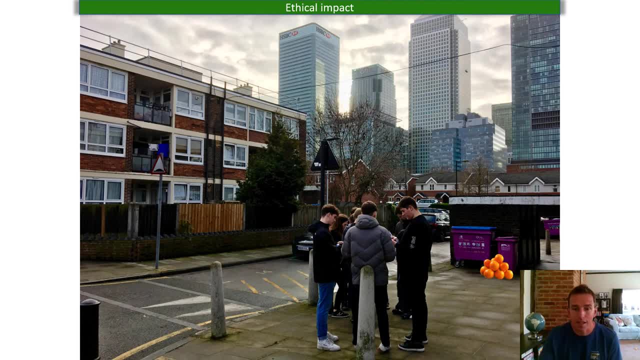 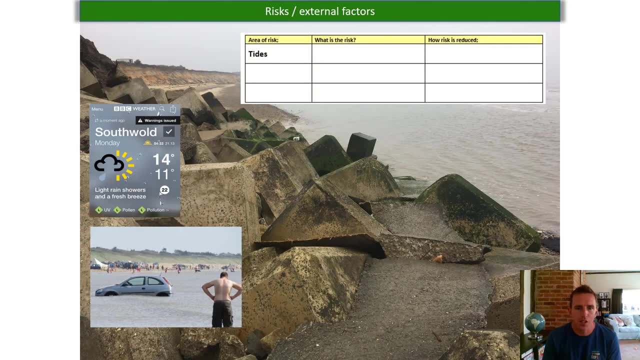 yes, good, They considered the ethical impact of their study and they can get credit for that. Finally, risks and external factors. For this one, then, it's not essential that you complete a risk assessment, Again, like a hypothesis. it's not something that exam boards are insisting on. 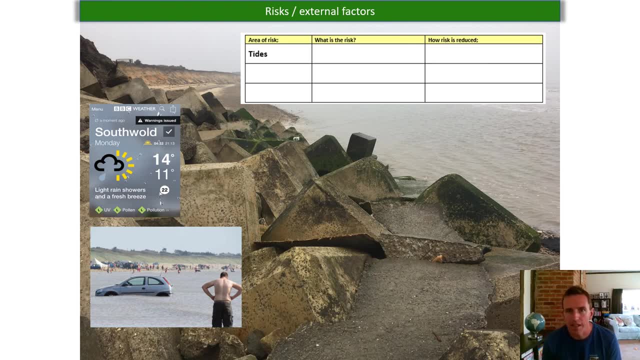 but it does show good practice, It shows good planning and it shows a good awareness that you are, you know, thinking about what you're doing in advance of you completing your fieldwork. So the logical place for a risk assessment to swap into would potentially be your methodology. 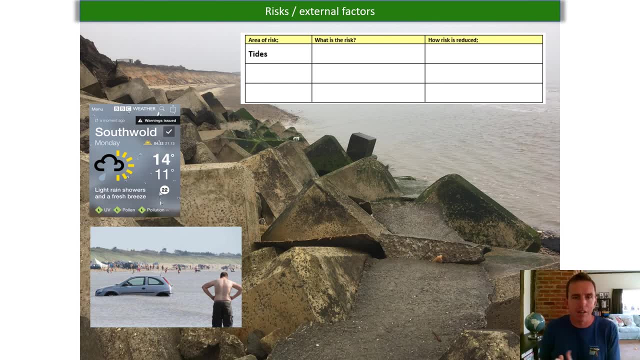 And, essentially, you could have a streamlined, slimmed down version of a risk assessment that just covers the key things that a risk assessment is designed to do, And that is to identify potential risks associated with the fieldwork that you do and then to simply state the measures and the steps that you've taken to reduce the risks of that fieldwork. 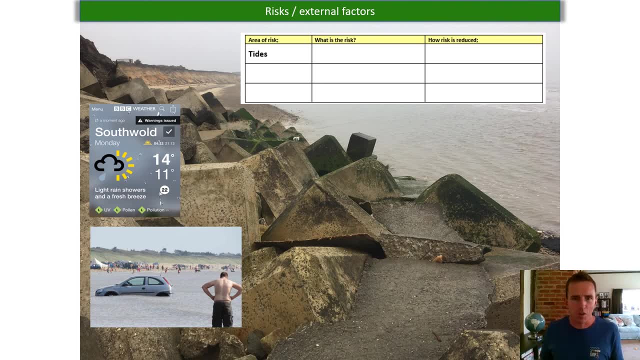 So, for instance, if you're working on the beach, a potential risk is drowning by being trapped by a rising tide. So, to reduce that risk, you have been aware of the tides on the day and you've restricted your fieldwork to sites that are not going to be affected by a rising tide and are working on much wider sections of the beach. 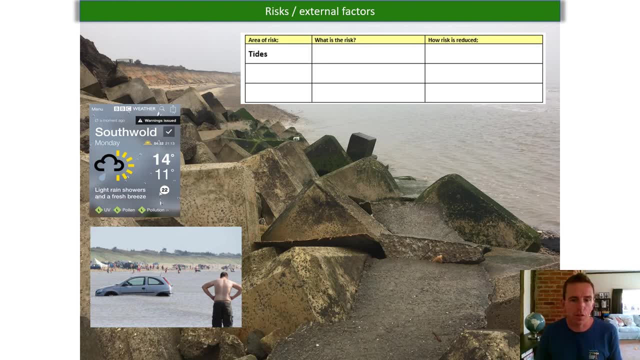 Here at Eastern Balance on the screen here. this is a section that does get cut off by rising tides And that's why I've said here that this is an area that you would not be able to go to unattended. And also you've got things like the algae in the moss you can see on the on the tri-blocks there. 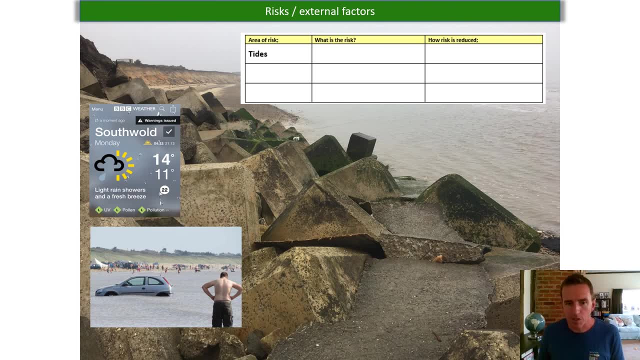 They're a hazard. So slipping on, you know slippery steps, crossing the road, anything like that can be hazards, And you then would be expected to highlight those and highlight how you've reduced those risks. Risk assessment is basically common sense. 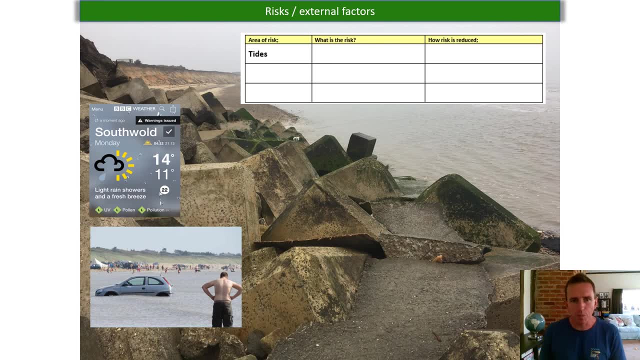 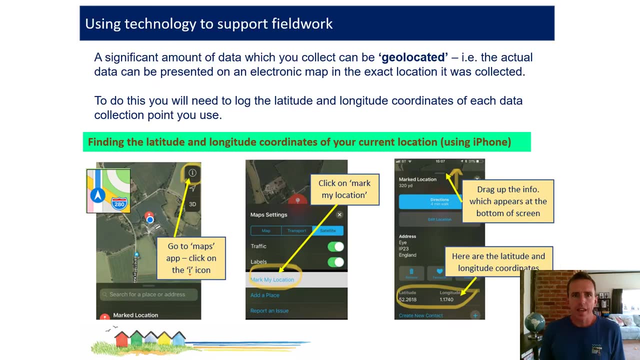 It doesn't have to be mathematically elaborate, But again, it shows good practice and good planning And I'd suggest that for most of you, it would probably be worth throwing one of these in there. Okay, last bits, that we're going to cover is just giving you a bit more of an idea about this thing called GIS and geographical information systems. 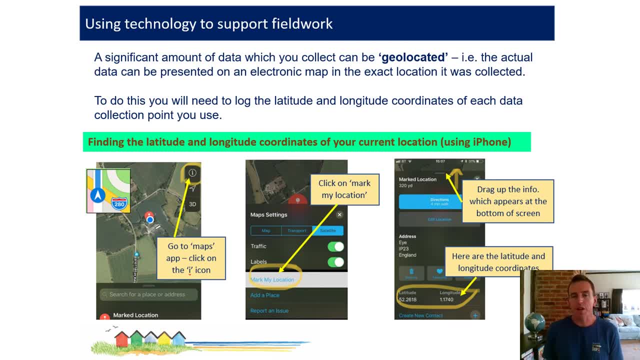 So, traditionally, fieldwork has had a long association with clipboards and booklets And, amazingly, even in the year 2020, we have students up and down the country that are using using clipboards and paper booklets to gather their data. 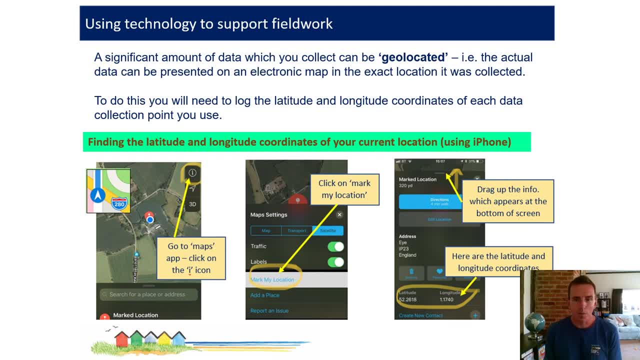 where in their pocket they have these devices that are so powerful, so useful and actually much more practical to use in fieldwork. So one of the things that we are real kind of champions of is using technology in geography and using technology within fieldwork opportunities as well. 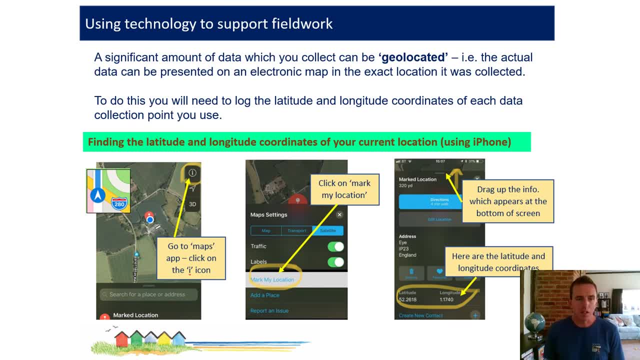 Now, even without using the Jogit app, there's a number of things that you can do just using your phone, particularly gathering the latitude and longitude coordinates using a maps or a compass app on your phone. So I would suggest that you do that and you. 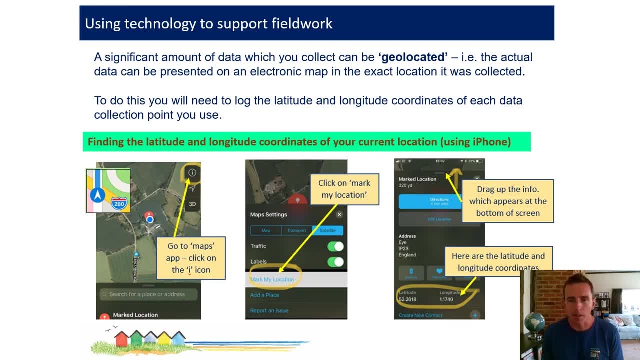 before you come, you work out what methods of data collection that you might be using might be useful to geostamp and work out how to gather the latitude and longitude coordinates from your phone. Some instructions here for the iPhone on Google Maps. but you will find that if you just type into Google and you've got an Android device. 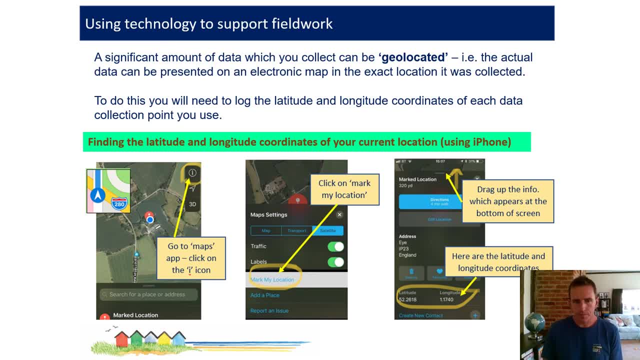 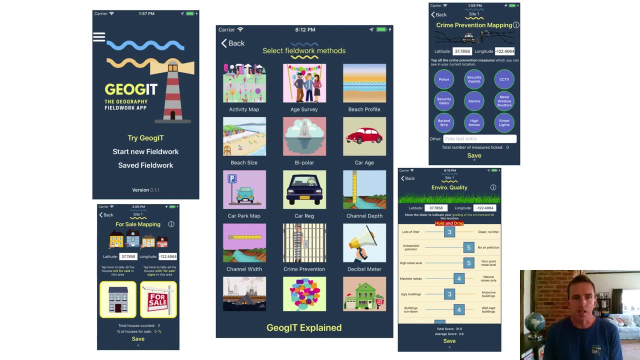 it's very easy to work out how to do it on any phone. So Jogit is the, the fieldwork app that we have designed specifically for geography students in the UK, And there are a number of different individual methods, things like a decibel meter app that you can get. 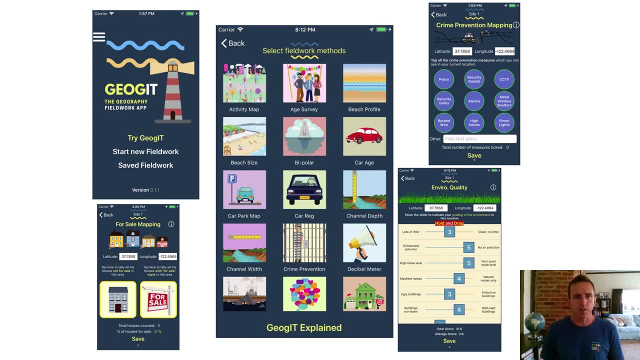 There are things that you can do with sketch where you can annotate photos. There is an ArcGIS survey 123 map, which is quite good for things like questionnaires and stuff like that, But there's nothing specifically that has been designed with geography students and geography fieldwork in mind. 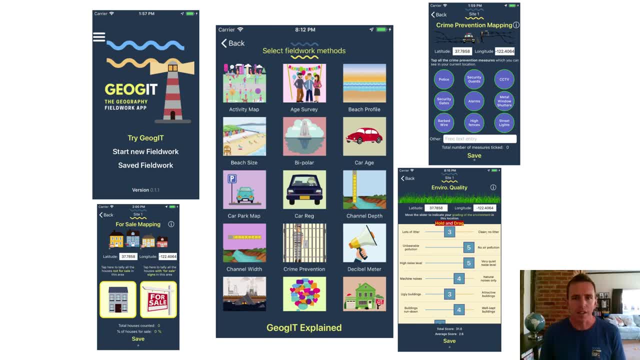 you know, as the forefront of those assessments And we felt it's time that actually we started trapping clipboards and making data collection much more modern by using the technology that we have on our phone. So we spent a long time developing Jogit. 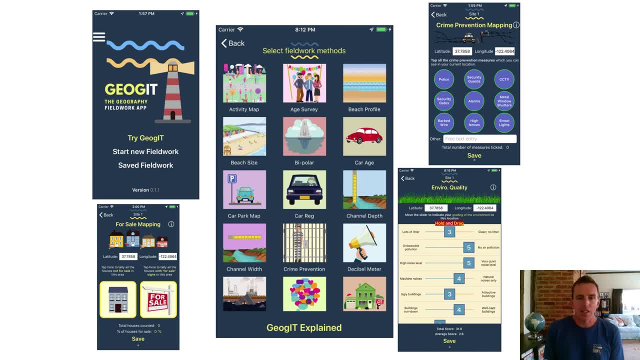 We're really happy with what it now does. It has 35 different methods of data collection built into it And you can trial all of these first by clicking on try Jogit and getting familiar with these methods. You can click on the little eye on the screens that you can see there for each of those. 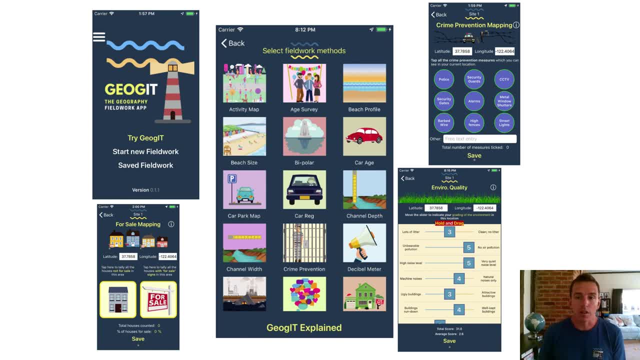 Those individual methods, which gives you a bit more information about how you can conduct that fieldwork and how you can present it as well. Some suggestions is how you can present it, But ultimately, when you're ready, you can click on the start you fieldwork button on the home page there. 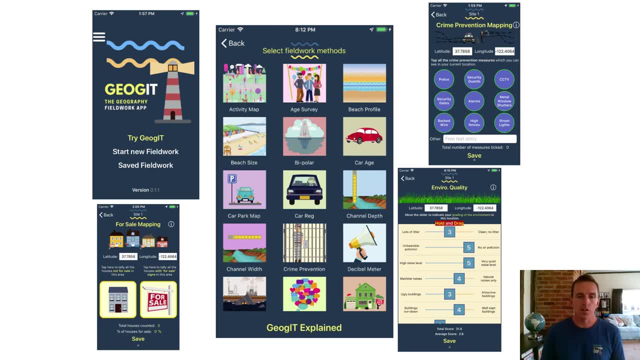 You select the methods of fieldwork that you want to use. You then select the amount of sites that you want to visit, and you then ultimately start collecting your data, but using your phone. What happens is then behind the scenes. is you have? 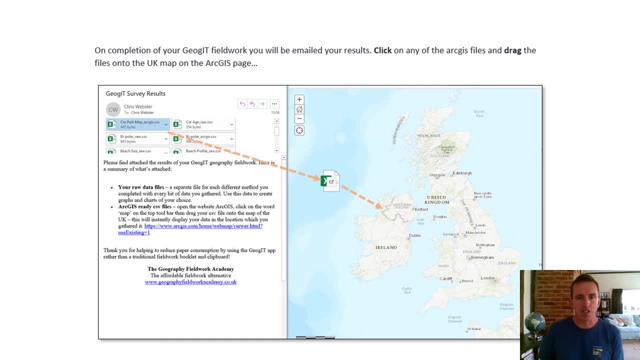 Several different Excel spreadsheets that are then built and added to as you collect your data. So your spreadsheets that you would normally manually fill in are being filled in as you go on an Excel spreadsheet behind the scenes and Jogit Ultimately when you finish your fieldwork. 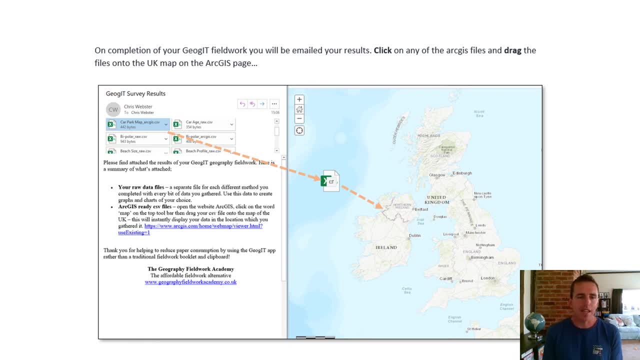 you can click on send me my results and a email is generated to your email, and you then receive an email like this and attach that email And that will be your Excel spreadsheet data. You're simply able then to drag that data onto a web page called ArcGIS. 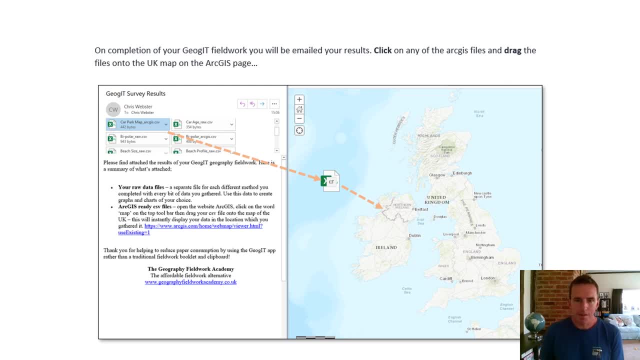 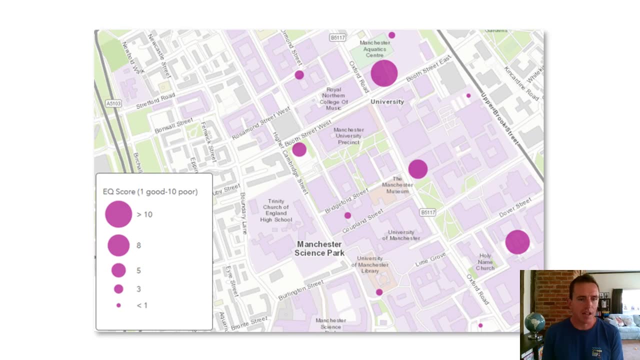 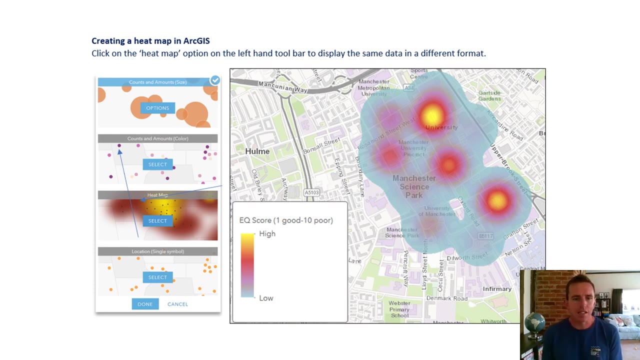 which looks like this map to the right here, and very quickly. Your data is then translated into proportional symbols and located in the exact location where you gathered that data from. You can then change and adapt and manipulate that data into various different formats. You can change these kind of base maps that you've got. 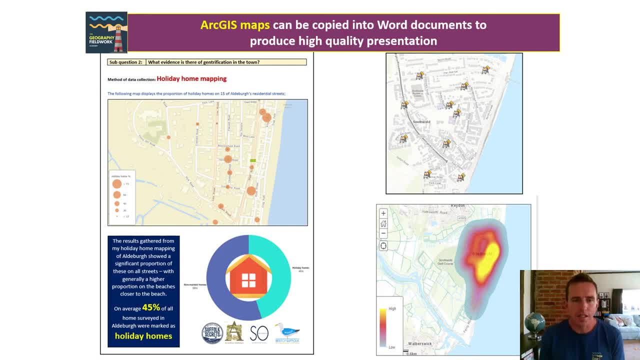 And you can then crop and copy and paste that map that you have made, So that kind of customizable, bespoke, you know homemade GIS map that you've made. you can copy that into a Word document and you can use it to create very modern bits of base presentation like we have on the screen here. 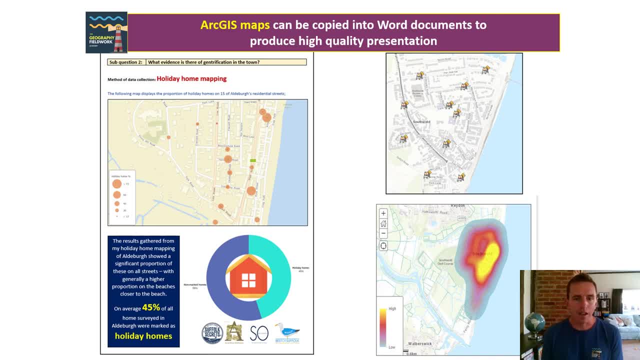 This person has done a GIS map to represent holiday home mapping for an examiner. That's absolutely spot on: high quality presentation, modern techniques of collection using latitude and longitude, using GIS and doing a number of high level things that they would look at and say. 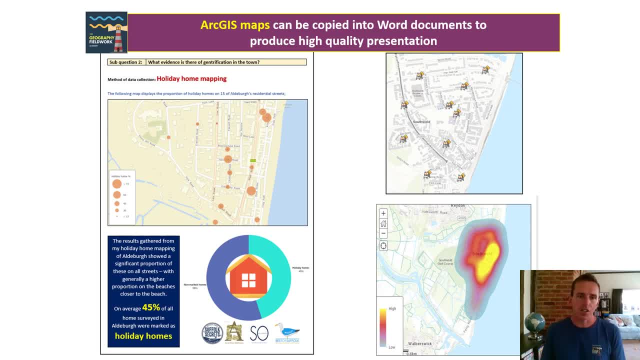 fantastic way better than a bar chart, for instance. So getting familiar with ArcGIS would certainly suggest- and in the back of the book that you have got here you've got a double page spread- as the step by step guide is to help produce a map in ArcGIS. 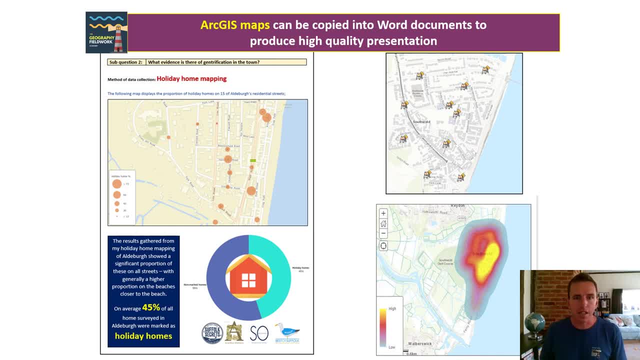 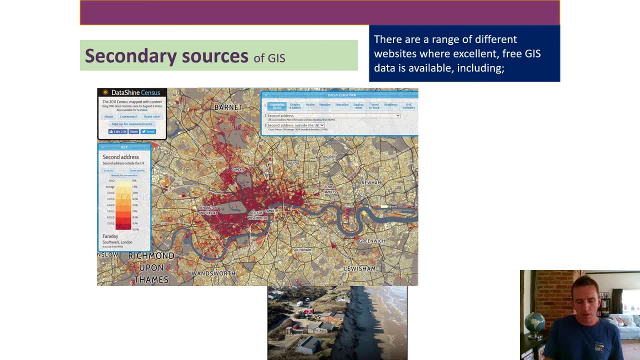 And it really is dead easy, particularly if you've used Jogit to collect your data. Finally, the last bit that I'm going to go through is just some recommendations before you come about doing some free reading and looking at some useful technical resources. 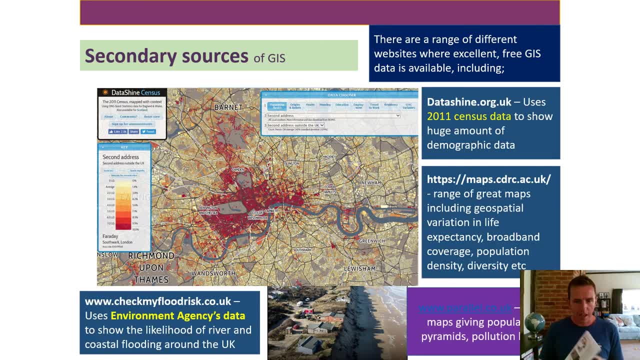 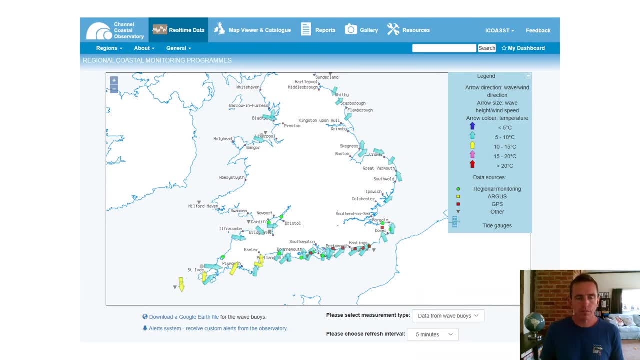 I'm going to skip through each of these because they're in your book anyhow on this page, but each of these websites have their own GIS maps that you're able to access and extract and use, and I'd recommend visiting them, particularly the ones that are going to be relevant to your study. 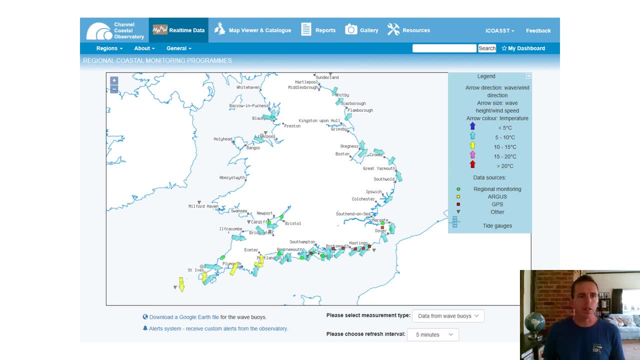 A couple of other ones that didn't make it into the book, but it's one called Channel Coastal Observatory. You're doing a longshore drift test. This, in particular, might be a useful web page. This has got live weather data taken from the buoys that are in the water around the UK coast. 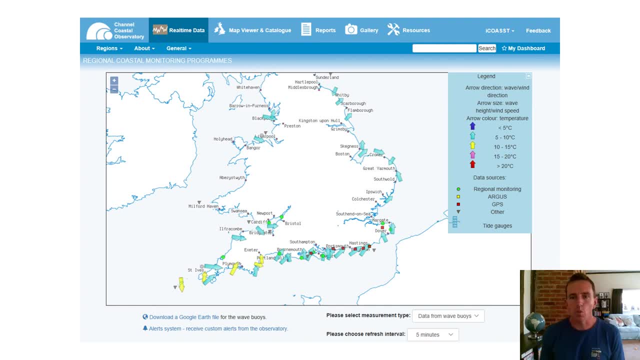 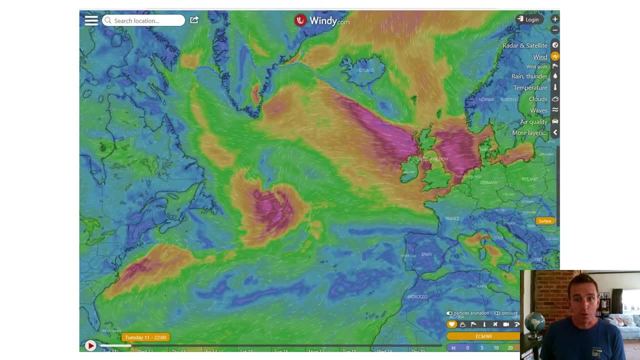 So you can get very accurate readings of wind direction and wave power and things like that from these buoy readings. Another good one for longshore drift test is a few actually is a good website called windycom and that has a number of different, different maps. 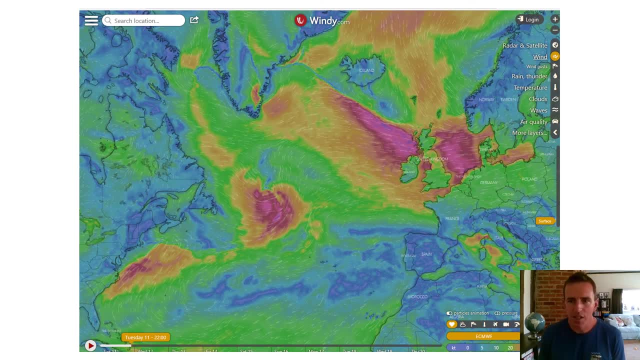 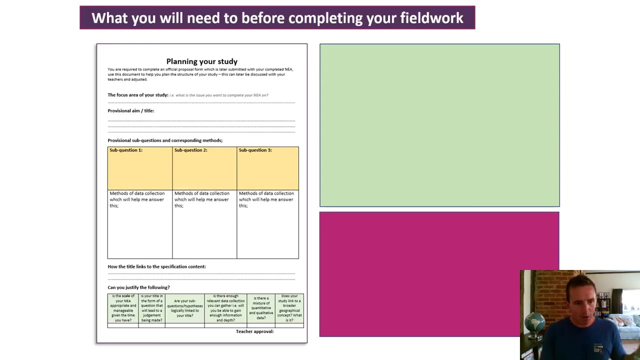 including, obviously, wind patterns, live wind patterns, but also swell and wave patterns too, and it can also a lot of weather and systems as well. That might be useful depending on what you're doing. So pretty much there, What an epic We're getting towards. two and a half hours worth of the video. 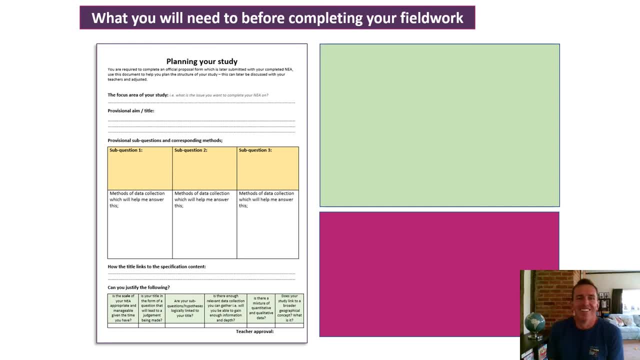 If you've watched all this amazing effort, I'm sorry that I've droned on so much, but by doing this you have saved yourself pretty much, which would be a day's worth of a course that we would normally do in Southwold. 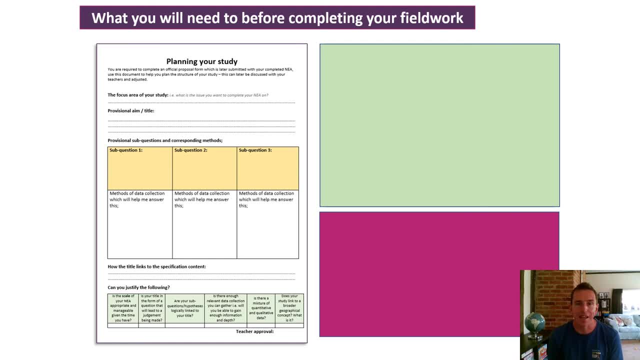 You've also got the tour of Southwold, So that would be your first day really. So you've saved yourself that and what you have now got is a setup where you hopefully got much more of an idea about what the NEA involves and what you can do physically in Southwold on your NEA. 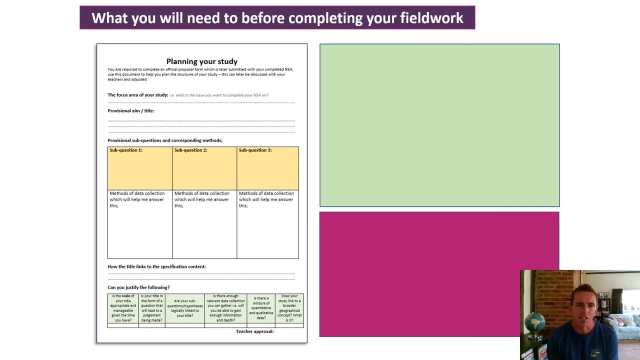 Ultimately, this is your challenge, then, isn't it Over the next couple of weeks, is to start planning your study, which is going to be referring back to that template that we looked at for the Holy Grail thing that I keep saying: The title, the sub questions and the methods. 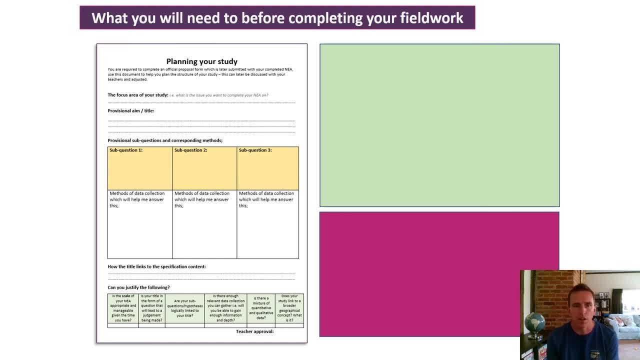 It's that kind of foundation that is going to be important for you to develop and to try and work on over the next few weeks. But if you can get that done then, as I said a few times, you can have confidence that when you arrive in Southwold. 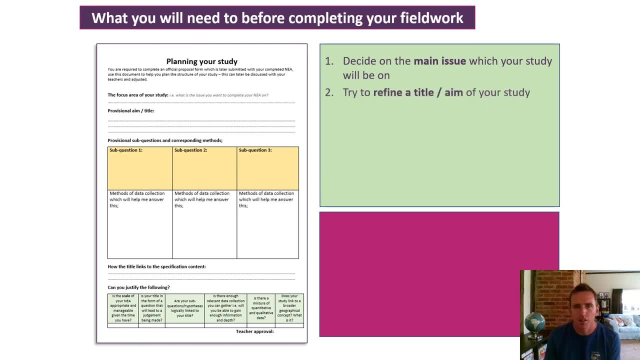 you're ready to go. First thing is deciding on your issue, then picking your title or the aim for your study, Coming up with three supporting relevant sub questions that are going to help you answer the aim that you've set, and then trying to choose at least two methods of data collection. 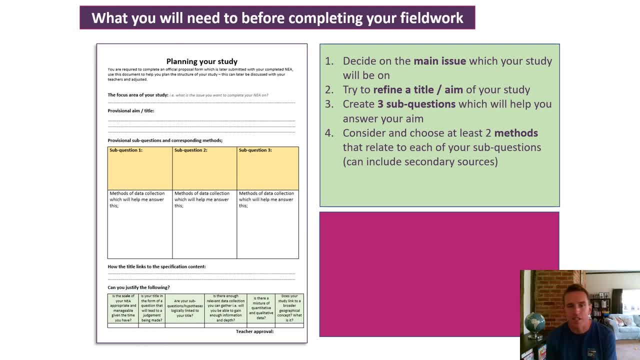 including a mixture of secondary and primary sources and hopefully qualitative and quantitative, to help you answer your questions. Ultimately, finally, we're looking for you to come to Southwold on the day's field work, that you have ready, to hit the ground running with your own booklet and your own itinerary and your own. 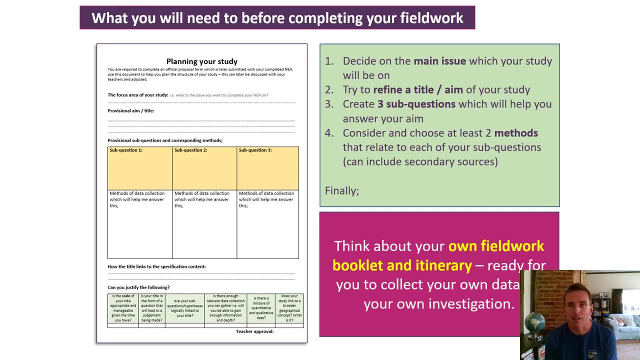 plan of what it is that you need to do to make the most of your time in the town where you need to go. Obviously, you can ask me any questions on the day in terms of demonstrating methods that you might want a little bit of help with or perhaps directing you to particular places that may be useful for you. 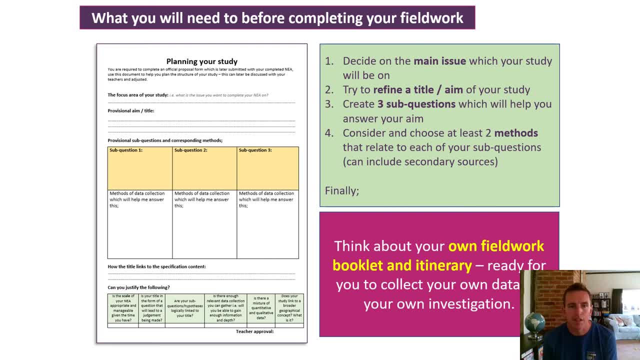 In advance of you coming as well. definitely contact me if you need to ask any specific questions about your field work. I'm more than happy to reply, give you some guidance, if I can, But what you've got to try and do is to arrive in Southwold. 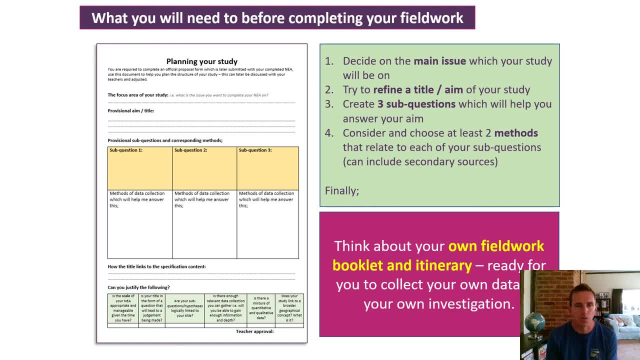 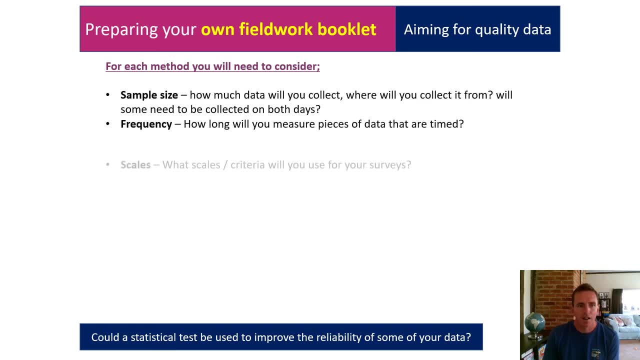 ready to hit the ground running, to get out there and collect your data and make the most of that time Before you come. these are the key things, just to reiterate again and I'll leave these up here. Sample size: it's going to be up to you. 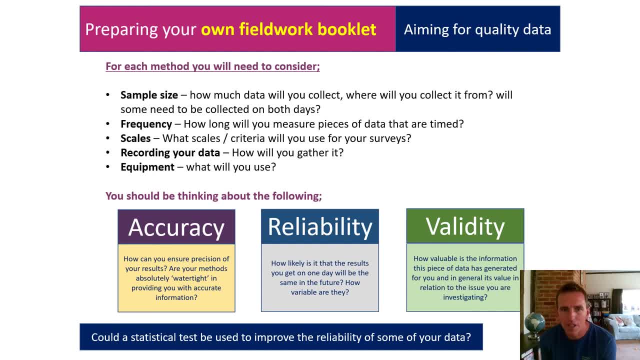 Frequency scale, how you're going to record your data, what equipment you're going to use. if there's anything specific that you're not sure I will have, email me first. If I haven't got it, I'll make sure I do get it so you can use it in Southwold. 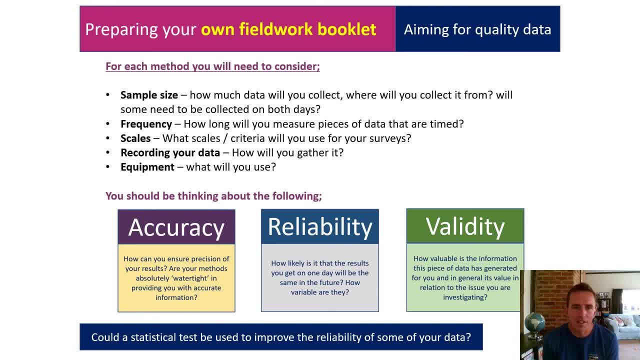 Thank you Ultimately, with your day of data collection. these are the three words that you're trying to have in your mind the whole time. Is the data collection that I'm completing, meaning that I'm creating accurate results? Am I getting accurate results? 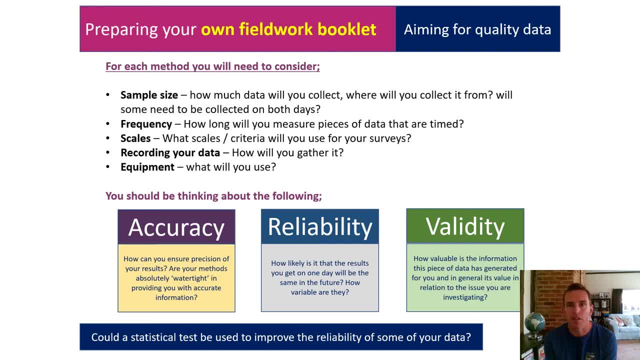 How am I ensuring accuracy? How could I perhaps make this method of data collection a little bit more accurate? And if that is not possible, maybe do I still need to make a note of it so I can talk about a limit later? How can I enhance the reliability of the data that I'm collecting? 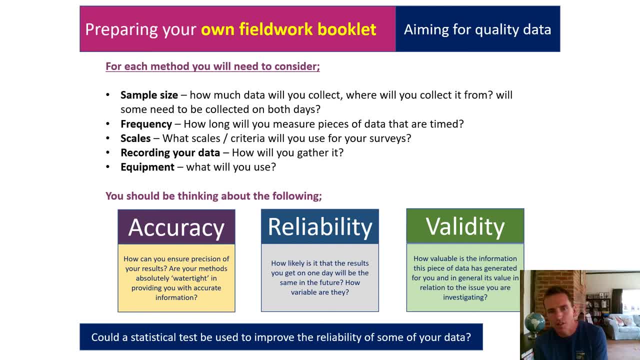 What could I take Extensions, could I do to potentially make my data more reliable And, ultimately, how valid is it? How useful and reliable and good overall is this data that I'm collecting? Is it going to be useful and valid to the questions that I've set and relevant to my study?